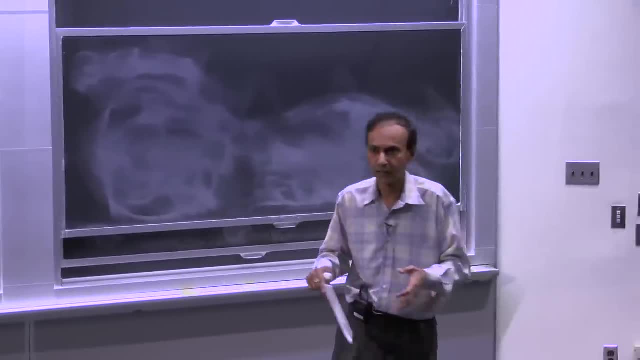 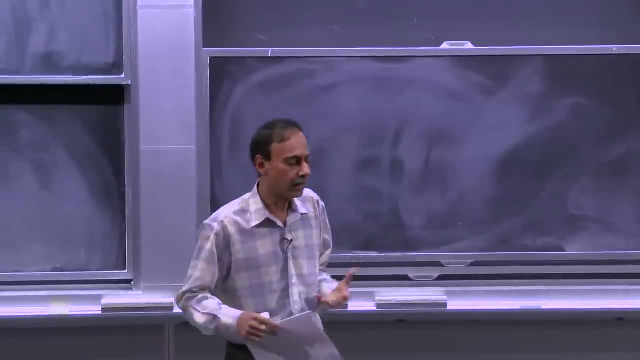 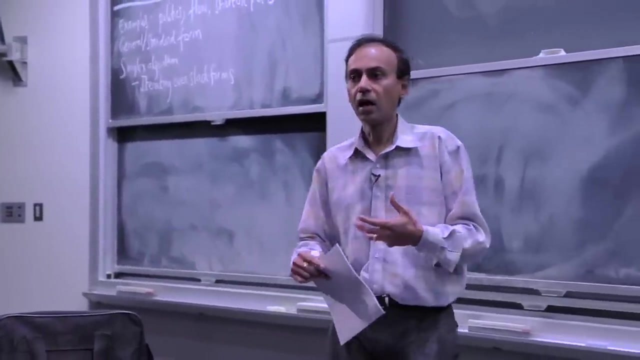 programming are a heck of a lot more complicated than max flow, And you can imagine that that would be the case because it's a more general purpose and more powerful technique. The history really is that it was an open problem Up until 1979, people did not know. 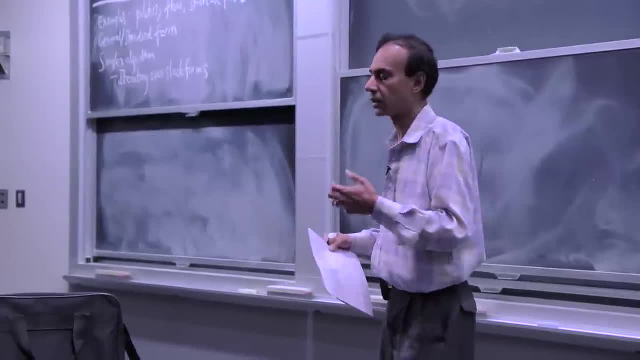 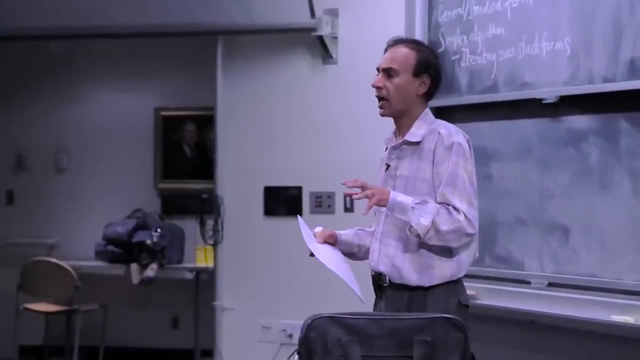 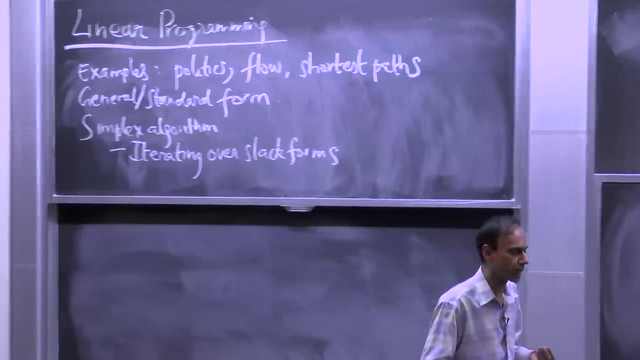 if linear programming was polynomial time solvable until Kacian came up with this ellipsoid method, And then there's been progress since. But the algorithm we're going to describe today and execute on an example input is the simplex algorithm that runs, in worst case, exponential time. 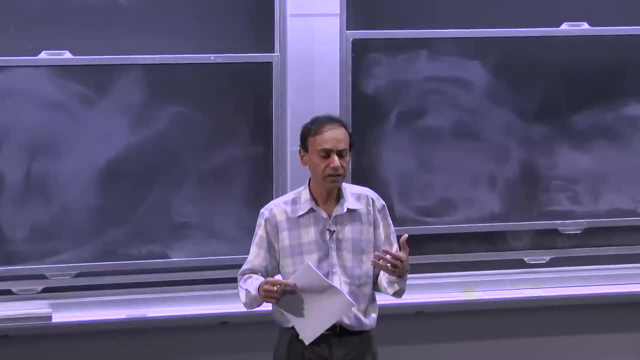 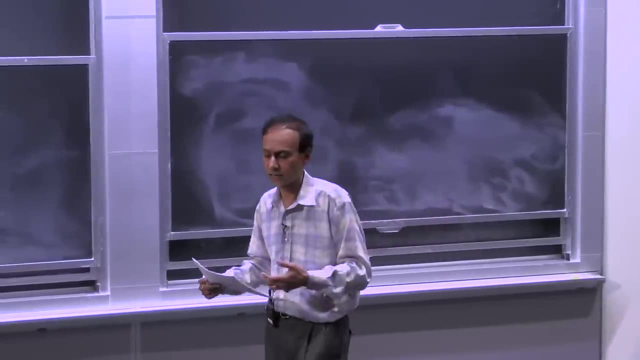 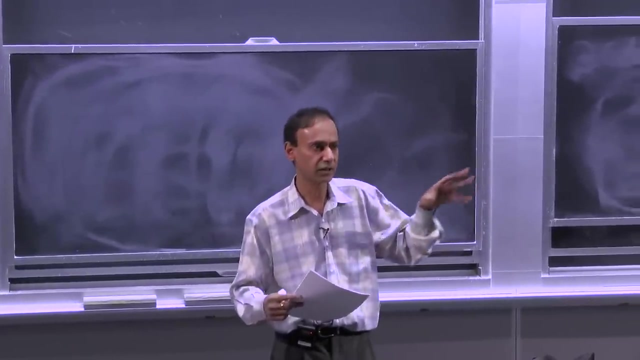 But it's very efficient in practice and it's held its ground even with the advent of more efficient, from a theoretical sense, polynomial time algorithm algorithms, namely the ellipsoid method, which actually is not that efficient in practice, and new interior point methods. 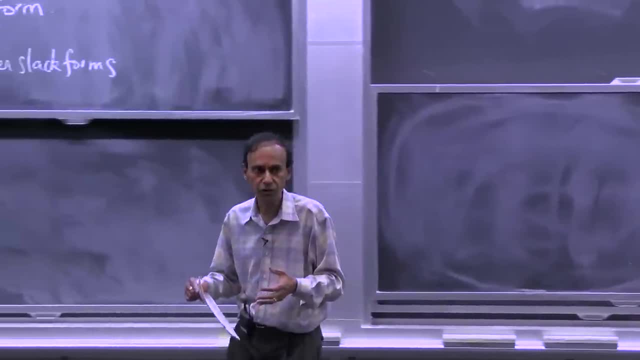 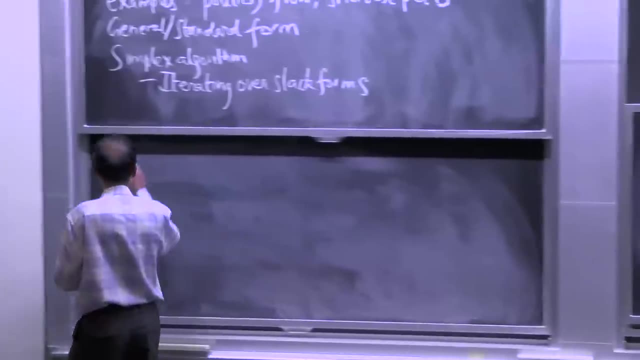 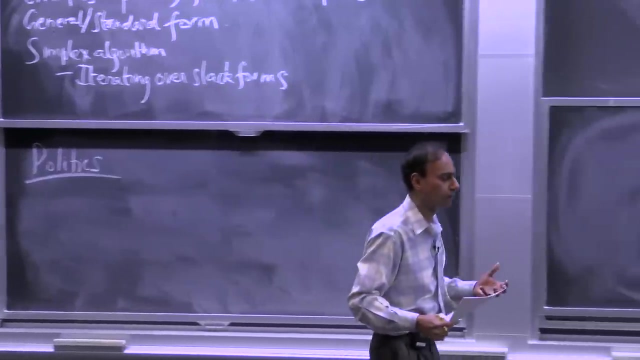 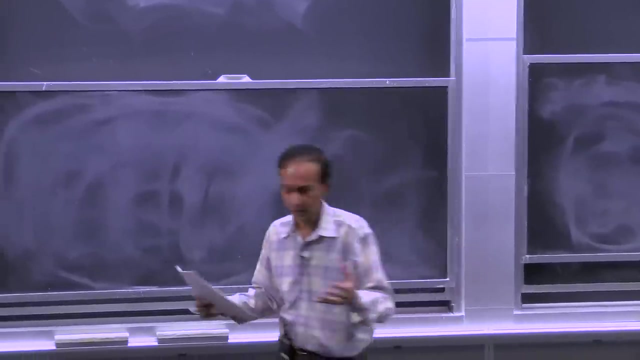 So a little bit of context. Let's just dive into an example of optimization in the context of politics and see how you could formulate this particular problem as a linear program. So how does politics work? You buy elections, So you don't want to spend a lot of money. 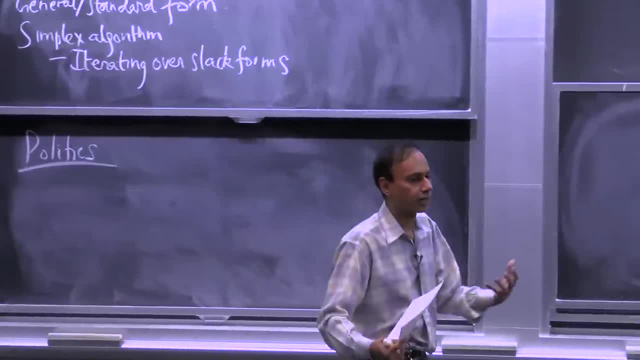 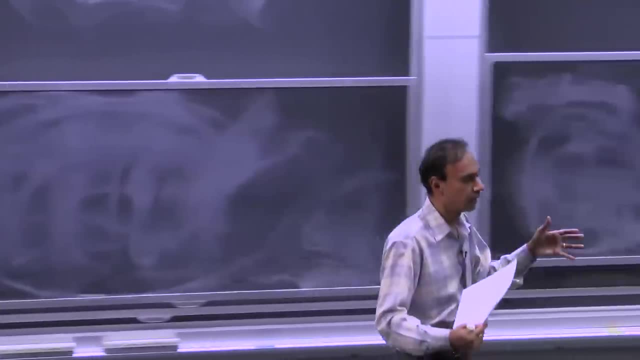 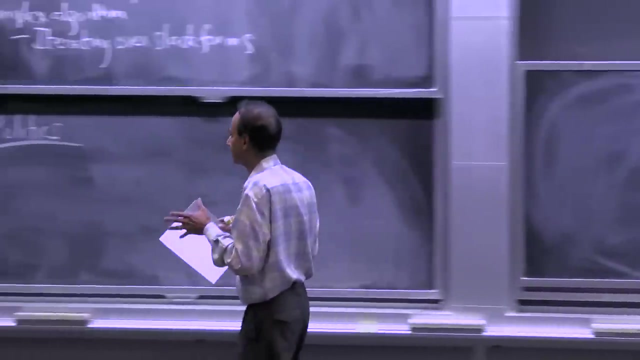 So you want to minimize the amount of money that is required to buy an election, And the way you buy an election is well, campaign. but you advertise And it doesn't matter. Facts are irrelevant, As long as you get to the right demographic. 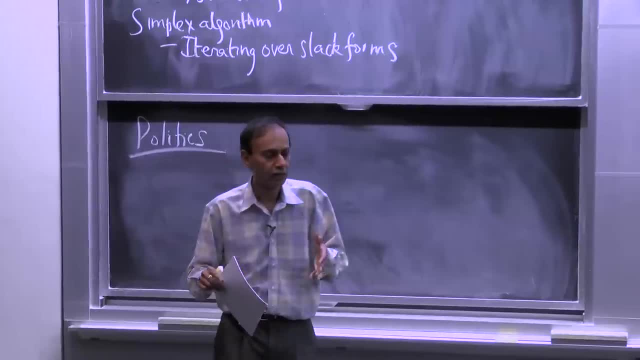 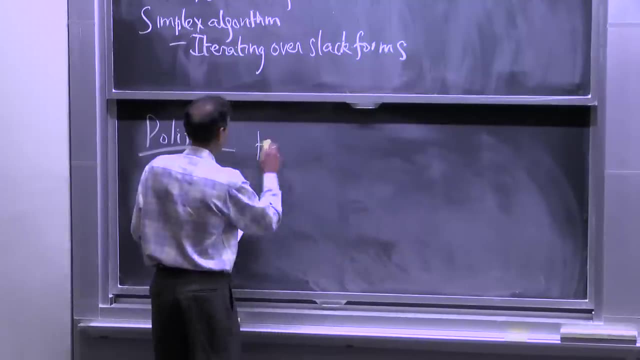 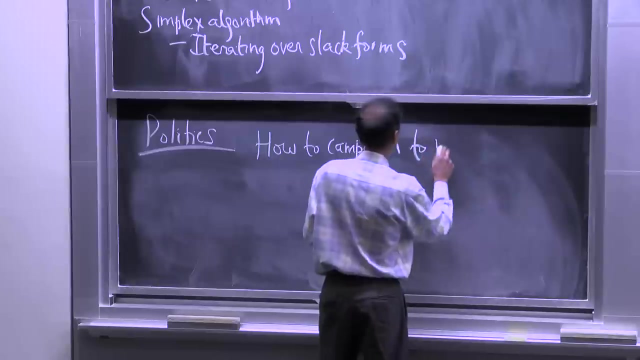 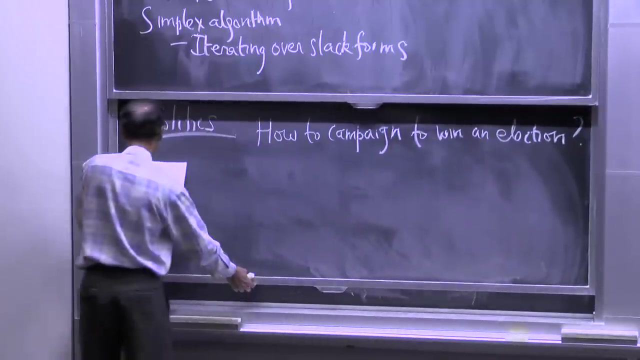 with the right message. let's assume that you're going to win the election. So that's our mathematical abstraction of campaigning and politics, all in 30 seconds. So how to campaign to win an election And, as I said, we're going to advertise. 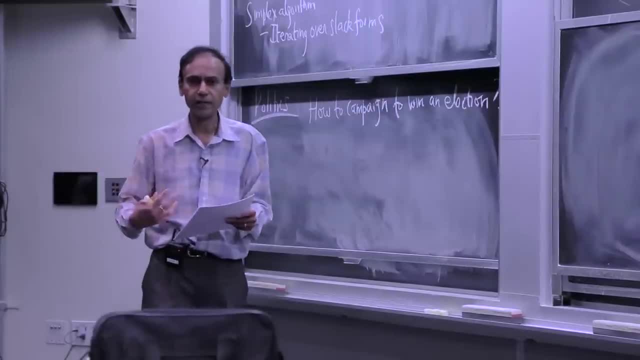 but you do have a little bit of work to do here. That's why you need your campaign manager. So you're going to advertise, So you're going to advertise, But you do have a little bit of work to do here. That's why you need your campaign manager. 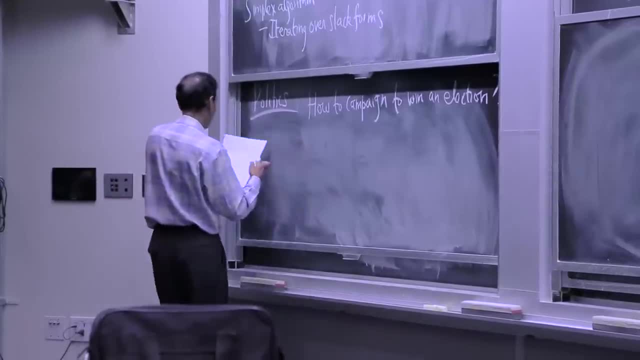 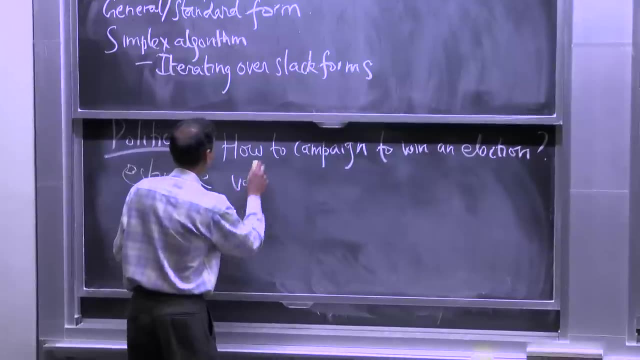 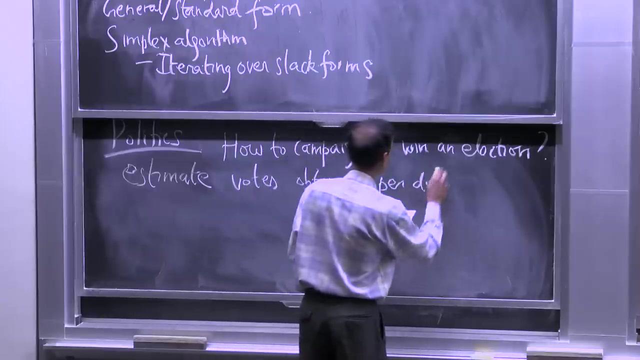 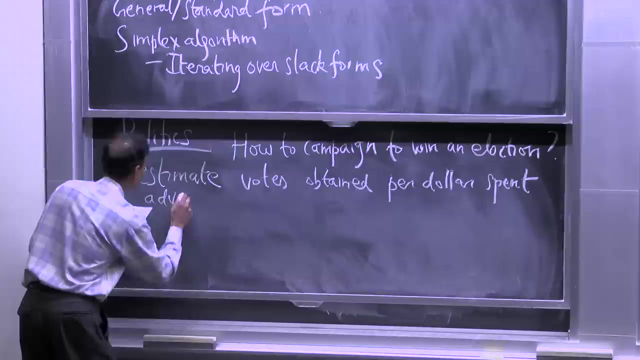 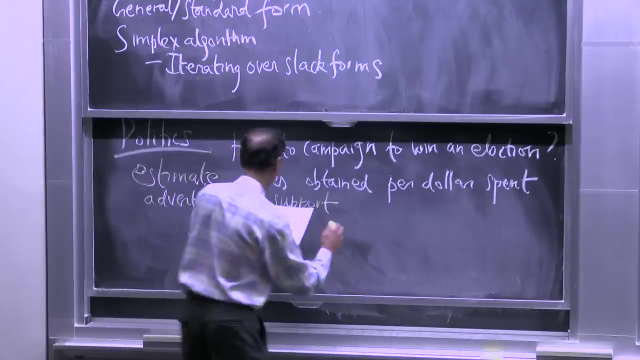 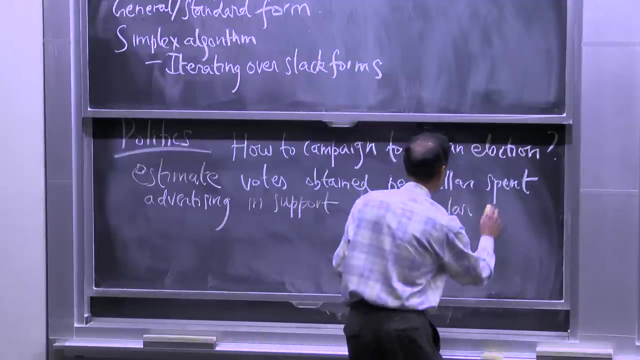 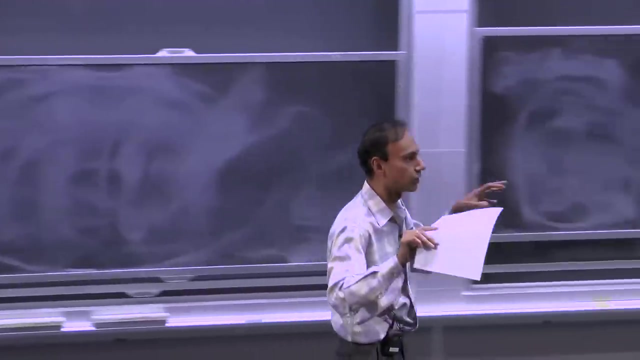 And this manager is going to estimate votes obtained per dollar spent. OK, But that dollar is spent advertising in support of a particular case or a particular issue, And contradictions are allowed. As long as you're sending different messages to different demographics, you're on the same page. 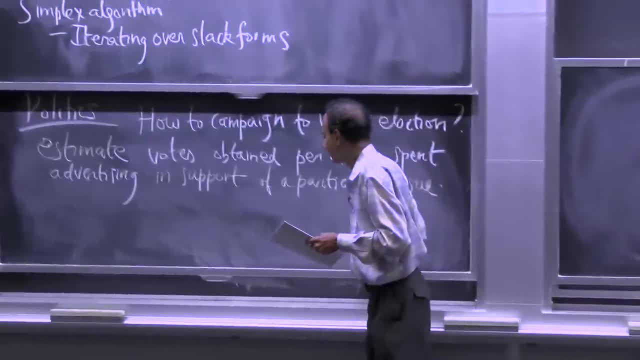 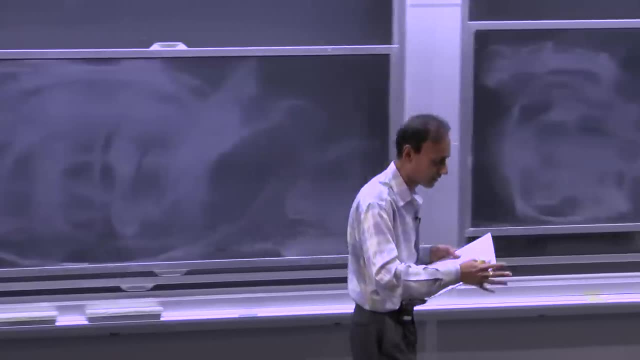 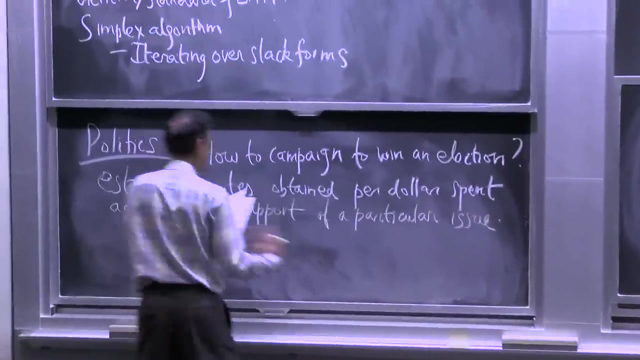 You're all good, right. You're assuming that people don't watch more than one channel, all right. So you're a Fox News guy, you're an MSNBC guy, You don't do both, OK? So now we get this estimate and it turns into a table. 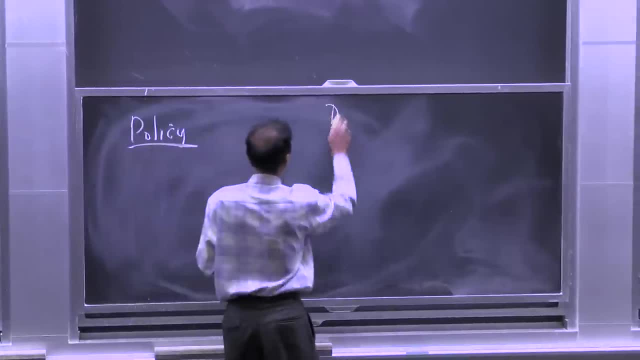 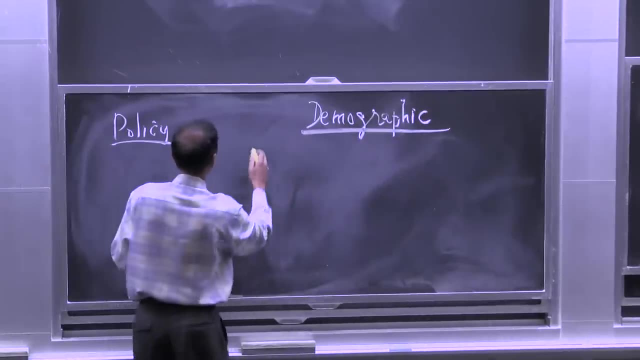 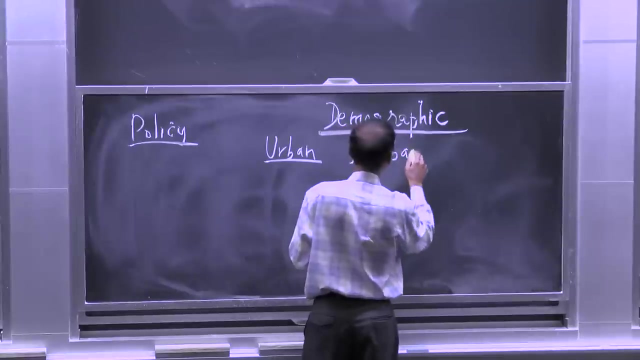 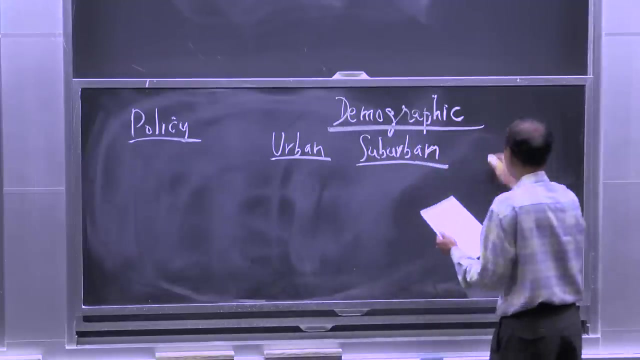 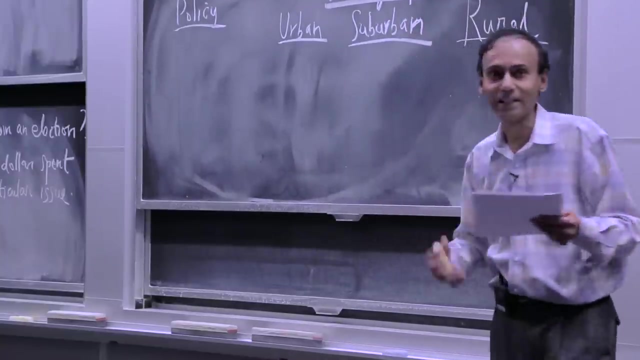 So you have your policy and you've got your demographic, So you've got urban. now think Detroit suburban. I guess you can think Lexington, where I live- and rural. I really don't have any idea what that means, but presumably there's places. 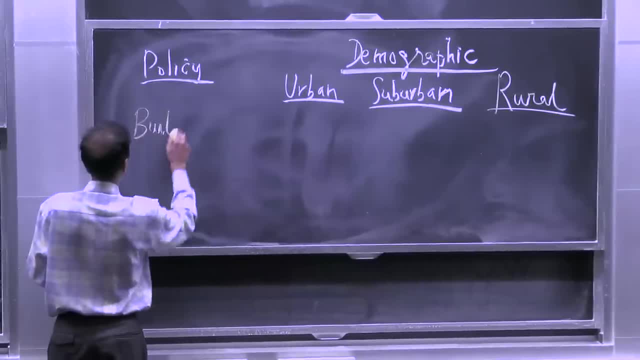 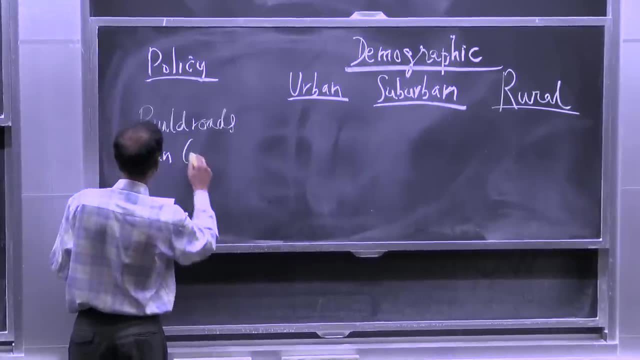 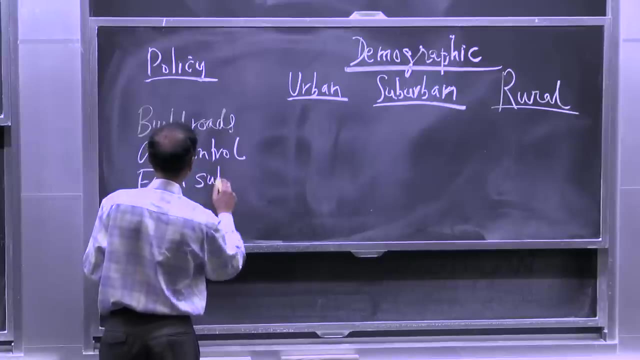 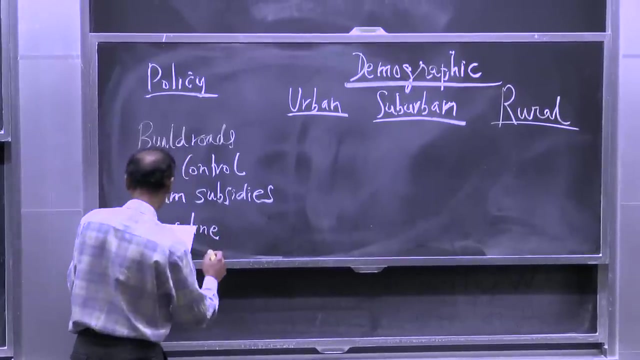 And here's our policy Right: Build roads- kind of boring, but some people are interested in roads. Gun control, oh very sensitive. Farm subsidies- you know who's interested in that- And gasoline tax kind of more. this hits your pocket, so more or less everybody's interested. 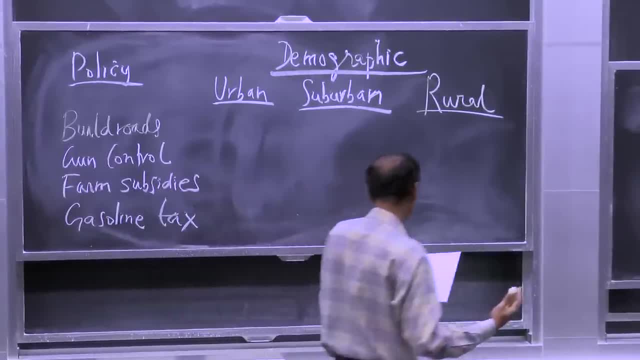 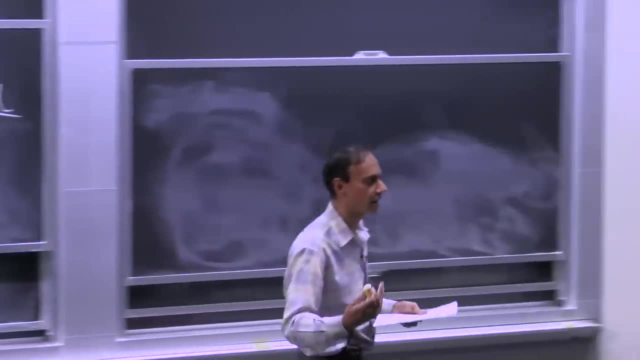 in that. OK. So you tell the urban guys you want to build roads, Build roads, And they don't like you, right, So you get a minus two there. So this can go. you advertise and it hurts you. you lose votes. OK, Tell the suburban people. well, typically it's a situation where you have these nice cars and you don't like potholes, so you like roads. if you live in suburbia, Rural people have 4x4s. They don't particularly care. 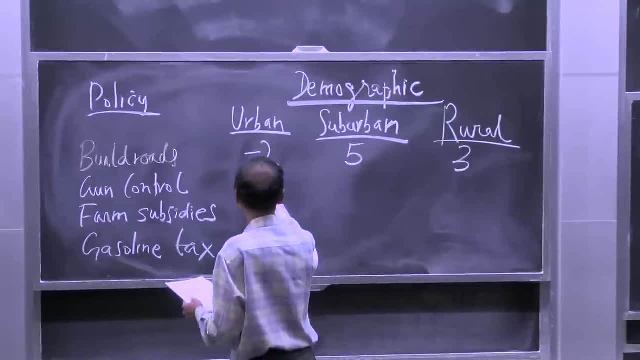 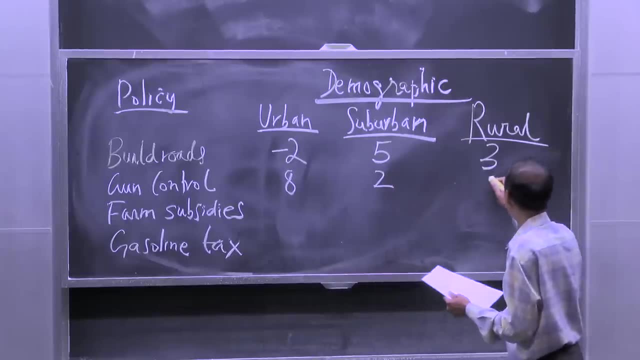 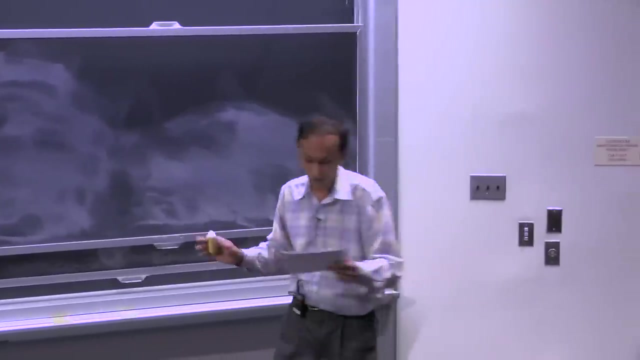 They don't care as much. OK, Gun control. Well, you can imagine the urban people like that. Suburban people are mm OK, meh, And the rural people hate it. right, You do not want to advertise on gun control? in the rural areas, right? Farm subsidies: it's like don't want to deal with that. What is a farm? And the rural people love it, right So and then gasoline tax. well, urban people are commuting And well, they typically don't have a lot of money. 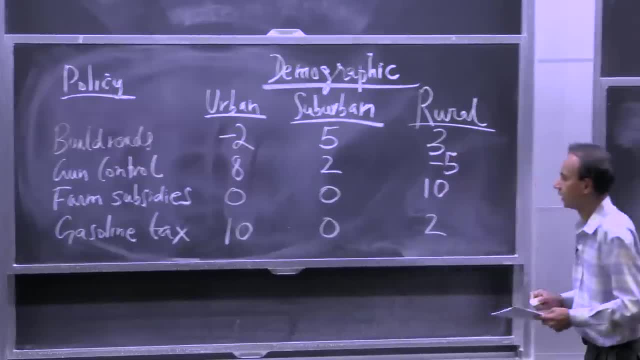 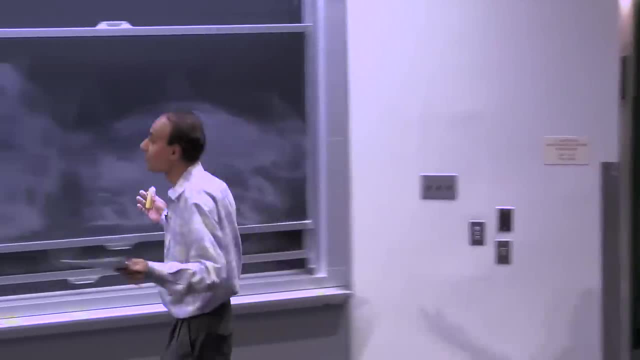 So there you go, And those are the numbers. I'm not going to justify every number here. OK, But you can put whatever numbers you want. I mean. so let's move on. This is just a table. It could have positive numbers. 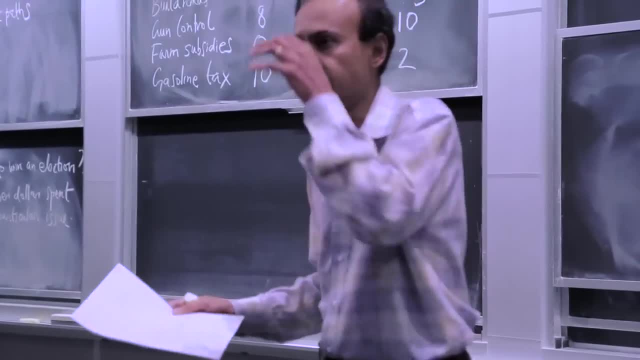 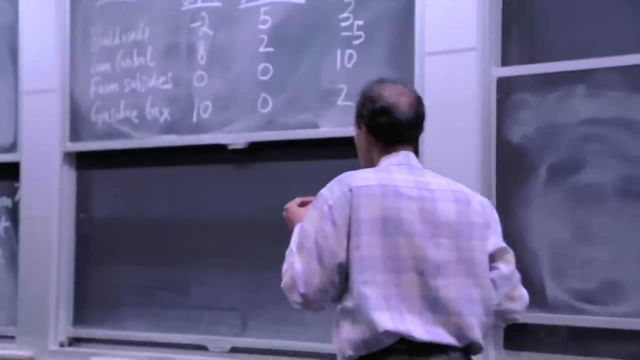 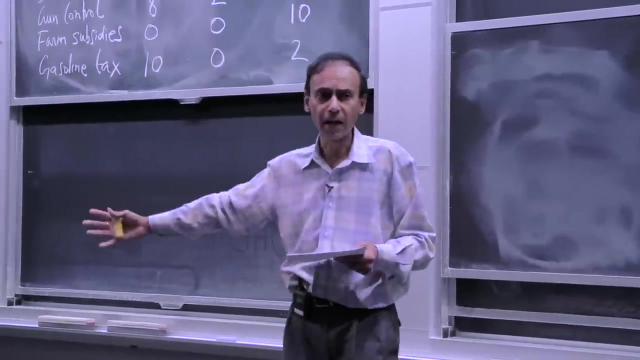 It could have negative numbers And you still want to win this election. Regardless of how crazy the demographics are, how crazy your electorate is, you want to win the election. So as long as you have a great campaign manager who can get you this table, it's all mathematical here on out. 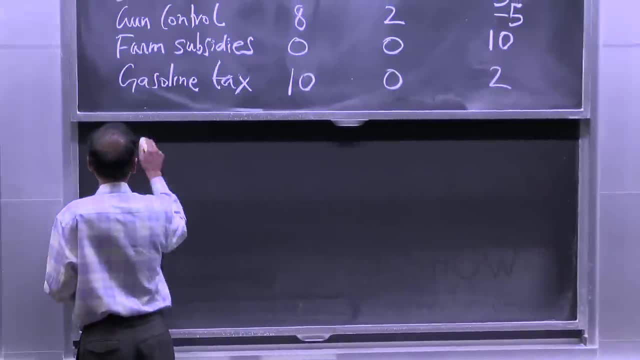 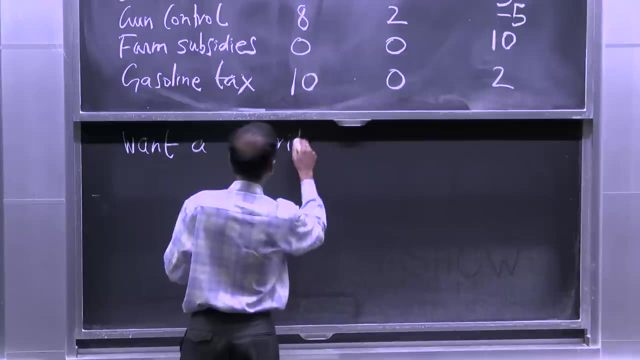 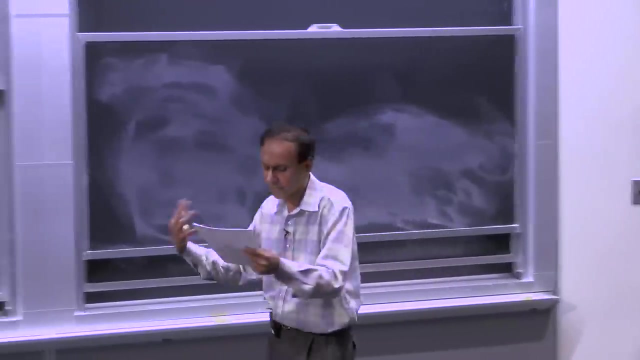 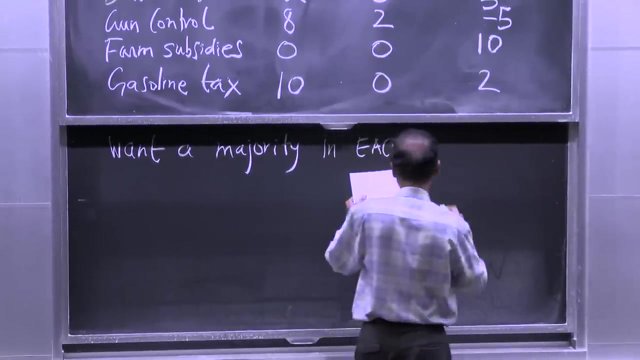 OK, You just got to figure out how you're going to win a majority, And you could argue that all you want is to win the election, And we're going to do something slightly different, which is something that's obviously going to guarantee victory. 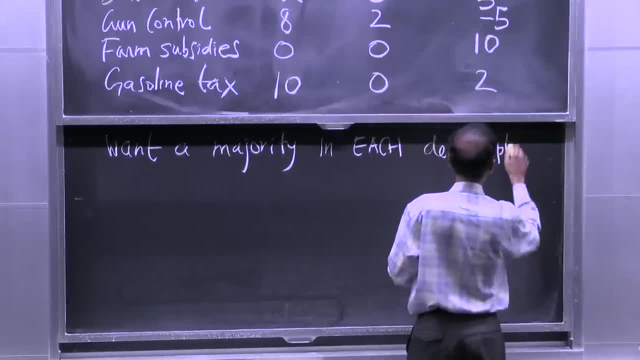 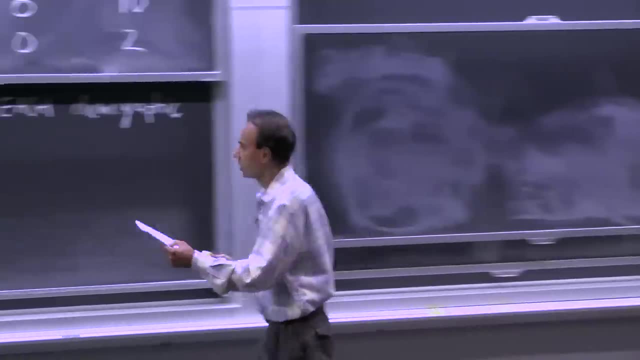 But you want to win a majority in every demographic right, Because the tables may be off by a little bit. You want to be careful, All right, Thank you, Thank you, Thank you. So the last thing, of course, in order. 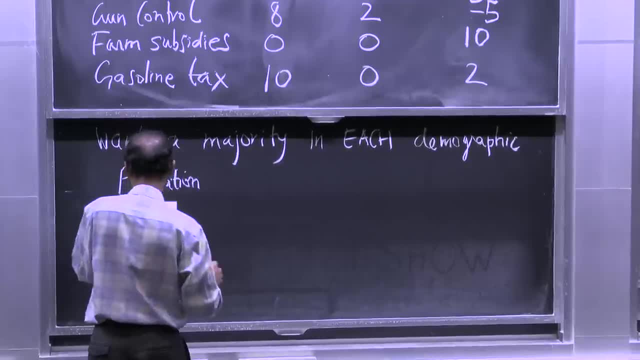 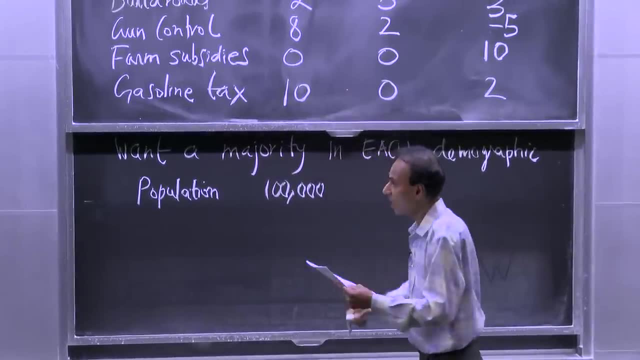 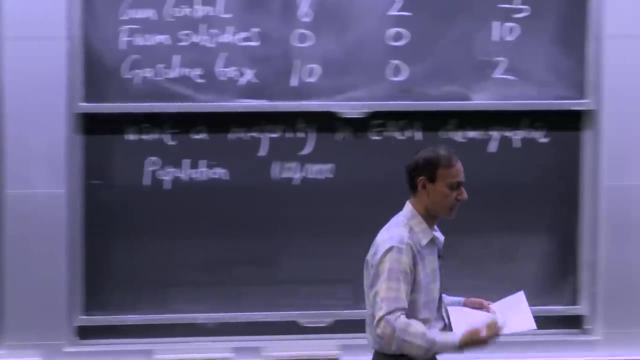 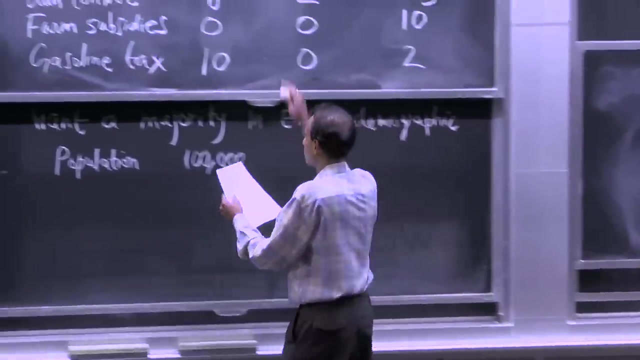 to estimate how much money you need. is the population here? So that's votes obtained per dollar spent right, So you're getting it's $10 a vote, It's $5 a vote, et cetera, And so we need to translate that to votes. 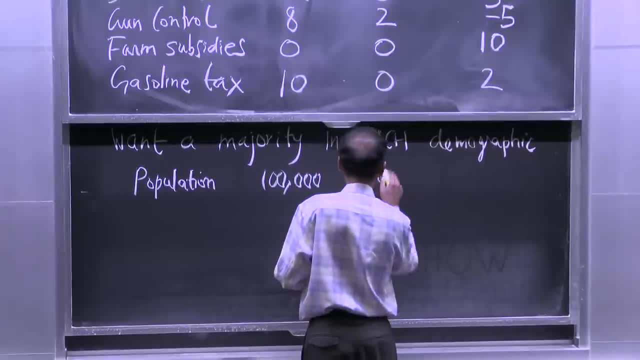 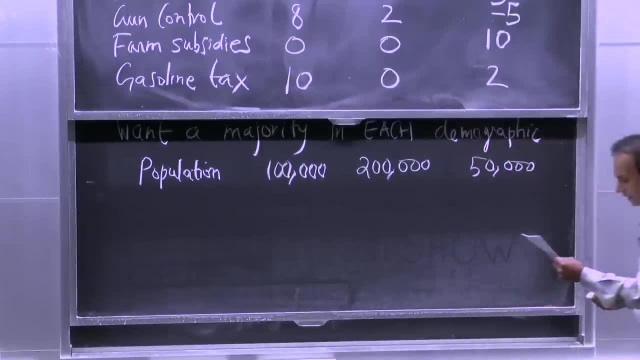 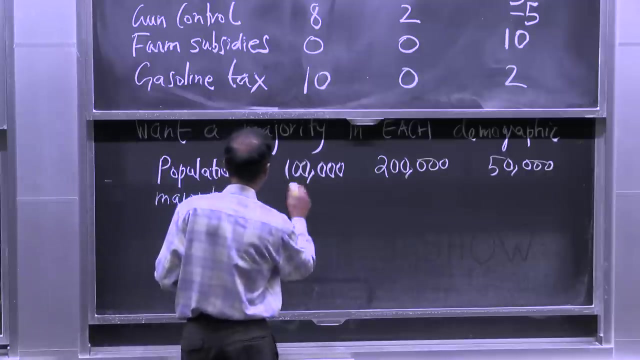 because that's the dollars And you got your population here corresponding to each of these areas And that's what you got here, The majority we'll assume you win in the case of ties, just to keep these numbers easy. So that's just divided by 2.. 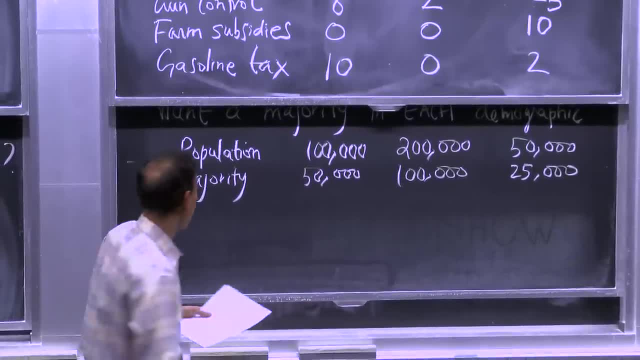 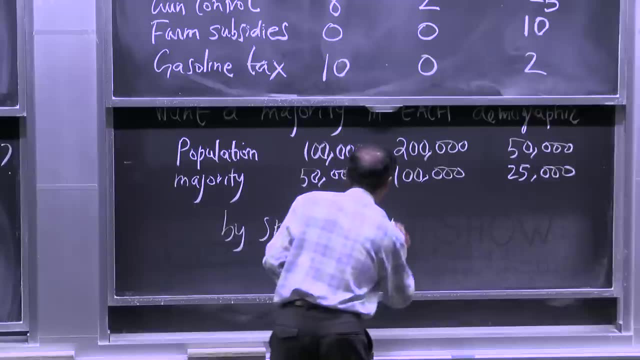 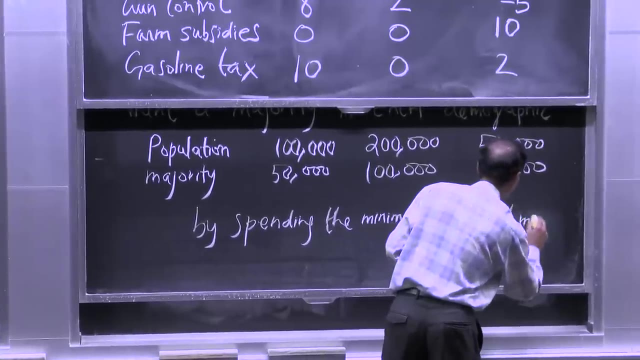 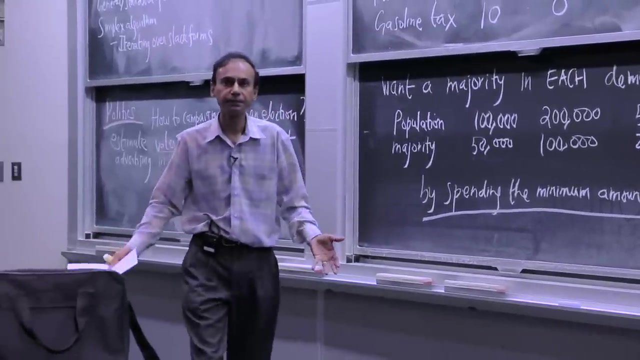 OK, So that's what you got so far, And You want to win by spending the minimum amount of money, right? So that's our optimization problem. So we can take this and we can convert it to a set of linear equations. 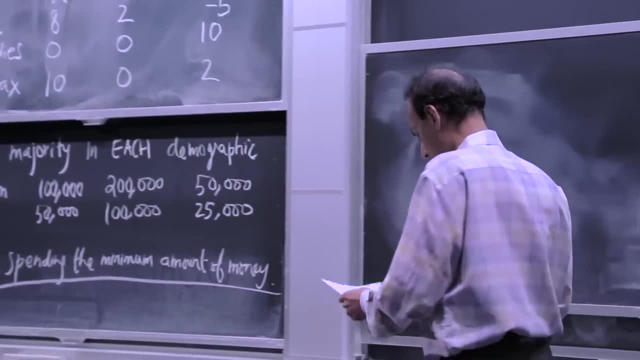 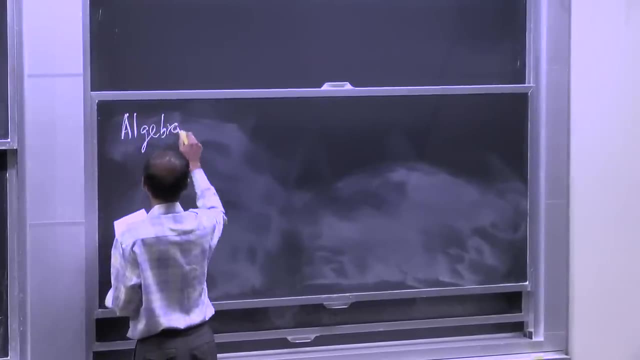 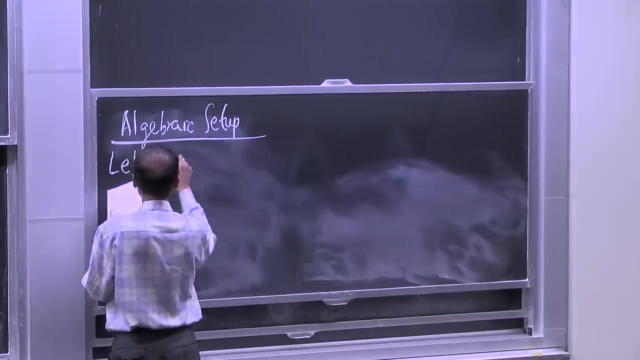 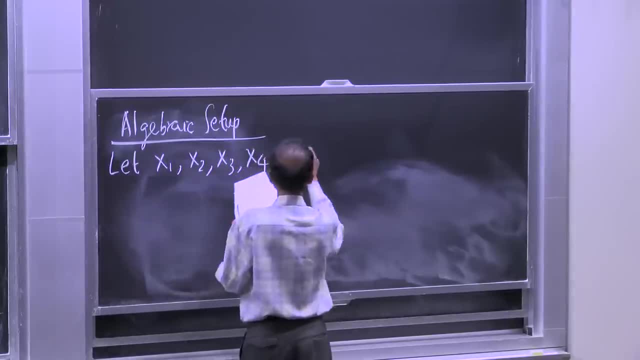 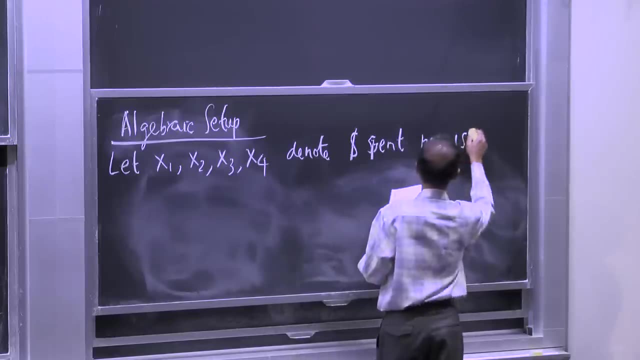 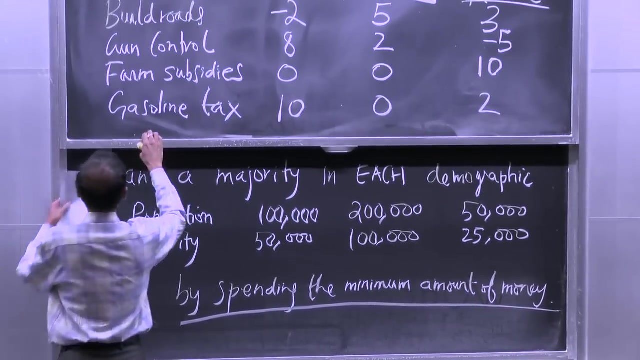 So let x1, x2, x3, x4 denotes the dollars spent per issue. So you've got those four issues up there. So let me write that out. It's important to Let me make sure you know what I'm talking about, with respect. 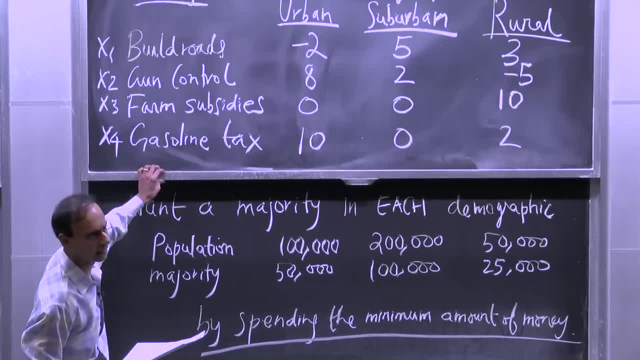 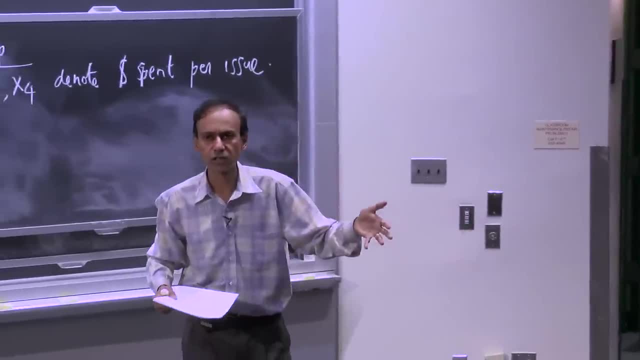 to a particular issue. So those are our four issues and those are our four variables. So this linear program has four variables. You're trying to discover the values of these variables to optimize, minimize your cost function. The second thing the linear program has: 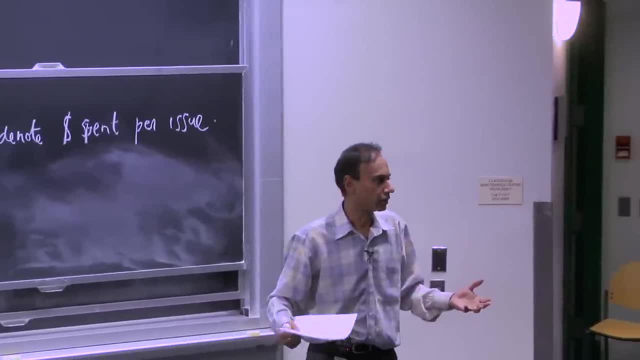 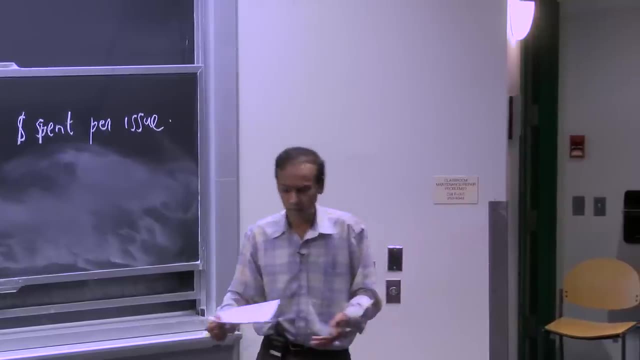 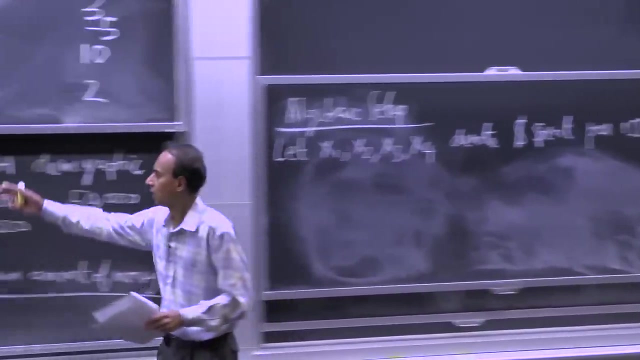 and pretty much the only other thing a linear program has are constraints, And these constraints are also linear. It gets much more complicated if you have quadratic constraints, and we won't go there. These constraints that I'm going to write correspond to this statement here, that 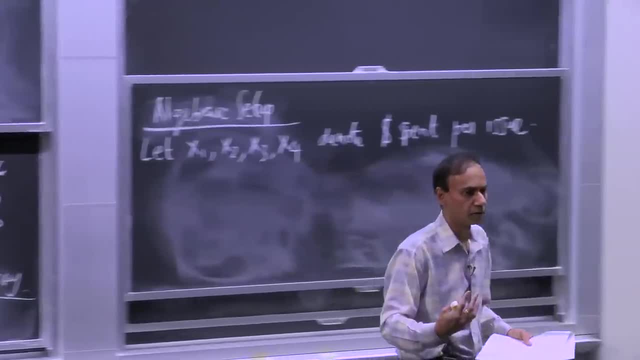 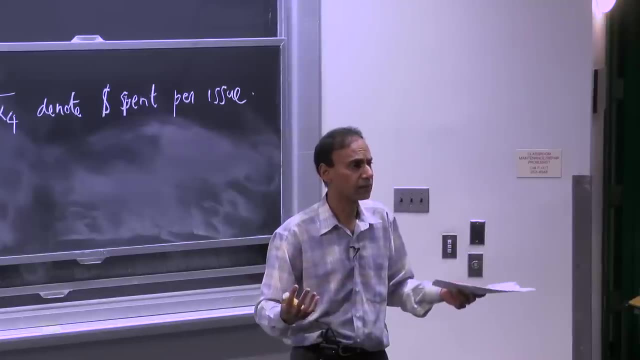 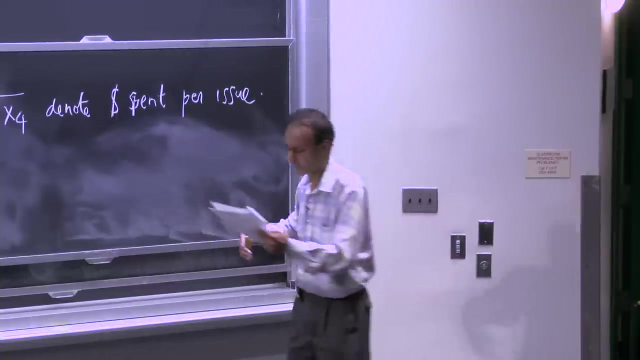 says you want a majority in each demographic. So you can imagine that because you have three demographics, you're going to have three constraints. You could have written this differently. There's just any number of variance here and you'll get the sense of that as we go to other examples. 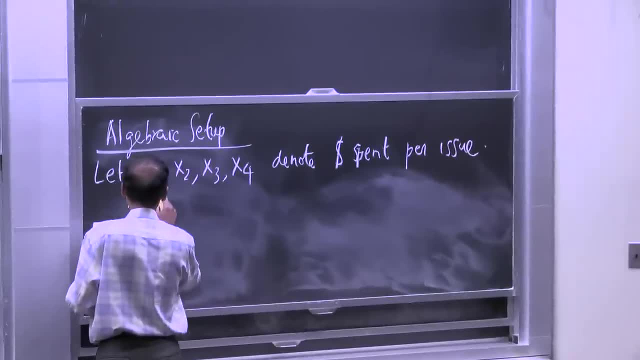 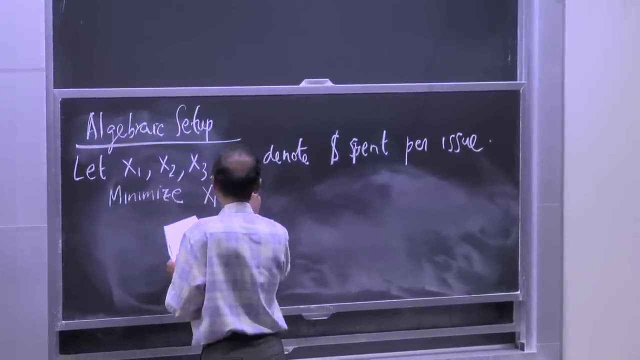 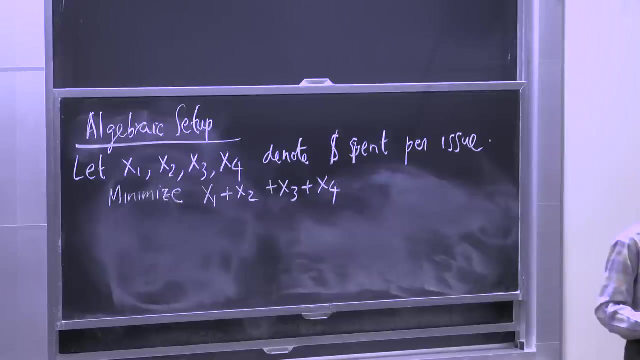 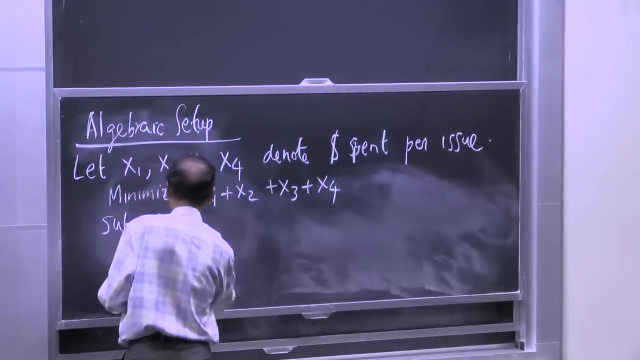 OK, But we'll just stick to one variant here. So now I want to translate everything that I've written in English over there into algebra, And so I got my minimization criteria: minimize x1 plus x2 plus x3 plus x4 subject to minus 2x1 plus 8x2. 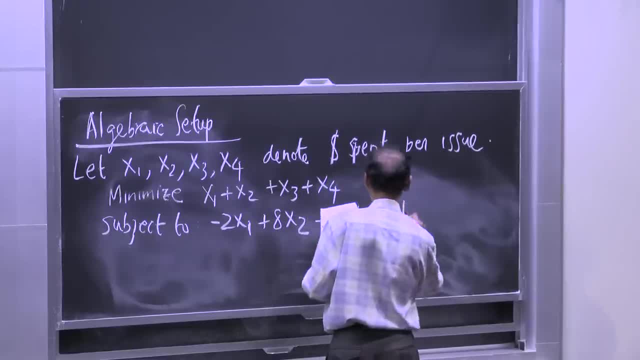 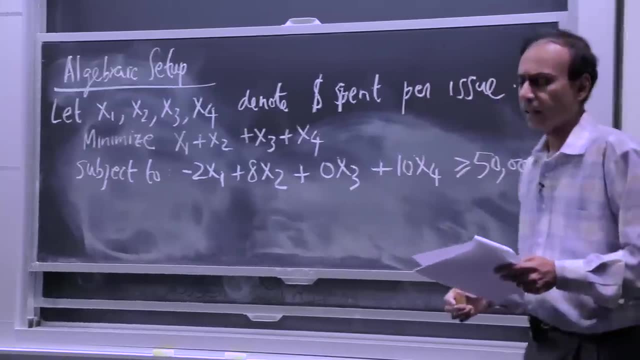 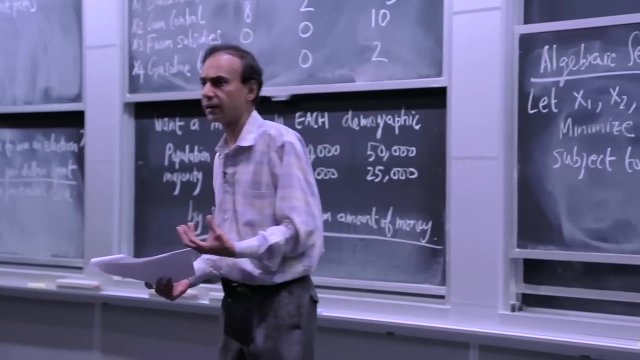 plus 0x3 plus 10x4, greater than or equal to 50,000.. And this represents the requirement that I want a majority in the first demographic, namely the urban demographic, And so I want at least 50,000 votes there. 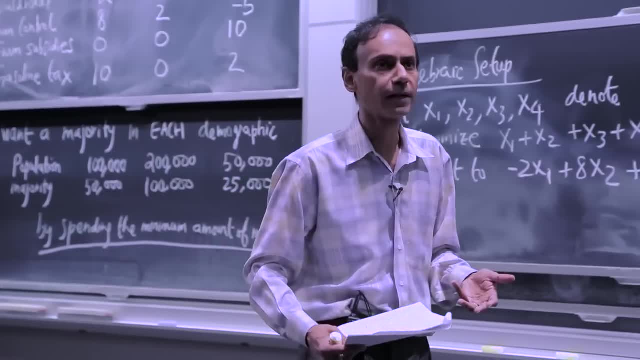 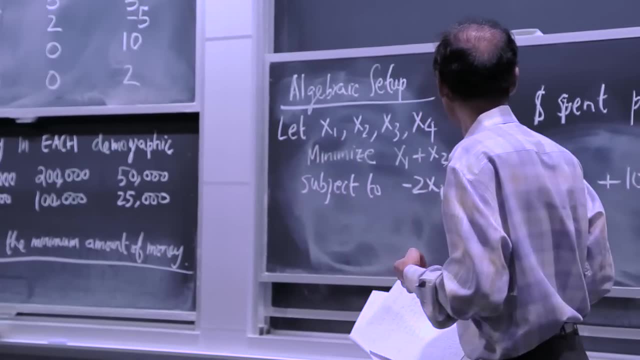 And I need to spend the money corresponding to the values of x1 through x4 in such a way that I get those 50,000 votes. And that represents that. and it's just reading off the minus 2,, 8,, 0, and 10 from the urban column. 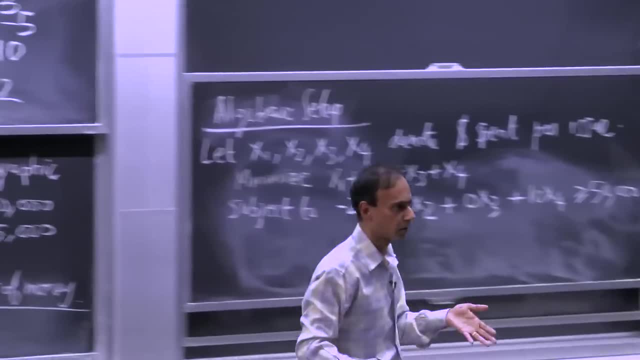 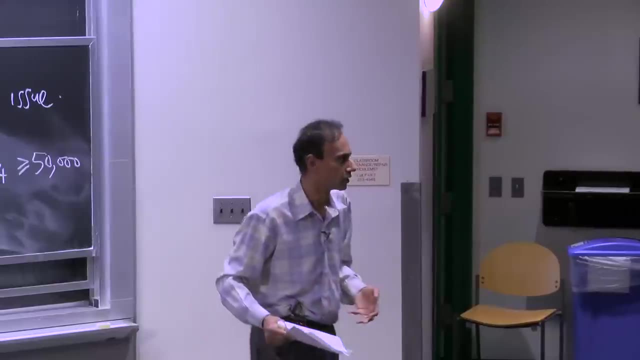 So those numbers that you see here correspond to the column, because I'm talking about the urban demographic And you can imagine that the next constraint is going to correspond to the middle column and the third to the third. So just write that out. I will call this constraint number 1.. 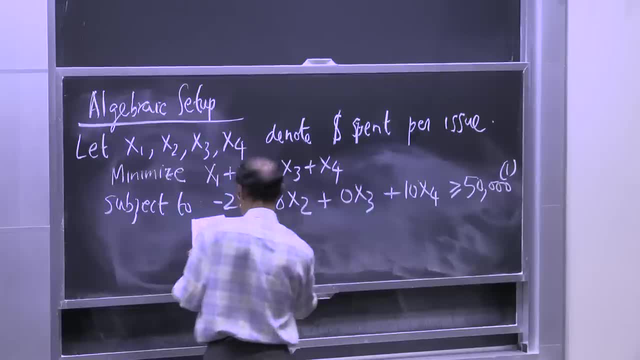 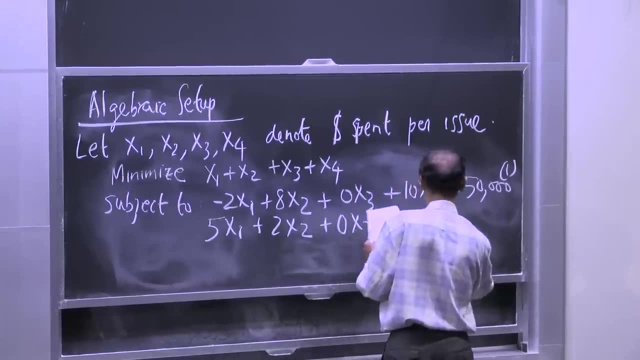 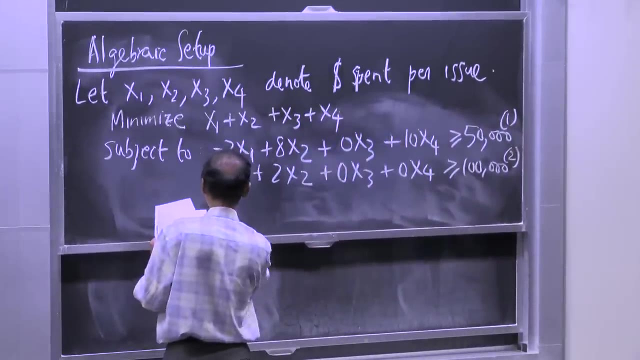 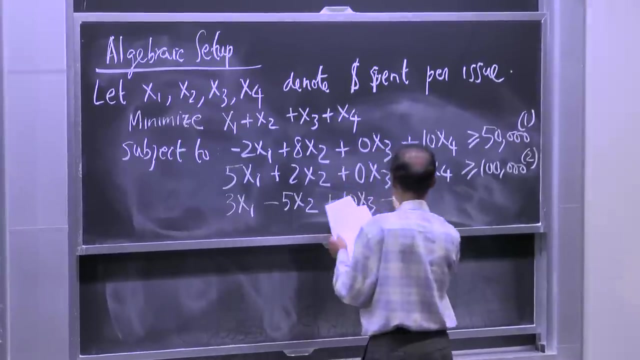 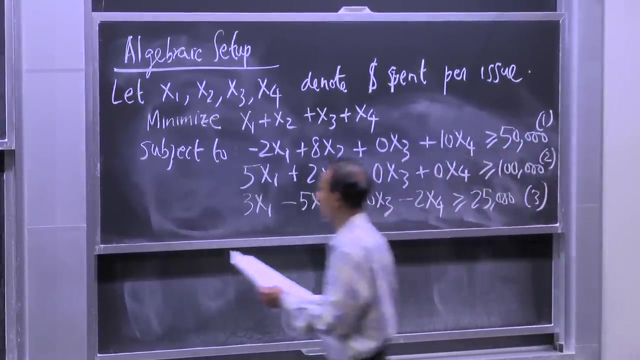 I might refer to it later: 5x1 plus 2x2 plus 0x2.. 0x3 plus 0x4 greater than or equal to 100,000.. I'll call this number 2.. And then, finally, 3x1 minus 5x2 plus 10x3.. 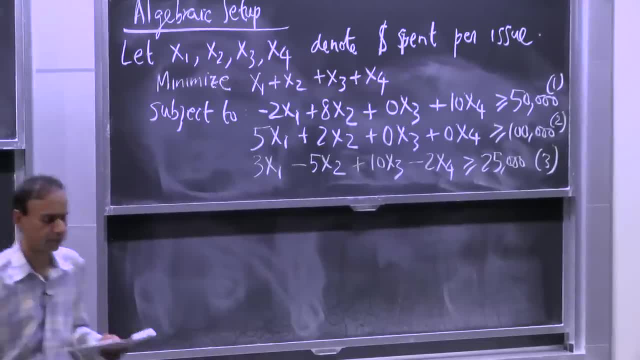 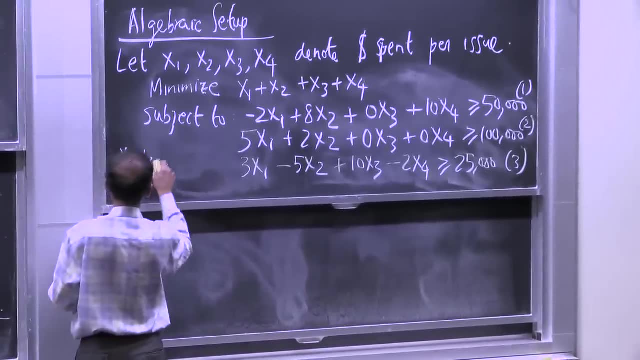 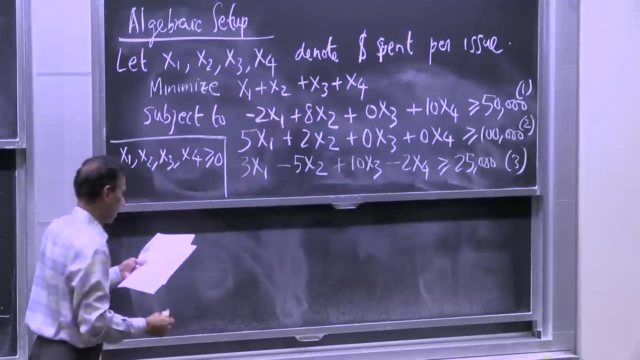 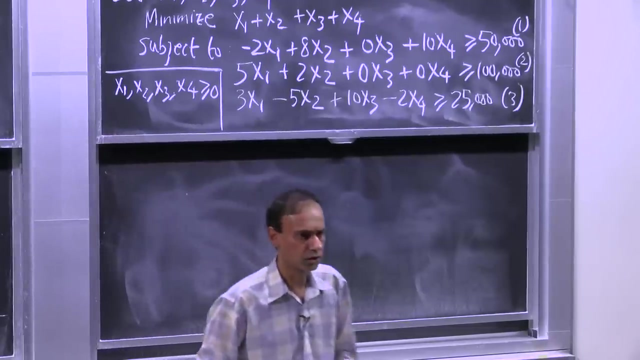 And that's our set of constraints, But this One more little issue that we have to be careful about, if you're being precise, And that is that there's no notion of unadvertising, And so you're going to spend positive dollars. 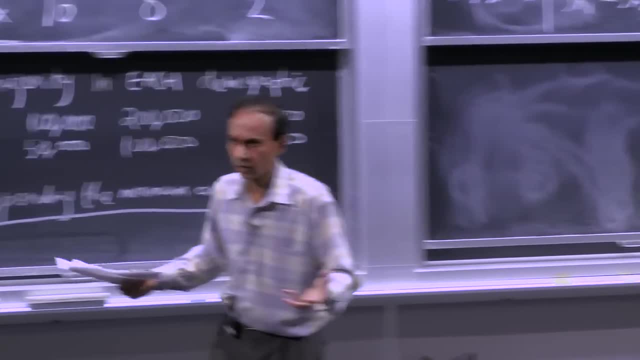 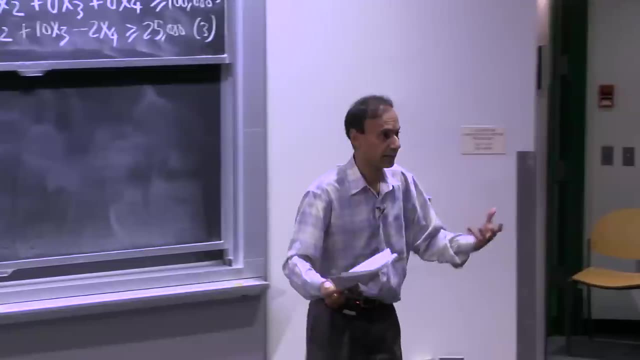 And so x1 through x4 is greater than or equal to 0.. So that's our first linear program And it came from this particular problem. It would be wonderful, and that's exactly what we're going to do for the rest of the lecture. 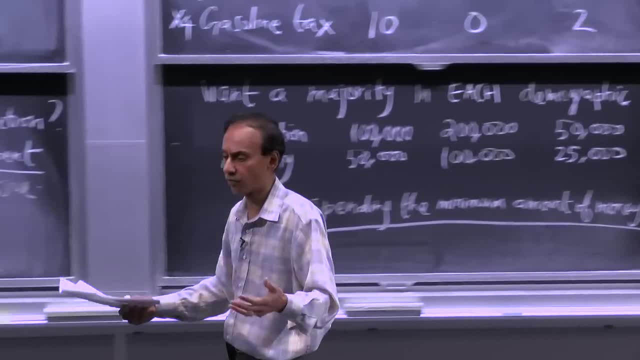 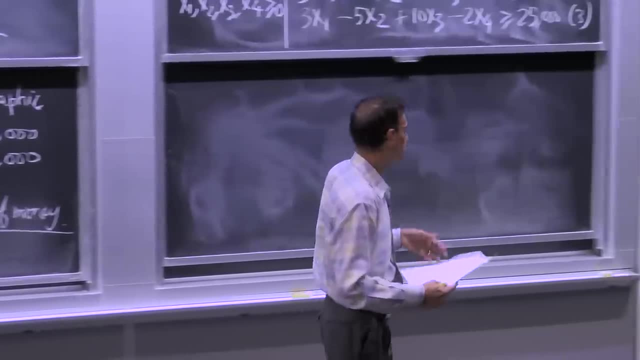 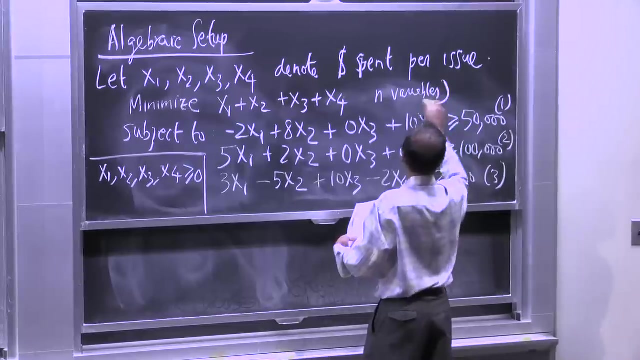 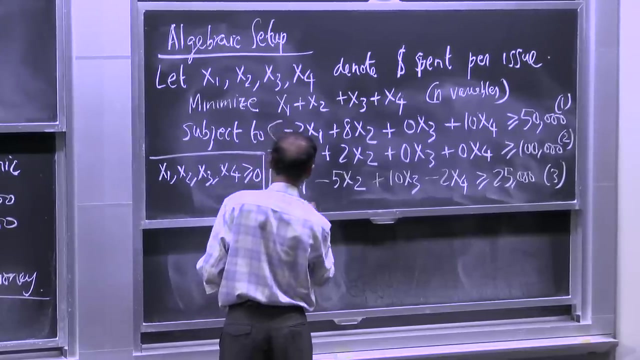 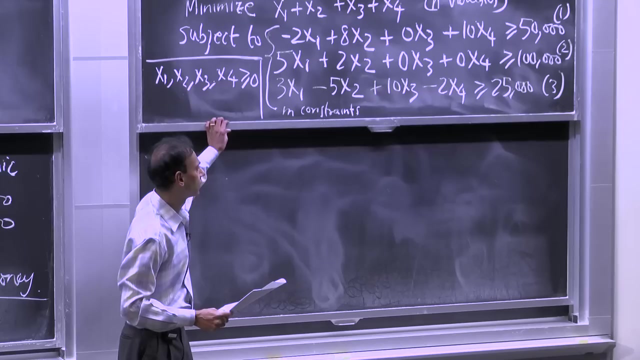 if we could solve this linear program and any possible linear program in an efficient way. And so the number of variables is small, n, And you can imagine that the number of constraints here, just talking about these constraints, are m constraints, And you certainly want a runtime that is polynomial in n. 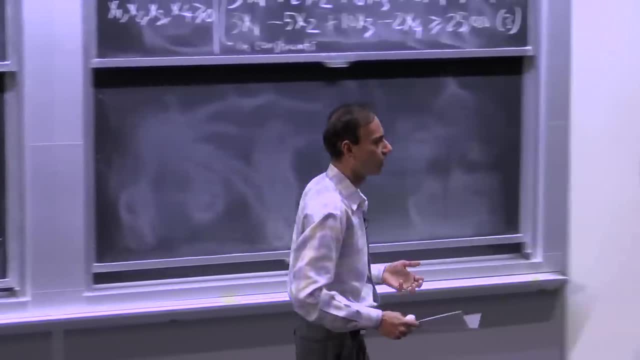 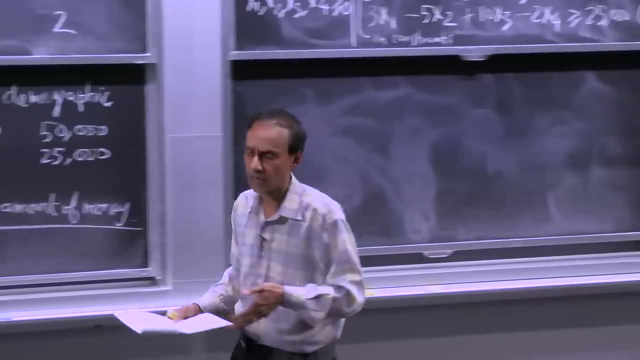 That's our goal here And, as I mentioned early on, it was unclear for the longest time- well, at least not until 1979, but people have been thinking about it for a long time before that- as to whether there was a general algorithm that would solve any linear program. 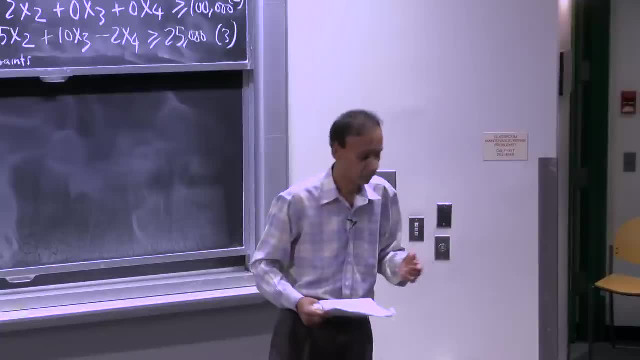 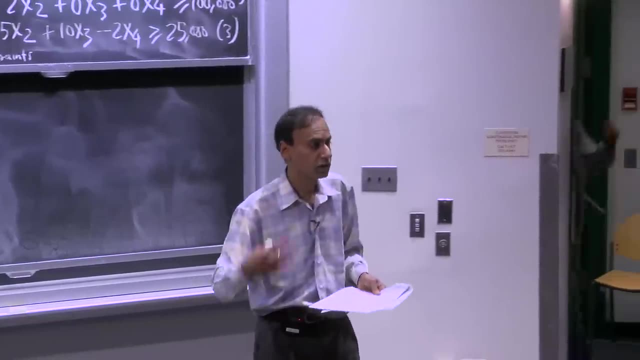 in time polynomial in n, And that was resolved in 79 by Kaushikyan. We'll look at a algorithm, simplex- that in the worst case runs exponentially in n but is simpler to describe and is very efficient in practice. 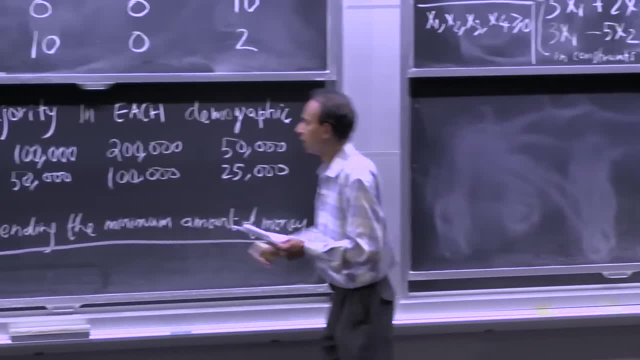 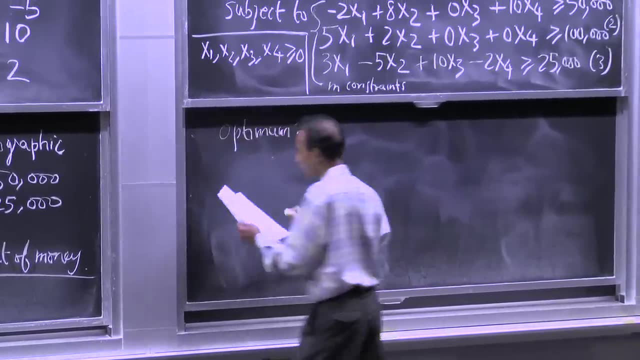 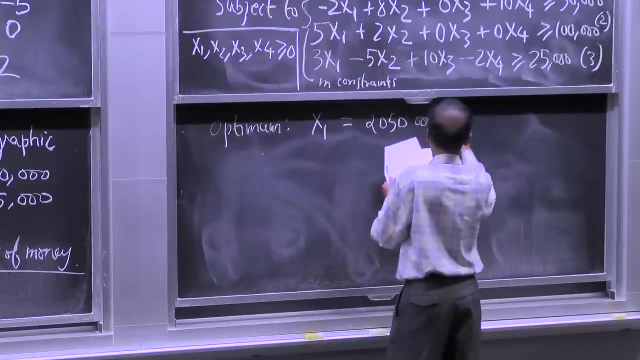 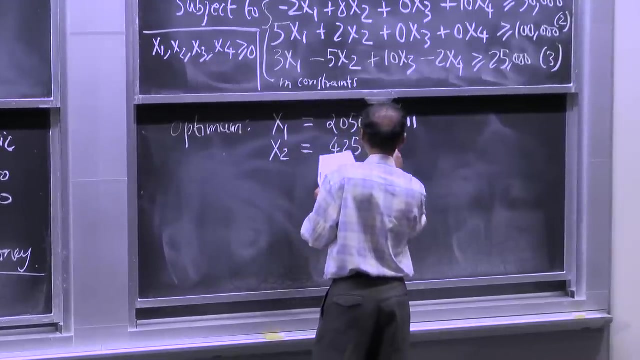 So in our particular problem, this one, it turns out you and I'm actually going to come back to this in a second, but I will just tell you that the optimum for this particular linear program with these particular numbers correspond to these numbers here. 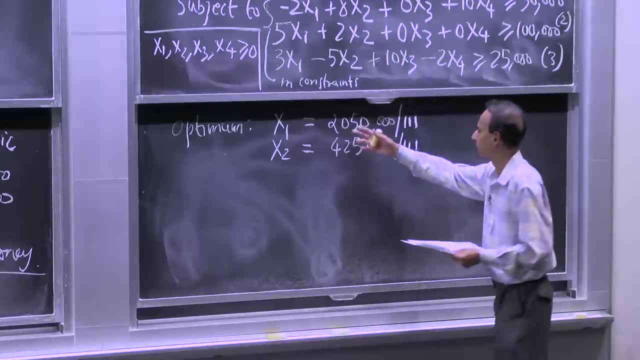 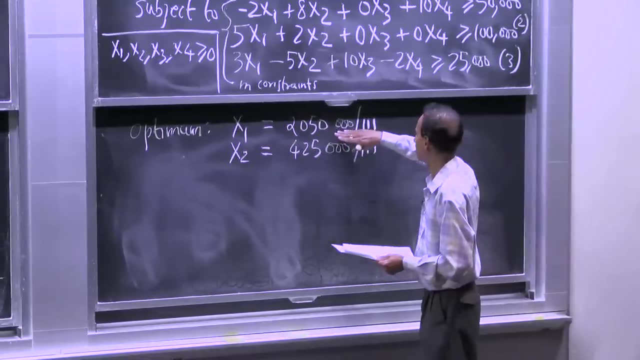 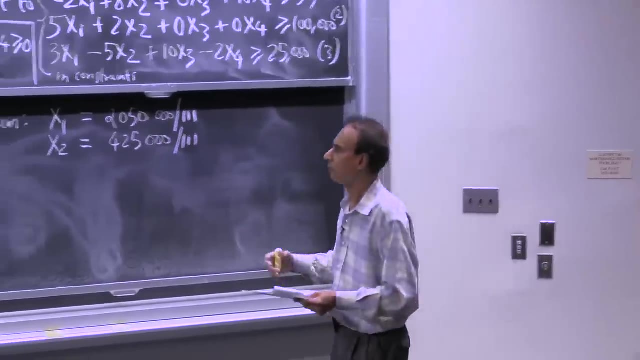 So you want to spend something of the order of $20,000.. So there's 100 here, so take away the two zeros, So spend something of the order of $20,000 for the first issue- building roads. Spend a bit of money for the second issue. 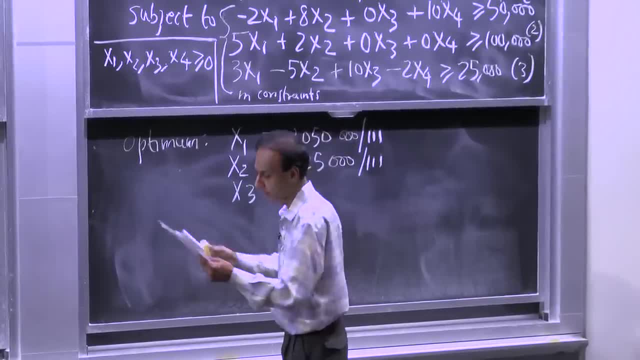 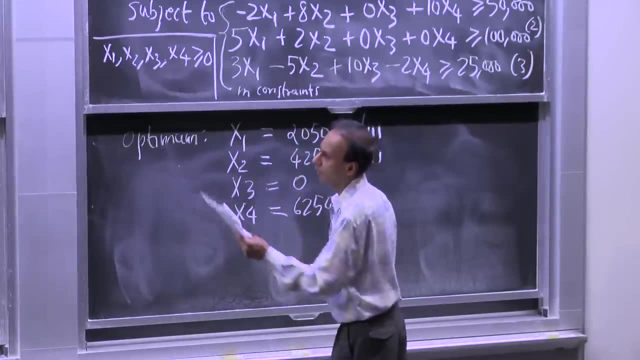 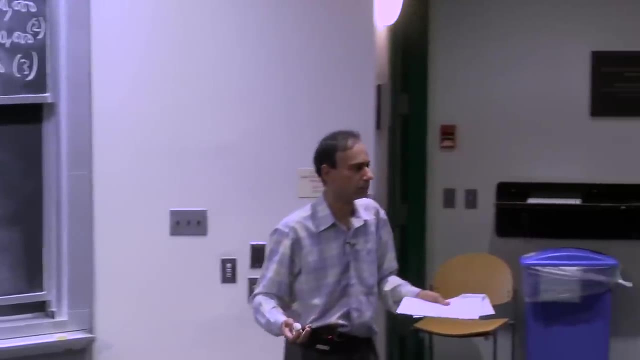 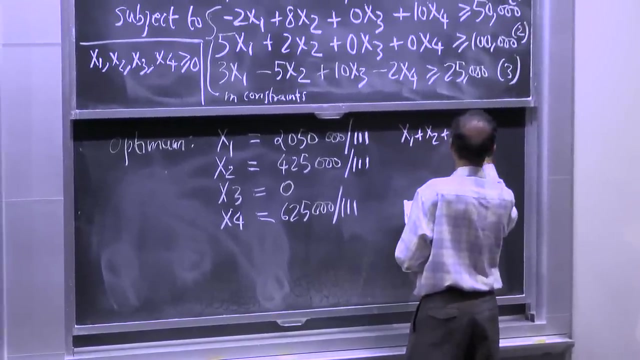 Ignore the third, corresponding to farm subsidies, And spend a bit of money for the gasoline tax issue, And these numbers aren't important, other than the fact that they happen to be optimum. So if you add up these numbers, then x1 plus x2 plus x3 plus x4 is something. 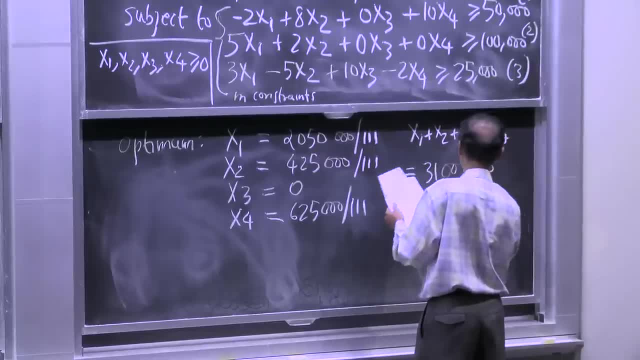 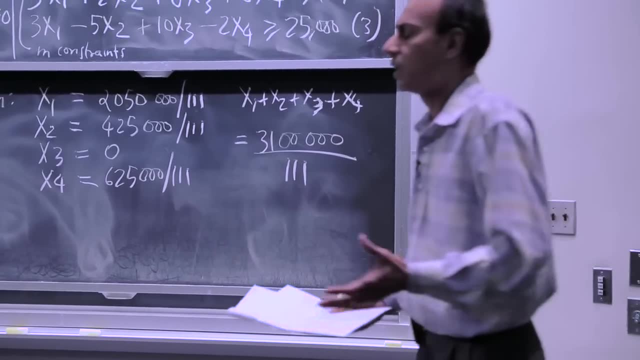 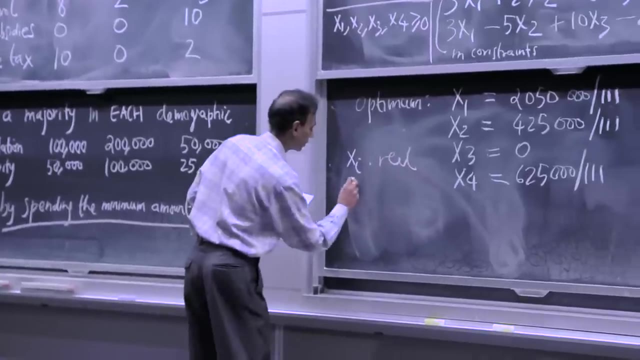 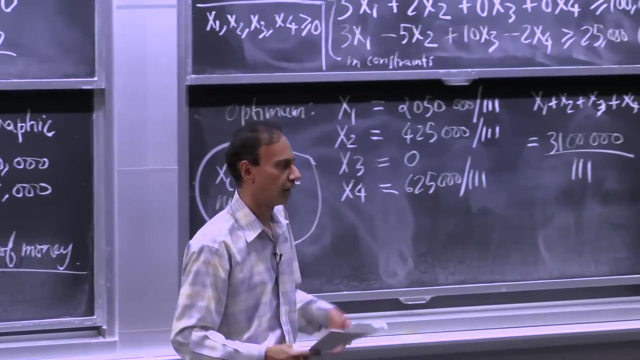 of the order of $27,000, though I'm writing it out as this fraction. So important consideration here is that these values xi are real numbers. That's it. It's not that they have to be integral. Clearly there are fractions here, for the optimum, some of them. 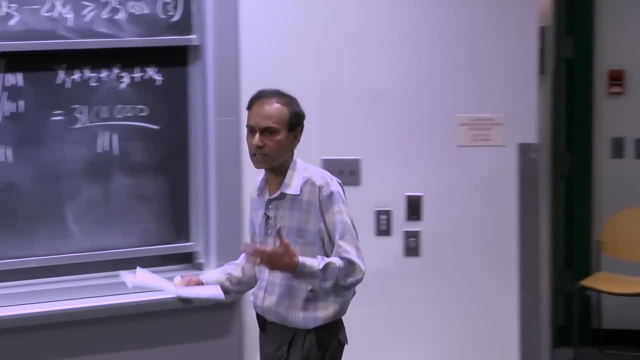 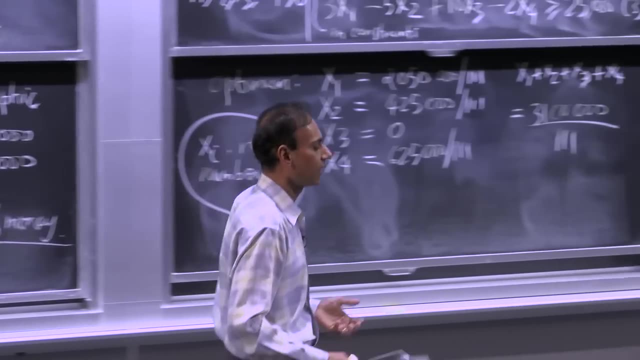 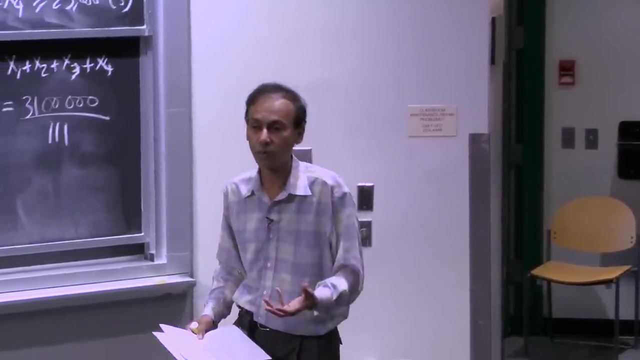 anyway. But in general linear programming says the variable values are real. There's also integer linear programming which is NP-complete, which adds the additional constraint that the xi values are integral. So it turns into a harder problem. You've got polynomial time solvable if the xi are real. 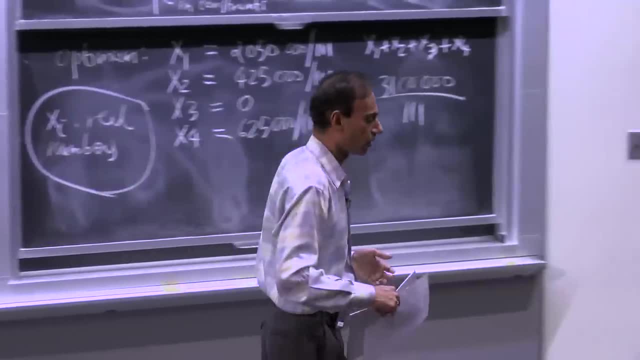 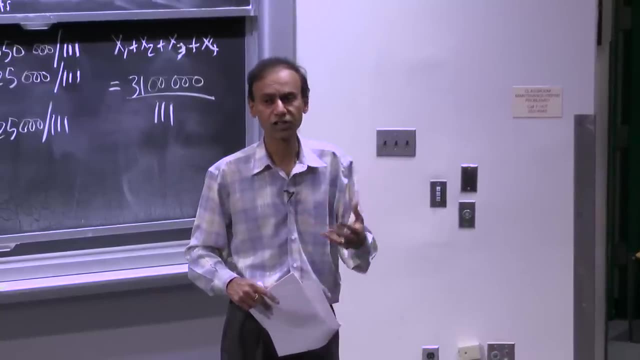 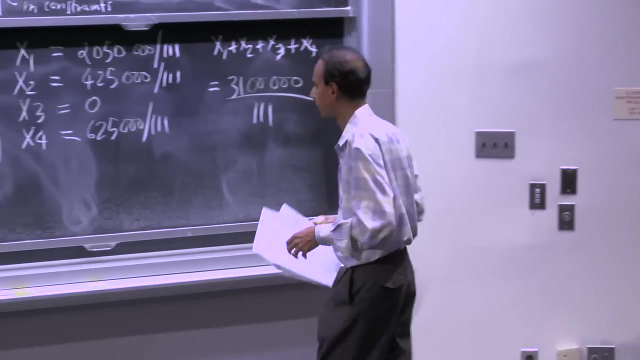 You've got NP-complete- NP-complete- which Eric is going to talk about on Thursday- if the values are forced to be integral. So this extra constraint makes things worse from a complexity standpoint. We won't talk about ILP anymore for the rest of this lecture. 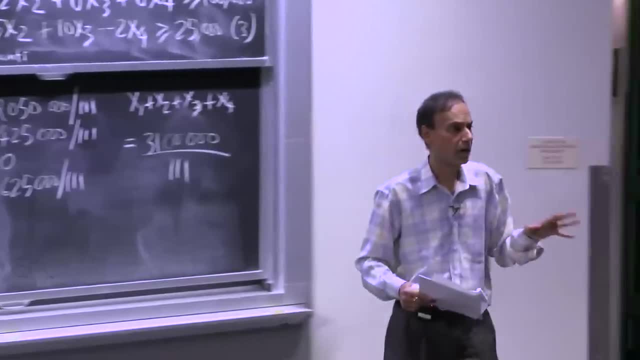 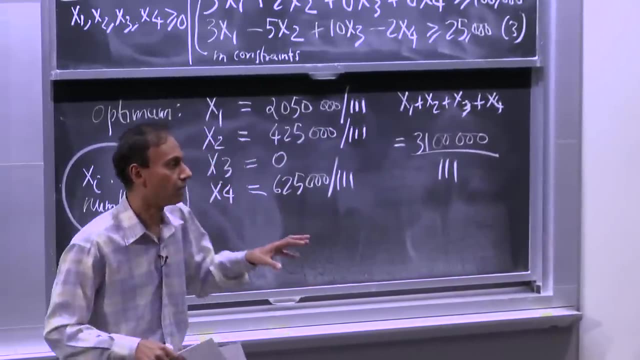 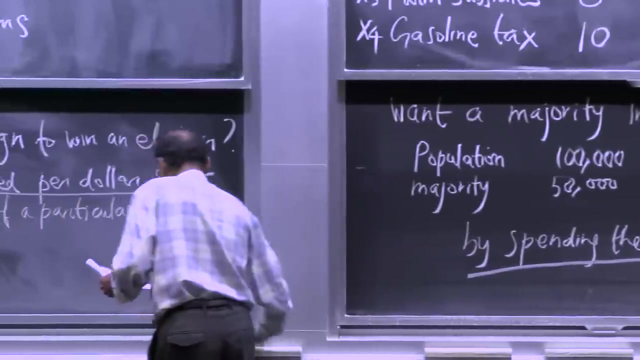 So I will come back to this And I'll talk about how we can show that this is optimum without actually going into a deep algorithmic dive. But what I want to do just before that is to give you the general formulation of a linear program. 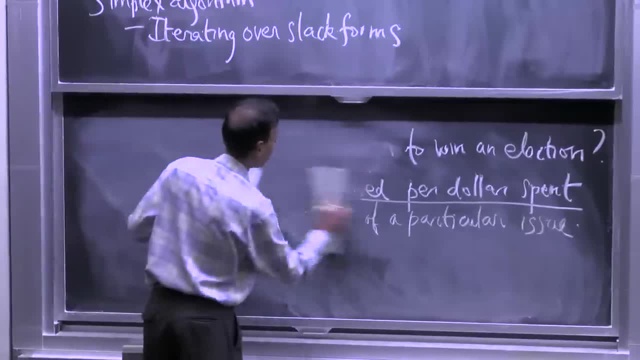 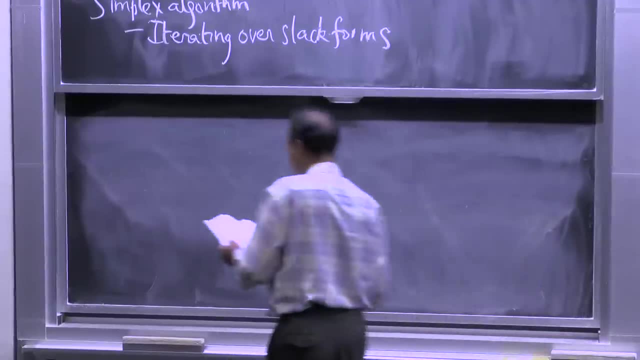 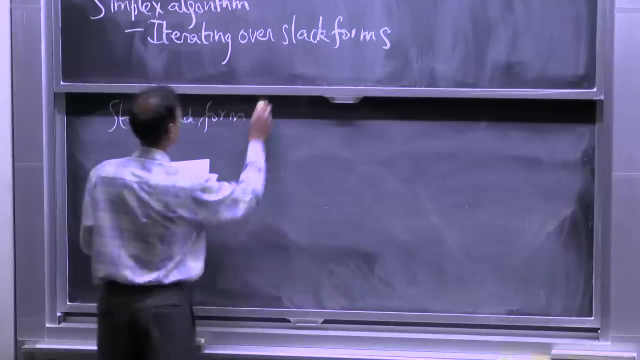 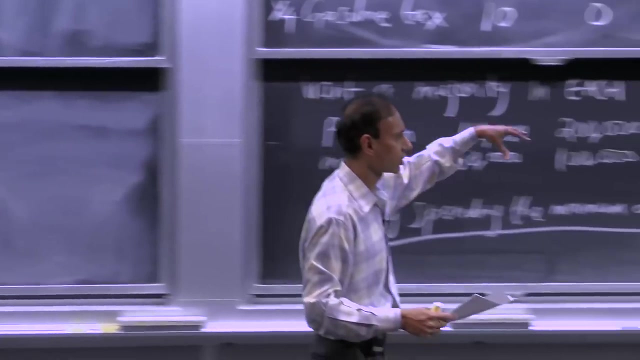 It's called the standard form in CLRS, also called the general form in some cases. We'll look at the standard form for LP And I want to pop up a level. I want to pop up a level about this example and give you the general setting. 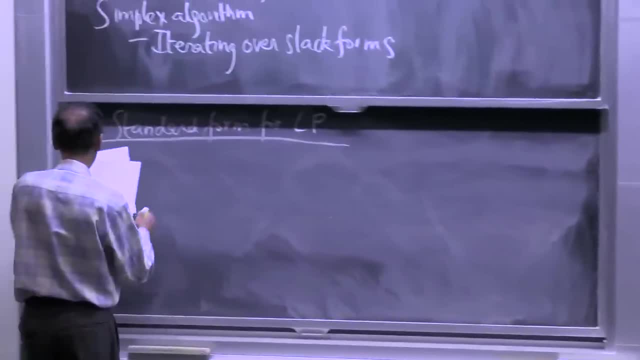 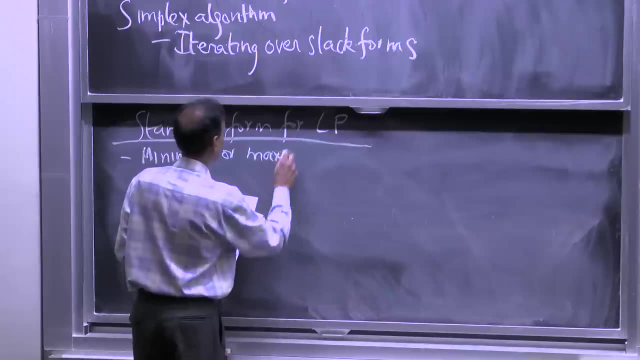 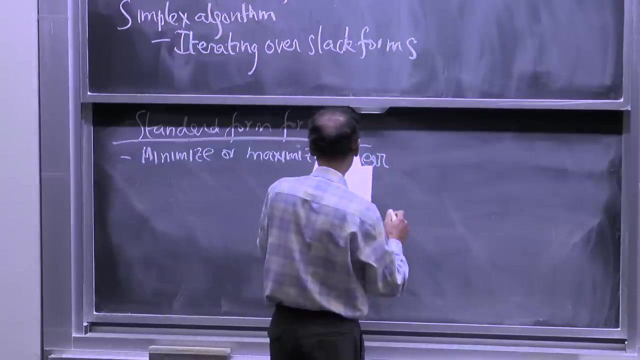 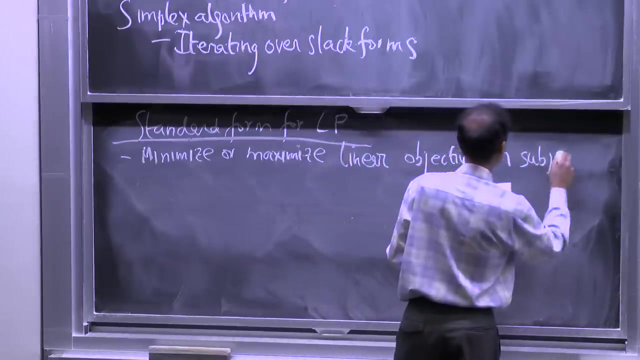 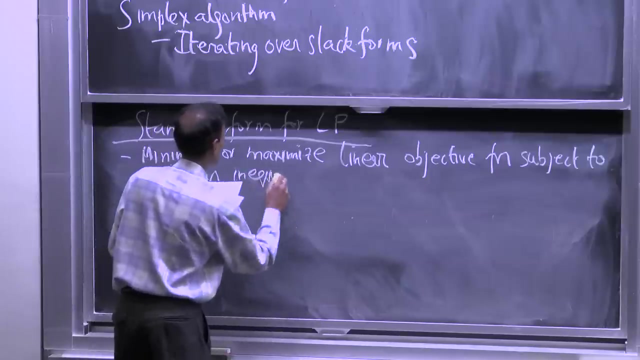 And we'll focus in on the general setting for the most part. But what I have here is I can either minimize or maximize. We had a minimization problem for the political problem. Minimize a linear objective function. subject: Minimize a linear objective function subject to linear inequalities or equations. 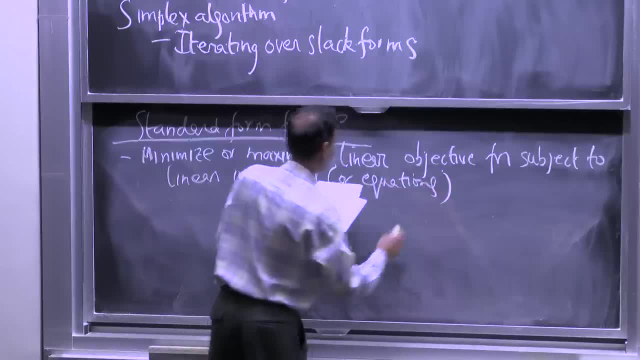 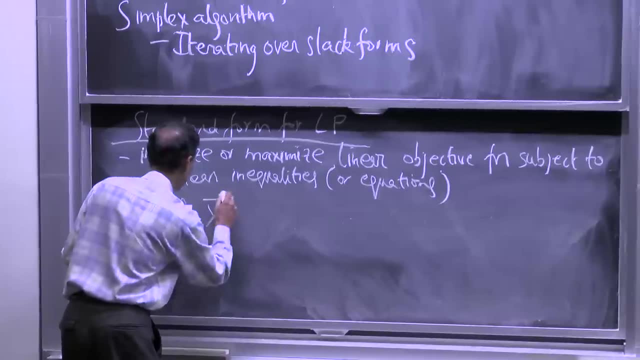 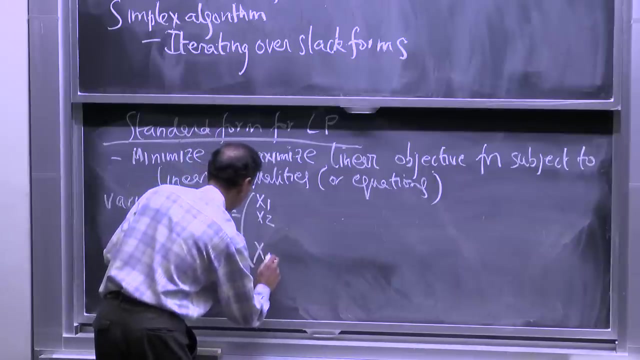 And the variables think of x as a vector. It's a column vector or x1, x2, all the way to xn. Minimize a linear objective function subject to linear inequalities or equations, And the variables think of x as a vector. 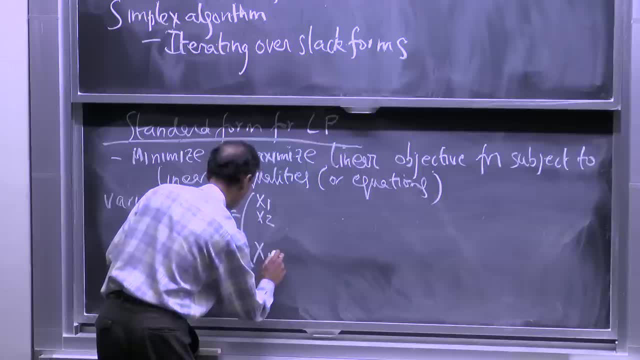 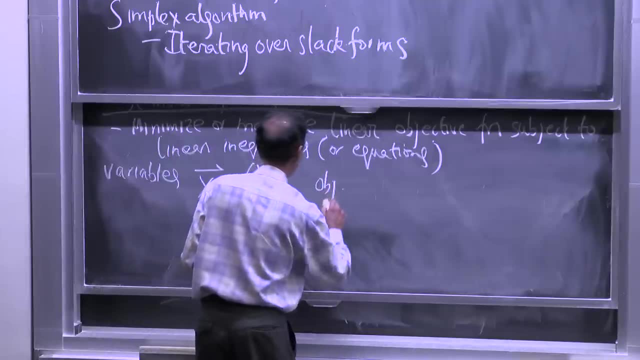 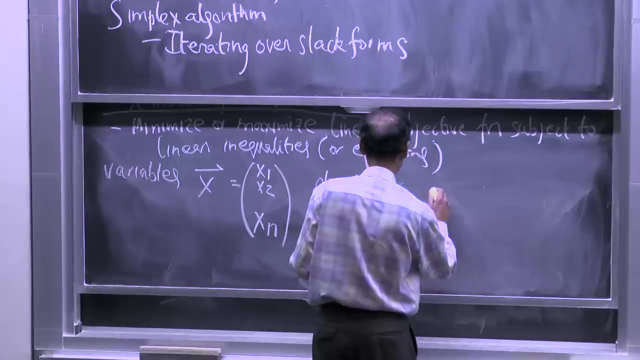 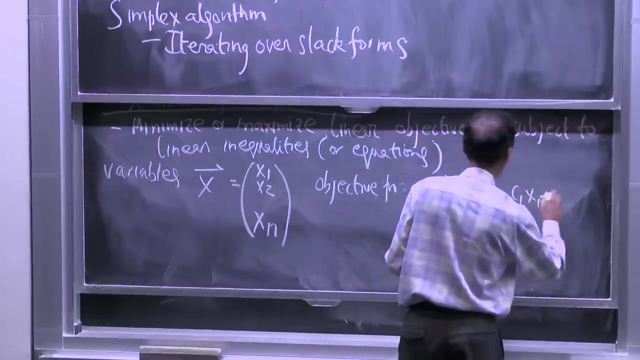 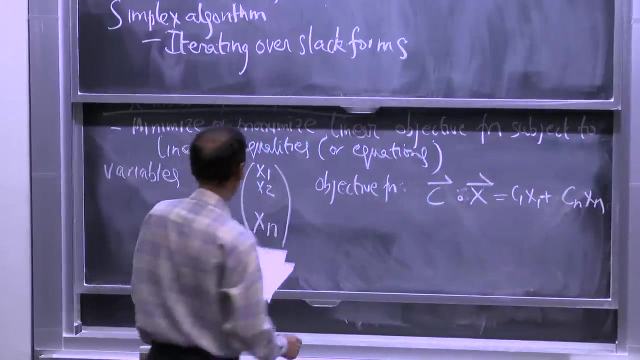 And the variables think of x as a vector And the objective function is c times x, So that's c1, x1, da, da, da, cn, xn, And we just had that All the way to x, All the coefficients being a 1 over there. 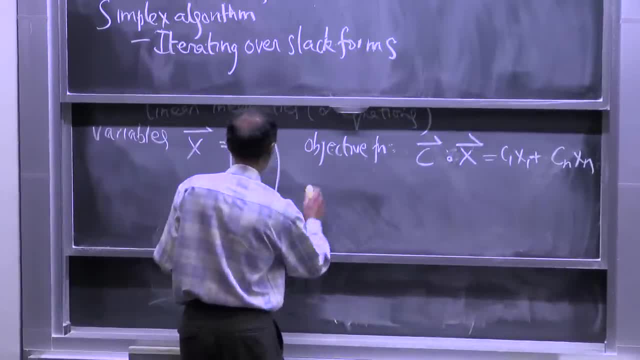 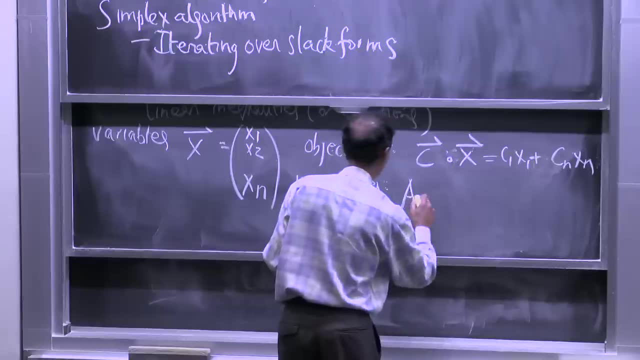 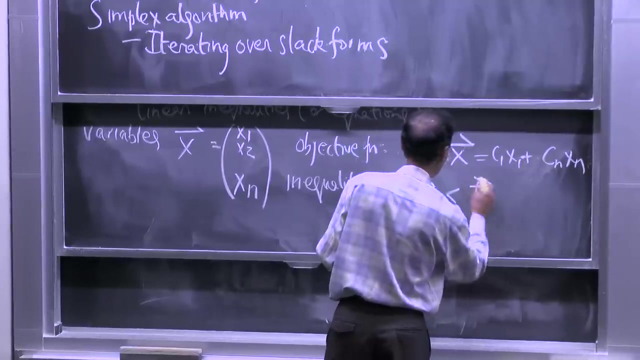 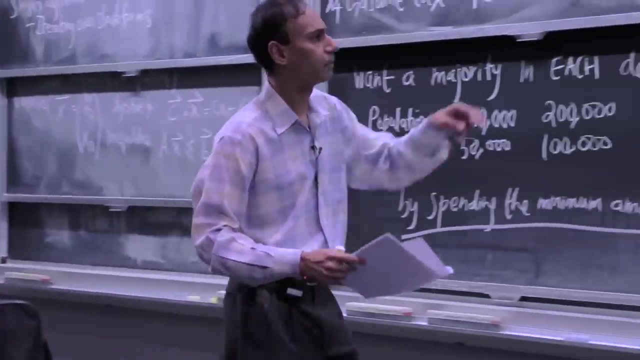 And inequalities. they're the fun part. You represent them as a matrix A, So A times x, less than or equal to b, And notice that this is the standard form that I'm talking about, And now I have diverged from what I had here. 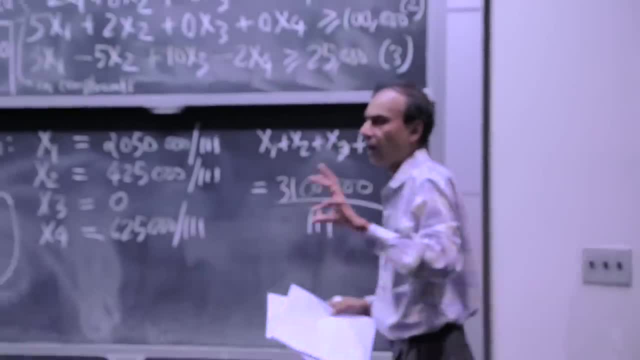 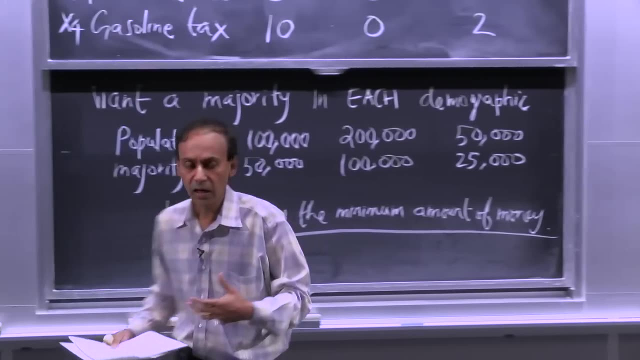 because I had greater than or equal to over here. So So it turns out: you'll see linear programs in different settings. Sometimes you'll have minimization, Sometimes you'll have maximization, Sometimes you'll have less than constraints, less than or equal to constraints. 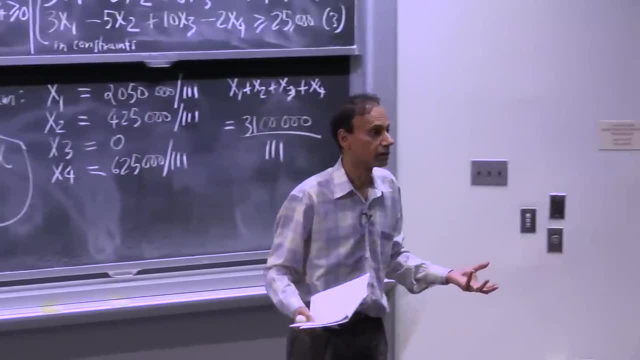 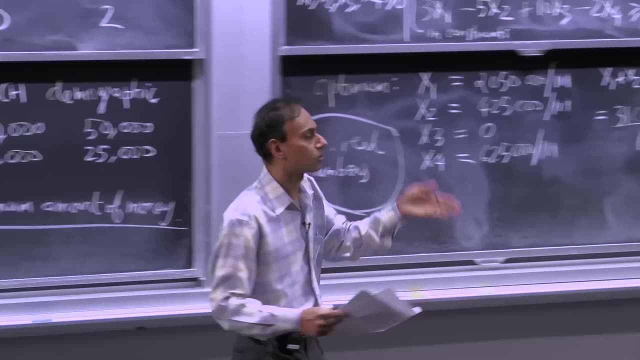 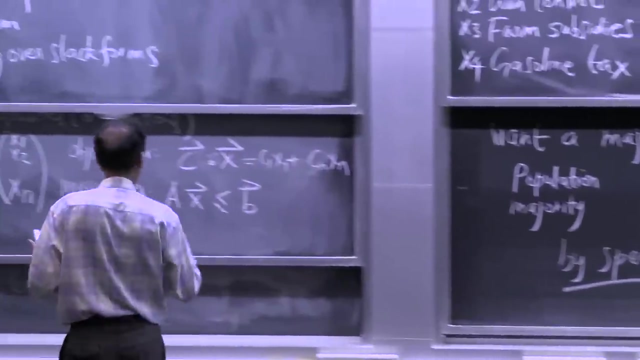 Sometimes you'll have greater than or equal to constraints. Sometimes you'll have equality constraints. We'll spend a little bit of time talking about how you can transform any given linear program into a standard form, right? So our standard form is going to be something that maximizes, or 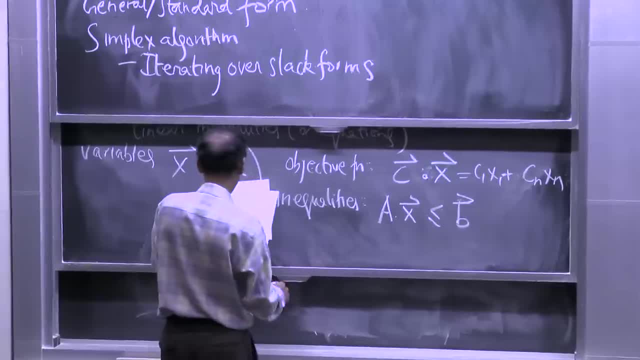 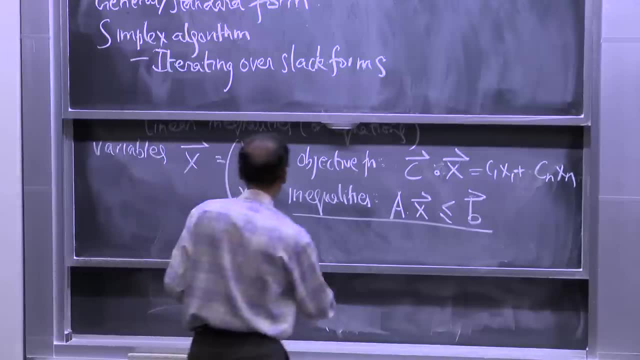 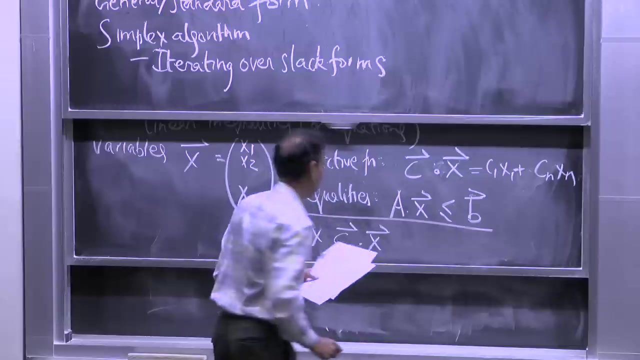 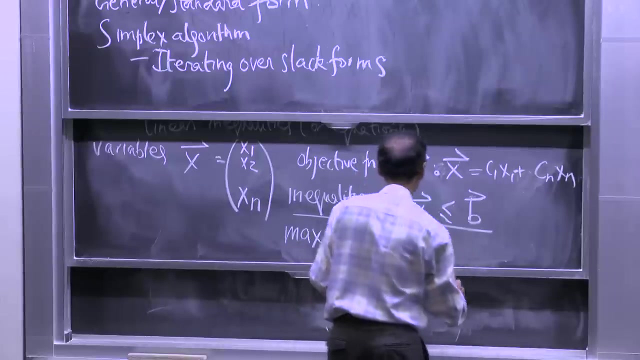 maximizes the objective function. So these are inequalities And they're represented as less than or equal to. That's the standard form. And you want to maximize c times x- Again max for standard, such that these set of inequalities hold Ax less than or equal to b. 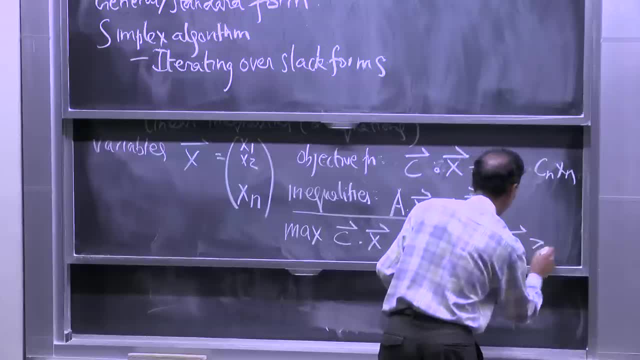 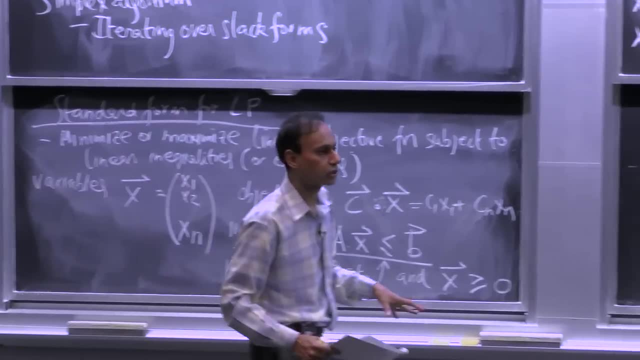 And as we go on, And as we go on. and x greater than or equal to 0. So, for each of the values that correspond to the variables, you want these variables to be non-negative in the standard form And you want less than or equal to corresponding. 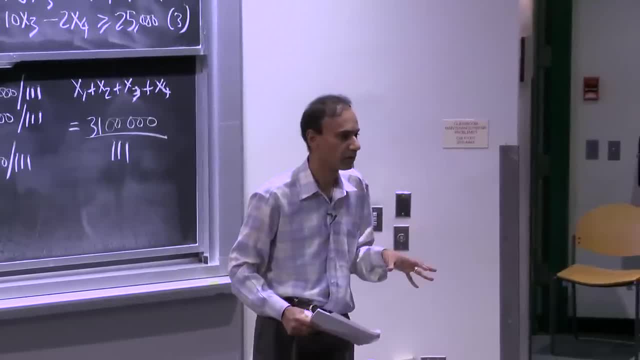 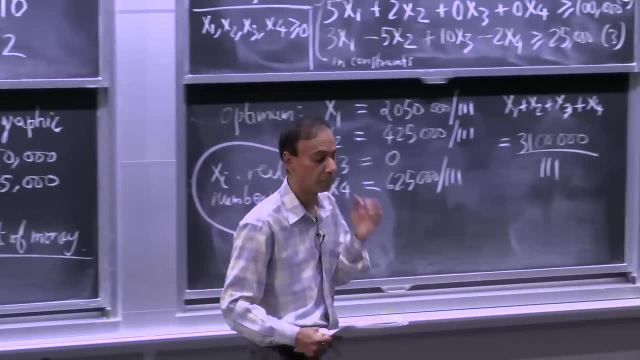 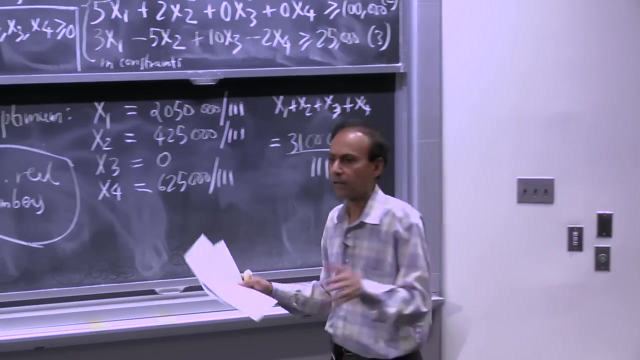 to each of the inequalities Not equal to, not greater than or equal to, but less than or equal to. And you have this linear cost function where you could have arbitrary coefficients, but you're maximizing it, So that's it. So it's all about polarities, not much more than that. 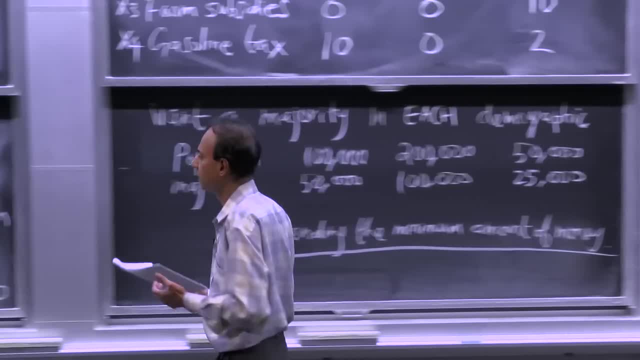 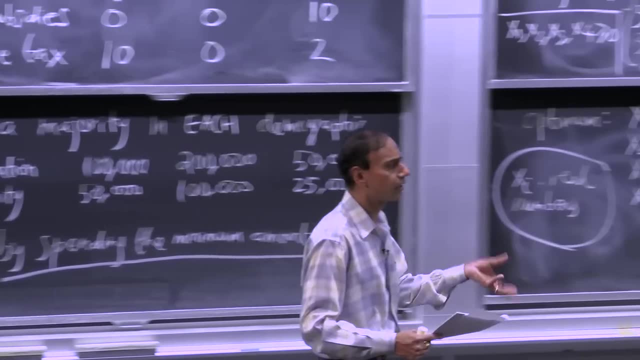 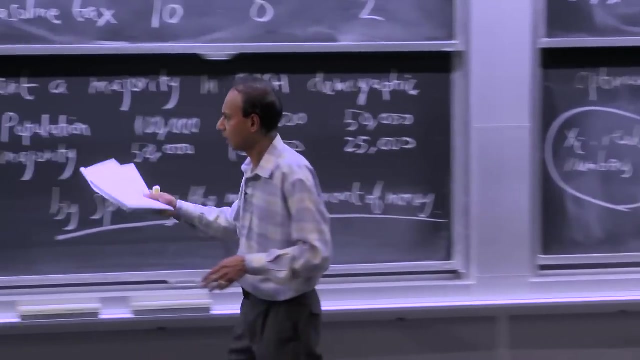 It's just about polarities, And if you get a specific linear program that doesn't conform to this, we'll spend a few minutes talking about conversions And it's going to be fairly straightforward. May not be immediately obvious, but we'll get to that. 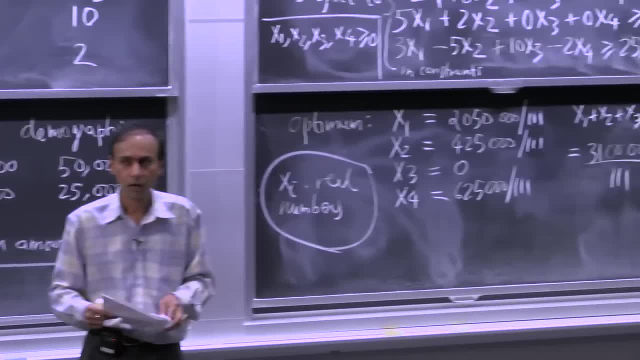 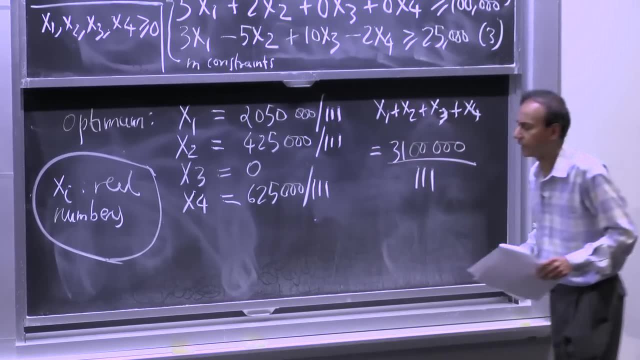 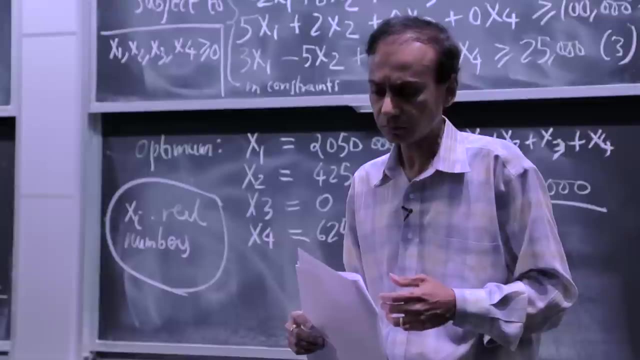 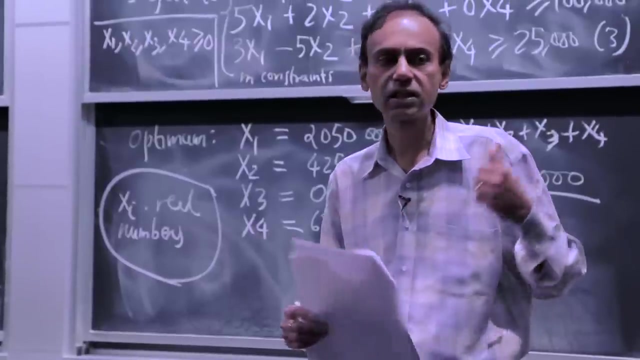 Any questions so far? OK. So I want to go back to this claim here where I said this was optimum. Now, without actually describing an algorithm to you, I'm going to be able to show you, convince you, that this value here, corresponding to whatever, 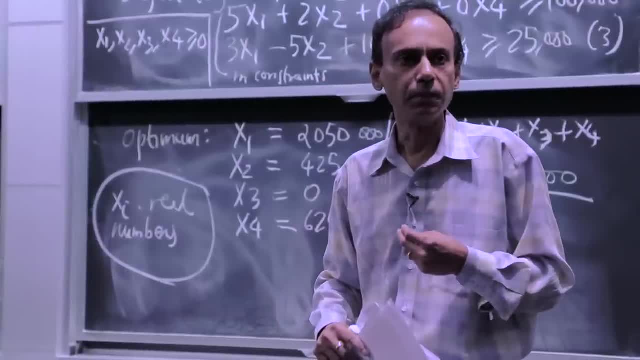 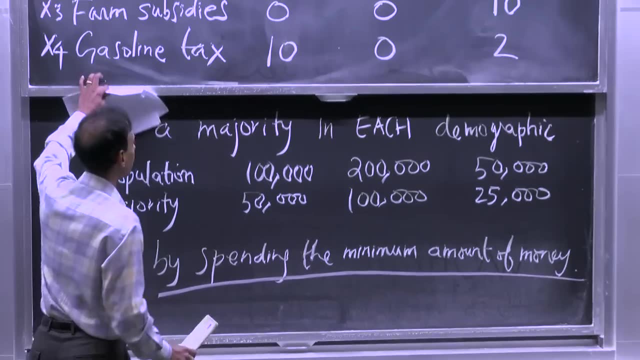 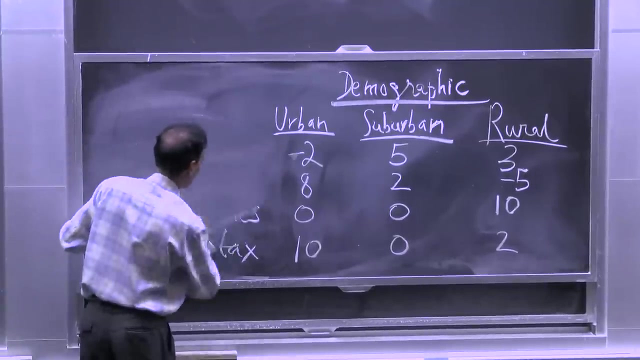 it is 3 million. 3.1 million is, in fact, optimum, Right, Right, And this is something I can do because linear programming has this powerful notion of duality. So what is that? Well, let's just first look at our specific example here. 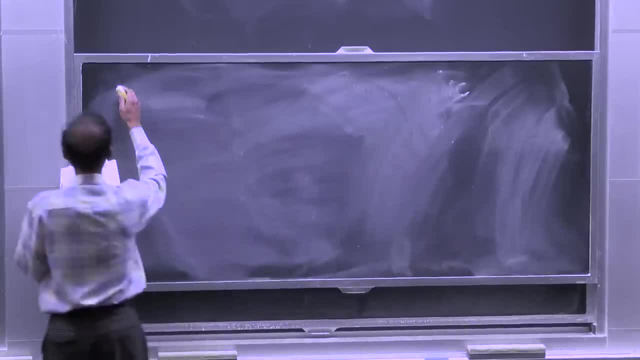 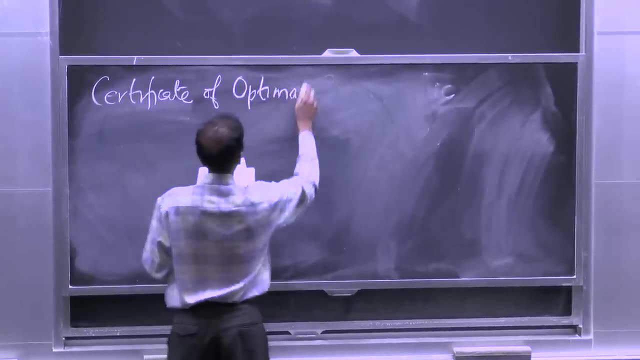 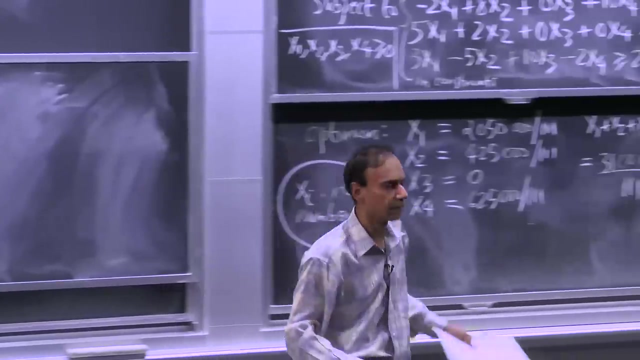 And I'll give you a very specific observation. I'm going to give you what you can think of as a certificate of optimality. OK, I'm going to give you a certificate of optimality for that set of numbers, And here's how I'm going to do it. 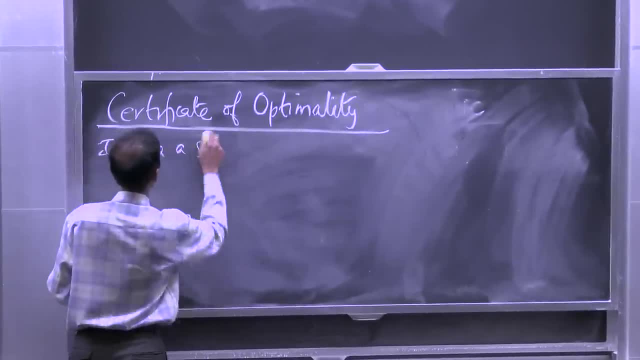 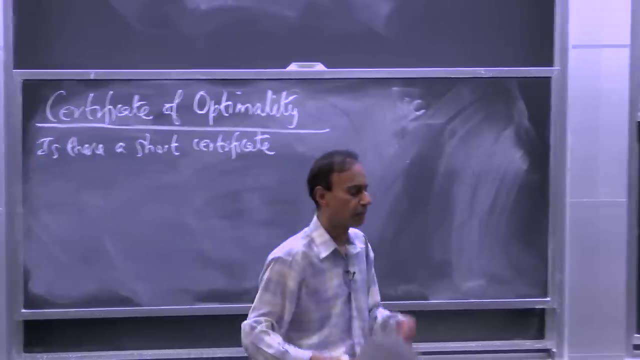 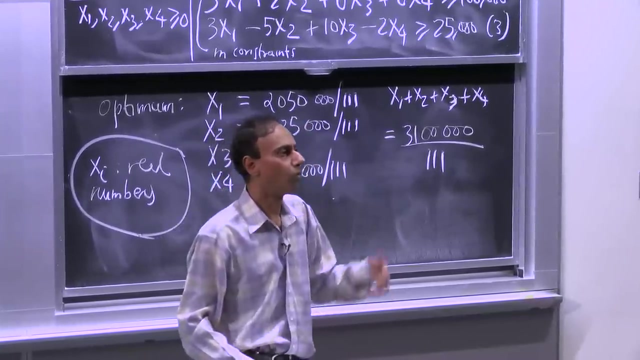 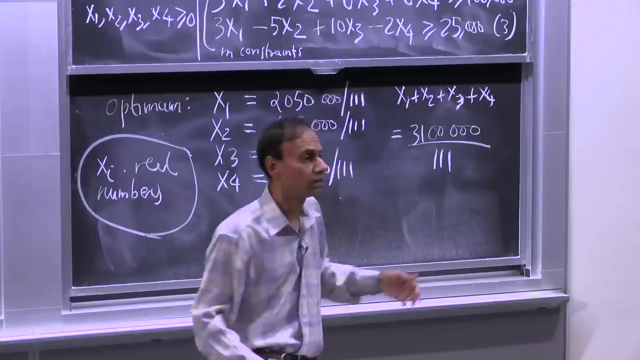 So is there a short certificate? I can imagine giving you a long proof that a particular linear programming algorithm always gives you the minimum answer, the optimum answer. Walk through that, Execute that algorithm on this particular example, And then you're convinced, of course. 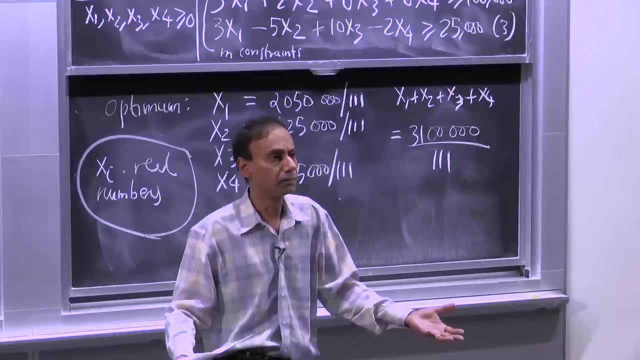 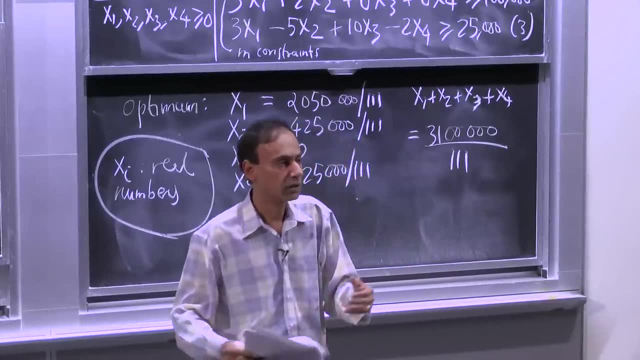 that the solution is going to be optimum, But for this specific example, I want to give you a certificate. This certificate isn't going to work for other examples. It's going to be short because it only works for this example, But it won't work for other ones. 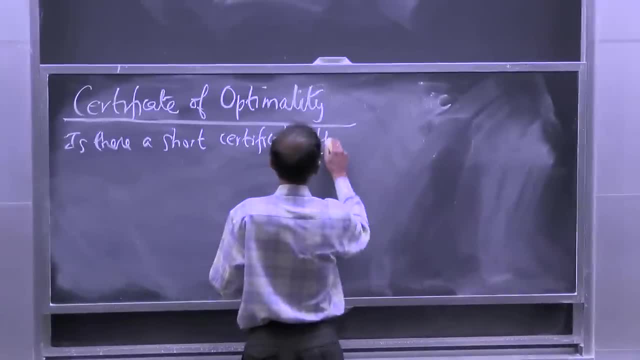 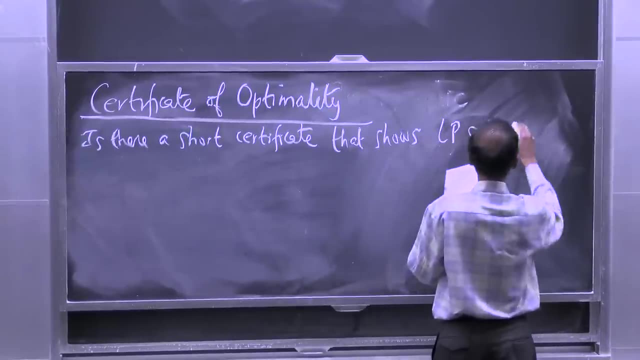 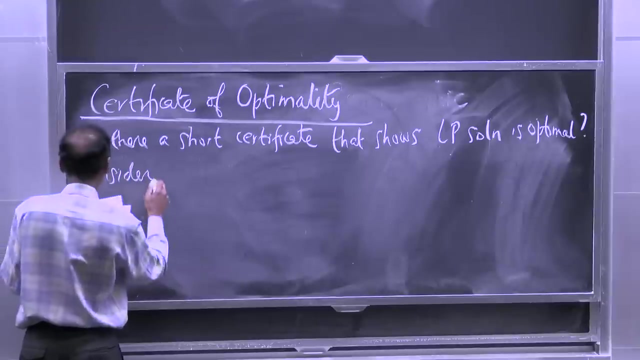 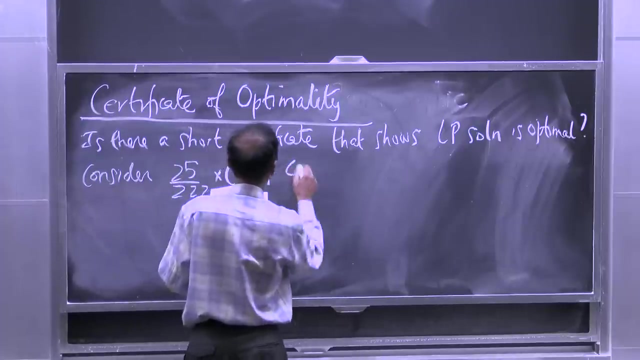 OK, And so how do I do that? So the answer is: I'm going to give you a certificate, OK. OK, The answer is, in fact, there is a certificate that shows that the LP solution is optimal. And consider that I compute this particular algebraic quantity. 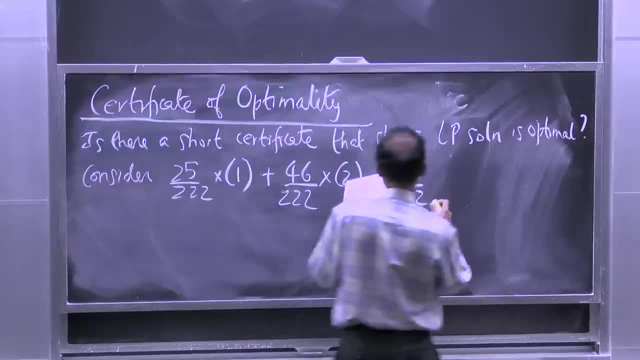 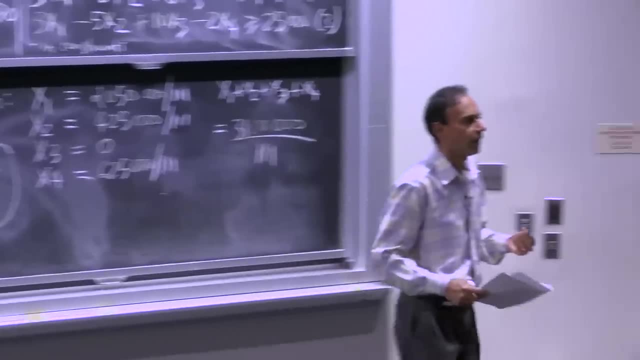 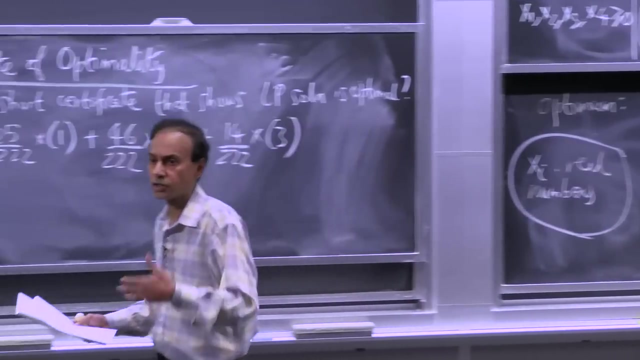 where All I've done is I've taken these three equations and I've multiplied them by these magical constants, And so I'm not going to tell you how we get this certificate of optimality, But I'm going to give you the certificate. 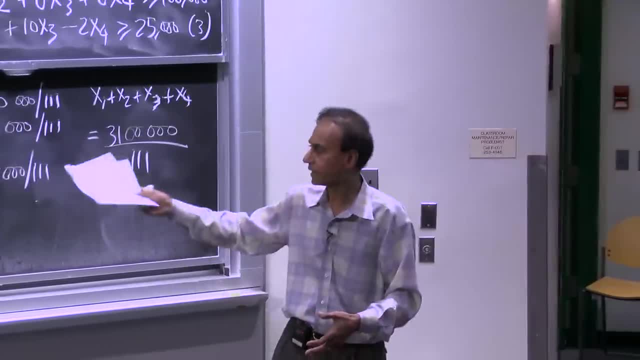 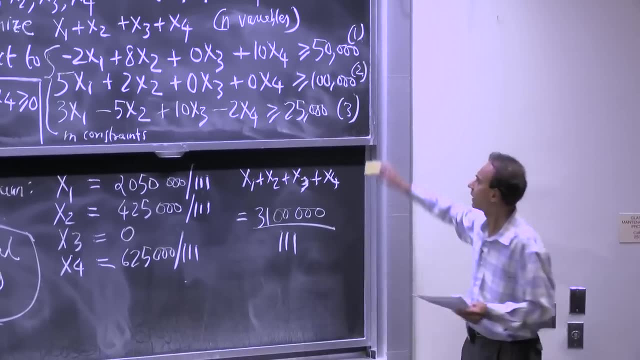 And it's going to be clear that it's a certificate of optimality, And if I take these three equations here, 1,, 2, and 3.. So when I refer to 1,, 2, and 3, they refer to the equations. 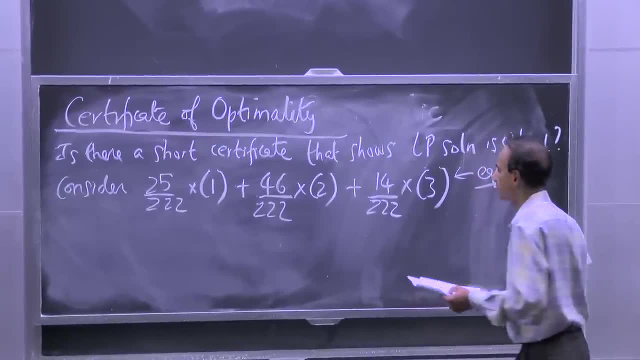 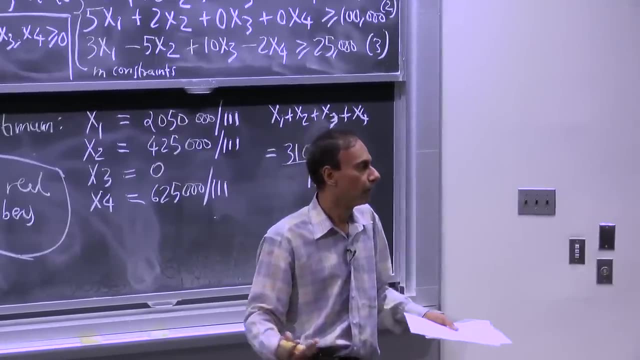 These are equations or constraints, And so I take that And obviously, if I have a bunch of equations and I multiply them out, I can certainly add them up And I get another equation at the end of it. Right, And it's all going to be linear. 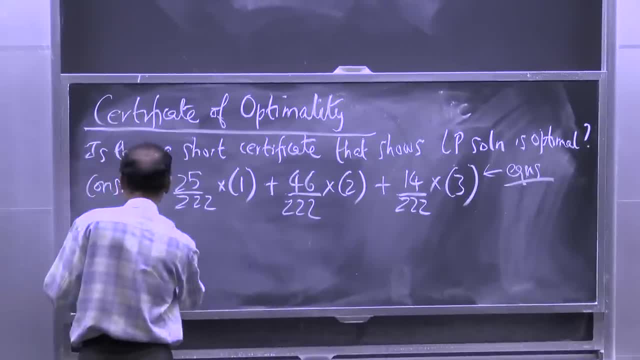 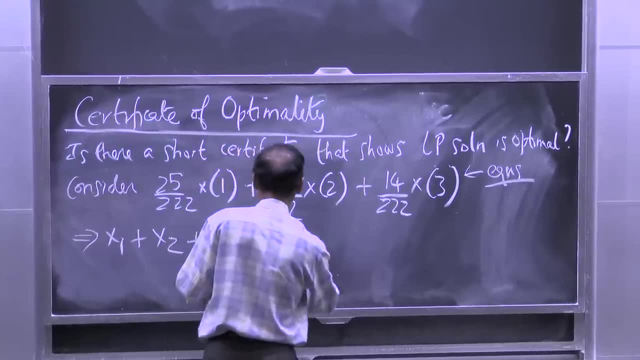 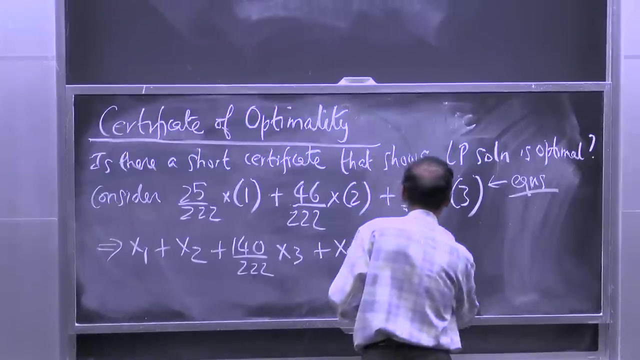 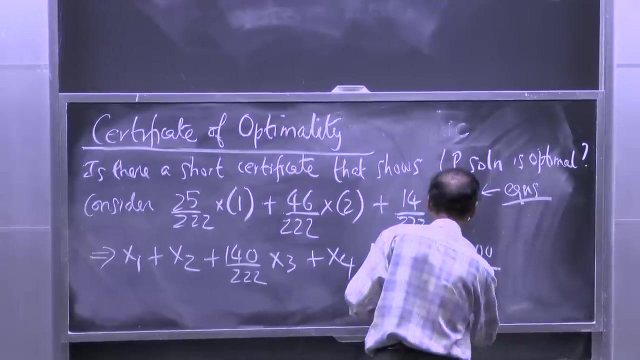 And if I do that, I get x1 plus x2 plus 140 divided by 222 times x3 plus x4.. So that's what happens to the left-hand side, And the right-hand side is- you'll recognize this quantity- five 0's divided by 1, 1,, 1.. 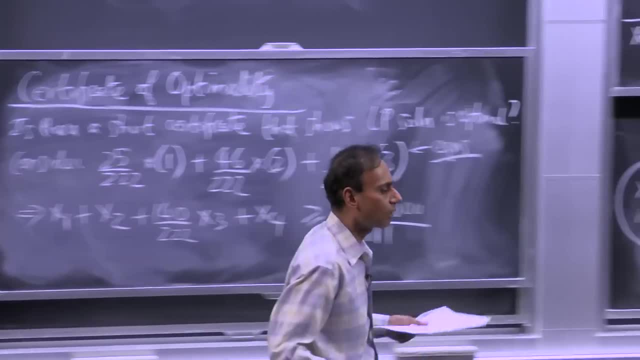 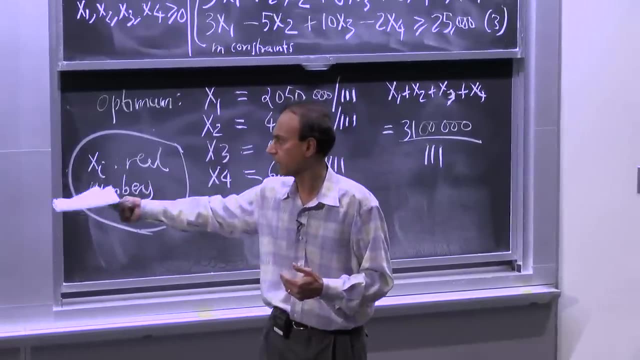 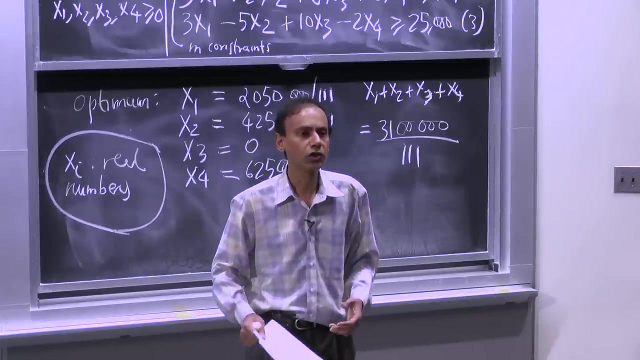 OK, That's what you get. So now can someone tell me why last step? why this is a certificate of optimality, The fact that obviously, this is all algebra once I've discovered the coefficients. So, now that I've done this, why have I just shown you? 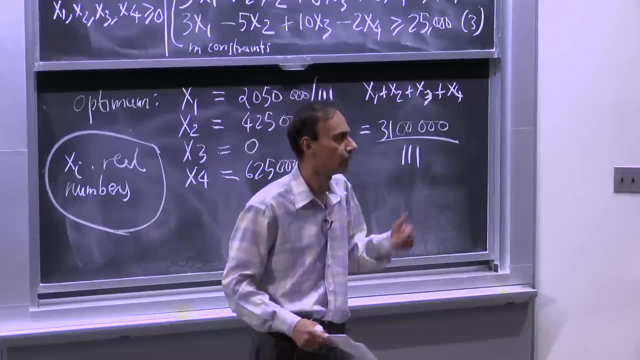 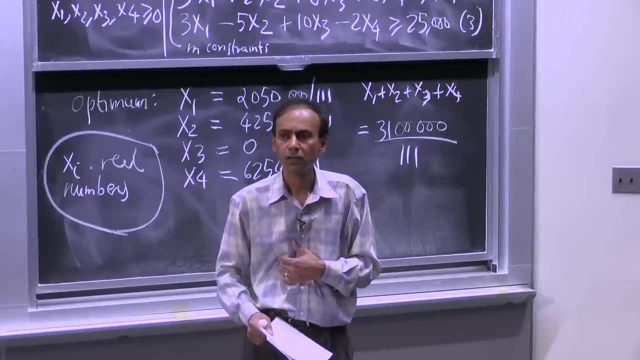 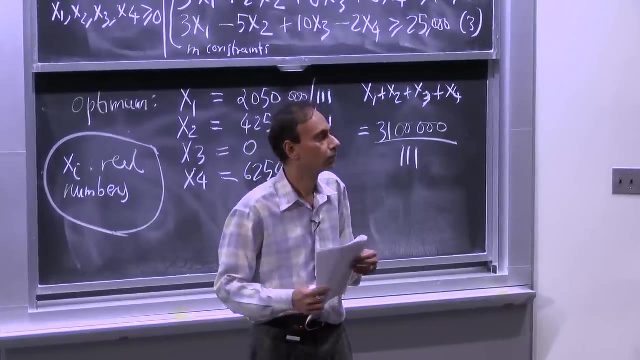 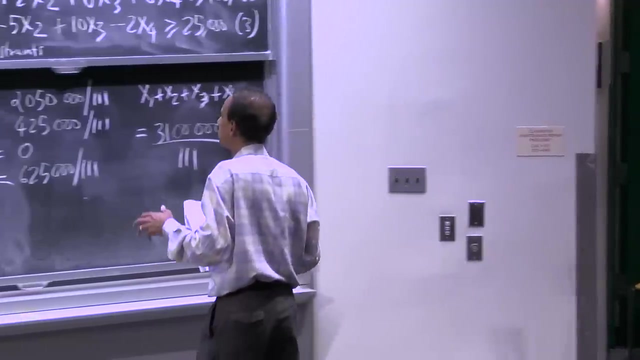 that 31, 3.1 million divided by 1, 1, 1 is, in fact, optimum. Can someone tell me this? Look at what you have on the left-hand side. No Yeah, SRINIVAS DEVADAS- Any other solution? 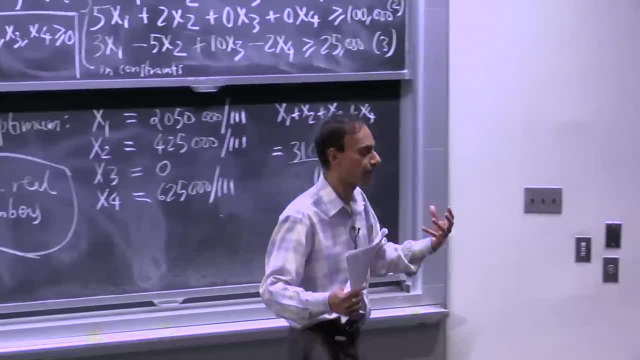 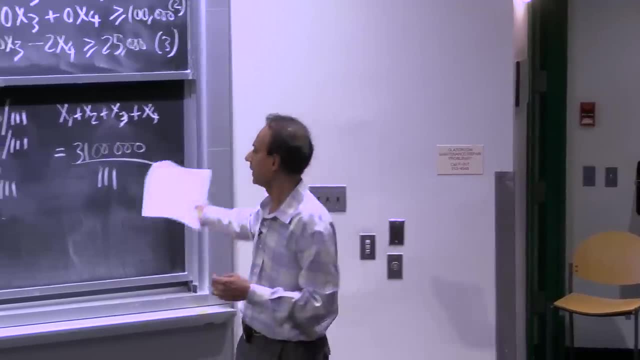 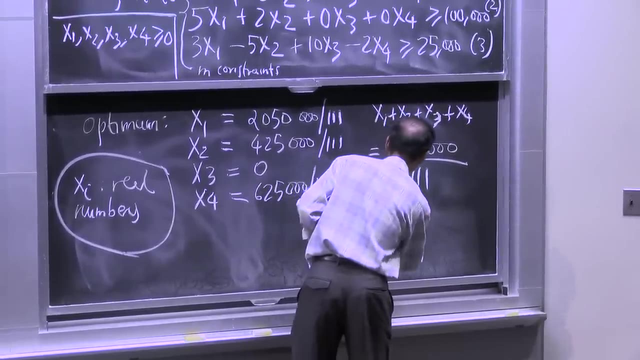 But I want you to relate that to what am I spending? SRINIVAS DEVADAS- Yeah, but I mean, this was a claim, This was a claim And, at this point, an unproven claim. It was an unproven claim. 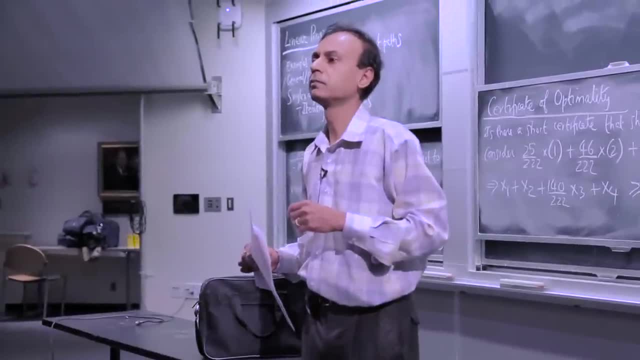 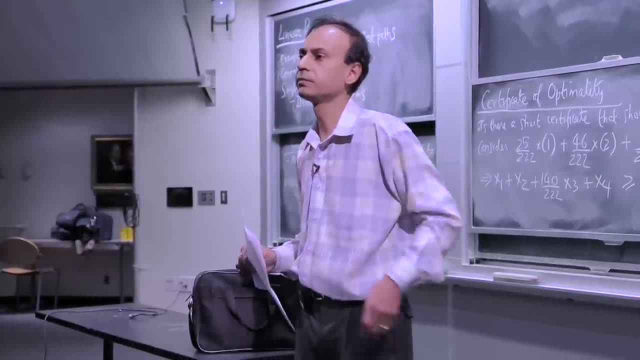 Yeah, go ahead. SRINIVAS DEVADAS- Correct, And what is x1 plus x2 plus x3 plus x4, to be clear? SRINIVAS DEVADAS- Yeah, exactly. 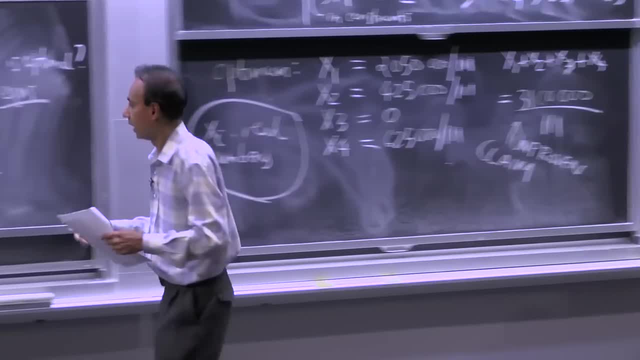 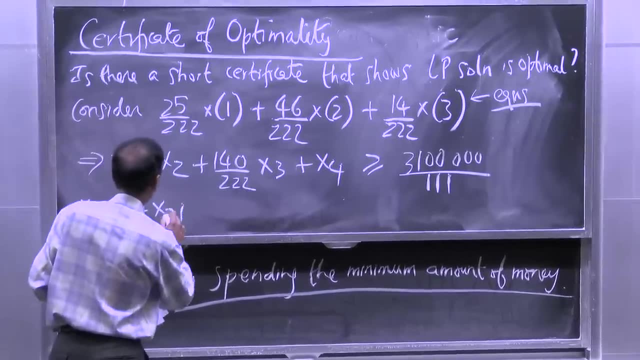 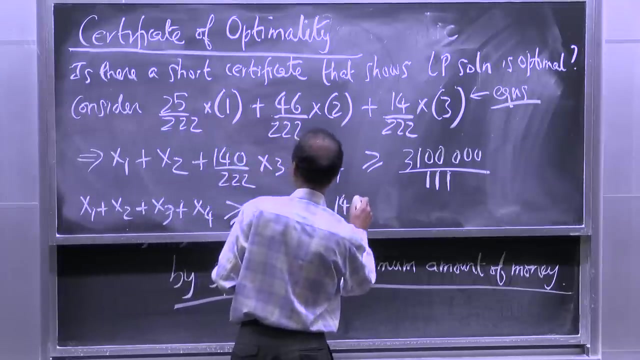 The thing you're trying to minimize. Exactly Right, You're almost there. But the key observation here is that x1 plus x2 plus x3 plus x4 is greater than or equal to x1 plus x2.. Because all of these are positive quantities, remember? 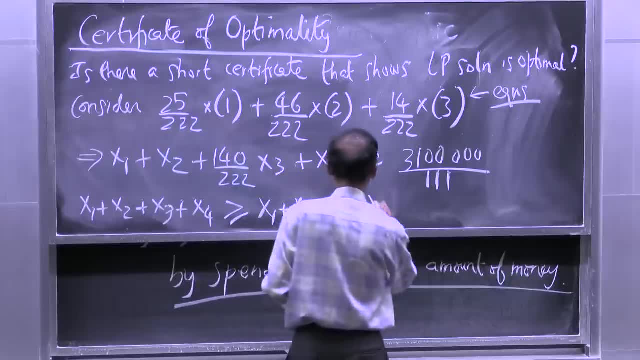 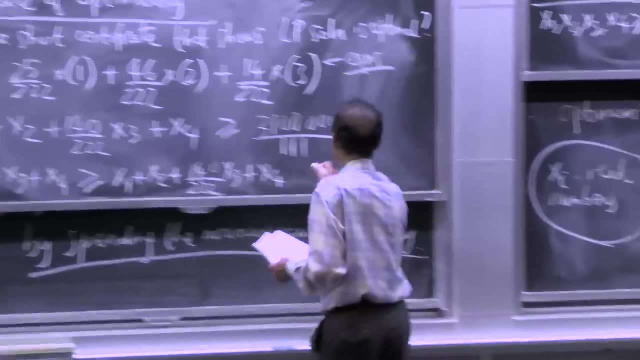 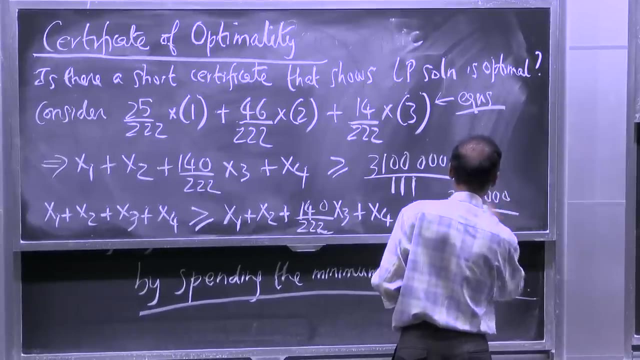 140 divided by 222, that's less than 1.. x3 plus x4. Correct. So, given that I can say that This is greater than or equal to 3,100,, five 0's, 1, 1, 1.. 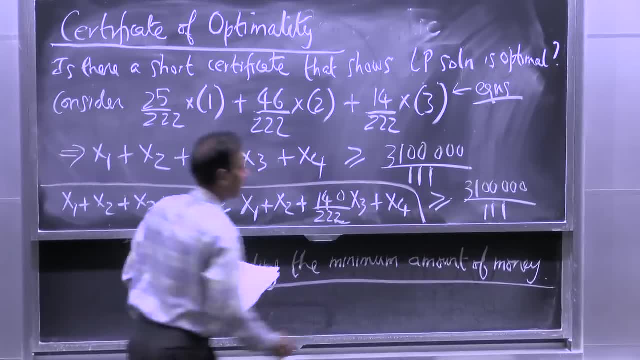 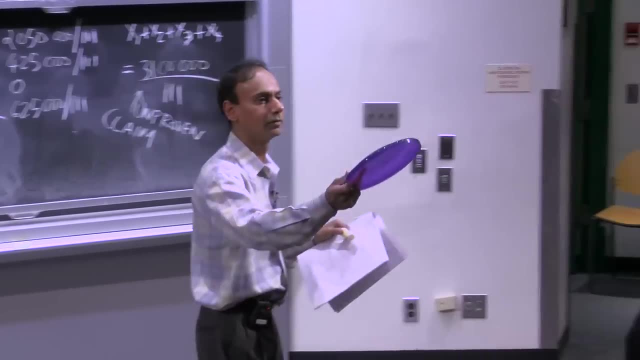 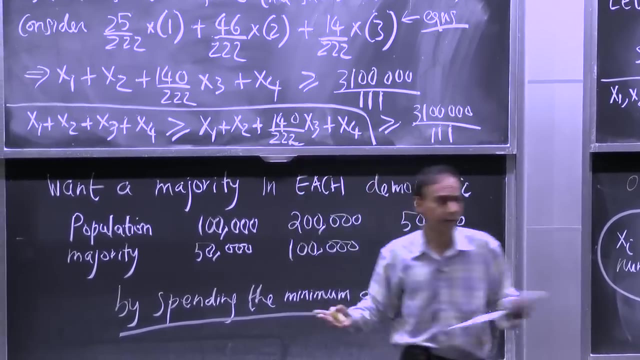 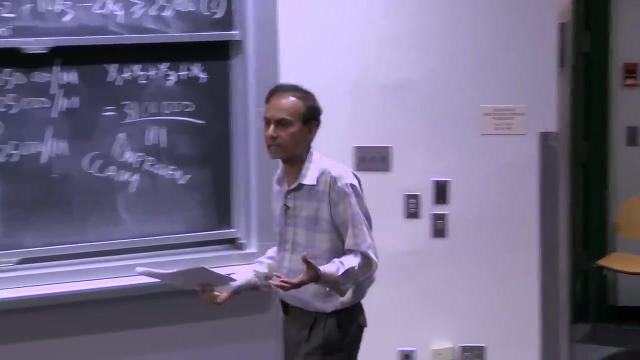 Right, It's because of this observation that it's a certificate of optimality. Right, She has her head down, OK Great, So that's pretty cool. Right, Just cooked up These coefficients from somewhere. Pull them out of a hat. 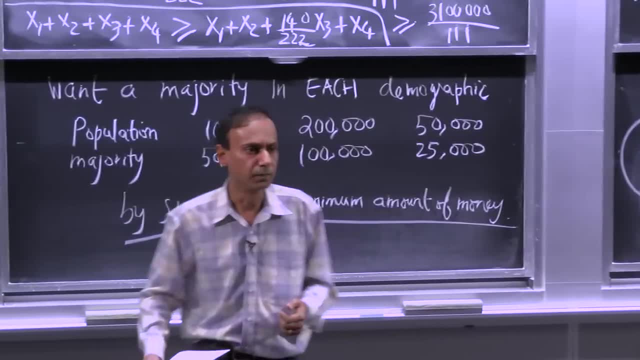 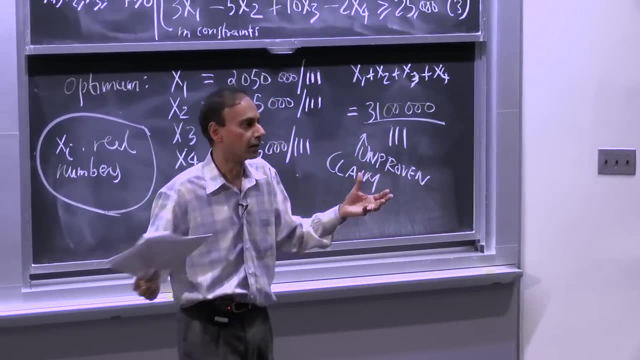 You're all convinced now that the value we got was optimum. Did not run an algorithm. Maybe I ran an algorithm. Of course you ran an algorithm to get those coefficients Right. How did those coefficients appear? So we're not going to spend a whole lot of time on this. 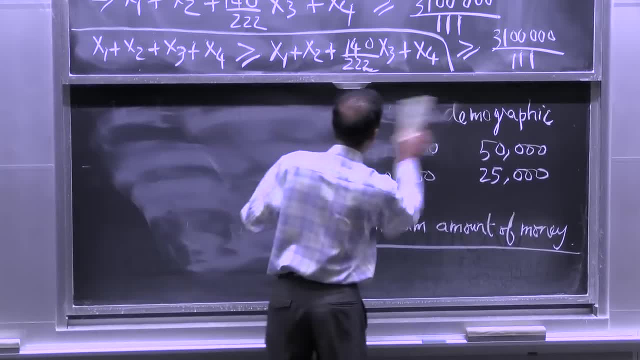 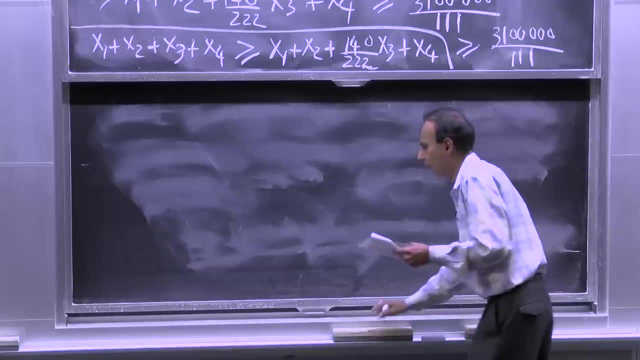 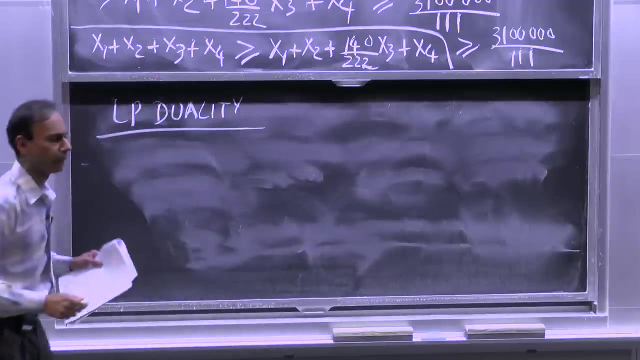 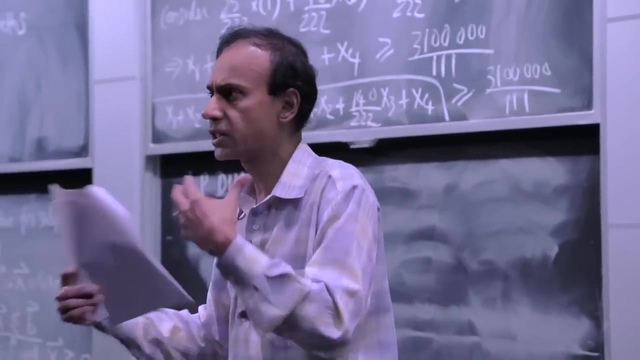 You'll see this likely in a problem set or perhaps in section, But in general I won't worry too much about duality other than knowing the concept And this notion of LP. duality essentially says that what just happened wasn't a coincidence. 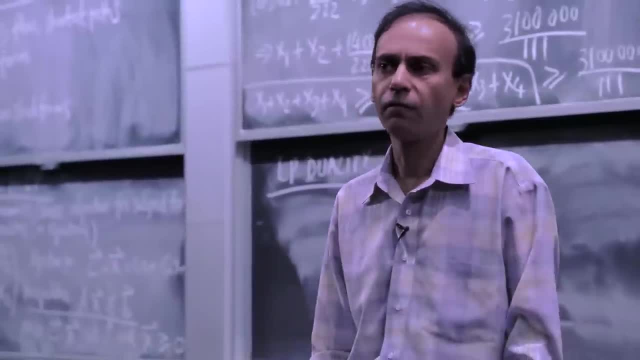 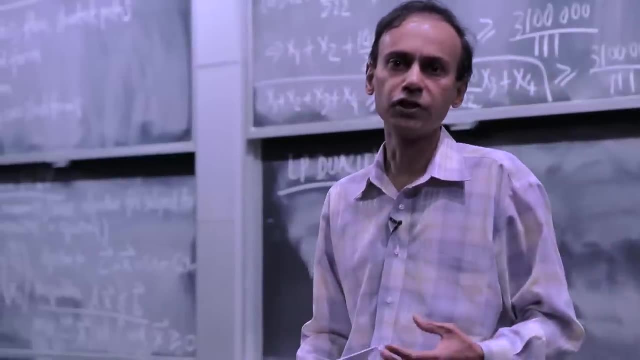 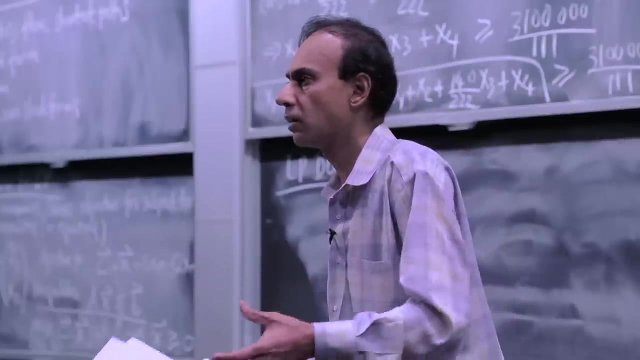 You can do this all the time. There will always be for a linear program, a short certificate of optimality that corresponds to some set of coefficients that you can do this particular math with by taking these linear constraints, multiplying them out, adding them up together and showing. 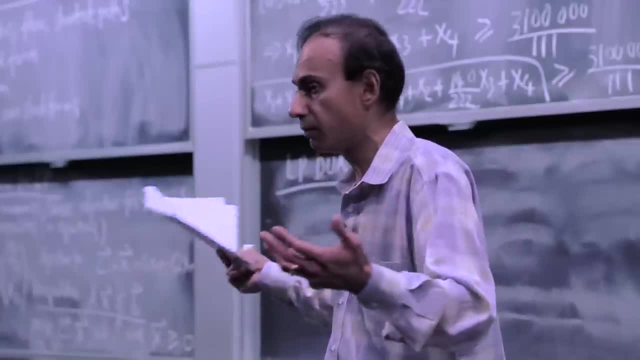 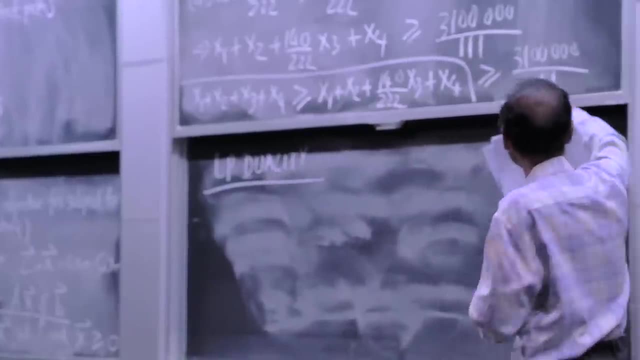 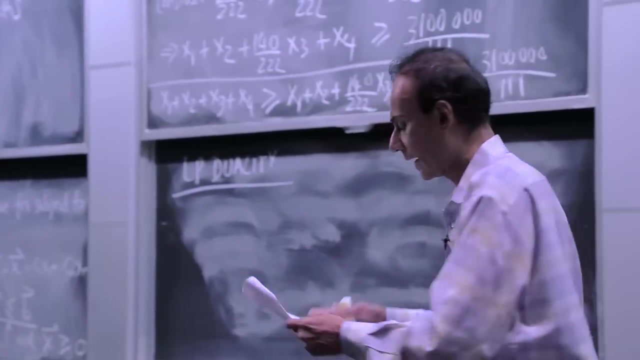 that you have a lower bound. in the case of this problem, You can't get lower than this And therefore, for a minimization problem, when you reach that, you've clearly found the optimal, And that's the notion of LP duality. 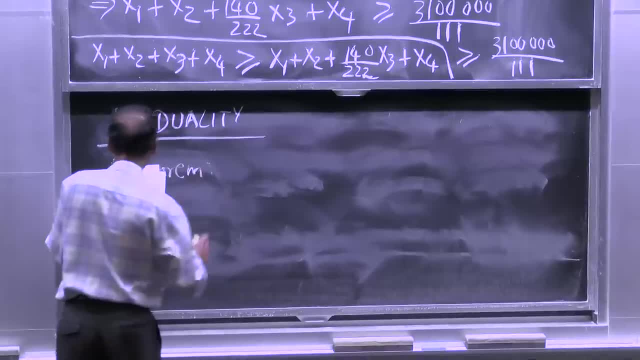 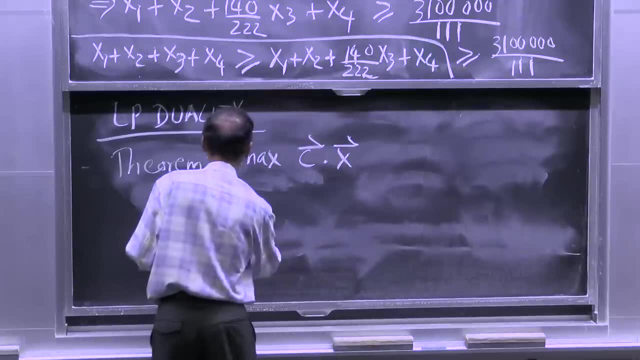 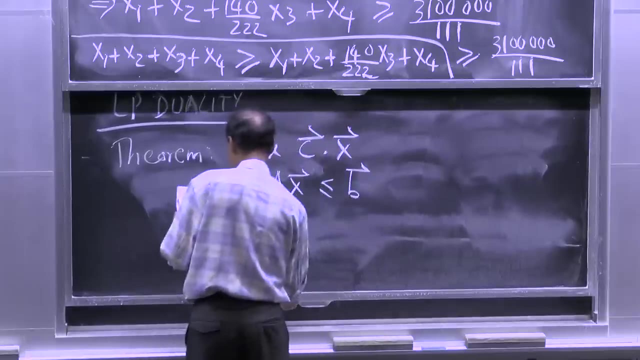 And the. The basic theorem- and this is really more as an FYI- we won't prove this theorem- is that if you had the standard form for the LP, which I'm just writing down again here, where you had ax less than b, 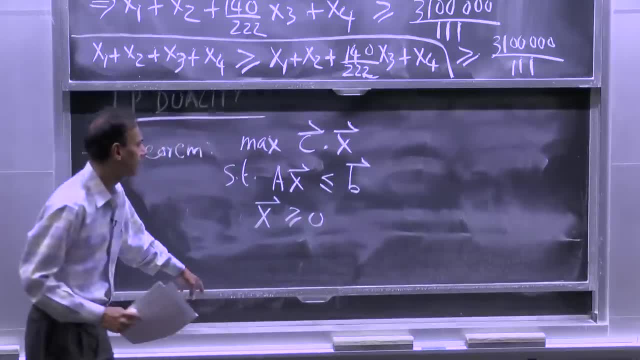 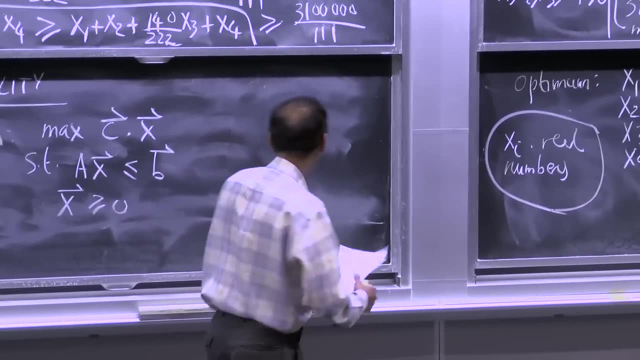 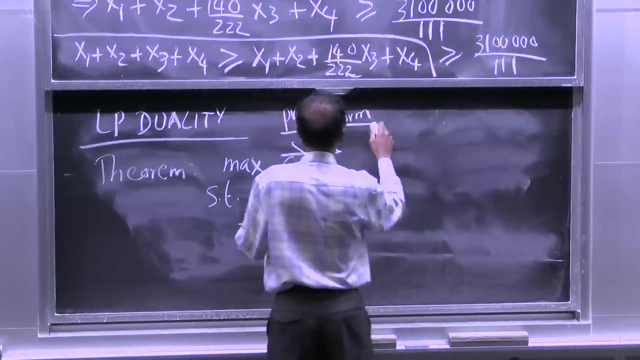 x vector greater than or equal to 0. So that's identically what I had up here or down here, corresponding to the standard LP form. Well, there's a dual. this is what's called the primal form. Usually, if you don't say it, you think of it as a primal form. 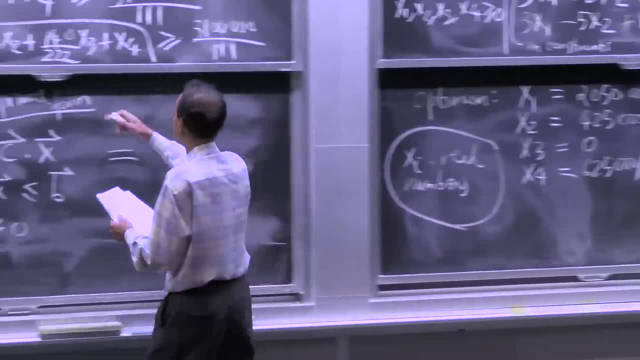 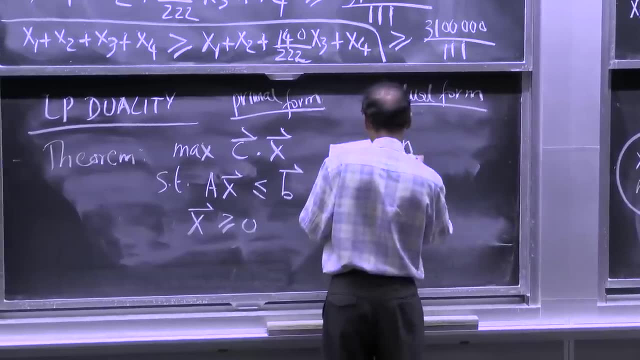 And if it's dual, you call it a dual And this is a primal form of LP, This is a dual form of LP or dual LP, And the dual LP flips everything And it's not just negation but transpose. 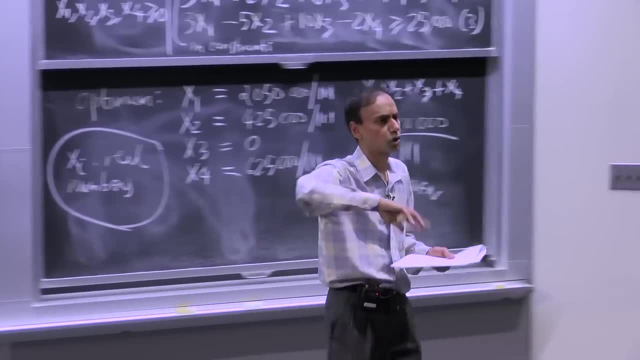 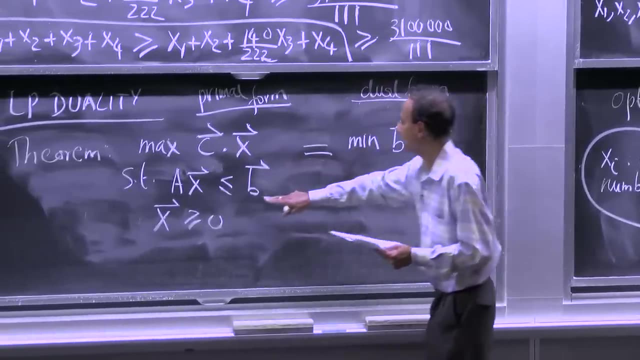 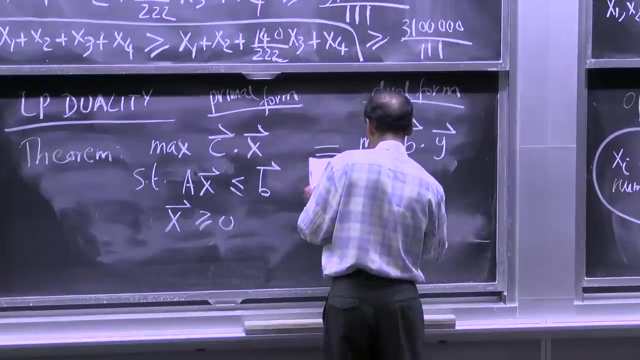 And the actual variables also swap functionalities, So it's really pretty cool. So your max turns into a min, The c gets replaced by the b, which is on the right-hand side of the inequalities, And your constraints are: a. transpose y, greater than or equal to c. 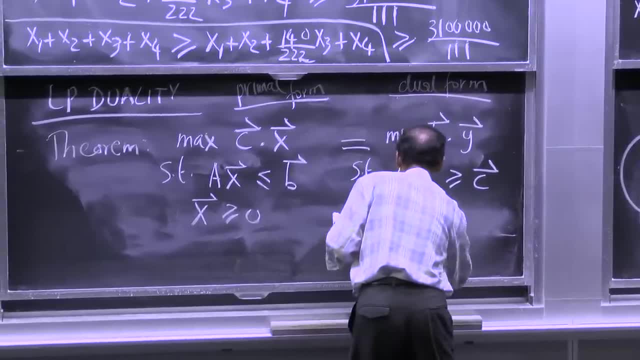 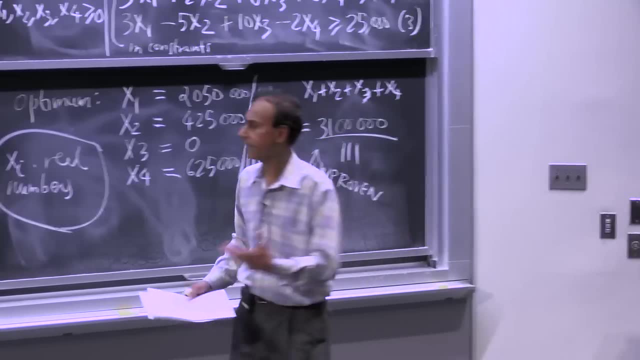 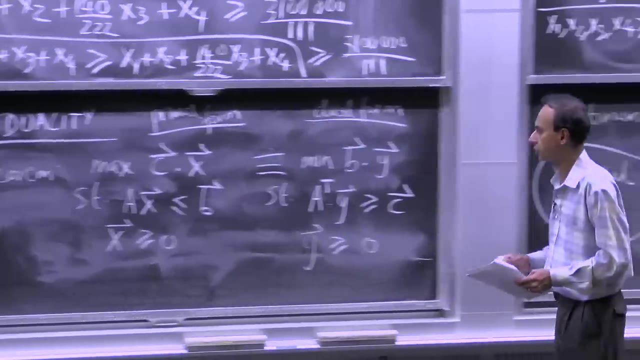 So there's a flip there as well, And y is greater than or equal to 0. So there's a bunch of things that's going on here And these two problems: They end up being equivalent, The primal and the dual. you can always do this. 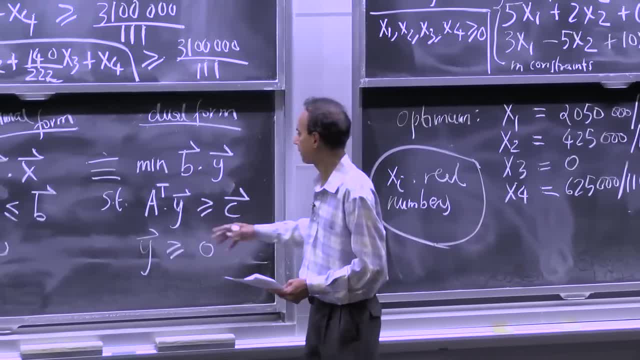 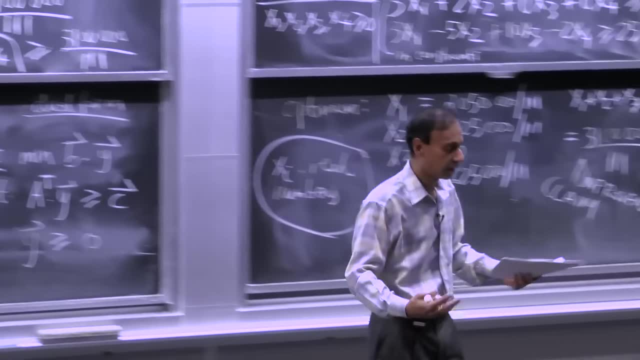 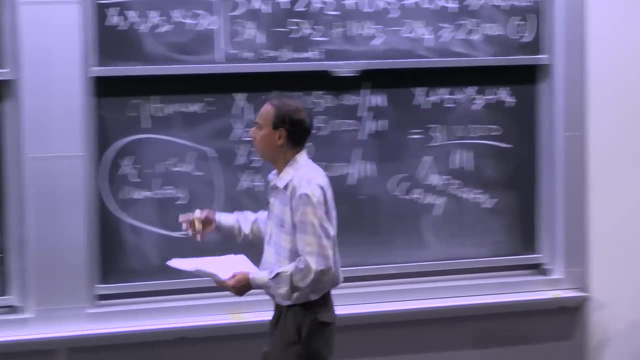 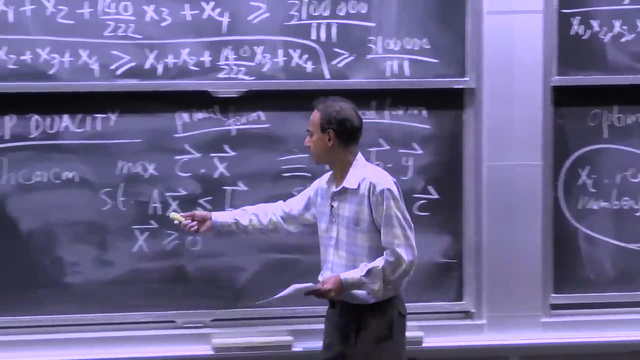 And essentially what is happening here is that you're solving these two problems simultaneously And there's lots of algorithms that keep flipping between these two forms for efficiency, But ultimately what ends up happening is, you see, that the the actual constraints that you had here corresponding 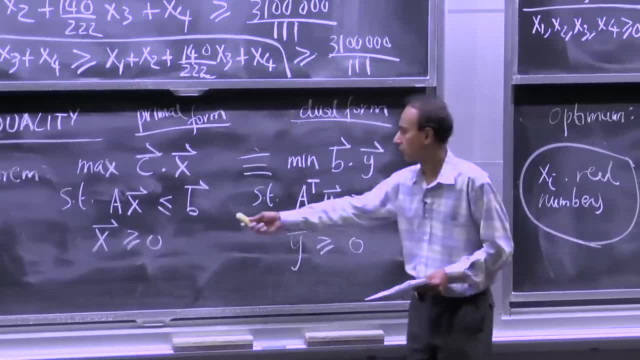 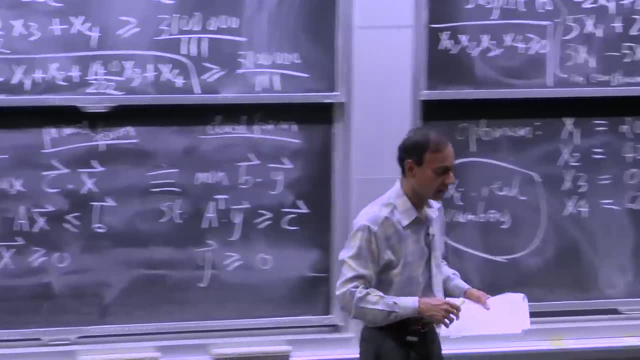 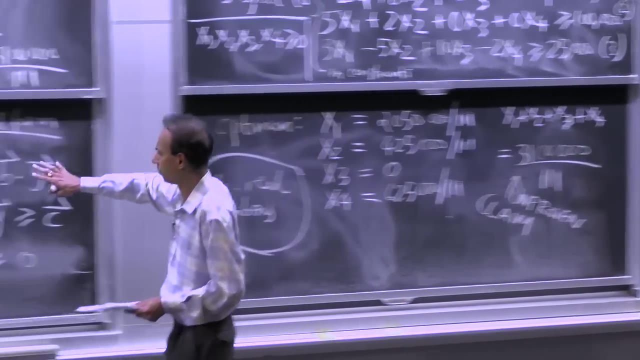 to the b constraints turn into the. b ends up in the cost function here, And that's essentially what's happening out here with respect to multiplying these equations out with particular coefficients. So, as I said, this is really more as an FYI. 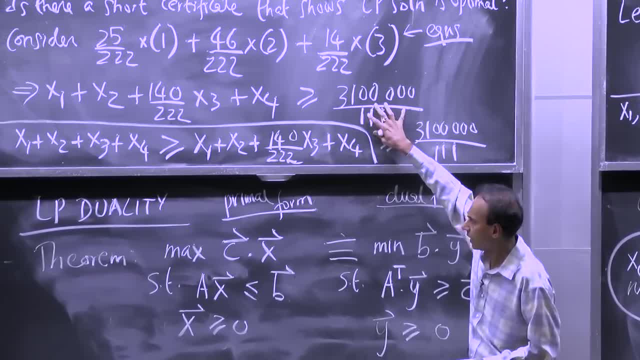 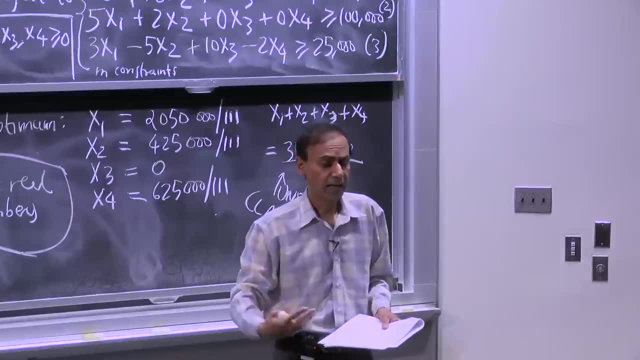 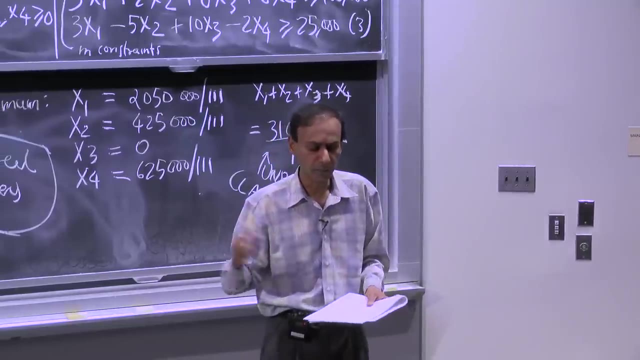 This is an obviously interesting and an interesting proof of optimality, which is a different kind of proof from proving an algorithm correct and applying that proof to a particular instance. And that's the kind of thing that happens in LP, especially when you flip from primal and dual forms. 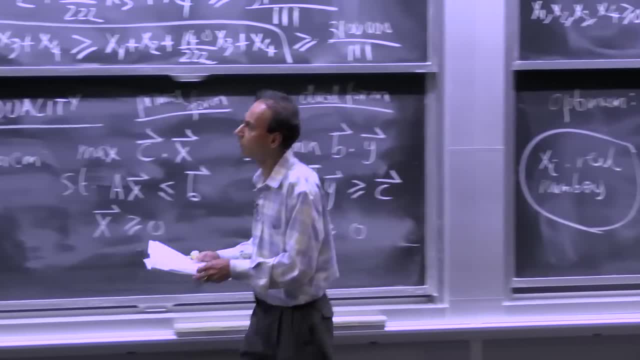 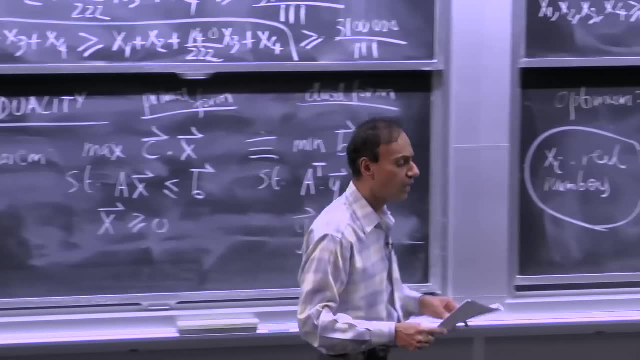 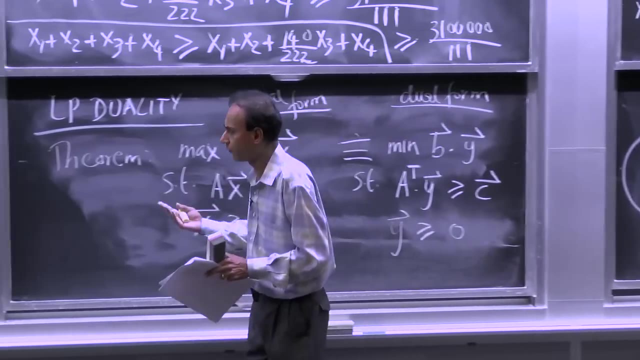 So I'll leave it at that. What I'd like to do is give you a sense of how we can convert to standard form so you can apply an algorithm that, for example, you have a program and it only requires standard form. It runs on standard form. 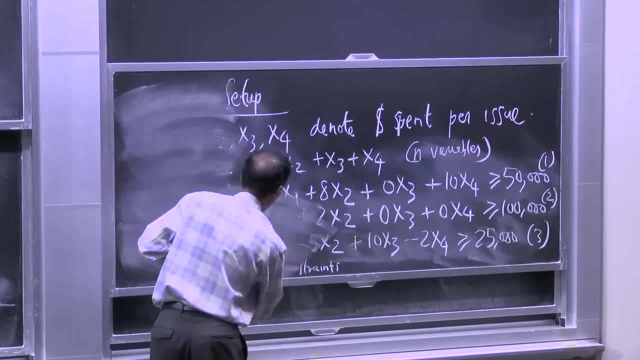 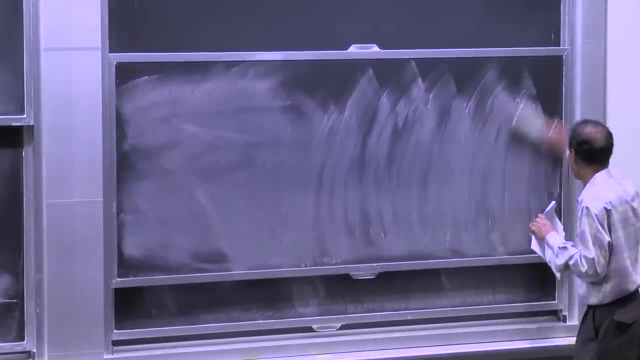 Let's go over really quickly- This is not going to take very long- A translation from different kinds of LPs- And we had a slightly different one here for our political problem that had a minimization, And how would we convert that to standard form? 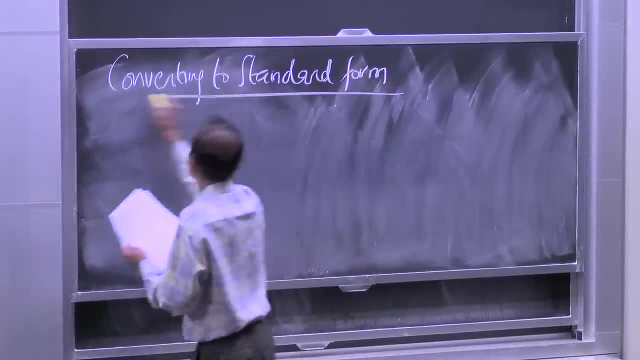 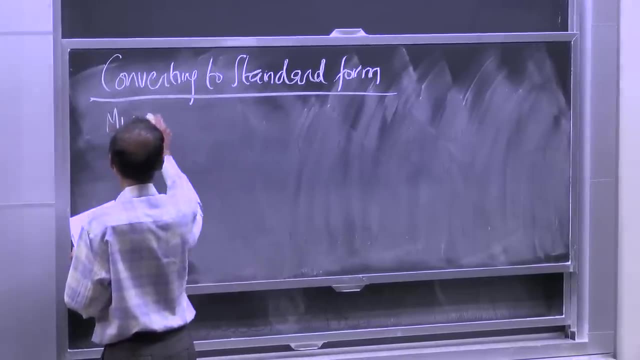 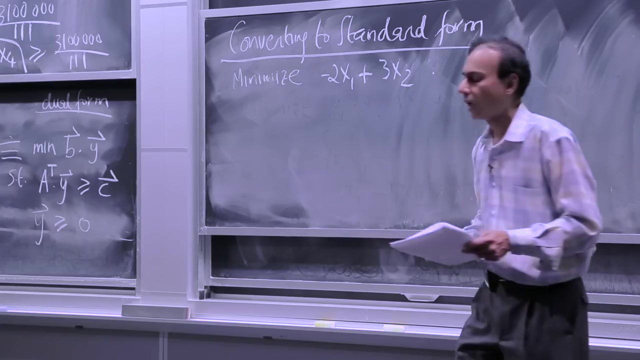 There's probably just one conversion here. that's tricky. So suppose I want to minimize minus 2x1, plus 3x2.. And I want to convert to standard form. All I have is a standard LP solver. What do I do? 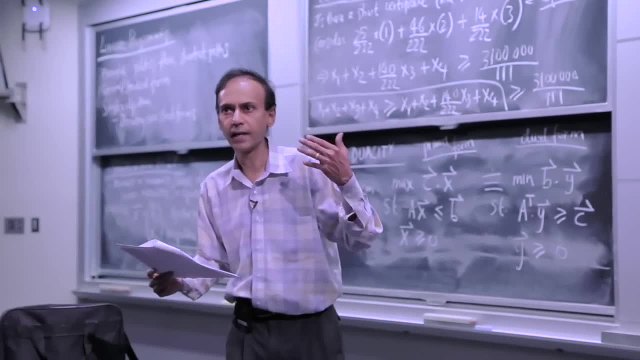 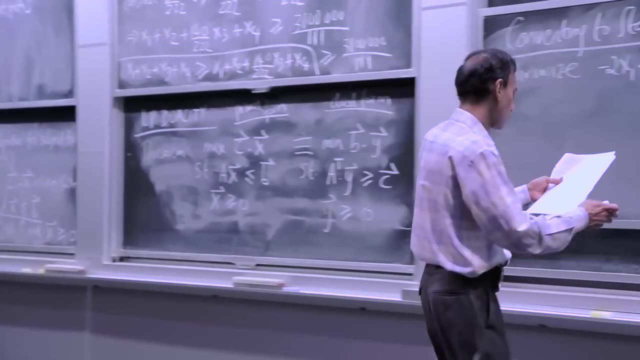 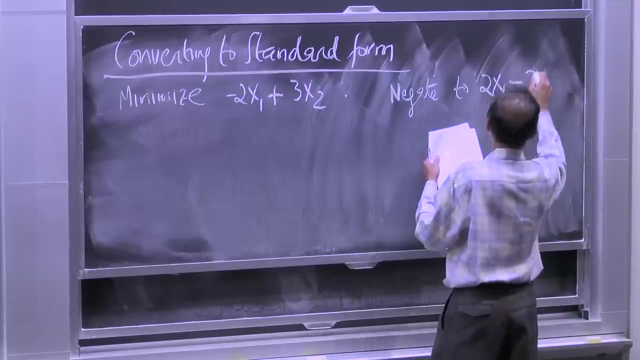 Should be easy. What do I do? What do I do? I had a solver that was maximizing, but I want to minimize the quantity. Just switch the signs right, So negate to 2x1 minus 3x2 and maximize. 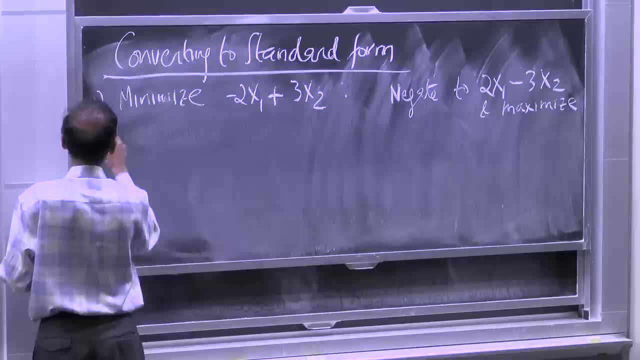 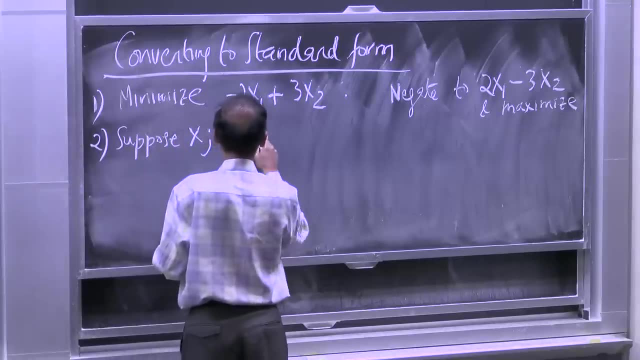 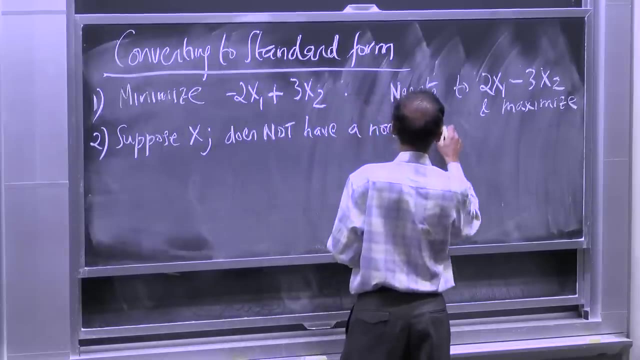 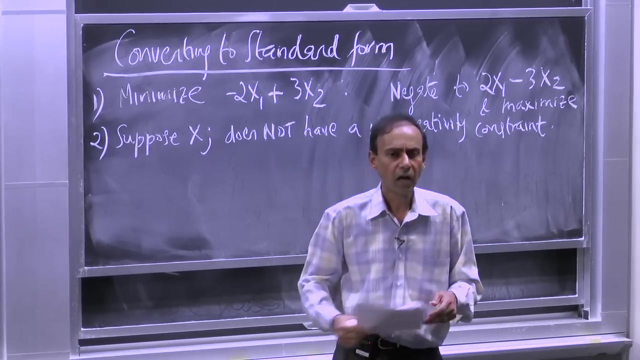 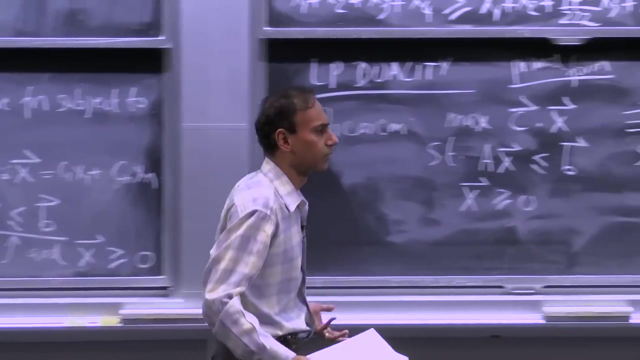 So that was easy. This is a tricky one. Suppose xj does not have a non-negativity constraint, So it just happens to be the case that it's not dollars but it's some other quantity that can go negative. It might be profit or loss. 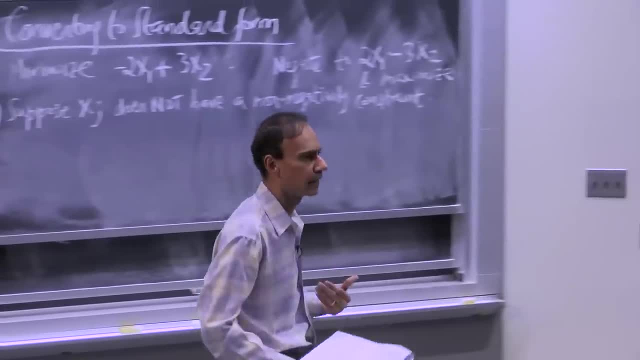 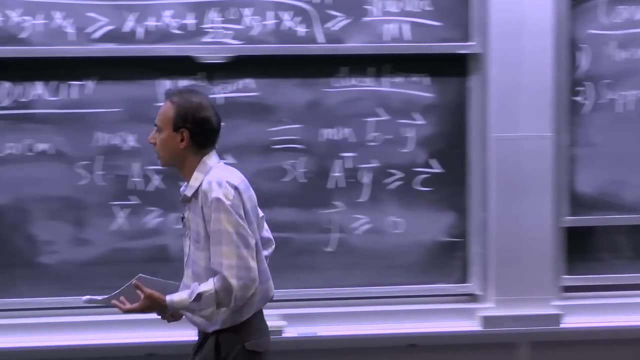 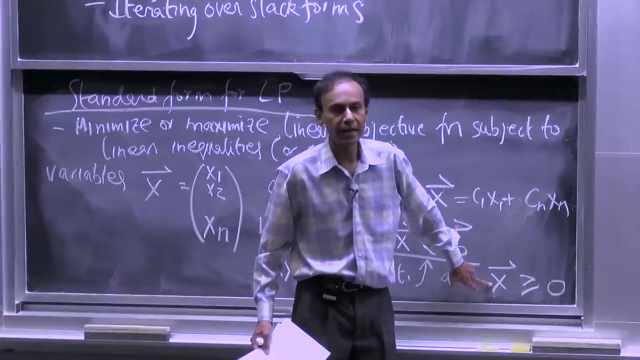 So that quantity represents profit or loss. so it could go negative if it's loss. So I don't have this constraint in my original problem specification. But my standard form and my LP solver requires this entire vector to be non-negative. So I got a problem here. 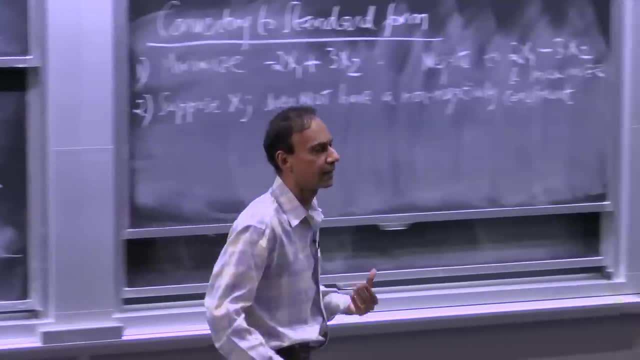 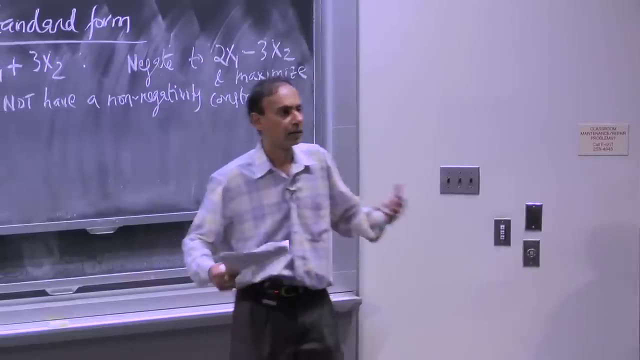 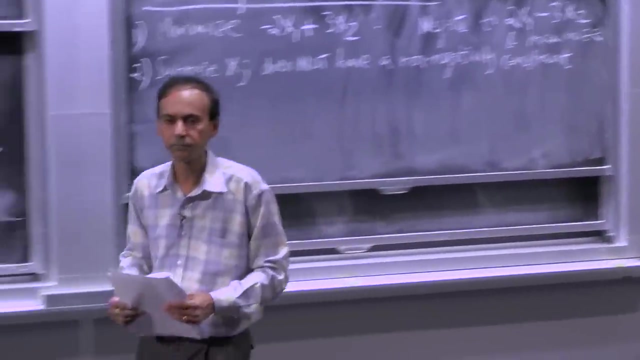 I can't use my standard solver because of this non-negativity constraint. So how do I fix that? How do I turn it into a problem that allows the standard solver to be used? Yeah, go ahead. You can break it up into two variables. 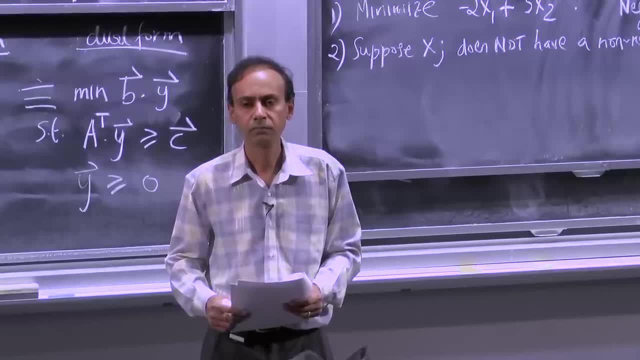 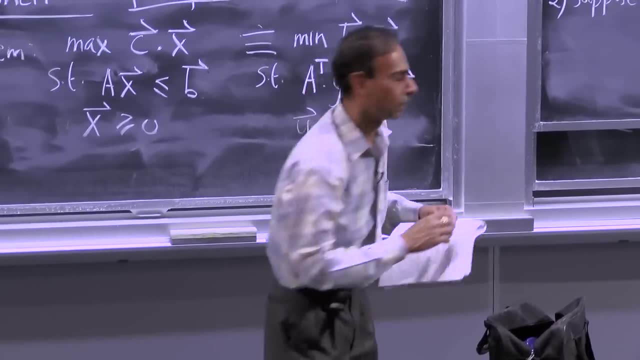 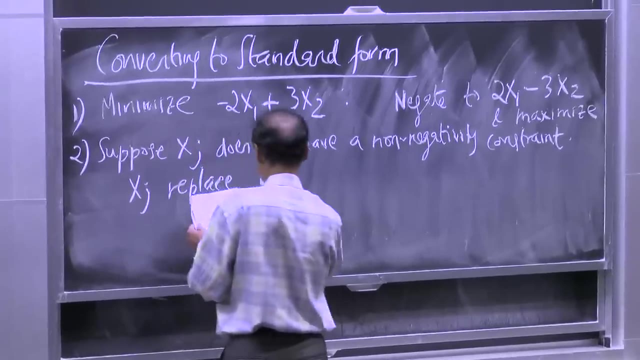 like xj1 and xj2.. Because xj1 minus xj2 equals xj, you go three times Perfect, Great, That's good. There you go. So what you do here is take xj and replace it with, let's say: 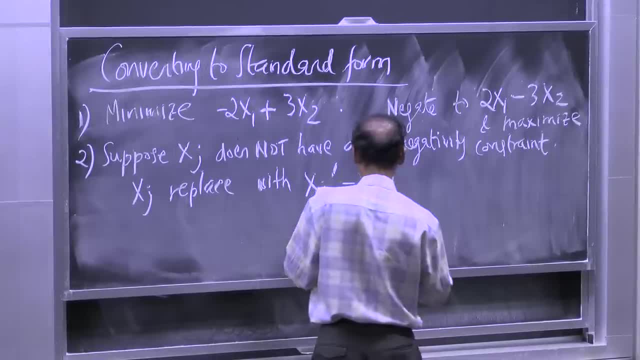 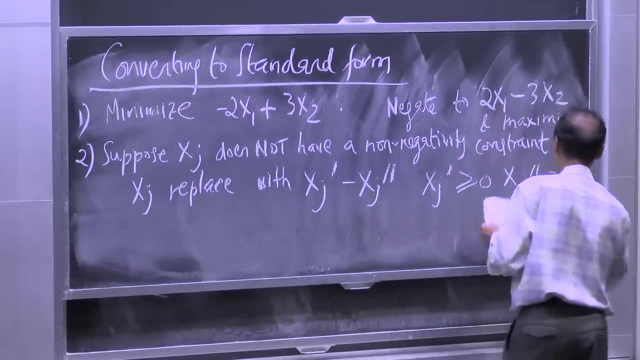 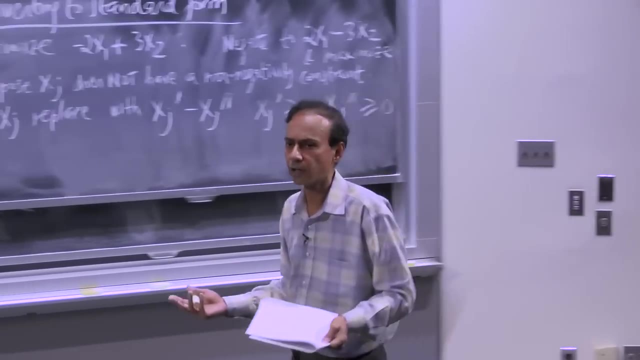 xj prime minus xj. So you have xj double prime And you have xj prime greater than or equal to 0, xj double prime greater than or equal to 0. But depending on the particular values in whatever solution you're exploring or the final solution, 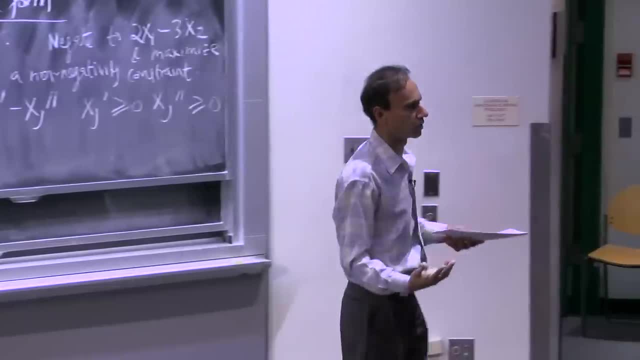 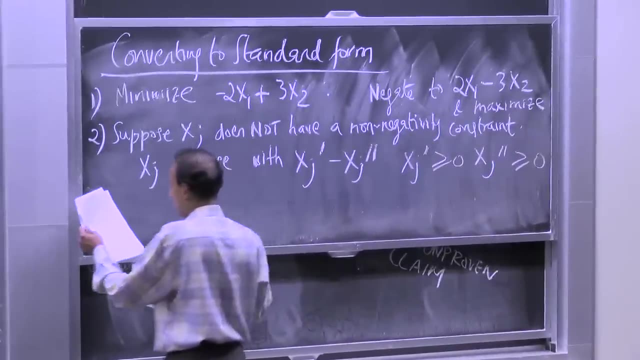 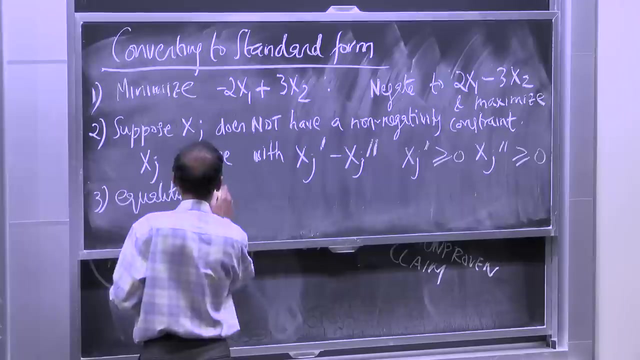 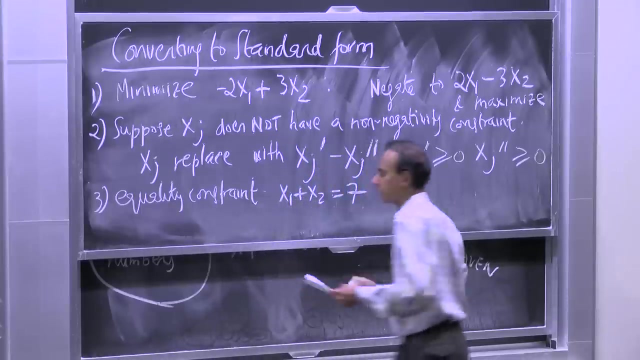 you may have an actual xj value that's negative or positive. So you added an extra variable here to your linear program And a couple more real quick. Real quick: Suppose I have an equality constraint corresponding to x1 plus x2 equals 7.. 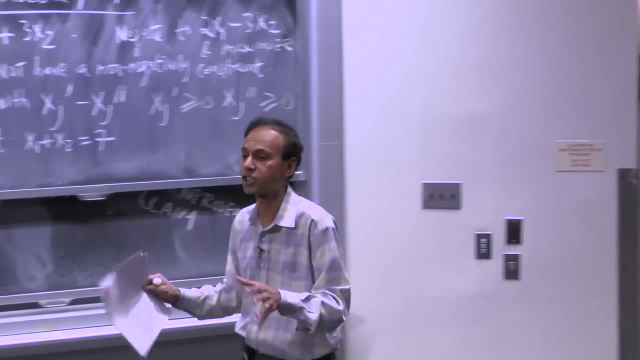 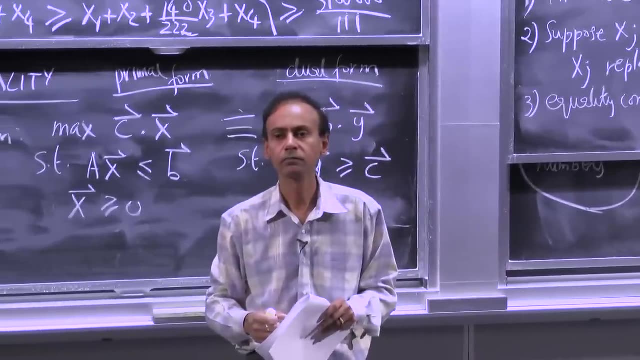 What do I do with an equality constraint where I have x1 plus x2 equals 7? Right, Yeah, go ahead. You could say: x1 plus x2 is greater than or equal to 7, and then plus 2.. No, you can't do less than or equal to. 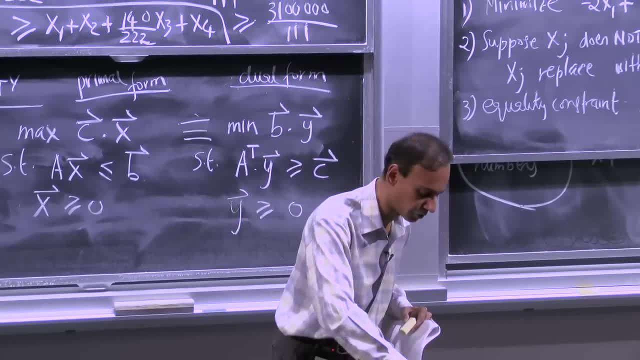 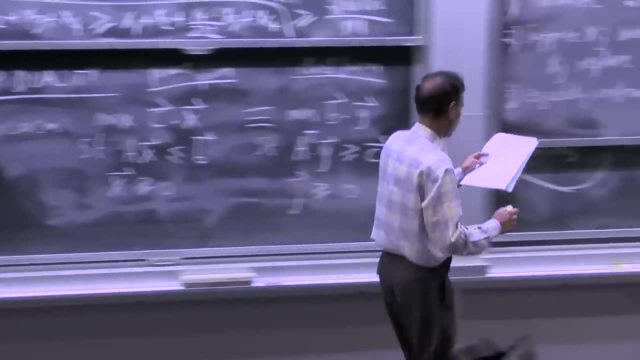 But then you could put it in: Ah, then you could flip the sign. So you have two steps there. Good, All right. So your less than or equal to needs another multiplier. So what you end up doing is something like x1 plus x2 greater than or equal to 7.. 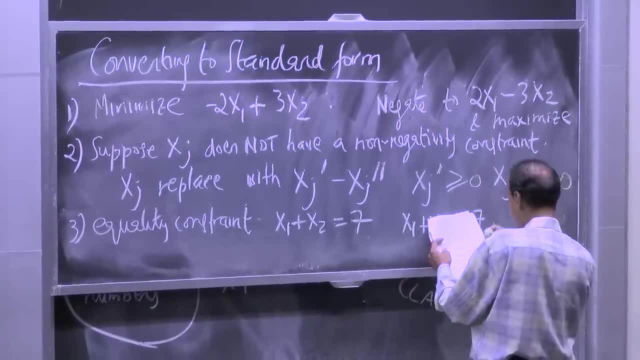 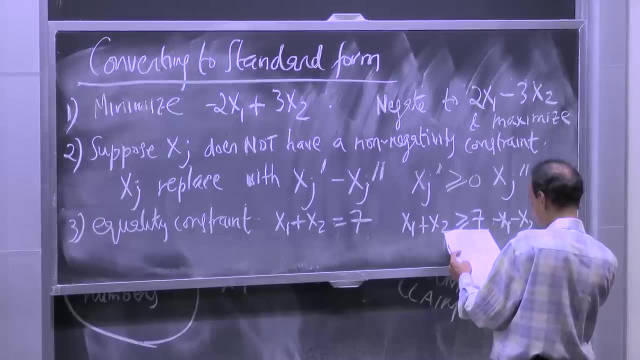 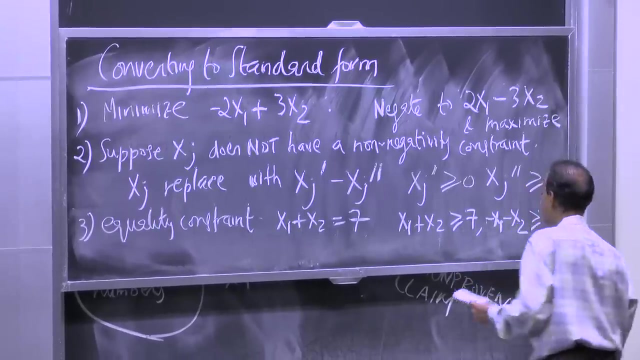 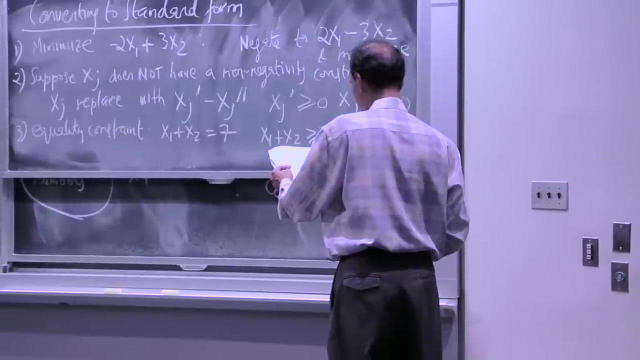 And then you need. if you do what the gentleman just said and flip the sign, you get minus x1, minus x2, greater than or equal to minus 7.. Right, Right, Is that right? No, I messed up. Oh, I want less than or equal to. 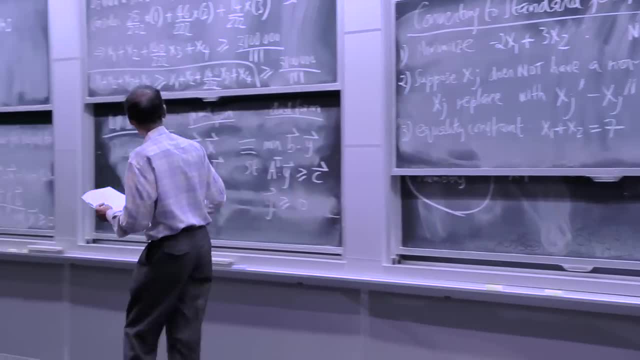 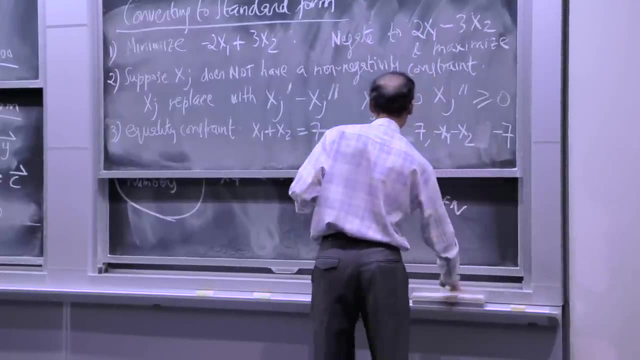 You're right. You're right, So I need less than or equal to. Oh, that's right, Of course. Thank you, Right, So I need less than or equal to in both places. All right, So that's the standard form. 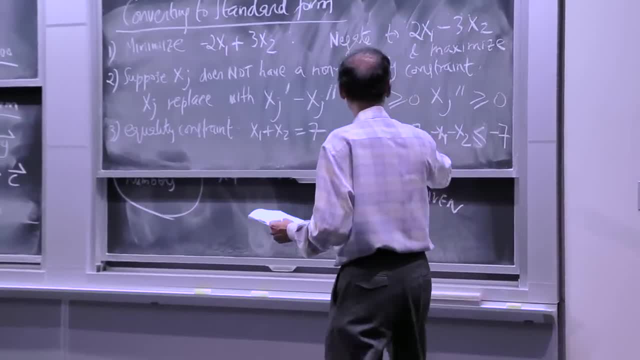 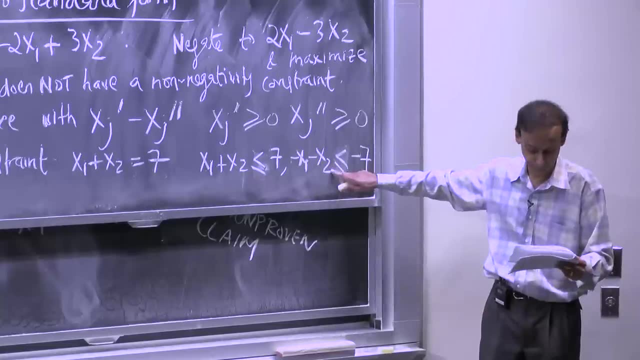 I needed less than or equal to Good Good. What you've done is increase the number of constraints by 1.. All right, Did I get this right Second time? All right, So that's pretty much it, The last thing which I won't really write out. 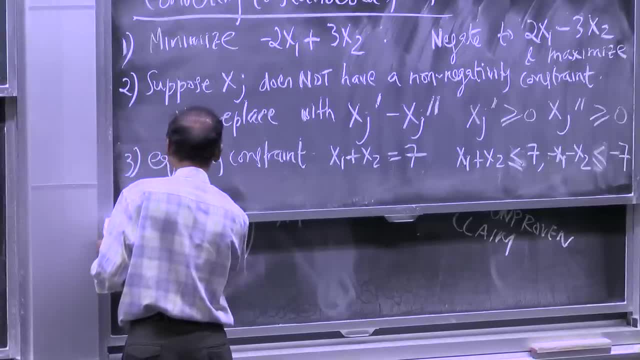 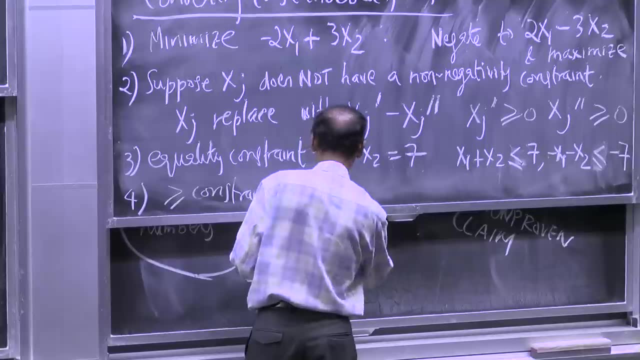 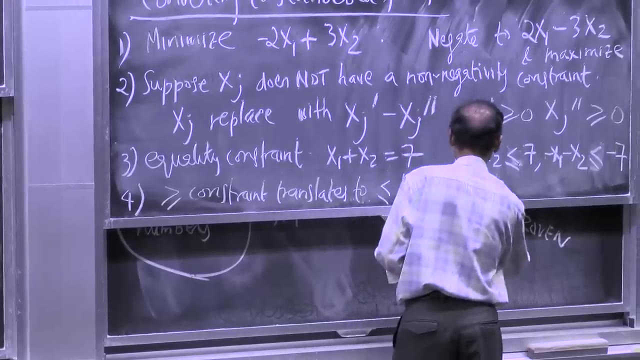 is- which we've done here already- greater than or equal to constraint translated. I want to give you an example of this. We have this already: Translates to less than or equal to by minus 1.. Plus 1 multiplied, So we had to invoke that in order to do the equality anyway. 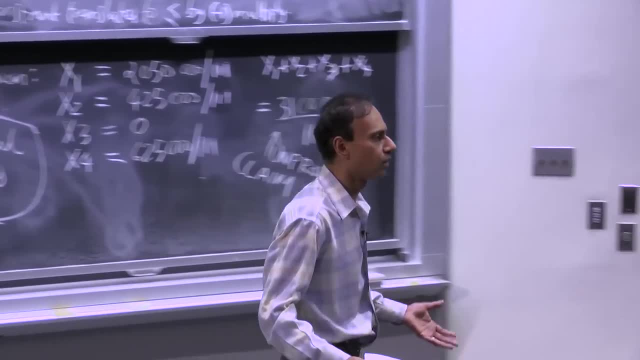 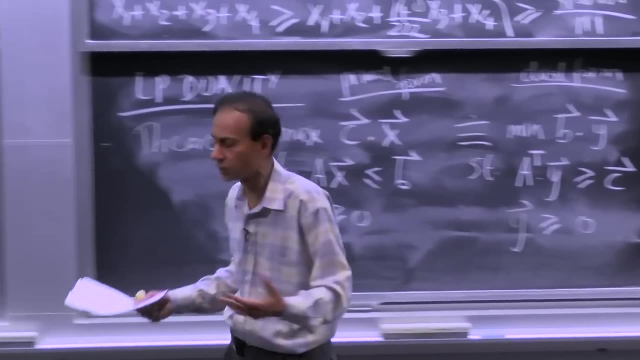 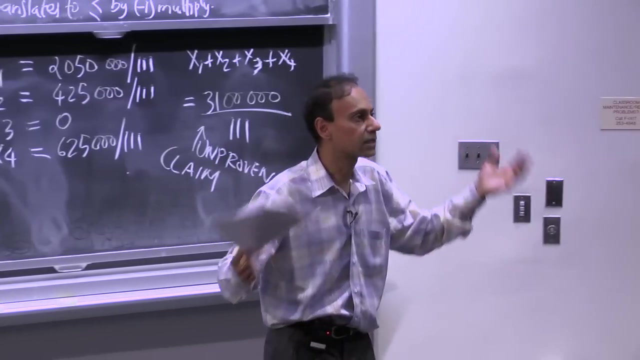 So you're in business. If you have a standard LP solver, you can take pretty much any optimization problem that is linear in terms of its objective function and has linear constraints, And you can transform it into LP. If you had nonlinear constraints, there's lots of work that goes on in linearizing. 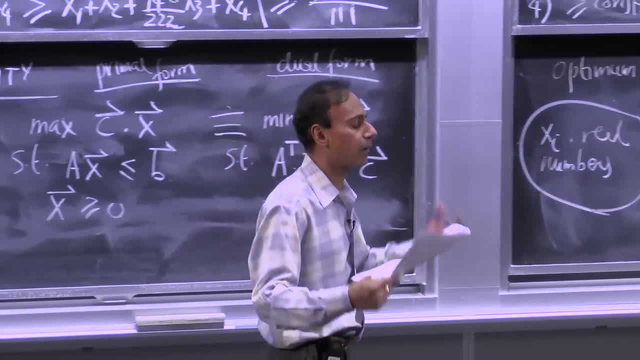 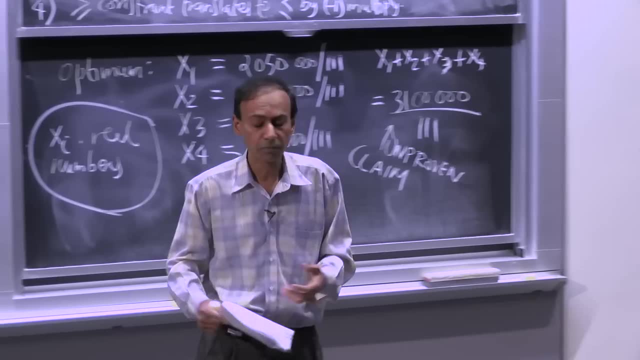 those constraints And, using LP solvers, it's a very practical thing to do. It may be something you'll end up doing invoking these powerful LP solvers- Typically they're commercially available. The best ones are commercial- And use it to solve your particular problem. 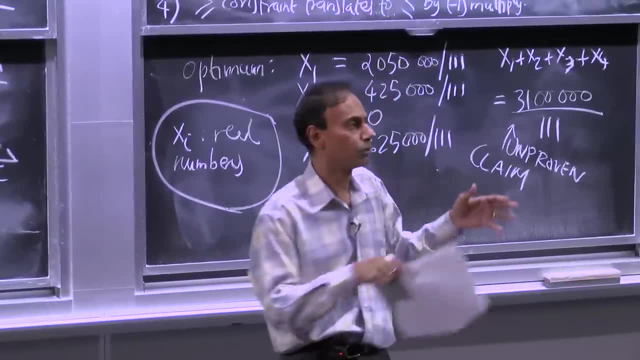 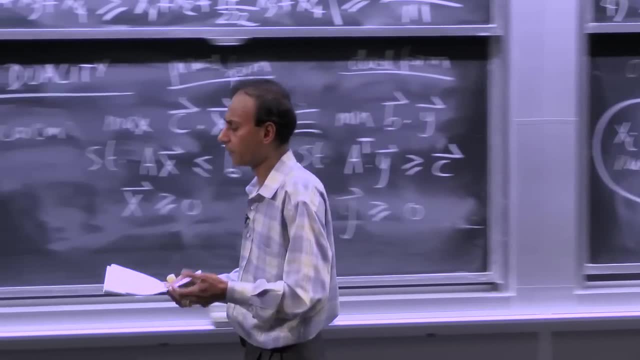 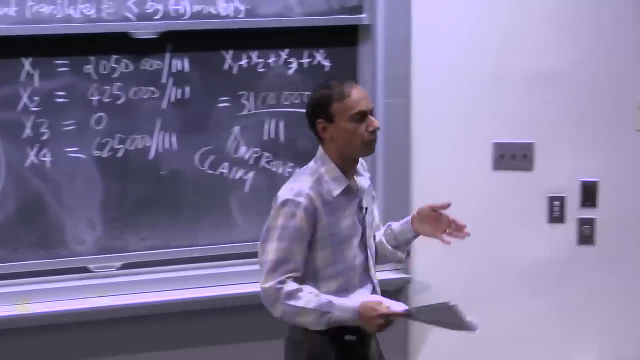 It turns your algorithm design problem into a reduction, And so you'll spend really the next couple of weeks thinking about reductions. We'll start that up right now, where we'll take existing combinatorial problems for which we already know algorithms for, and we're going to reduce them to LP. 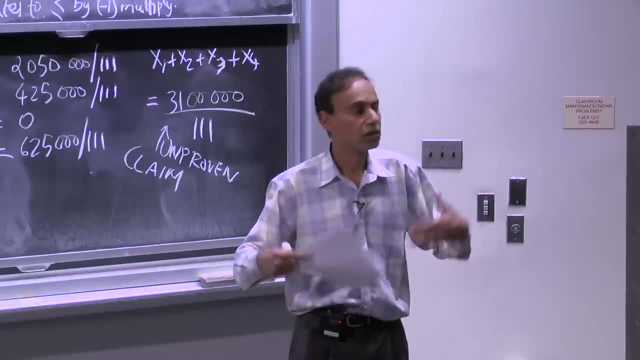 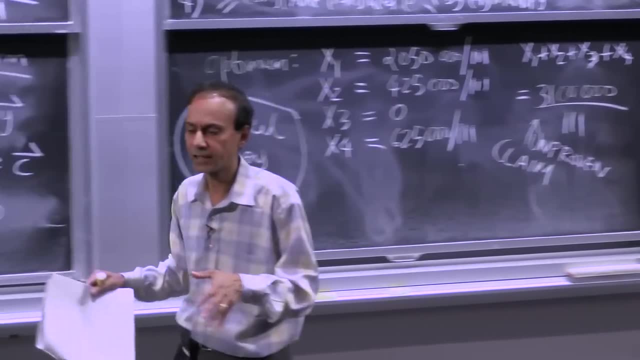 just to give you a sense of what the power of LP is. But this notion of reduction is very powerful. You can use it to do complexity proofs Here. we're just using it as a convenience in today's lecture to use our LP hammer. 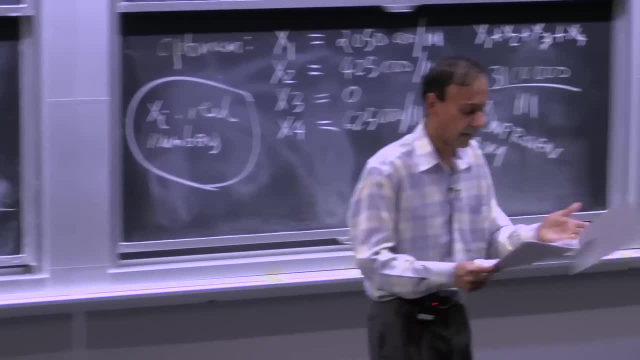 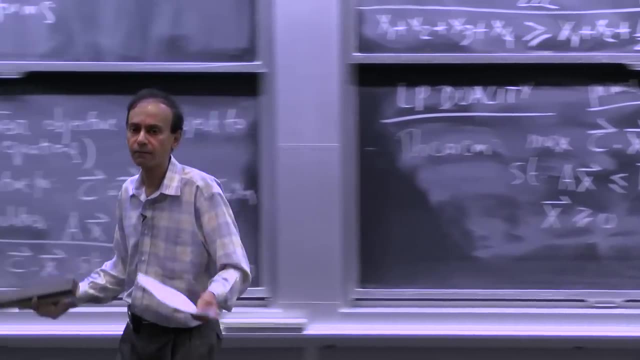 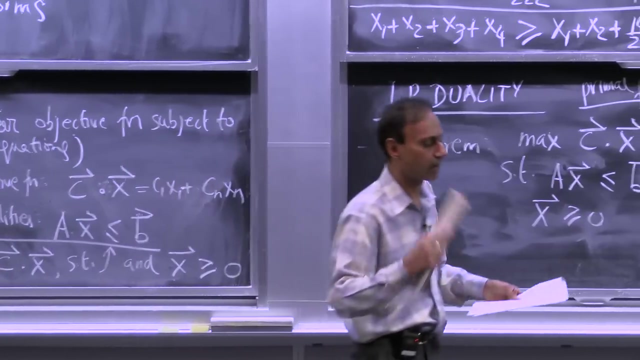 So let's say that I have our favorite problem of the week, namely max flow, And I want to convert that to LP. So I go back a week ago, and right about this time a week ago, and we'd set up the max flow problem. 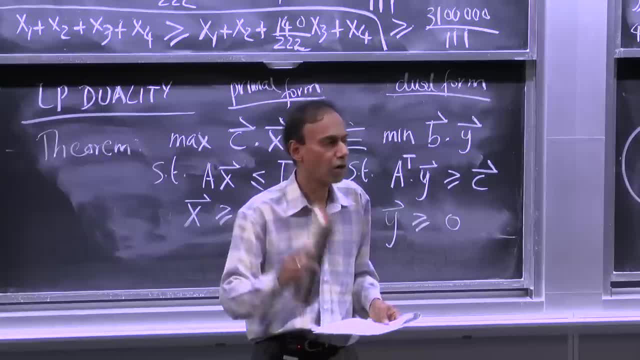 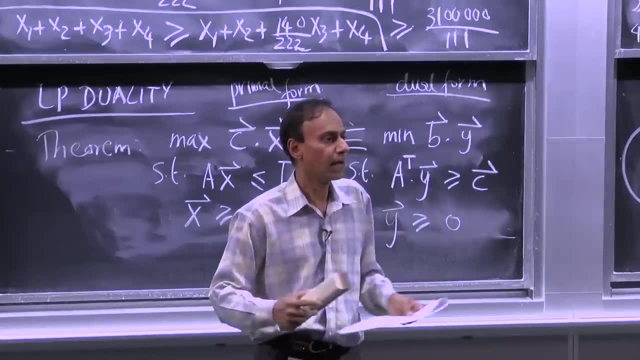 And let's assume that we went back there and we didn't talk about augmenting paths and we didn't talk about residual capacities or min cut or anything like that. But we knew LP already and we just want to solve max flow using LP. 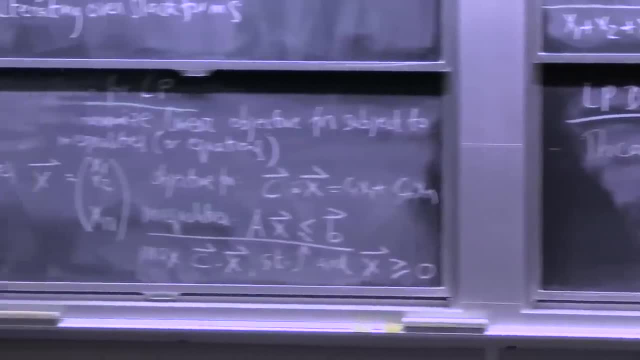 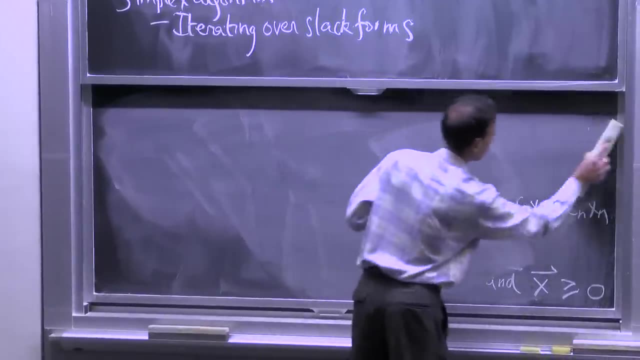 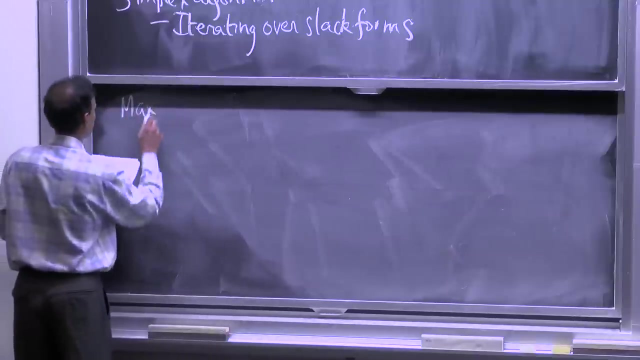 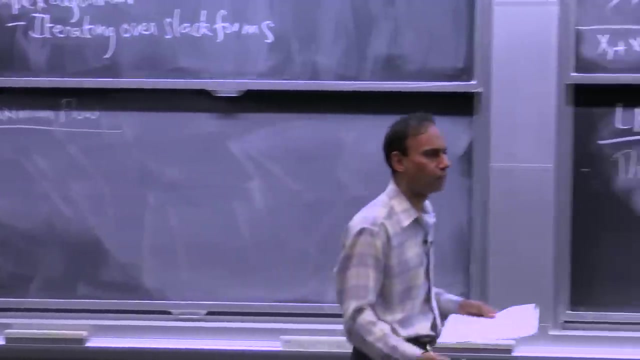 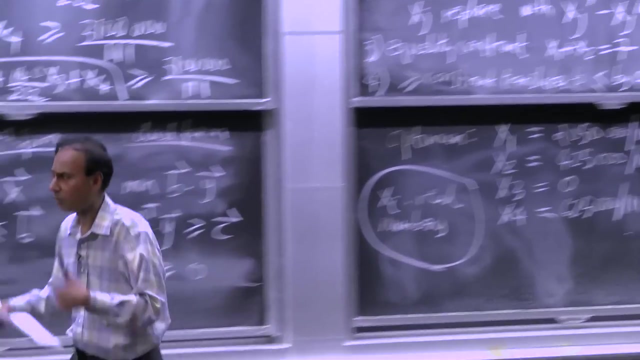 So let's do that. So this is maximum flow. I'm not going to bother with converting to standard form. We know how to do that, given what we just did here over there, So I'll just do whatever I want to keep things simple. 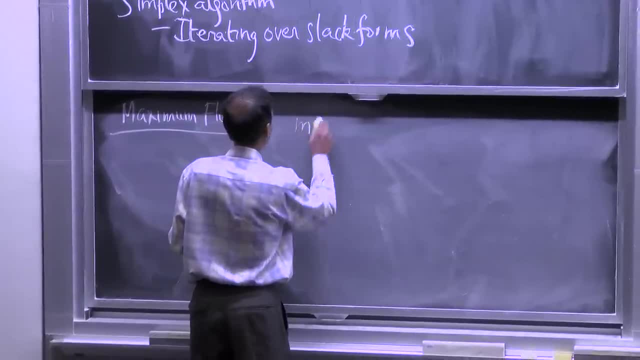 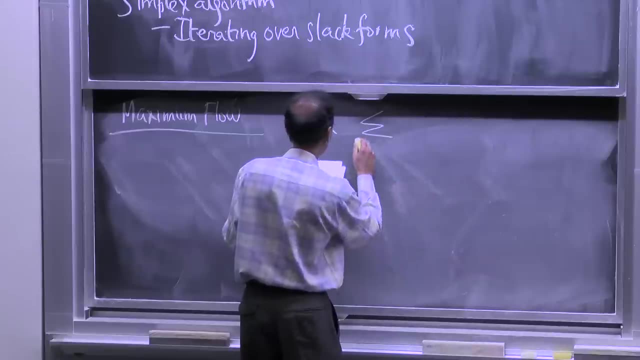 Max flow is obviously a maximization problem And, using the same notation we've used, it's not going to look like A, X and B, just because I want you to recall what max flow is And we're going to translate that. 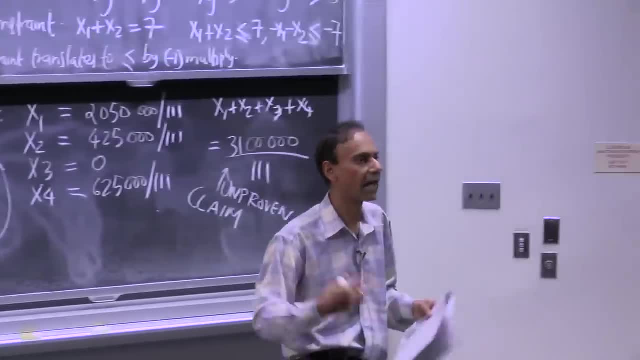 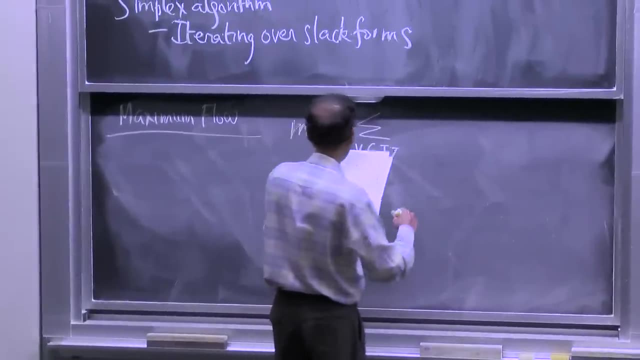 And the values of these variables or the names of these variables, whether they're X or F, it shouldn't really matter. We know how to do LP at this point, Or we know how to formulate LP, I should say, at this point. 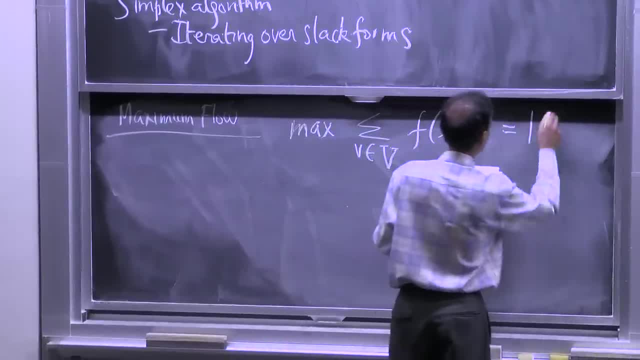 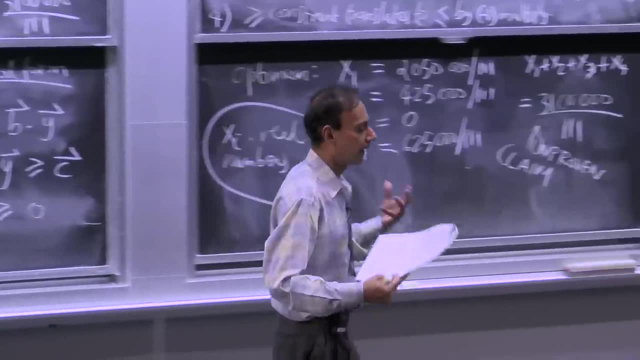 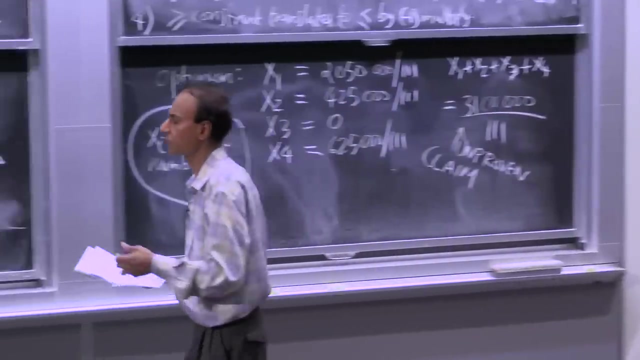 And we're assuming that we have an LP solver. So what I want to do here- the maximum flow problem is maximizing the flow value, And it's simply: you grab the source, you have a variable associated with the flow from the source to every other vertex of V and you have to maximize that. 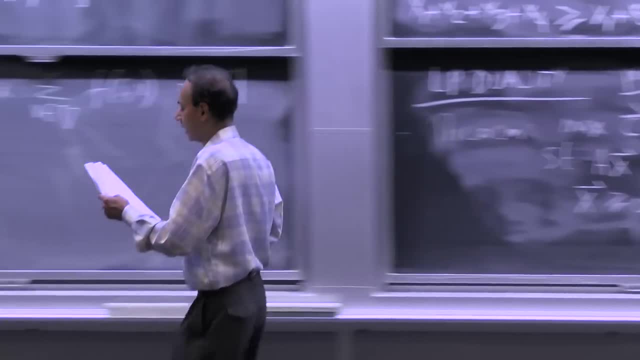 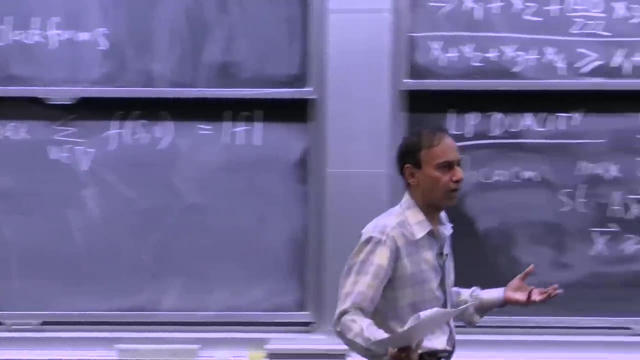 So that was the setup for max flow. I'm not changing that. What do you think the three constraints, or whatever set of constraints that we have here, are going to correspond to the LP? You spent a week on max flow. looked at the problem set. 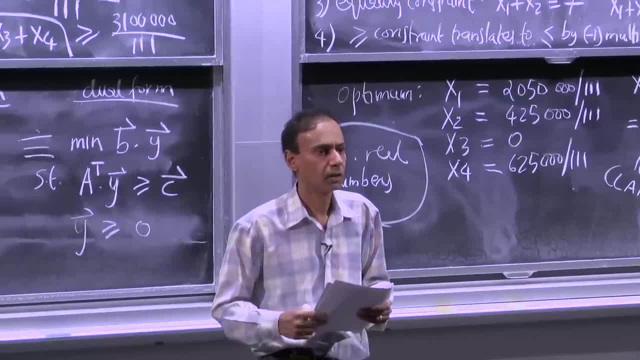 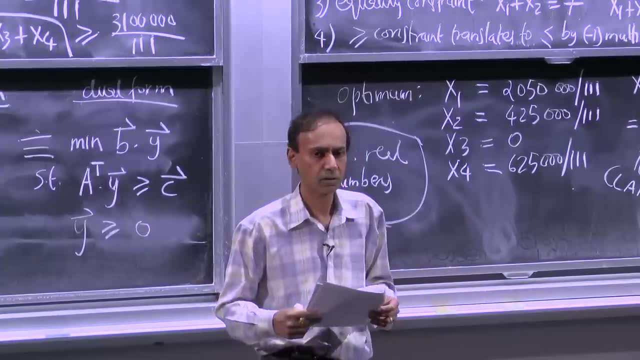 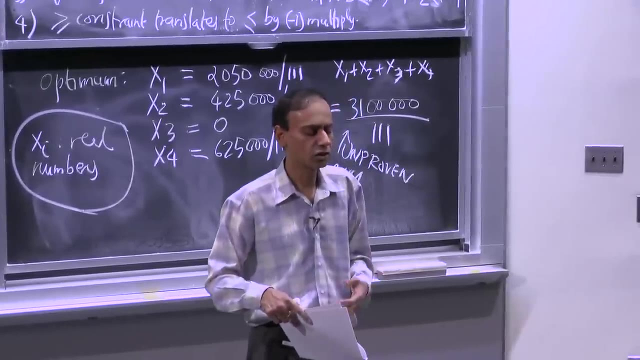 What constraints am I going to have to put up there? I'm going to have to put up capacity constraints. That's an obvious one. What is another one? Conservation constraints. Right, All flow. OK, Entering a node that is not the source or the sink. 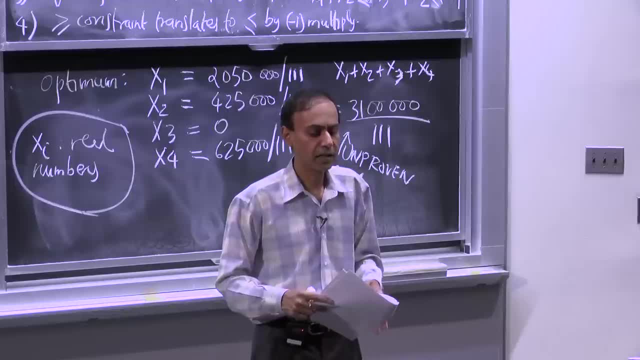 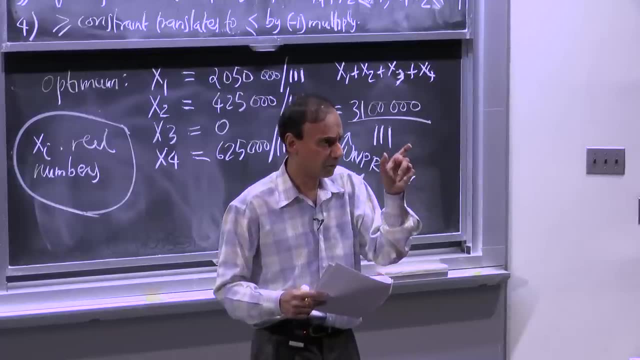 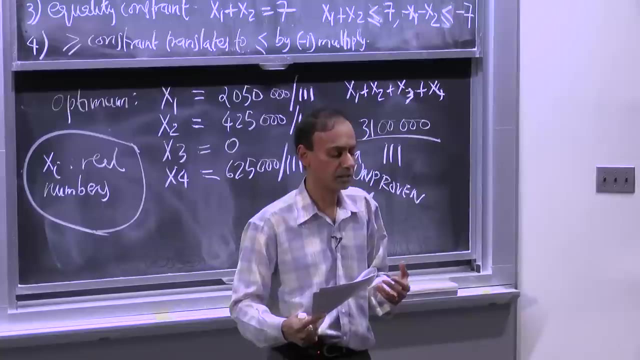 has to leave it right- Is in the original network. is there a concept of negative flow? No, you will define it, going in the other direction. So we did talk about negative numbers et cetera, But you're going to have positive quantities. 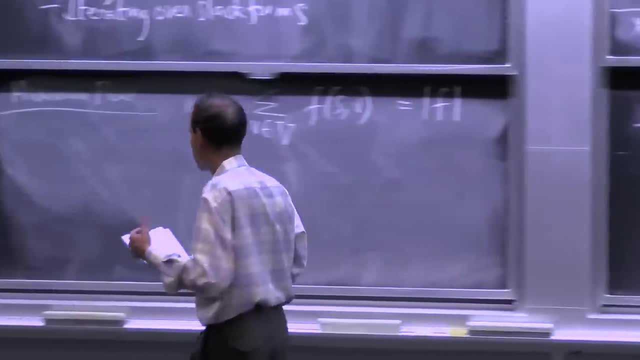 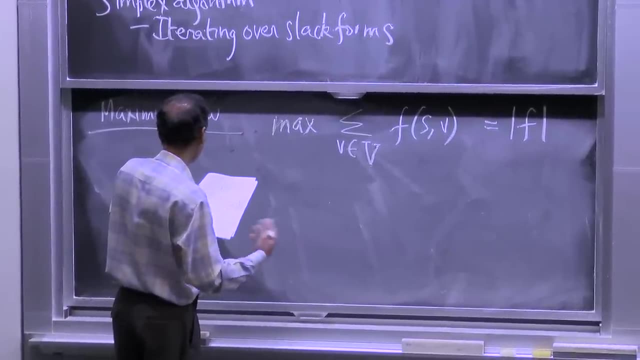 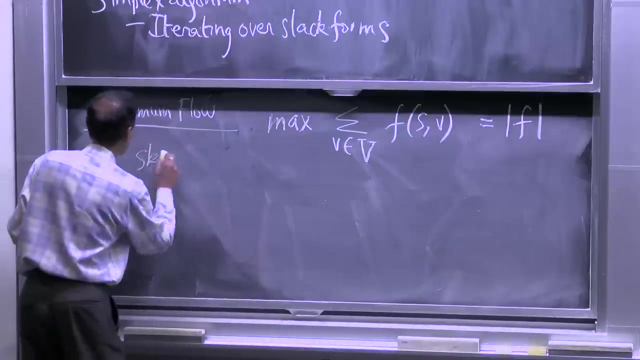 especially if you look at net flow, the version of the flow that we zoomed in on in the Tuesday lecture from last week And you also have in the general setting. you're going to have these skew symmetry constraints as well. So the three things that you need here: 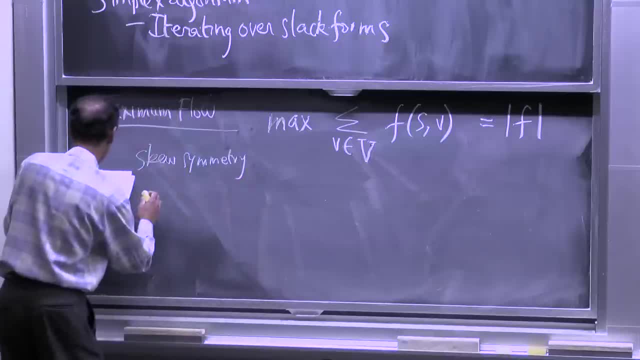 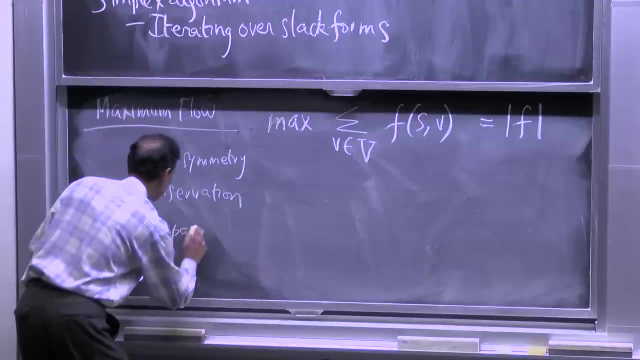 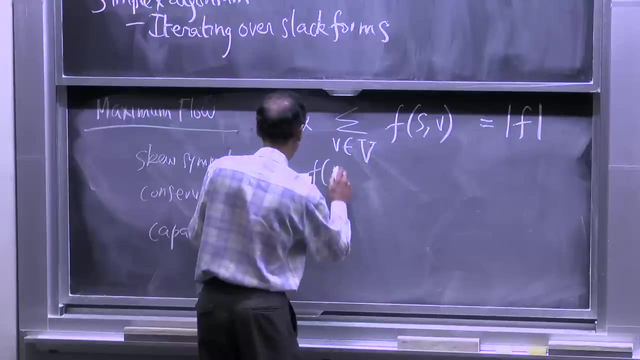 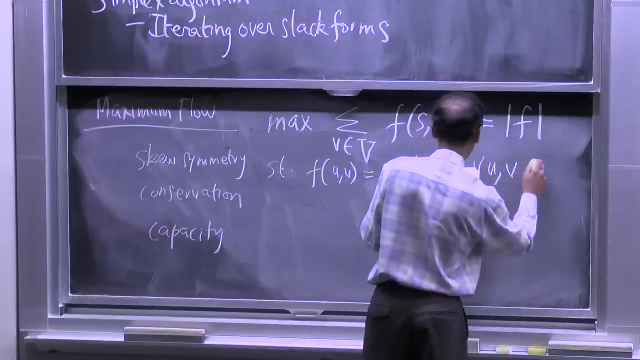 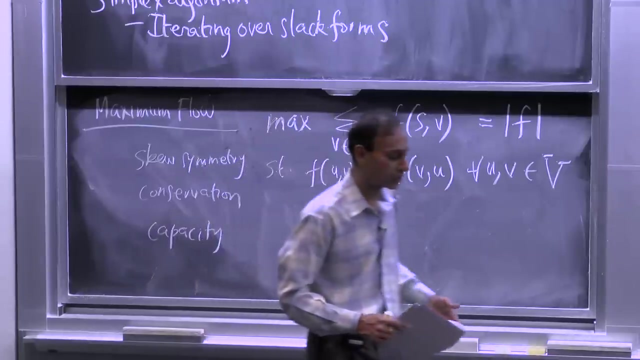 are skew, symmetry, conservation and capacity. All right, So you have, OK, So you have to have a network such that fuv equals minus fvu for all uv belonging to v And, depending on the kind of network that you have, if you constrain it to a certain type where you 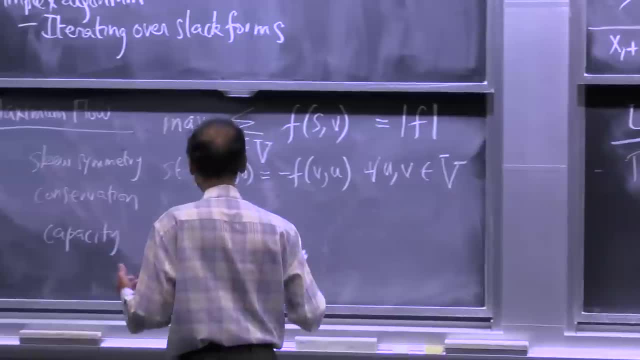 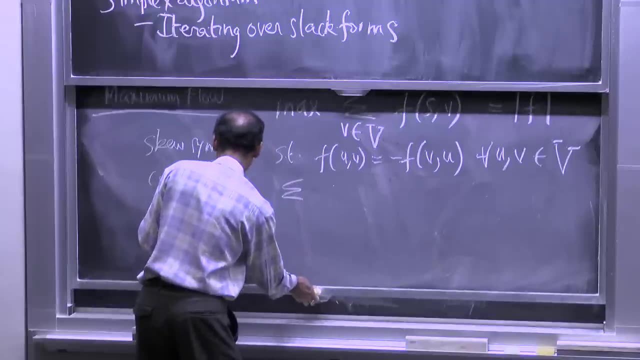 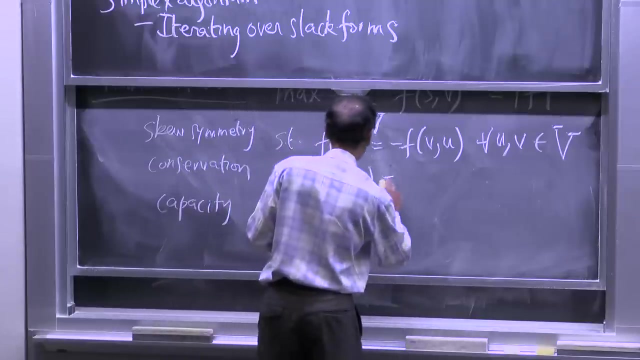 don't have these two-way edges. you could certainly remove some, if not all, of these skew symmetry constraints. The important ones are conservation and capacity, And this should seem pretty familiar to you. But the key, the reason I'm writing these all out, 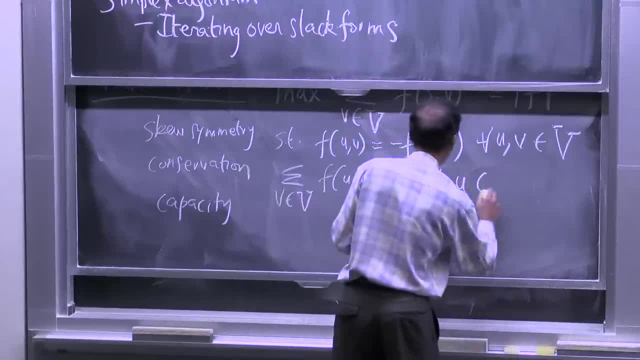 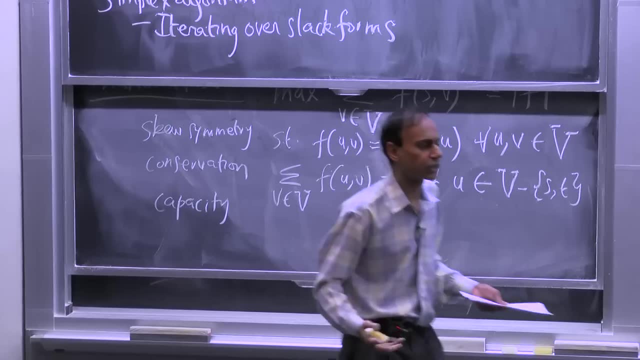 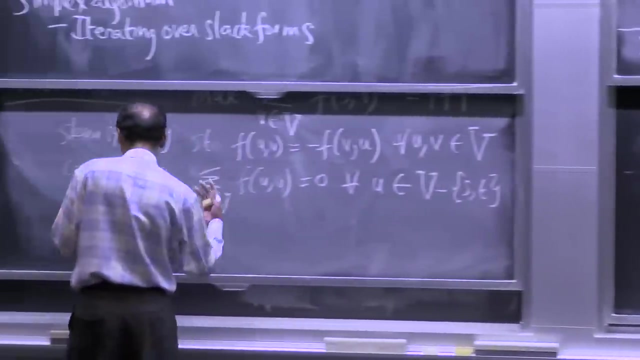 is primarily to ensure that you understand that these are all linear constraints. So that's pretty much the only thing that you need to observe here. Obviously, these constraints you've seen many a time from the two lectures last week, But notice that they're all linear. 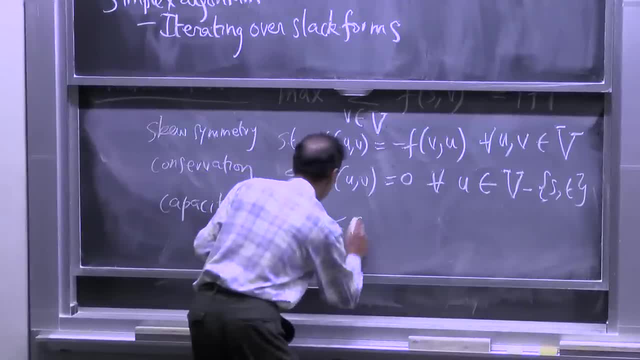 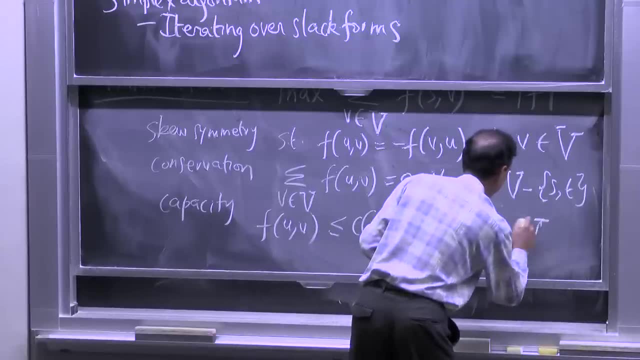 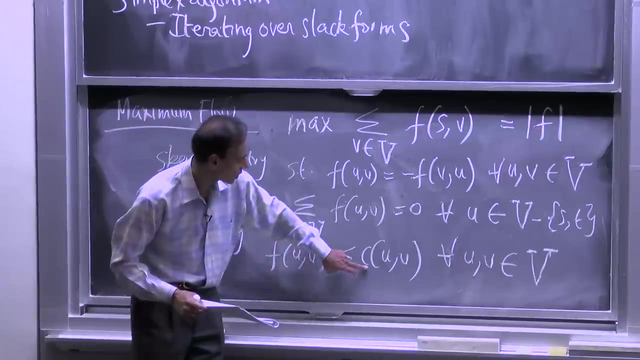 And finally, this one is fuv, less than or equal to v. It's equal to c of uv for all uv belonging to cap v. All right, So this is f, That's a variable that's less than another constant clearly linear. 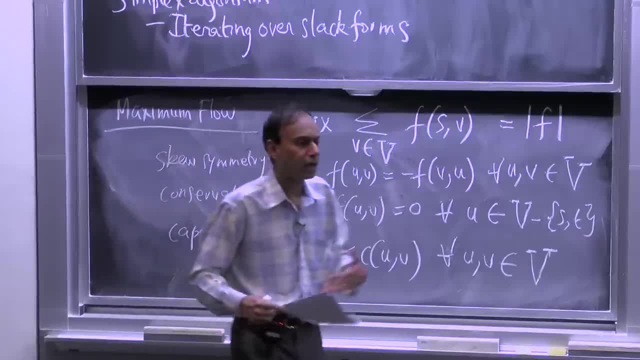 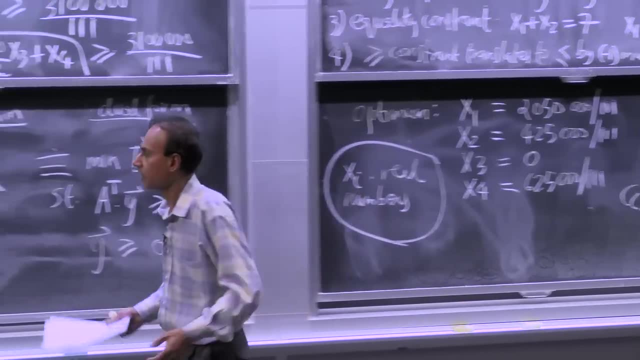 Doing a bunch of sums here, I could obviously have multipliers- scalar multipliers In this case, for conservation I don't have scalar multipliers, But it's clearly linear. Skew symmetry got two variables in here. One of them is the negation of the other- clearly linear. 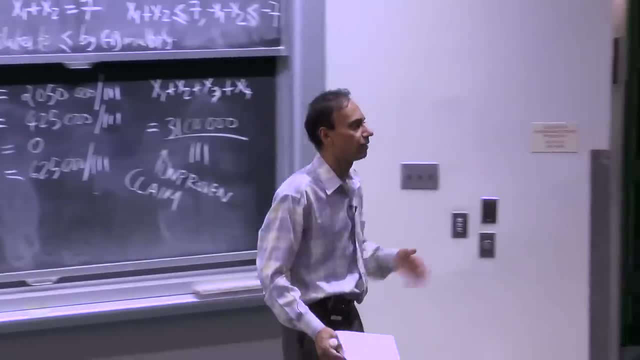 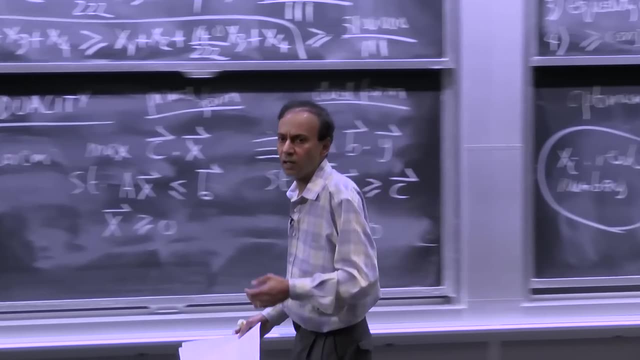 So that's why this is an LP, And so you might say: well, I know better. A max flow is much more efficient than any LP solver that's out there, And you would be right If you have a max flow problem of this variety. 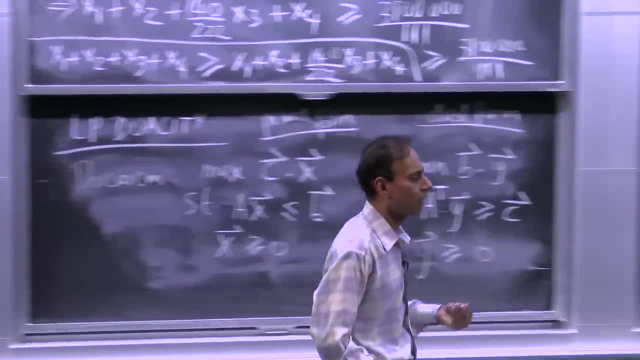 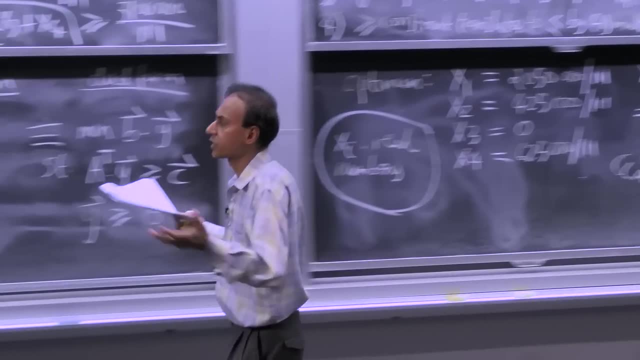 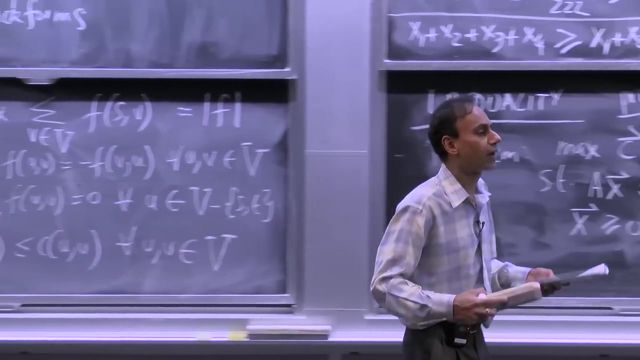 it's difficult to imagine that you would get empirical performance from running an LP solver, But there's a general problem. There's a general problem. There's a generalization of max flow, that's multi-commodity max flow where you just don't have. 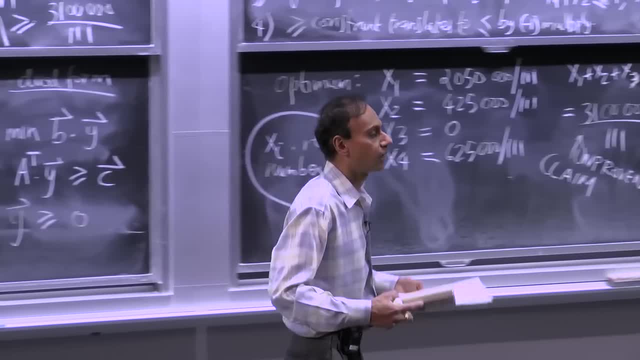 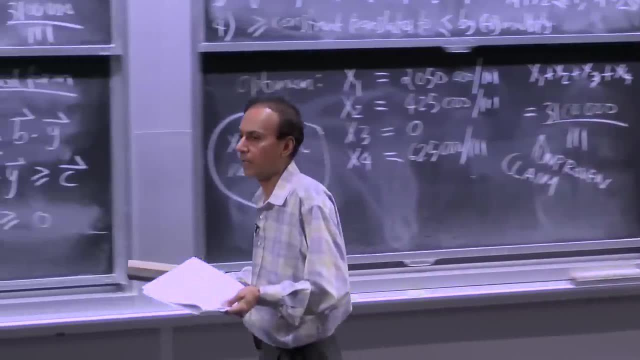 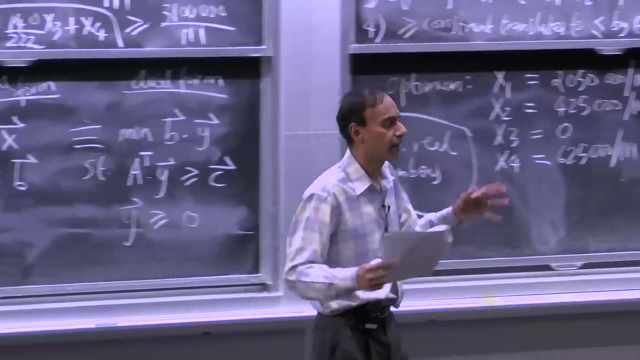 one commodity flowing through- You may be counting cars and trucks on a road- Or there's two different kinds of liquid flowing through the same pipe, whatever gas or liquid, And so when you have multiple commodities, you may have a linear but more complicated cost function. that's. 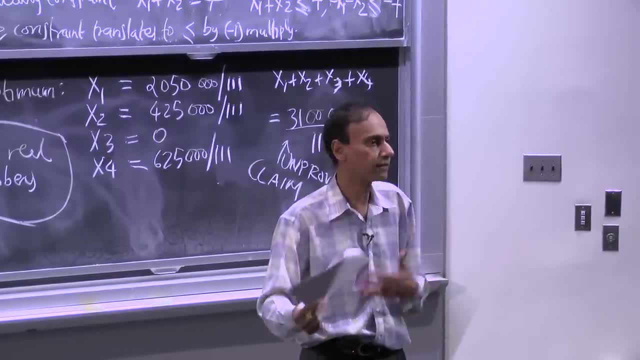 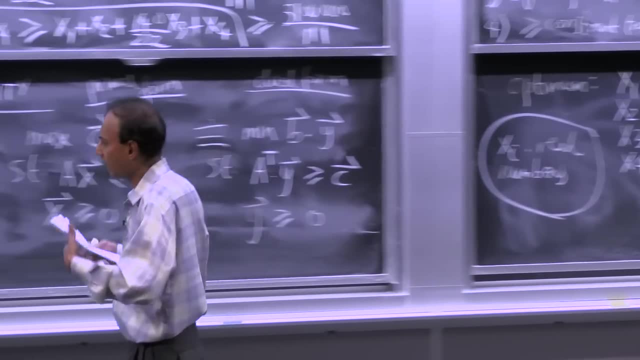 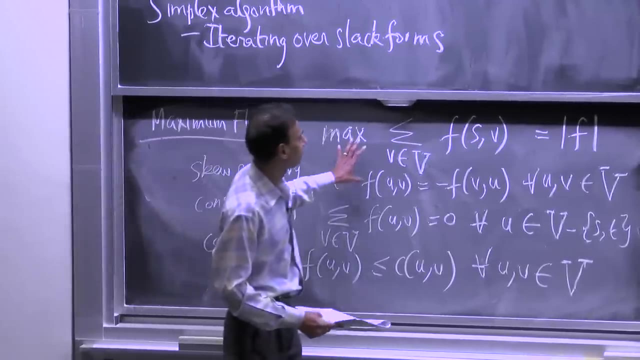 a function of the flow of each of the commodities And they may have a certain weight associated with them. So there's a lot of things that could be a more general, There could be more general settings corresponding to max flow, And I'll just leave you with the thought. 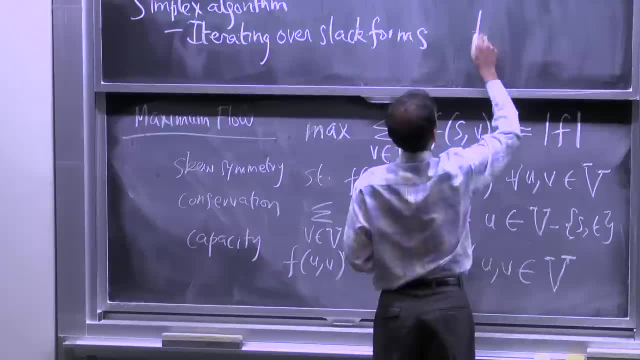 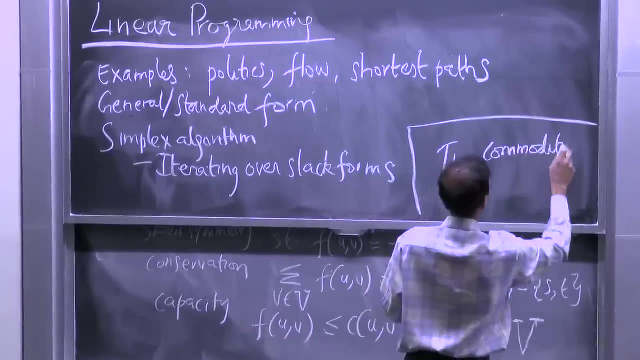 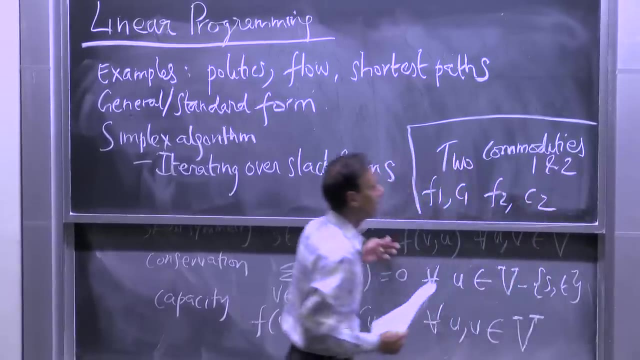 that you could simply have two commodities, and we'll just call them 1 and 2.. And so now you have the F1s and the C1s and the F2s and the C2s. Each commodity has to be conserved. 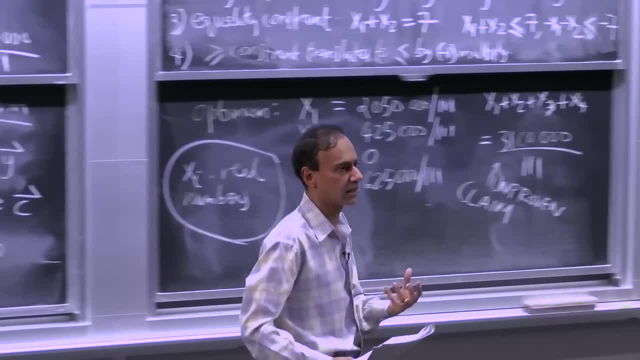 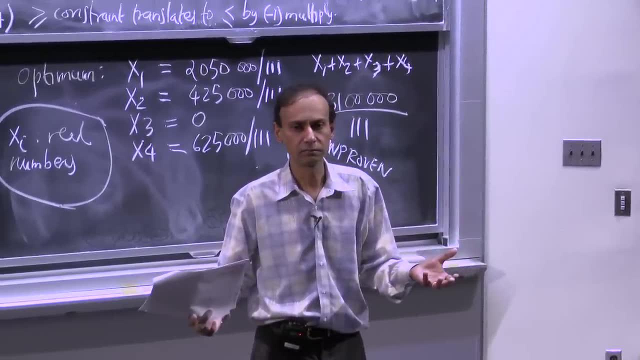 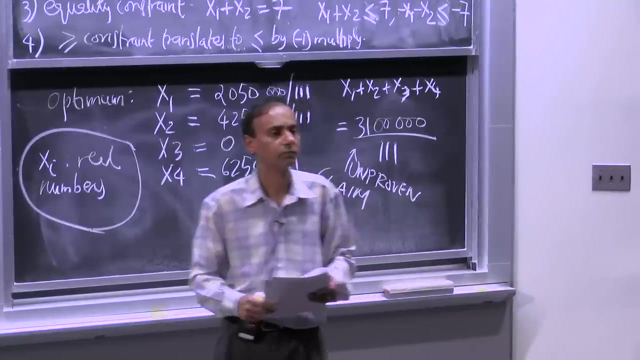 But what about the capacity? What do you think happens with the capacity? Let's just assume these are two different kinds of cars. So what would the capacity constraint look like? Yeah, You can say either C1 or C2.. That one would have to be like the three heads. 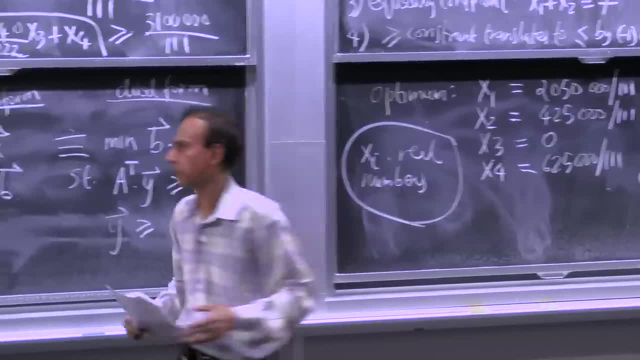 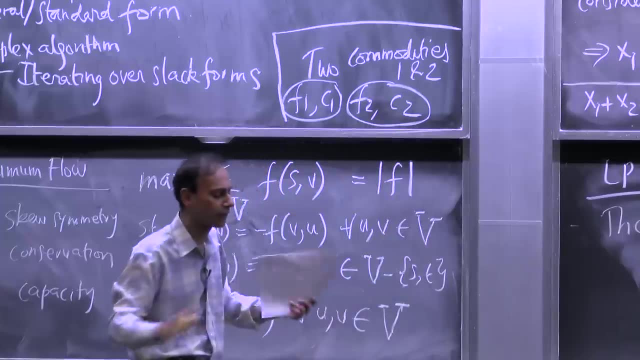 You can add them together or you might Exactly. That's right, So good point. It may be the case that I have distinct capacities And, in fact, if you have completely disjoint problems, you're right in that you can solve them separately. 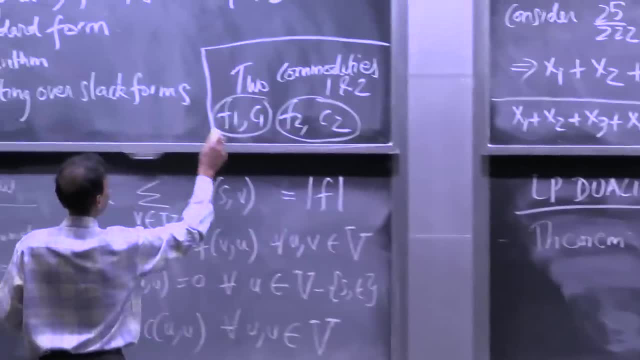 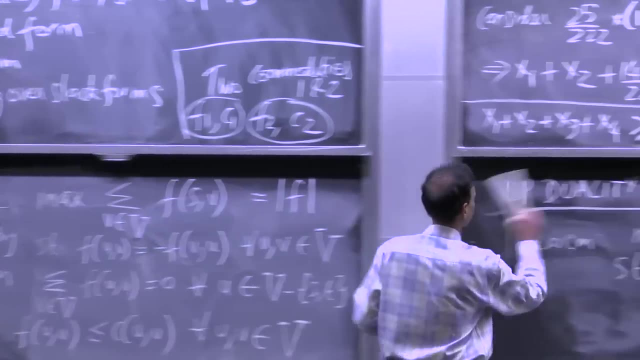 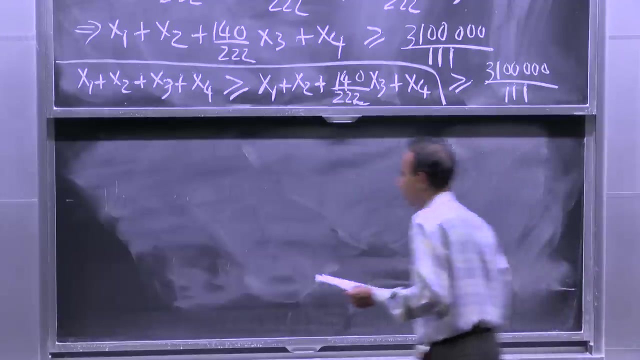 But actually the more interesting case would be that you have a single capacity C. So you'd have- let me just write this out here- if in fact you had two distinct things, So if you had F1, C1,, F2, C2, the question: 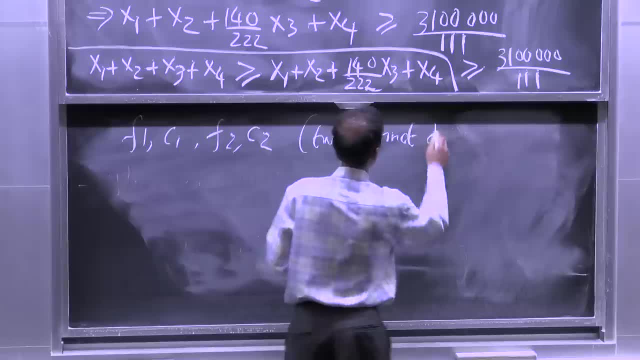 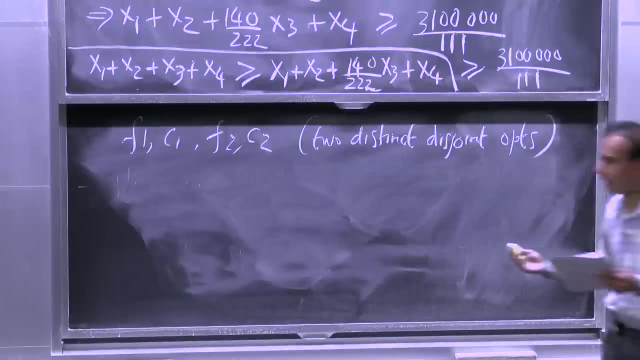 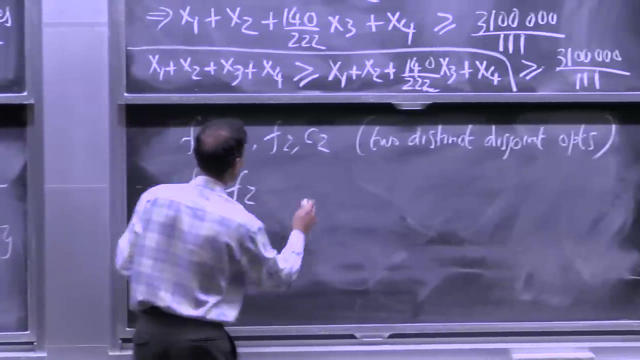 is: do you have two distinct disjoint optimizations, In which case you could just use max flow twice? On the other hand, what's more interesting really- and I should have used this example for starters, but here's a better one- You have two commodities and a single capacity. 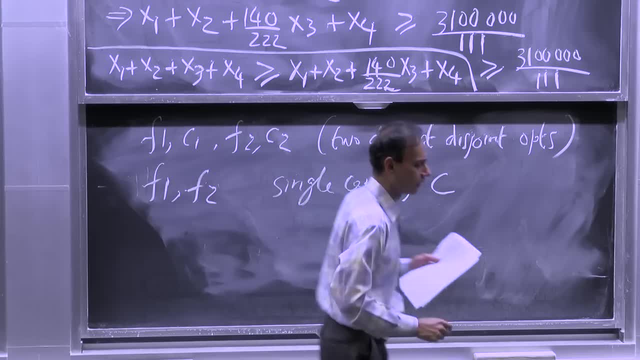 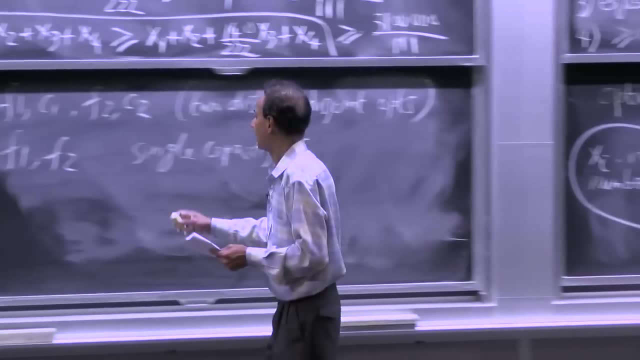 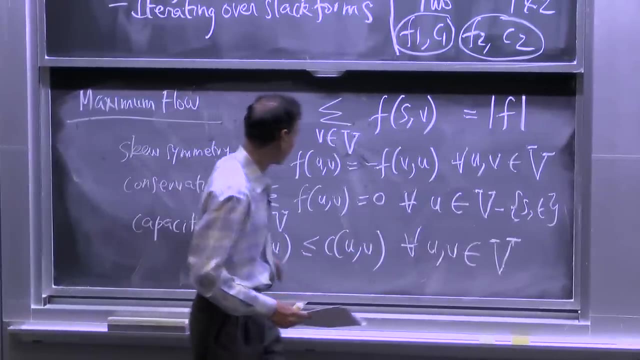 So the road is a good example. Both the cars and the trucks share the same road. It has a certain capacity, And now your capacity constraint is looking like F1 plus F2 over here, And that's the flow through the particular edge UV. 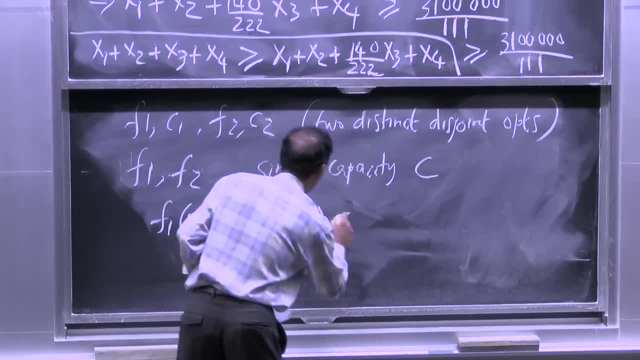 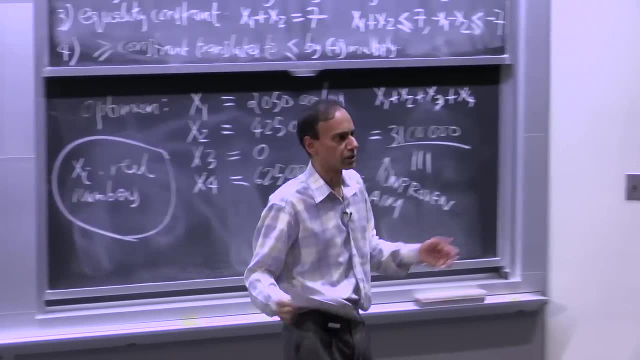 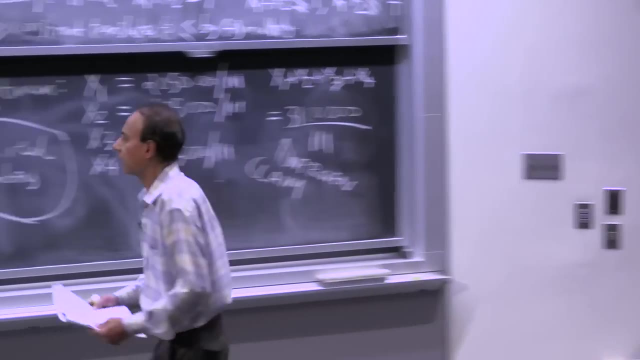 So you have something like F1 UV Plus. F2 UV is less than or equal to C UV for this total capacity And that's pretty much it. So that is linear. The nice thing is it's linear. You could put weights on it. 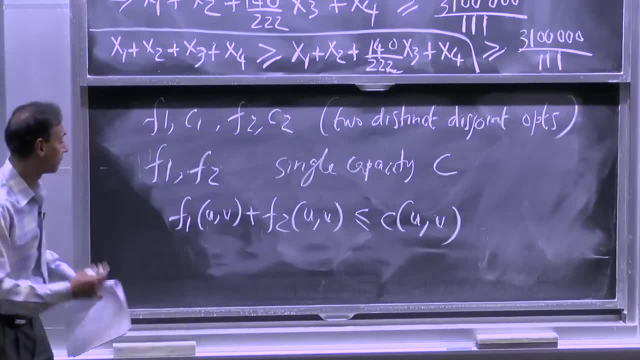 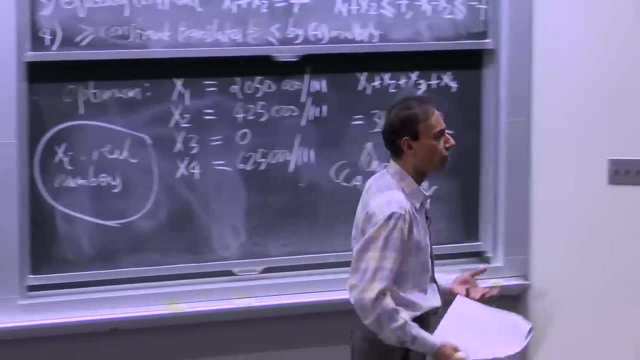 If you wanted to claim that a particular commodity one uses up because it's a truck, it uses up more space on the road and you can accommodate fewer of them, you could put a multiplier. Put a multiplier in there Still stays linear. 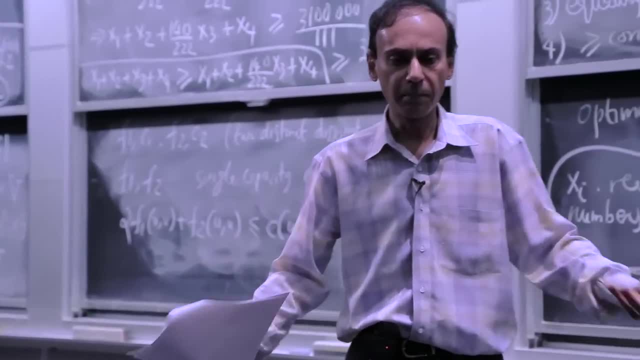 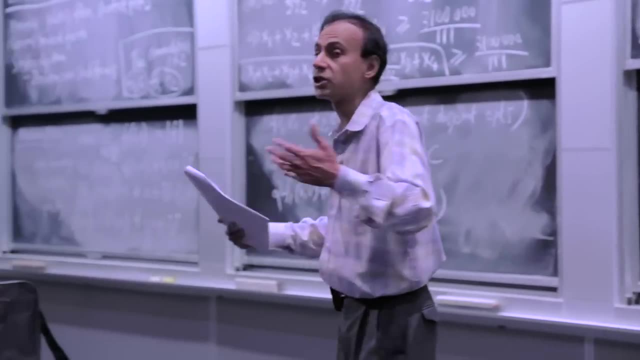 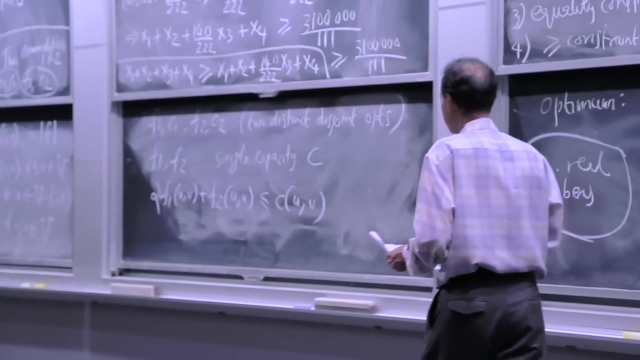 So that's the power of having an LP engine. You could translate problems that are not exactly max flow. They're multi-commodity flow. You may have additional linear constraints that you could add And you could still use your LP package. So that's the reason why this is interesting and powerful. 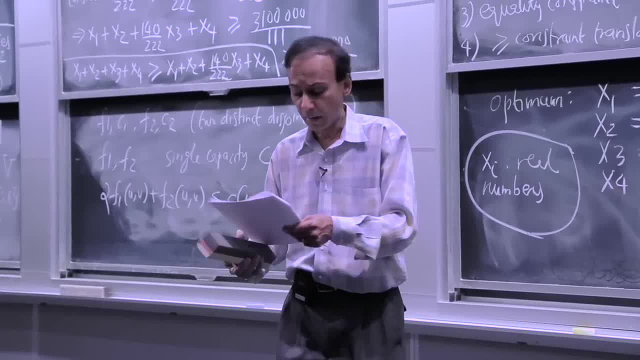 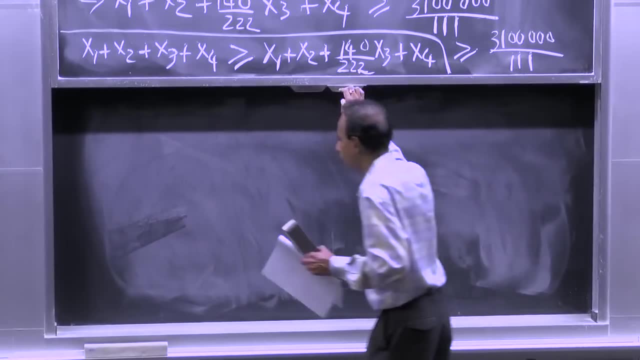 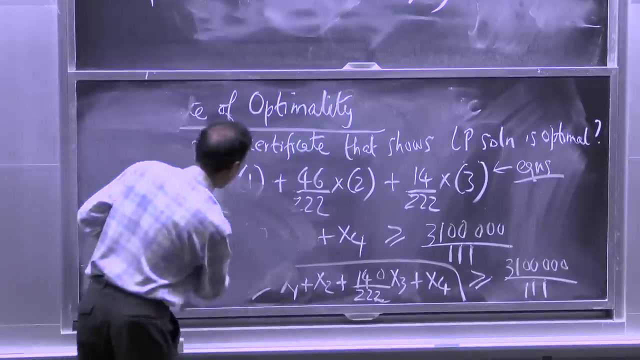 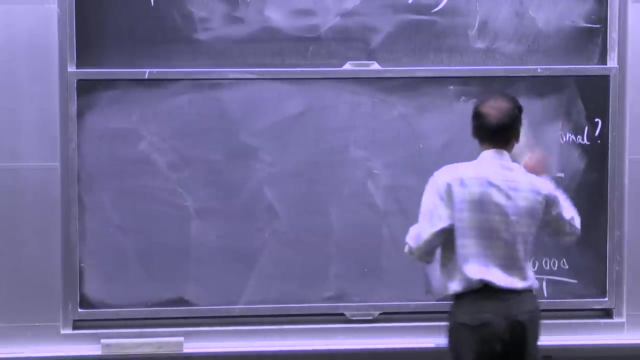 So that was kind of an obvious one corresponding to max flow. Let's look at something that's a little less obvious And it's going to be a little tricky to convert the shortest path problem to LP. Not a lot of work, but one little observation. 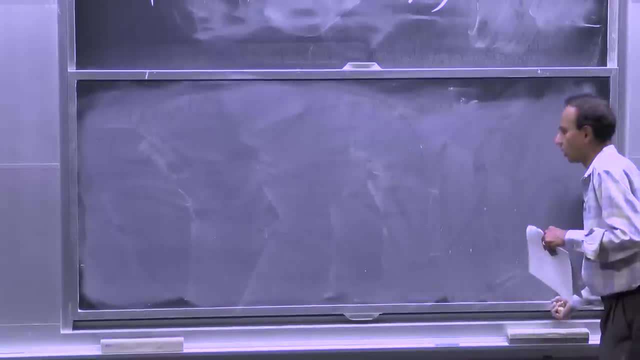 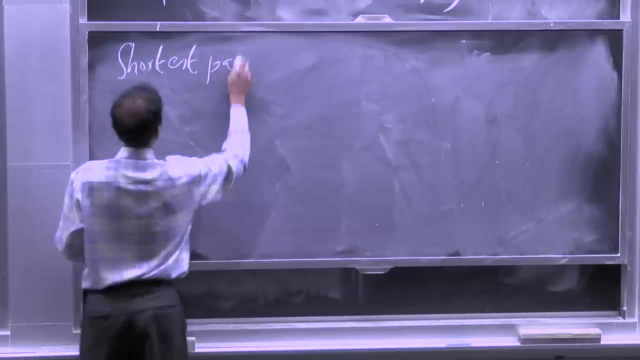 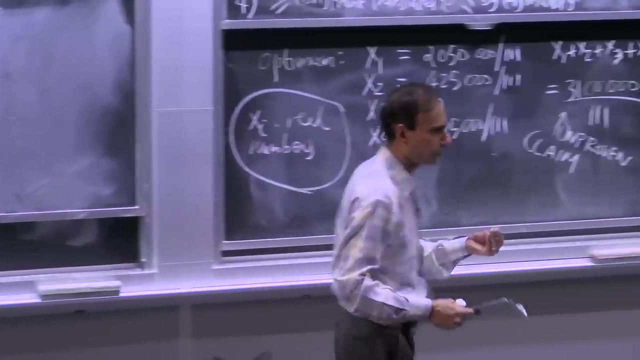 that's going to be important to make in order for the whole thing to flow through or actually work out. So we all know the shortest path problem We want to find- let's just call it the single source shortest path problem. You have a specific source, that's. 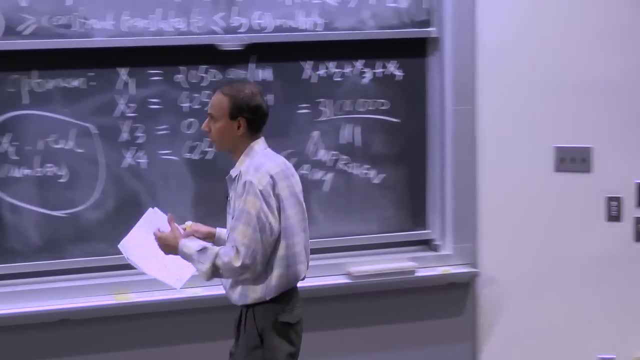 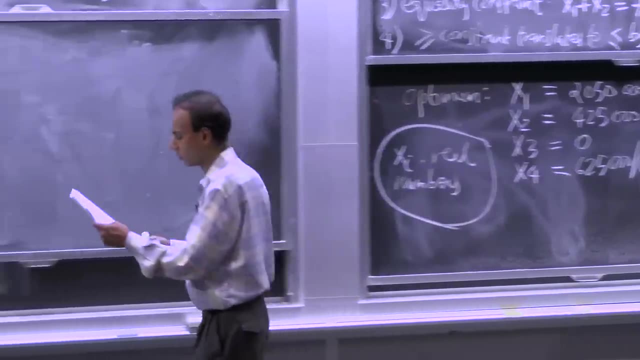 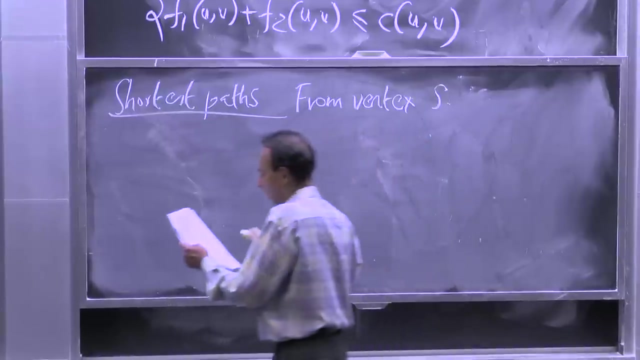 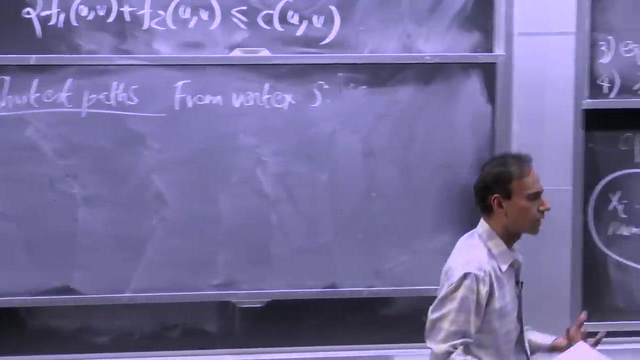 going to turn into the point from which you're going to start computing the distance. That's what Dijkstra does, and that's what Bellman-Ford does, And so this is from vertex S, And what I want to do here is obviously set it up as a set of linear constraints. 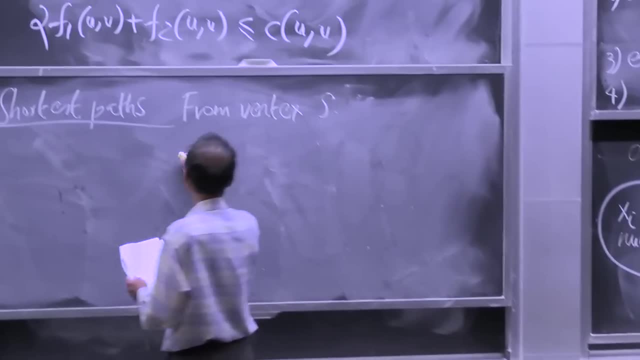 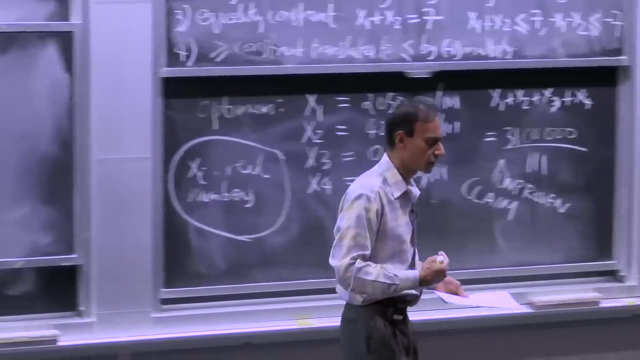 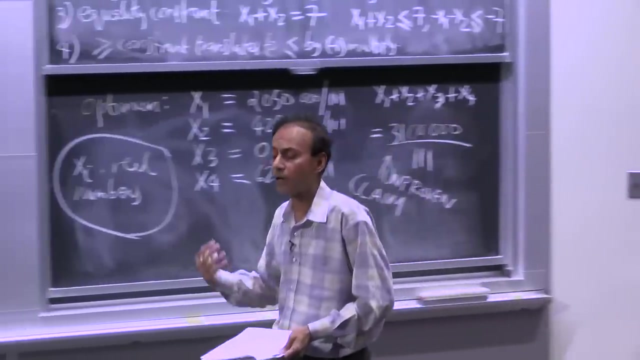 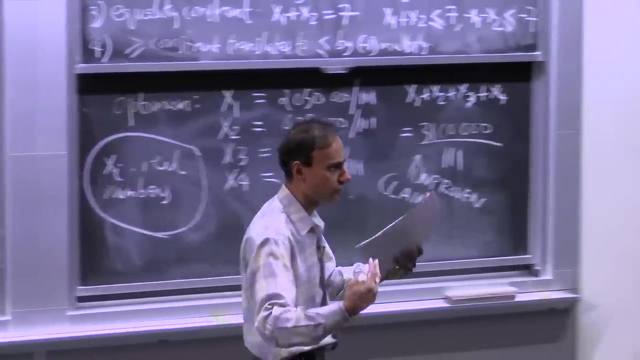 If I have dv corresponding to the distance from the source, so dv represents the distance from the source And eventually I want dv to be the shortest distance from the source. That's our notation for shortest, Shortest paths. dv represents an existing path. 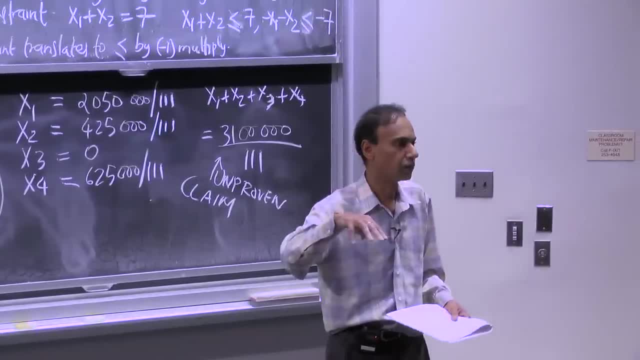 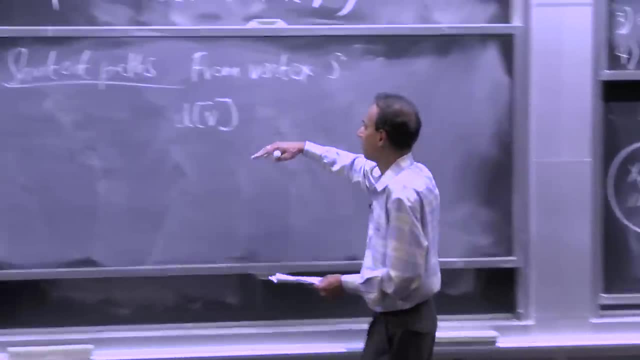 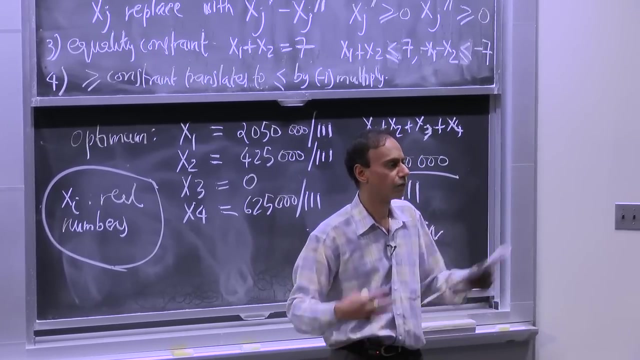 It may not be the shortest path from s to v, the value of that But dv monotonically decreases as you run through. It's initially infinity in Dijkstra, going back to Dijkstra, And then we shrink it through a process of relaxation. 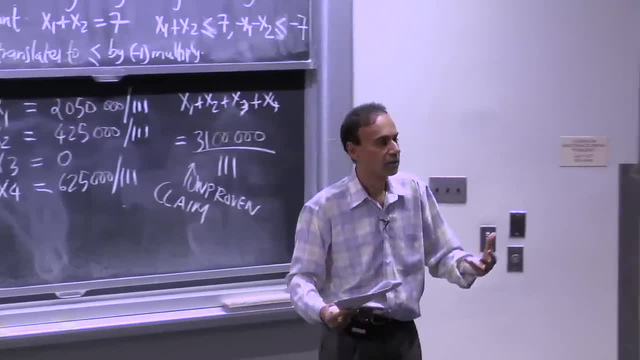 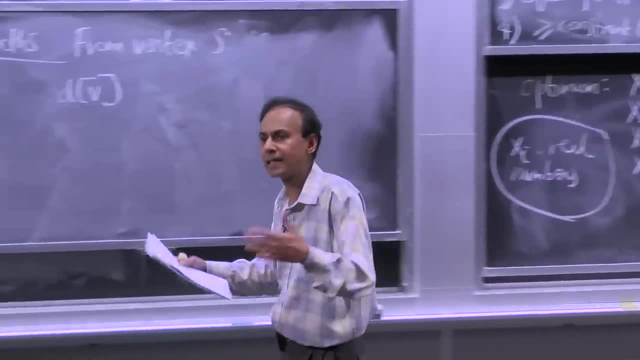 Now I want to try and model that. I want to try and model all of this as an LP. So it's not me And what I think where that's happening is very, very obviously the thing that the flow networks had where we had these constraints. 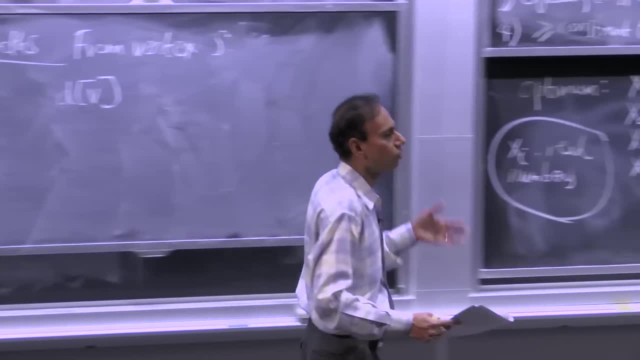 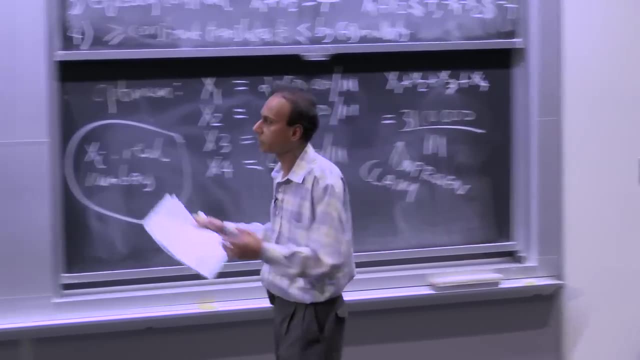 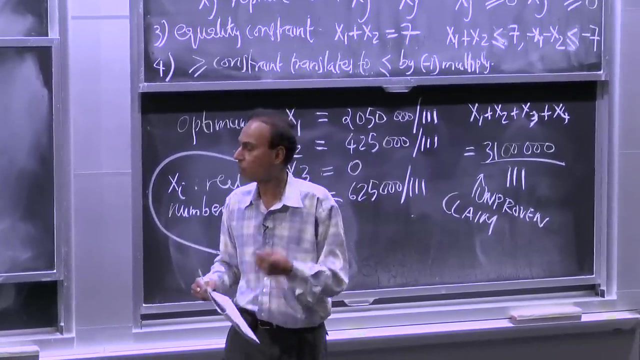 We had capacity constraints and conservation constraints And we could turn that constraint into an inequality And it was pretty smooth, just pretty easy. So what I need to do here with shortest paths is something that's a little more subtle. So what basic constraint do I have? 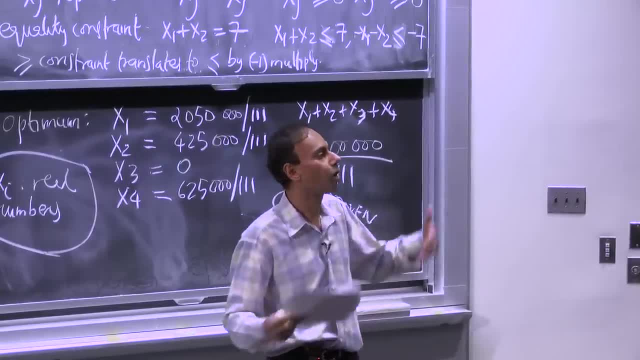 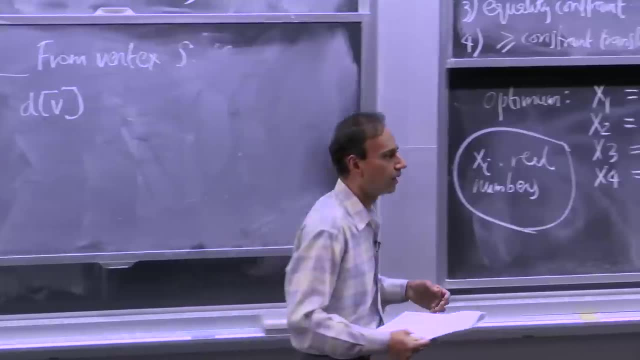 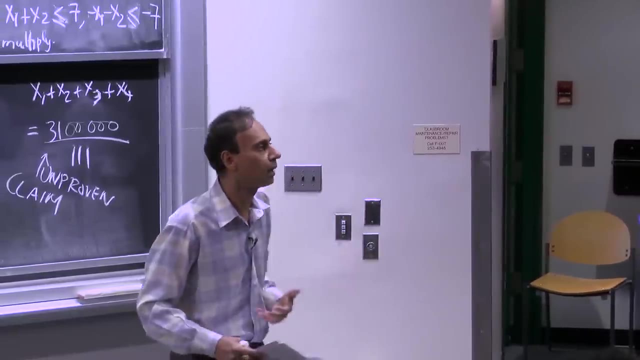 algorithm. What's an inequality? Do you remember an inequality from shortest paths that we kept talking about The triangle inequality? So we're going to have to go over the triangle inequality and take the triangle inequality and use that to create an LP formulation of shortest paths. 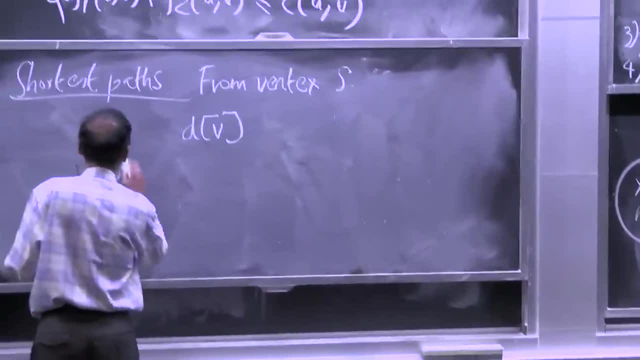 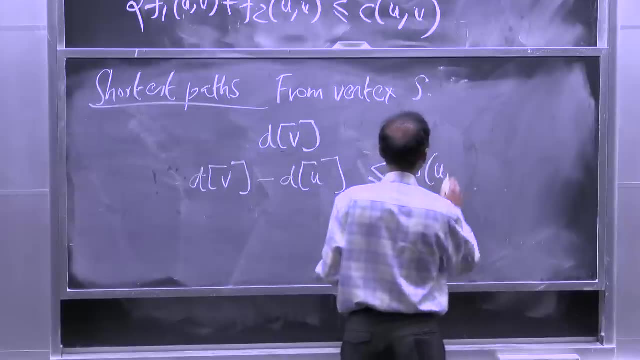 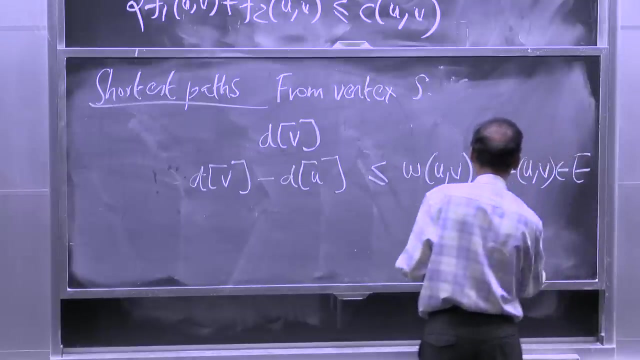 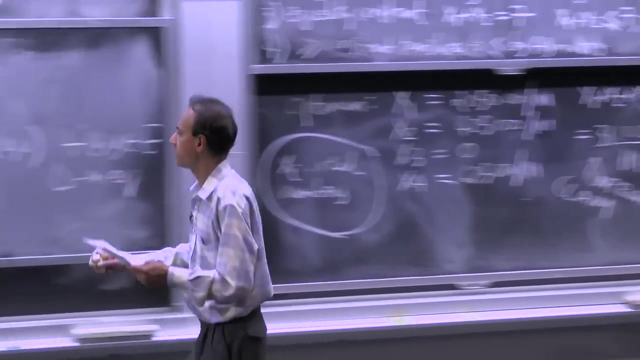 In particular. what we have here is that I can write: dv minus du is less than or equal to wuv for all uv belonging to e, And that's the triangle inequality. OK, And I'm going to have d of s equals 0.. 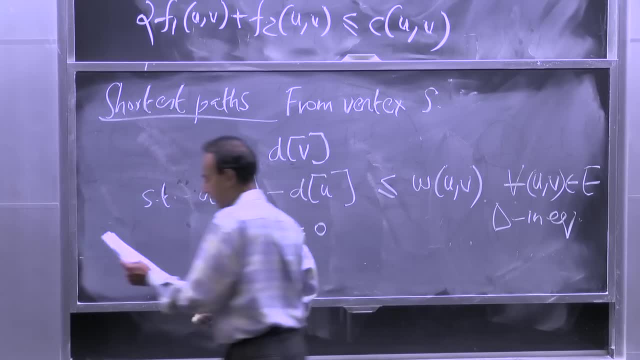 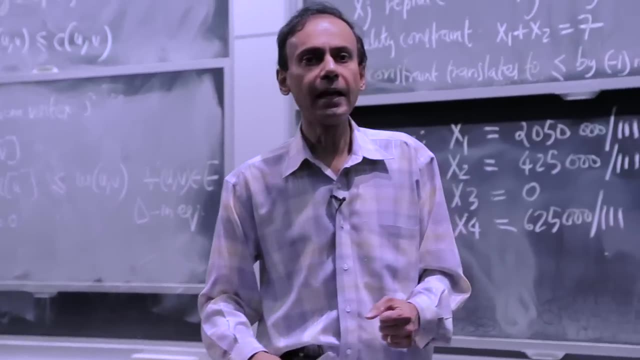 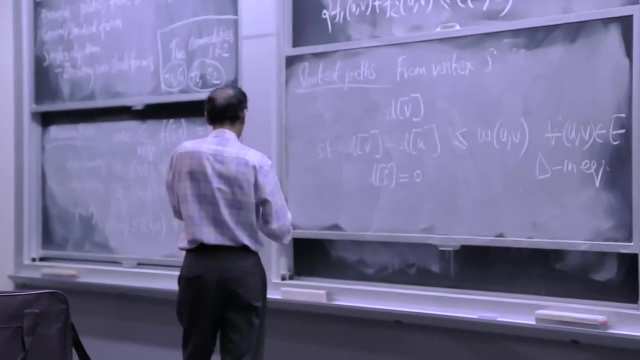 That's the only thing that I start with, right, And so what's happening out here? It's simply that there's different ways of getting to v, And my shortest path is going to be the best way of getting to v. So, in particular, the way you want to think about this, 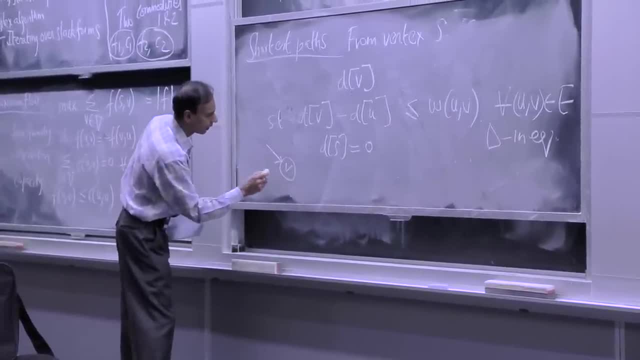 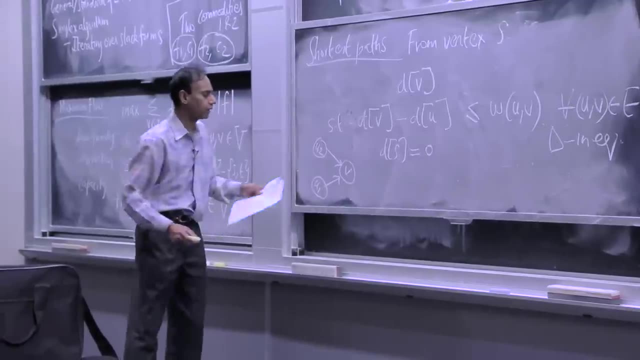 is that if I have a v and I can get to it from, let's just say, u1 and u2, and maybe the source is over here- and these are the only two edges that can get to v right. So I'm just looking at a fairly limited setting. 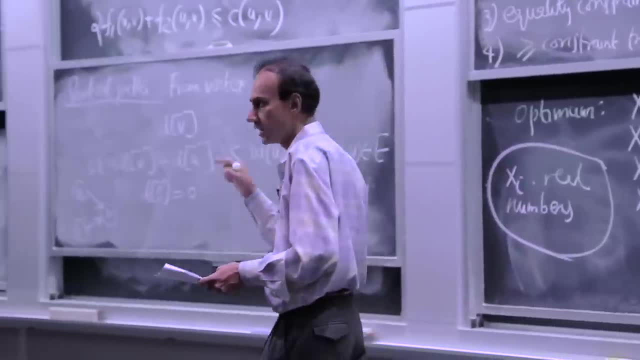 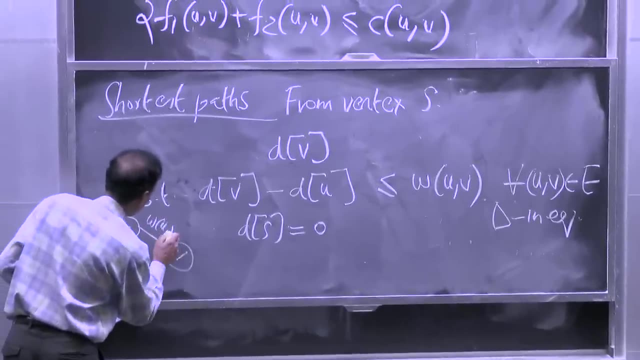 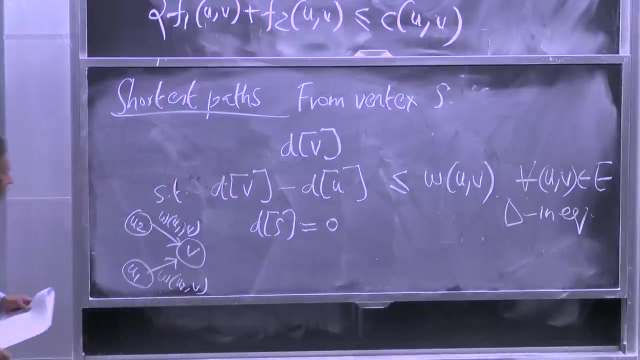 u1 and u2 are going to have to be the two vertices. One of these two is going to get me to v, right, And I got w u1 v here, And I got w u2 v over here, right, And so what this is saying is: I'm going 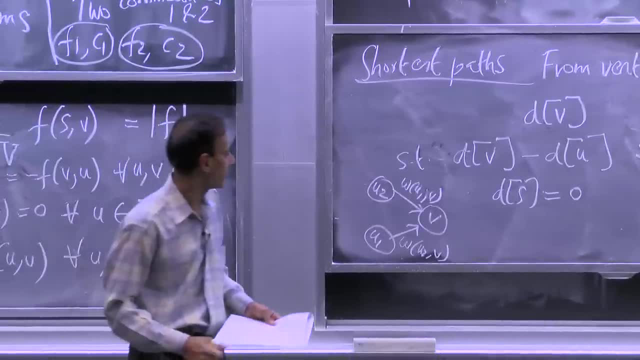 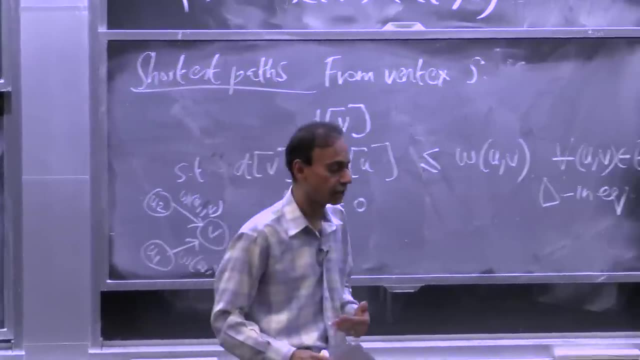 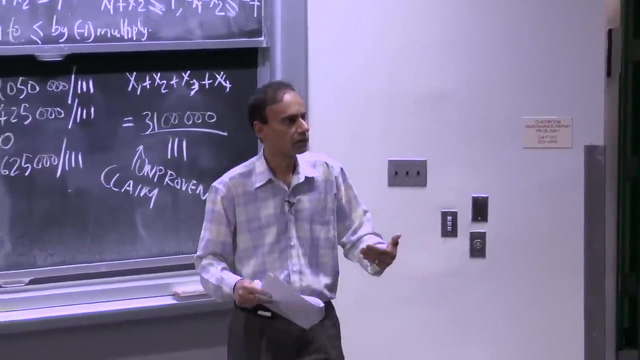 to have to write this out for each of these edges. For each of these edges, I'm going to have this constraint And that says that the dv value, if I want the shortest path, should obey both of these constraints. And if I want to obey both of these constraints, 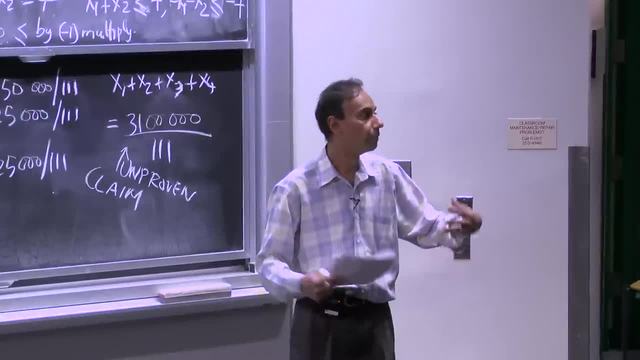 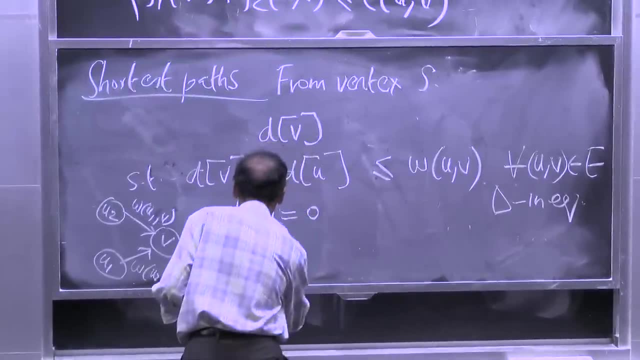 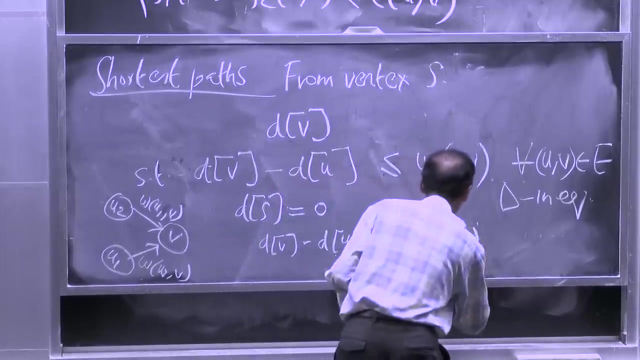 one of them is going to be my limiting constraint And I'm going to get the min of those two Correct. So, in effect, what this translates to it's an and right. So dv minus du1 is less than or equal to w u1 v. 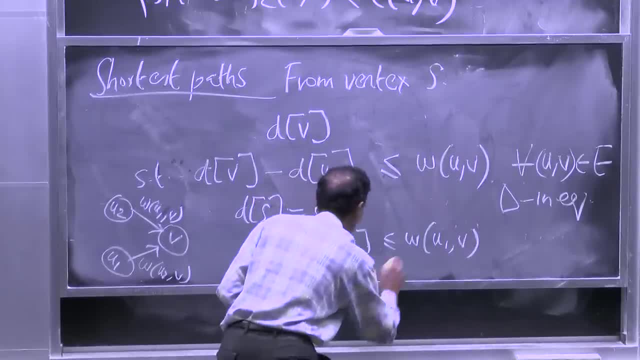 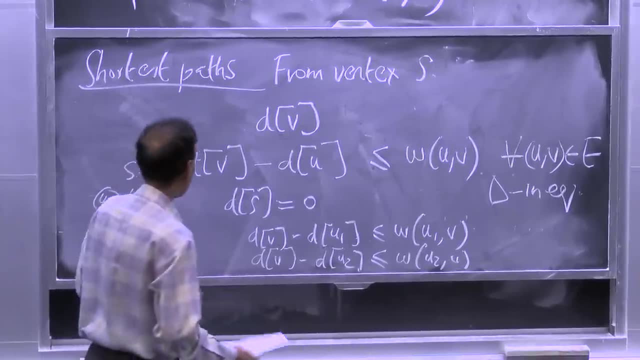 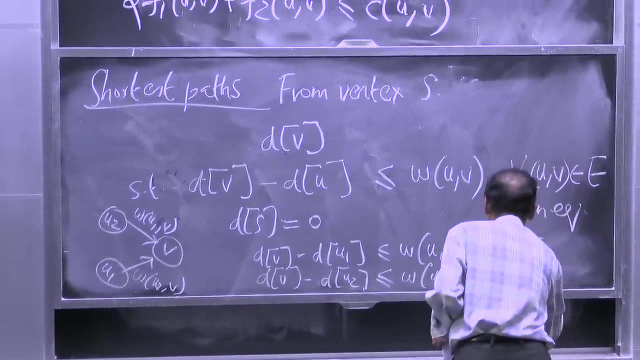 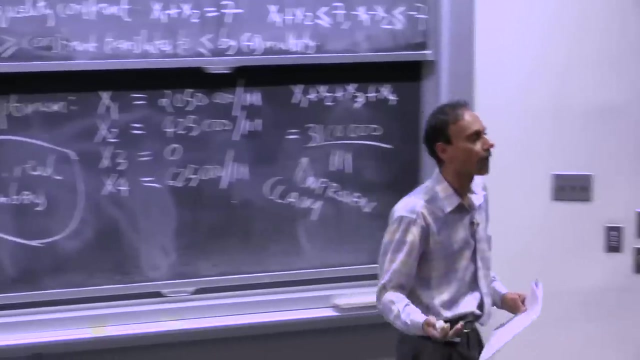 dv minus du2 is less than or equal to w, u2, v. That's an and because I'm putting both of those constraints in here, And that essentially means that dv is going to be the min of the two quantities, the du1. 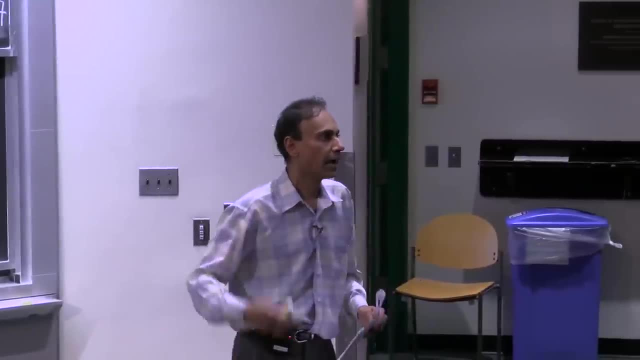 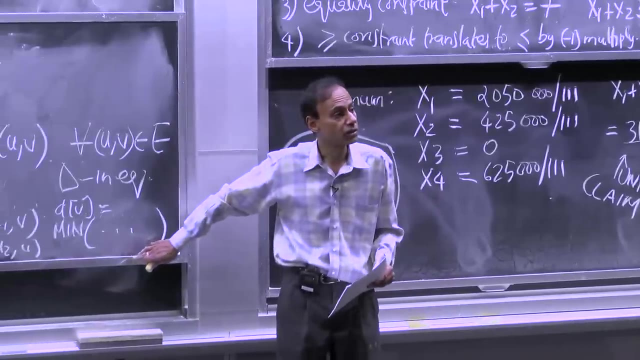 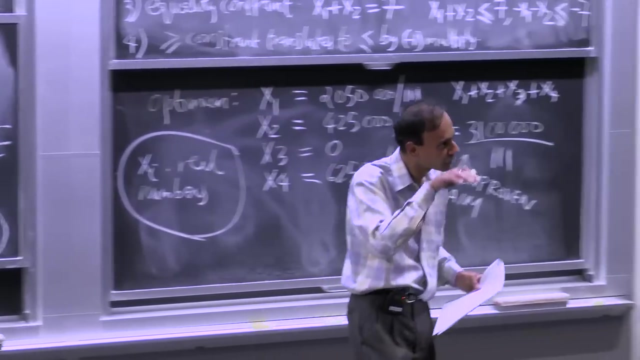 quantity plus the w u1 v and the du2 quantity plus the w u2 v. That makes sense. Ask me questions if this is unclear. So that simply corresponds to the fact that I'm doing an and over here. I'm adding all of these constraints in there. 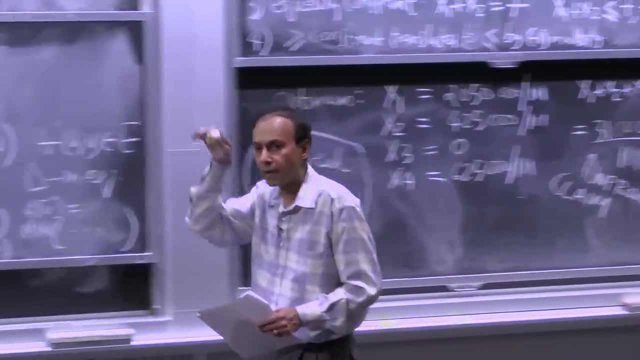 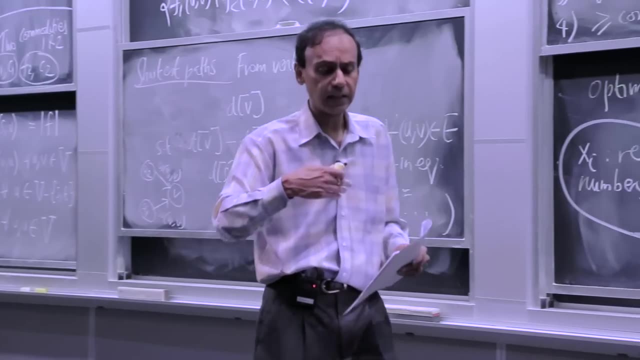 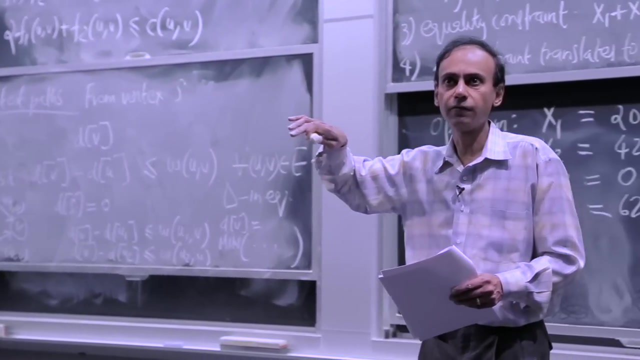 So I'm applying the triangle inequality to every edge, to every relationship between a vertex that has a path ending at it And you're pushing it forward to this vertex. v. All the differences, All the different ways that you can get to v. 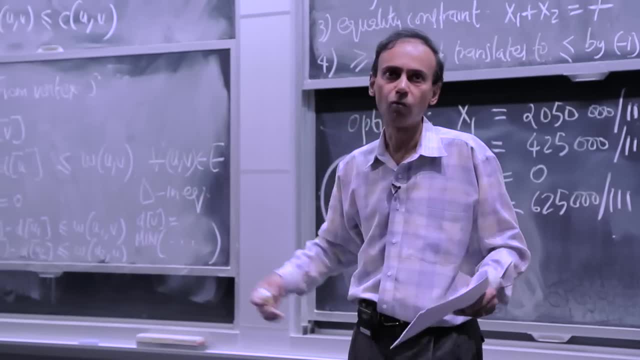 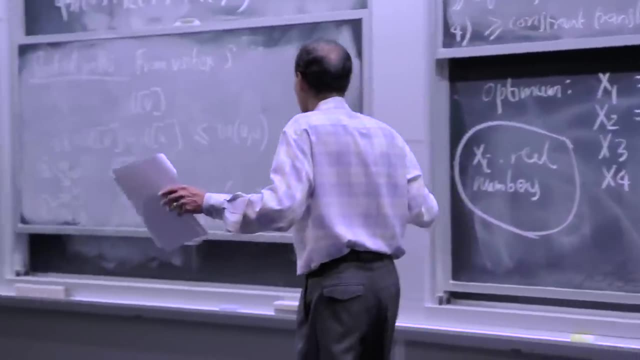 In this case, there is two sets of ways, one from u1 and one from u2.. And the last step is a minimization step. All right, OK, so you think you're done or we're done, but we're not quite done. 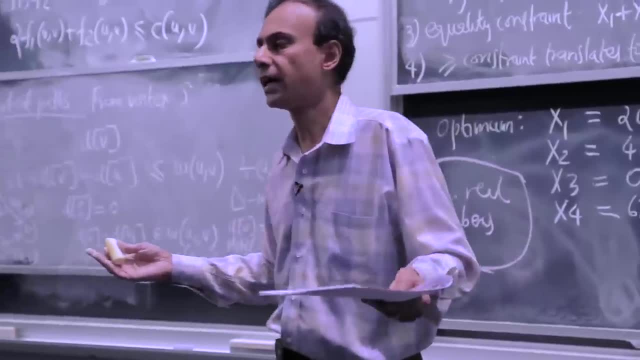 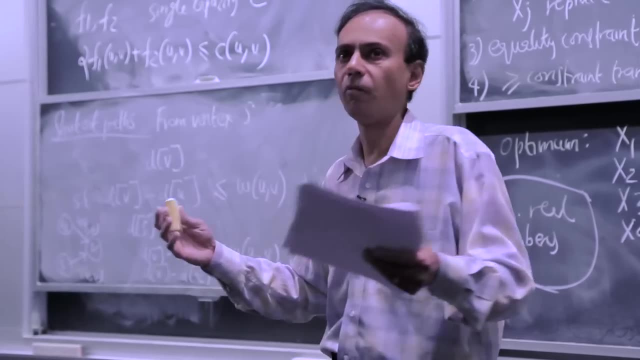 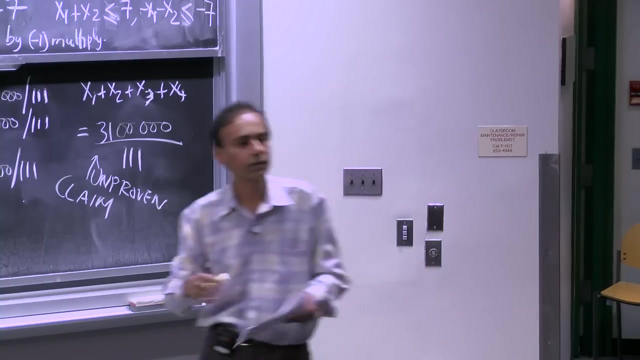 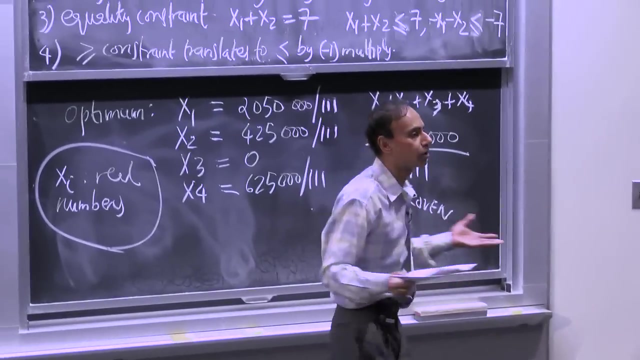 Because what's missing here, in terms of my formulation of Lp, What else do I have to do here? Well, sure, Non-negative, Let's do that. Sorry, Objective, Objective. Who said objective? You again. So we are missing an objective function. 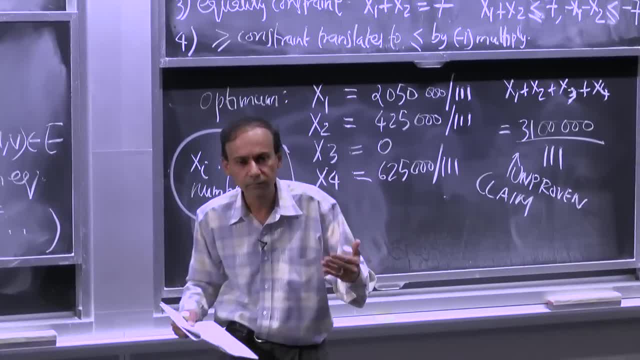 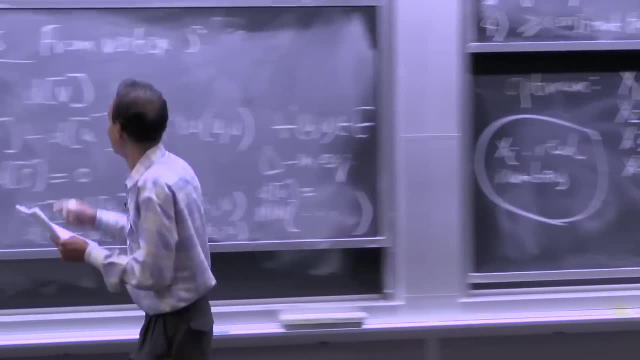 Right Now, shortest path is what kind of problem? again, Short means minimum, Right, Minimum, Minimum height, whatever. So what happens if I put a minimum in here And let's say that I do something like Minimum Minimum? 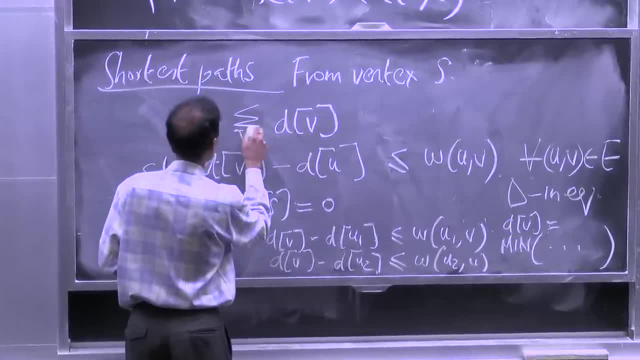 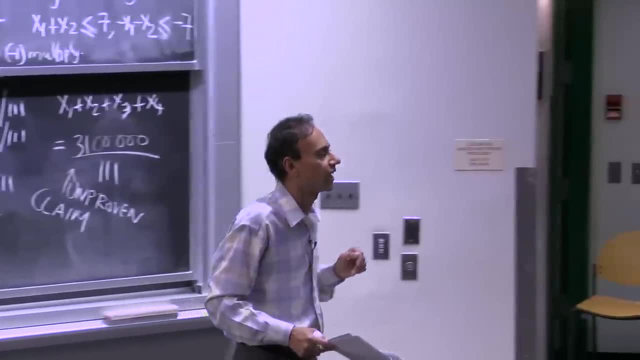 Minimum, Minimum, Minimum Sigma over v, cap, v, dv, because I want to minimize, Or I could pick a particular one, I could pick a particular single source, single destination and I put a minimum there. OK, What happens? 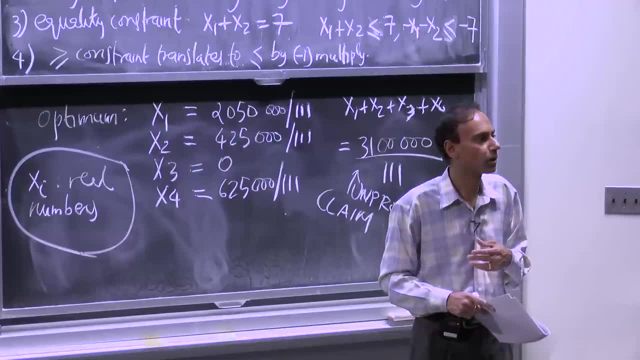 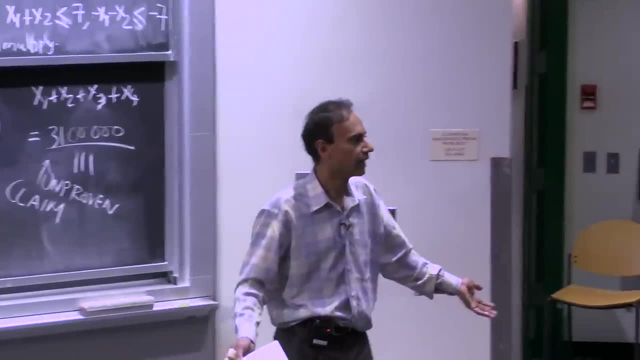 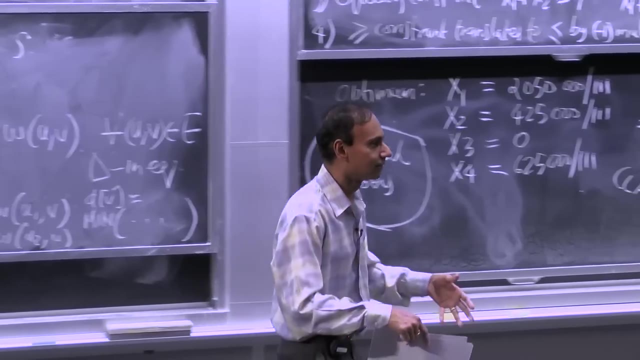 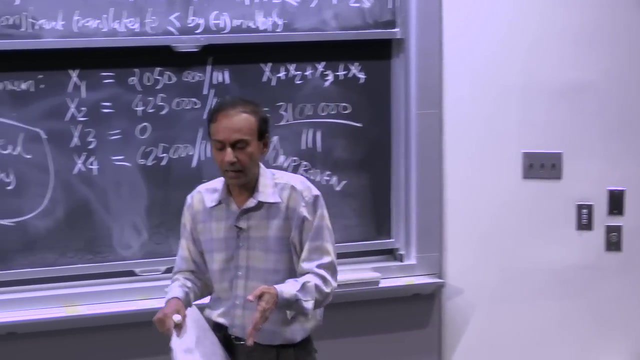 Does this work? What's the solution to this problem if I minimize the distance 0, because the 0 value is going to work Right. So there's something I haven't put in the constraint that I do want a path. I do want a path from s to v for any v that matches one. 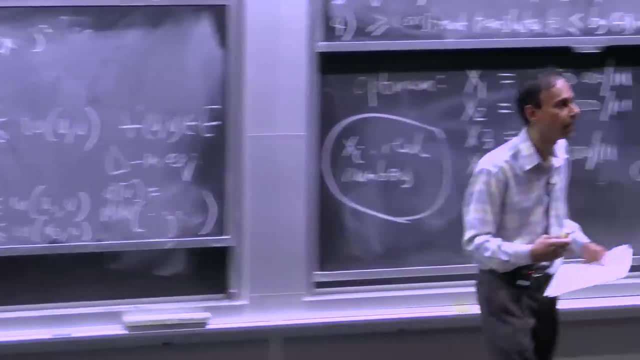 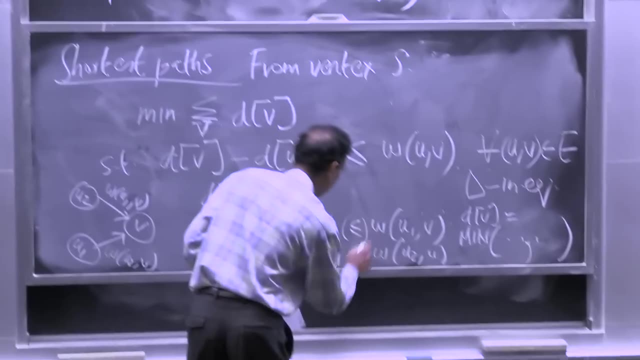 of the quantities in the min, because the min says: I have equality, Right. The big issue here is: this is a less than or equal to, And that's why the min doesn't work in the objective function. All right, It's a less than or equal to. 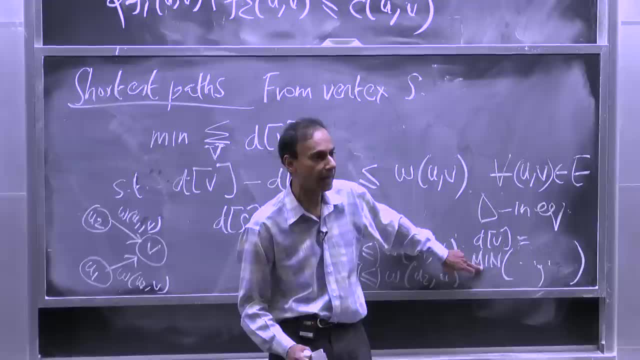 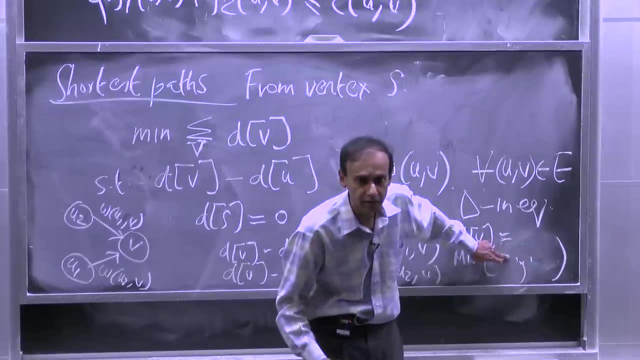 But this min over here, which is the definition of a shortest path, is saying that it's either equal to this quantity or equal to that quantity. There's an equality over here that is missing from this side Right, And that's the key observation. 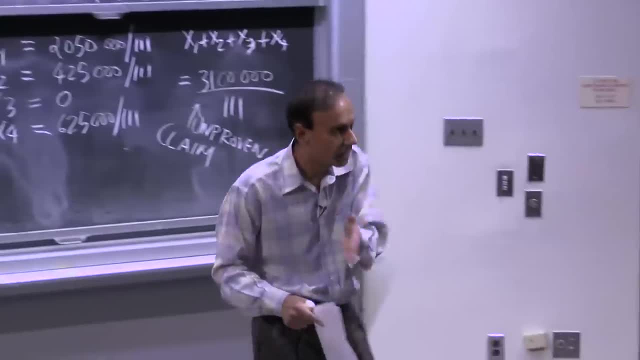 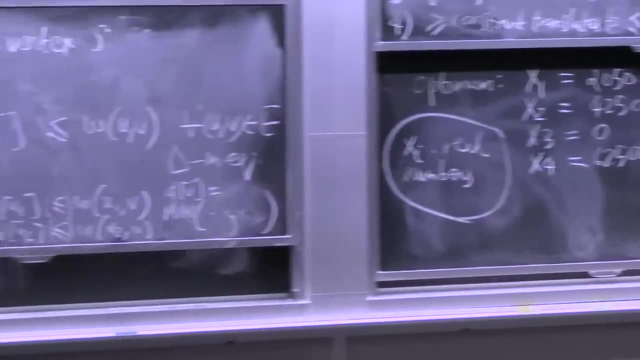 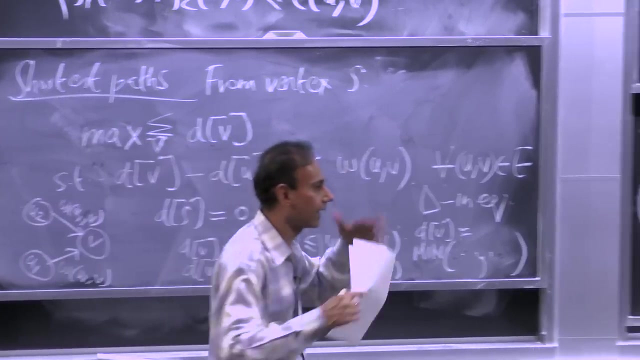 Once you've observed that, that you need equality for one of these constituent quantities of the min, then you'll see that what you have to do is simply change this min. It's going to change into a max. OK, So you say: how the heck did a min change into a max? 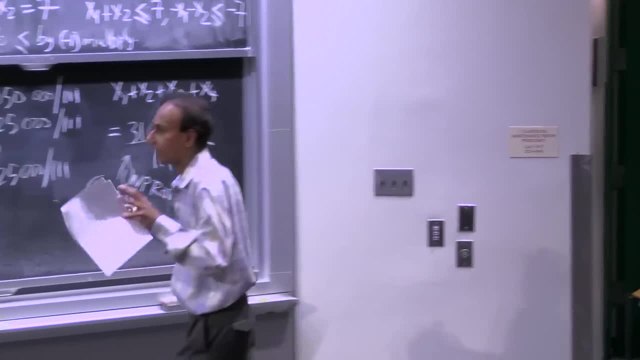 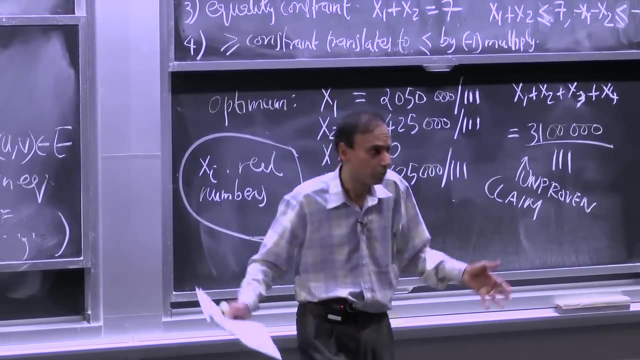 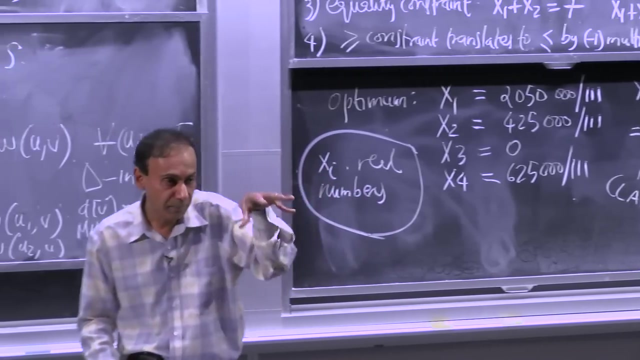 And I'm not sure I'm going to convince every one of you in the next minute or so, But the bottom line is it comes down to I do have a min already in my inequalities because I'm anding each of these inequalities and I'm putting down each of those inequalities in there. 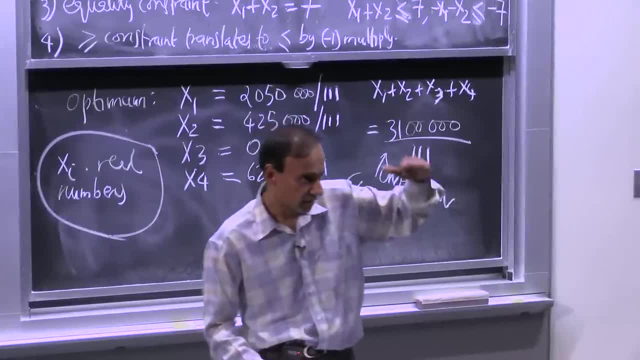 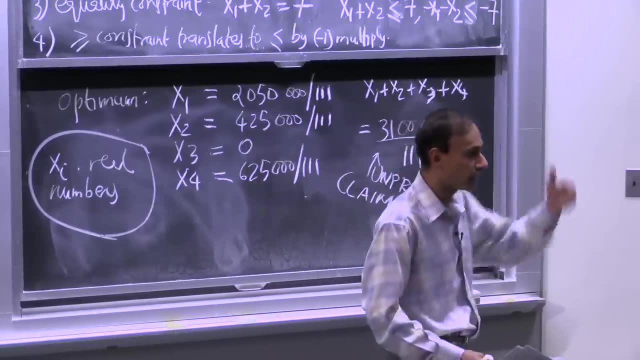 Right. So each of them is going to force me into a new condition, because they're going to constrain me to not go via u2 if u1 is better, because the other constraint, corresponding to u1, is going to force me down, Right. 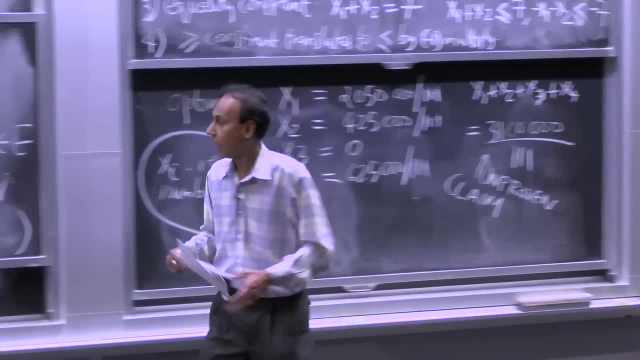 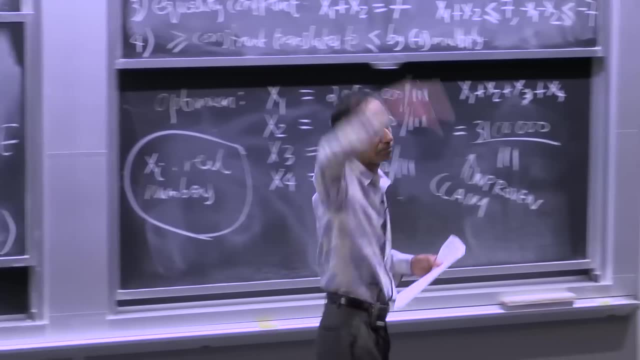 So there's an additional min in there, because the anding of the less than or equal to's And then in order to actually force the equality for one of those, I need to push up as hard as I can or as high as I can. 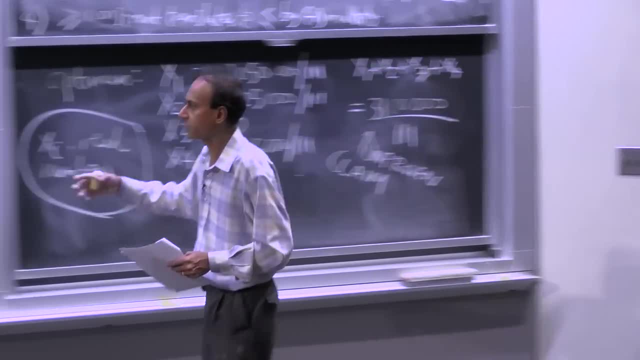 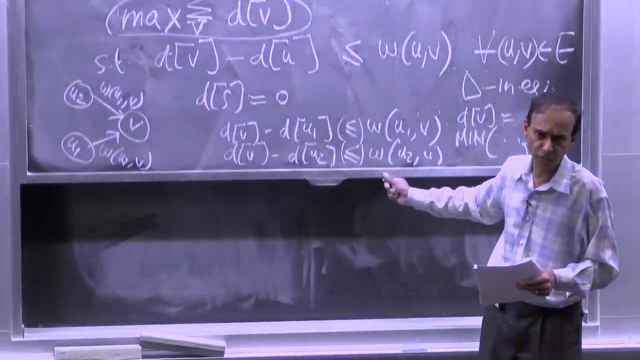 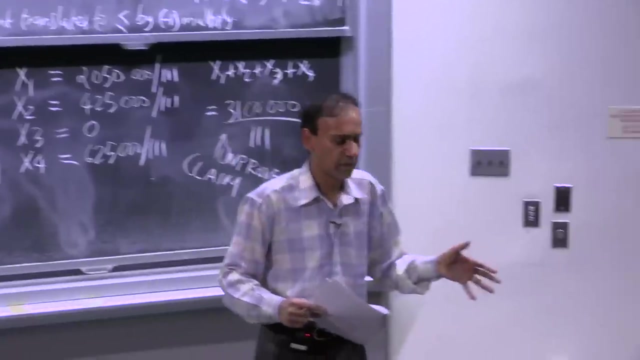 All right, So think about it. Play around with a couple of examples. I choose A simple example for starters and you'll see that this is the correct formulation. All right, So you can see that it's not completely clear in some cases. 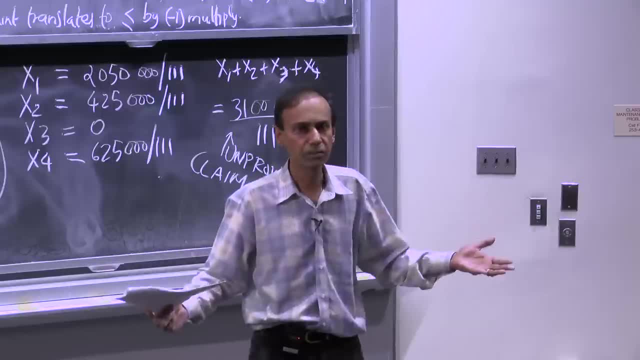 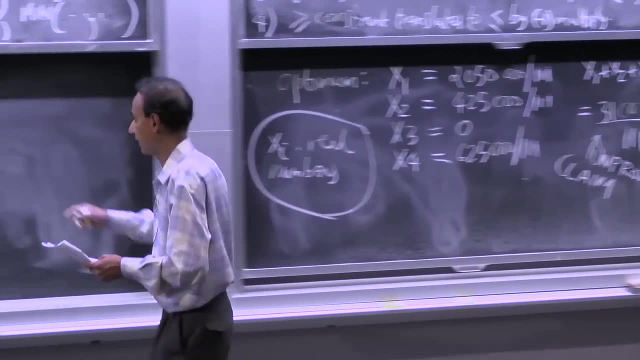 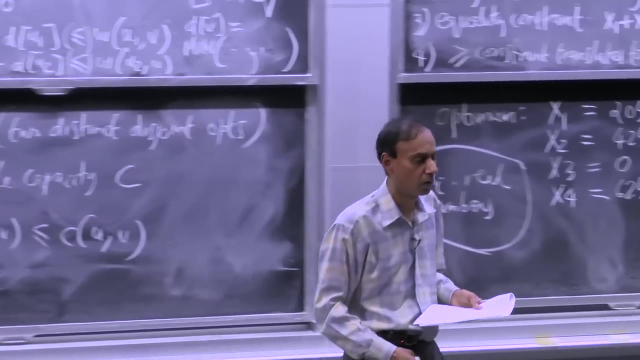 how to transform problems to LP. But even in those cases sometimes you can. All right, So there's just a ton of different problems. A good skill to have to be able to take combinatorial optimization engines like LP or even max flow. 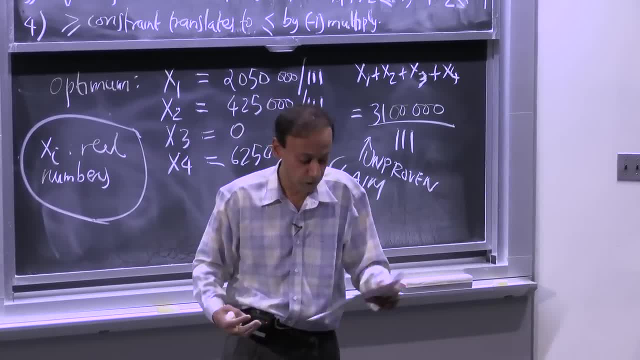 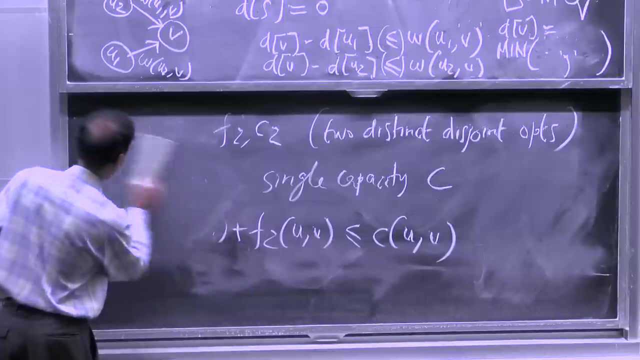 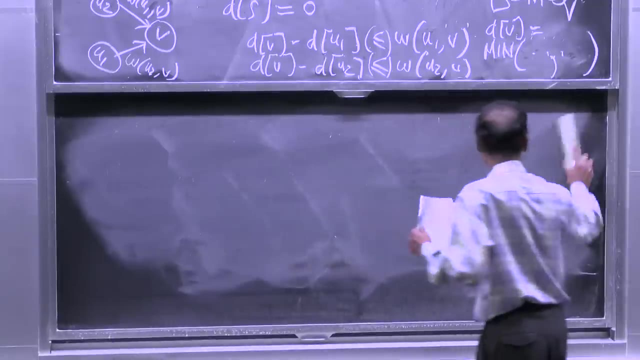 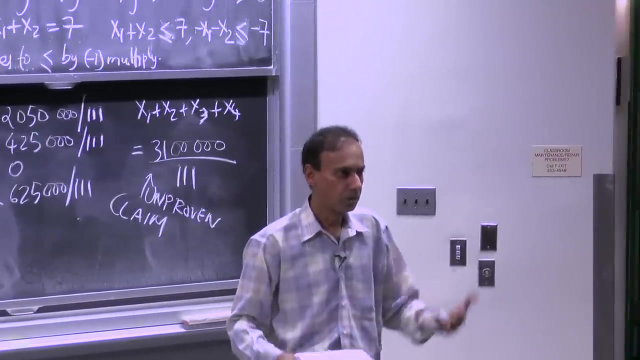 And be able to translate problems to them. This is something that you'll probably do if you stick to algorithms in your careers or exploiting available algorithm packages. So the last thing I want to do here for the rest of the time is to give you some sense for how an LP program is actually. 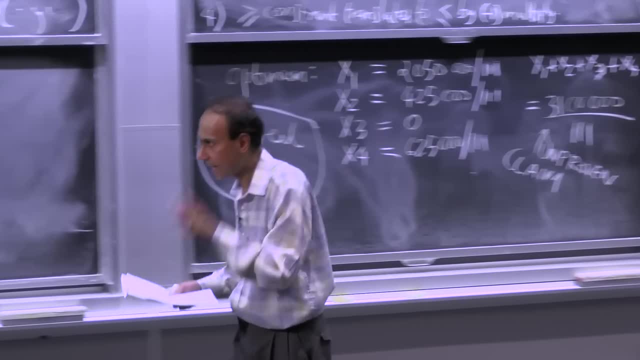 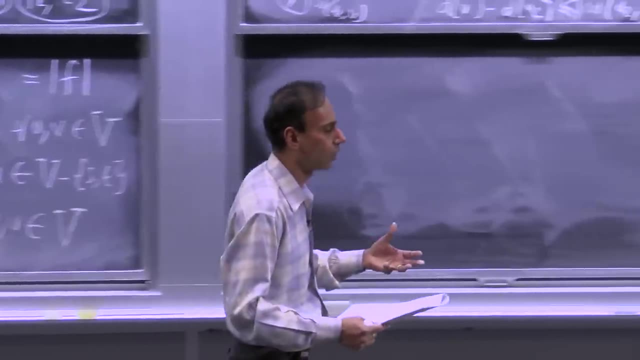 optimized. How can you possibly? How can you possibly, How can you possibly Take the standard LP formulation, which is a general setting? You know nothing about shortest paths. let's assume Nothing about max flow. It's not about a specific problem. 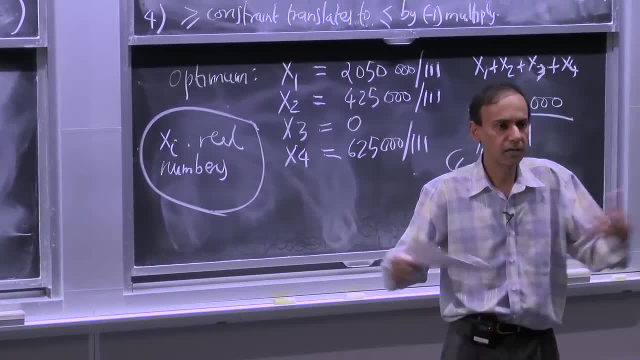 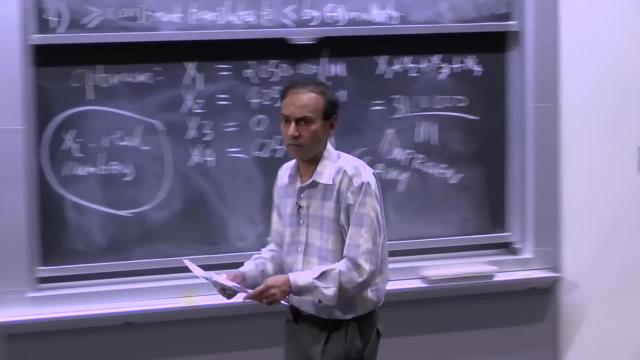 It's about the general setting. How can we solve the general setting? Because that was the theme here. anyway. You had this engine and you want to use this engine, But now how do you build this engine? So what we're going to do is look at a fairly simple example. 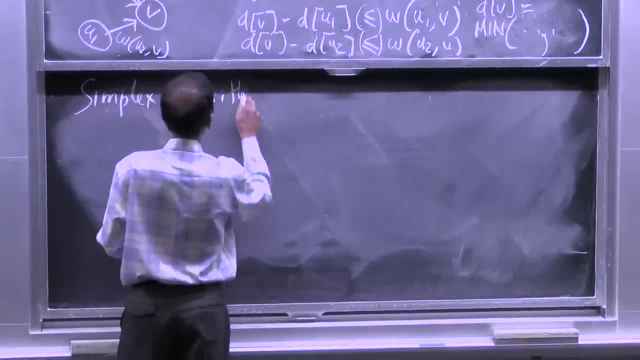 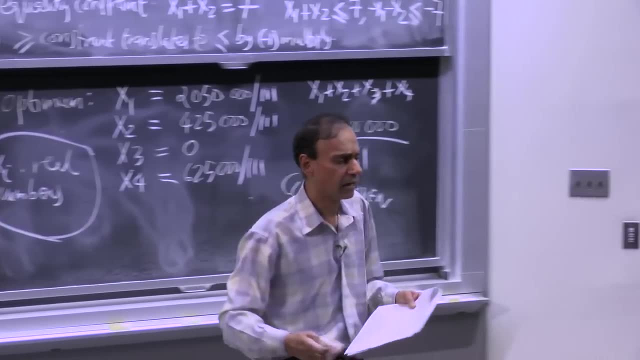 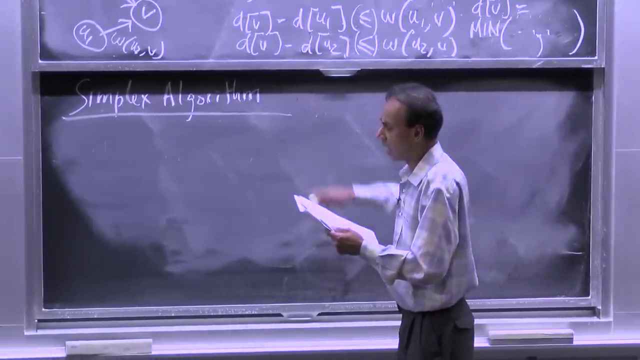 of the simplex algorithm: And And, And And. this algorithm is in the textbook And it will be in my notes, So I'll get as far as I can. It's not that complicated to describe, especially from an example standpoint. 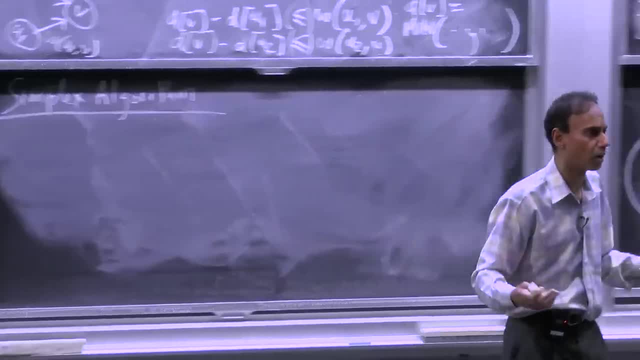 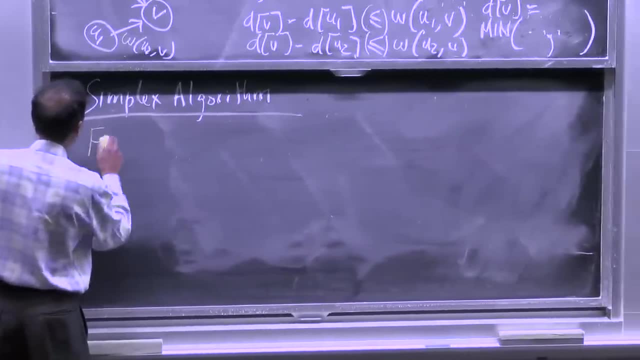 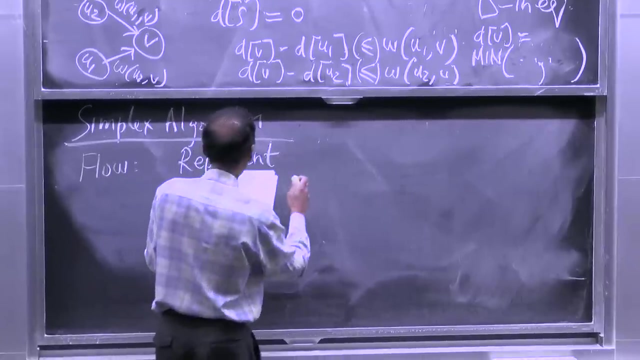 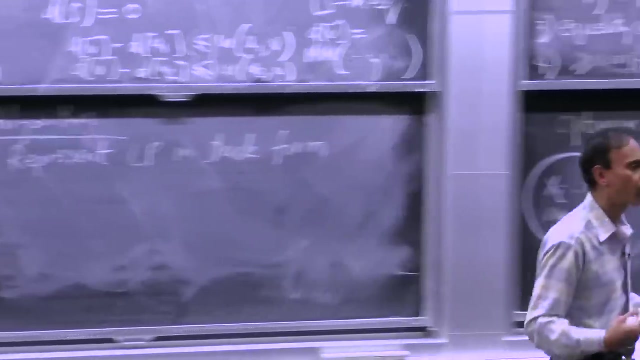 But I may not get through all of the steps to get you the optimum for this particular example, given how much time we have. The most important concept in simplex is yet another form of representation for simplex, which says that you can represent the LP not. 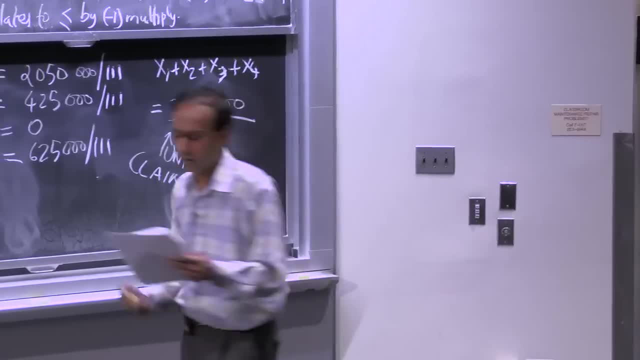 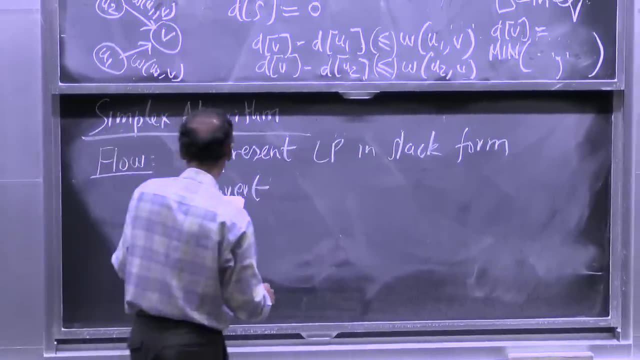 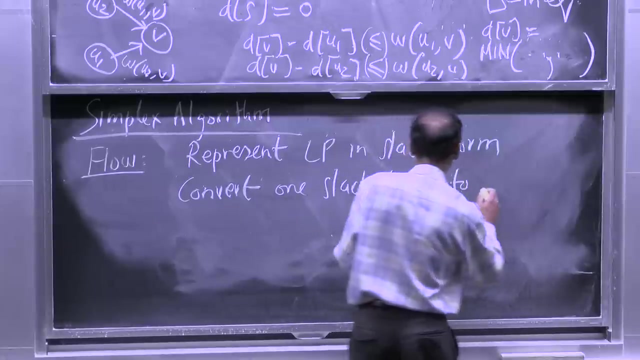 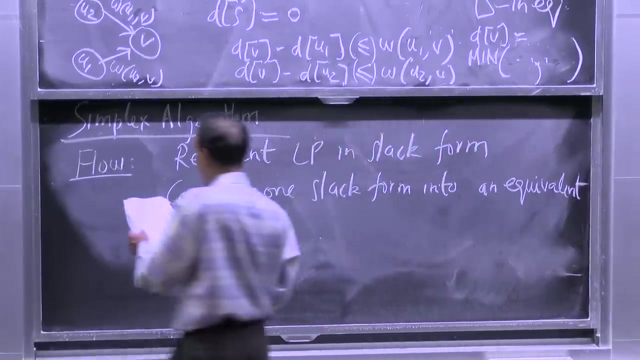 in standard form, but in slack form. So I'm going to tell you what slack form is, And then what we're going to do is the flow of simplex. algorithmic flow is to convert one slack form into an equivalent. obviously, you don't want to do something that's incorrect. 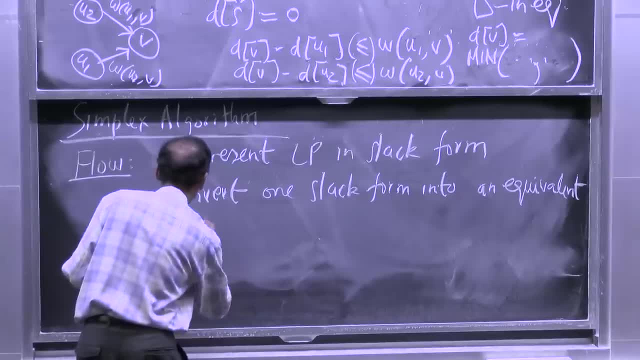 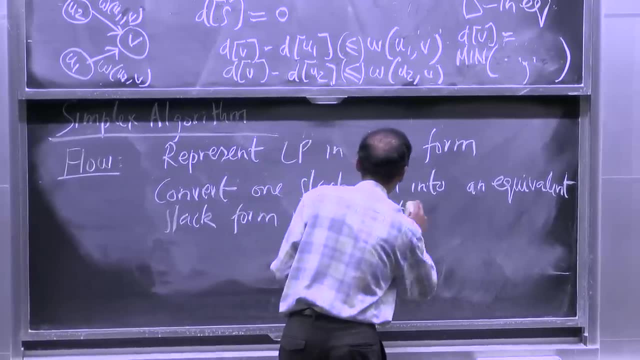 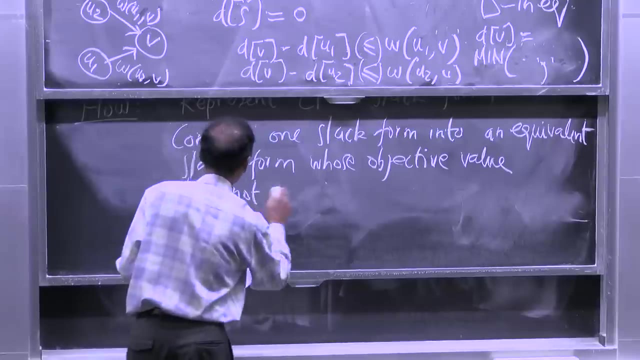 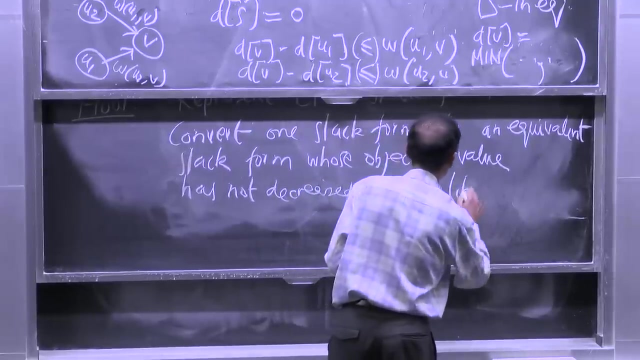 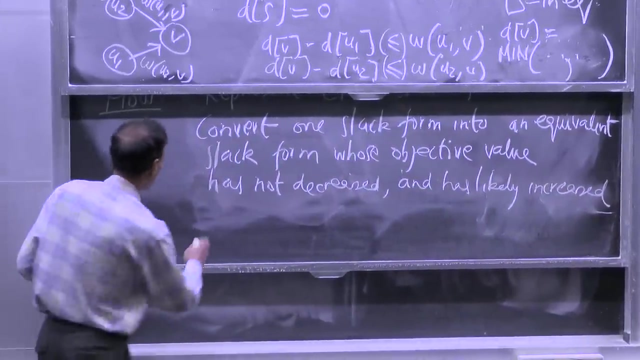 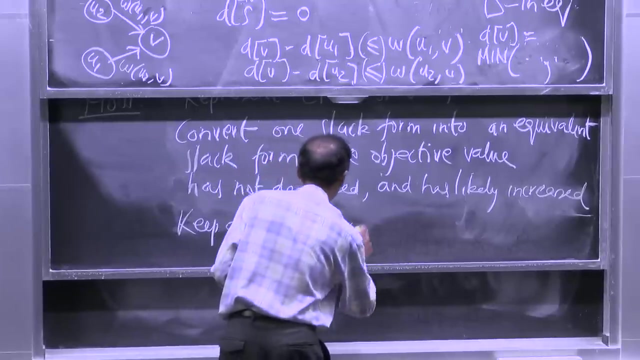 But it has to be an equivalent slack form whose objective value has not decreased and has likely increased. So you're guaranteed that the objective value has not decreased, You're not guaranteed that it's increased, And then we're going to keep going till the optimal solution becomes obvious. 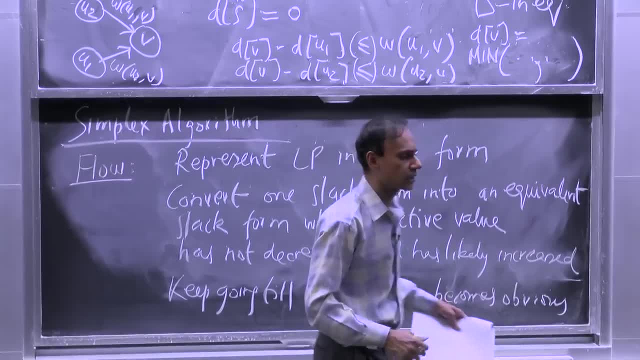 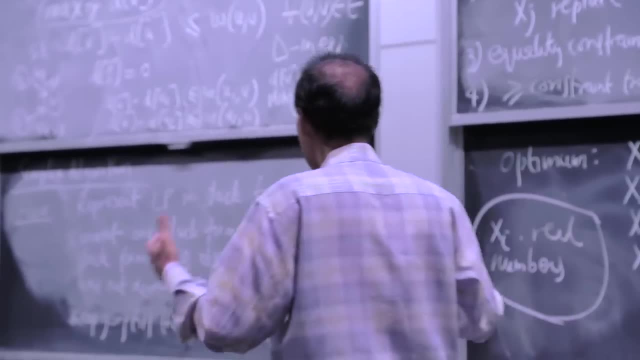 And you might say: how is this obvious? That's the reason why I talked about the short certificate of optimality. It's definitely a relationship between The termination of simplex and the fact that you can now say: hey, I know, I'm done here. 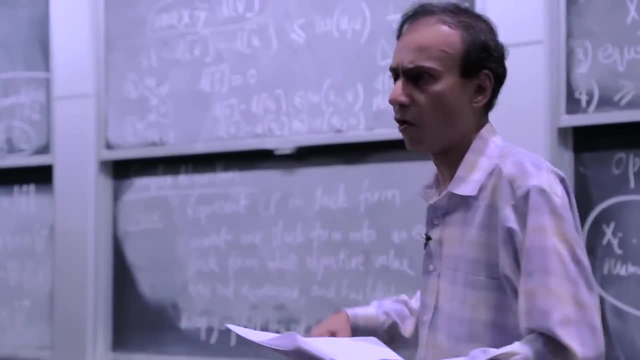 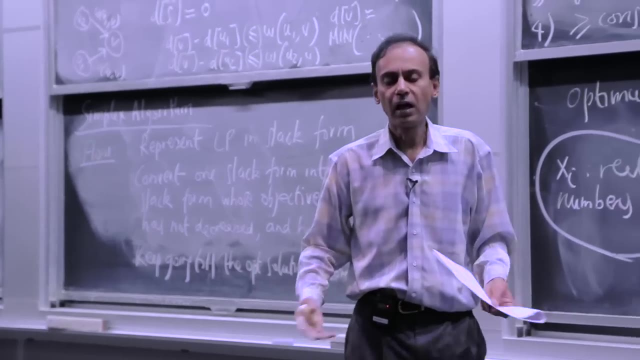 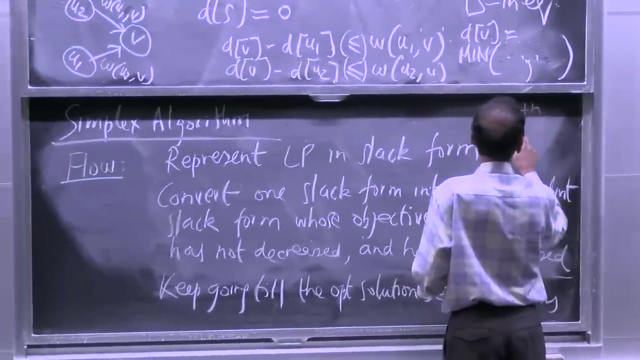 It's kind of obvious that I can't do any better, And hopefully you'll see that by the end of this lecture in this simple example. So that's it. It's an iterative algorithm. It's exponential, unfortunately, because this takes m plus n. 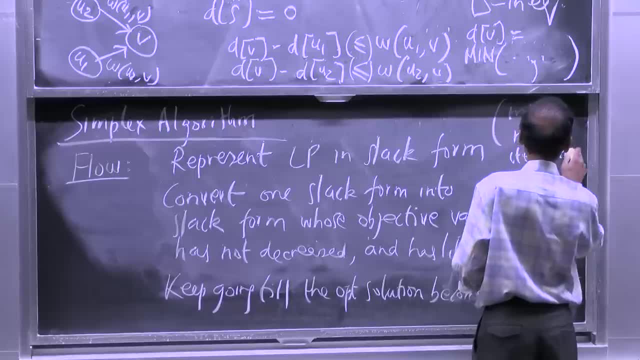 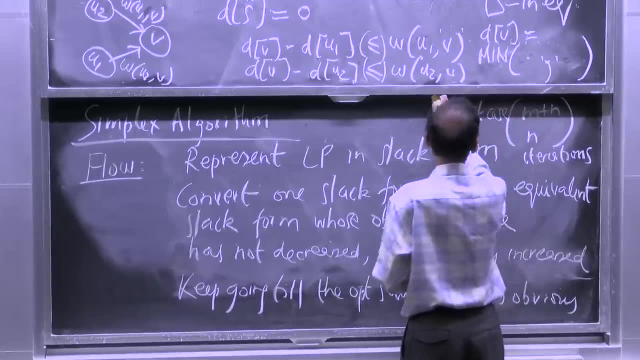 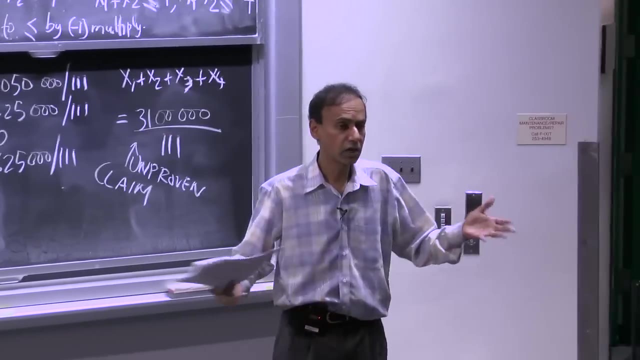 choose n iterations in the worst case, where n is a number of variables and m is the number of constraints. Most of the time it does a lot better, But that's the only bound that you can actually prove in the worst case, And so you're stuck with an exponential algorithm. 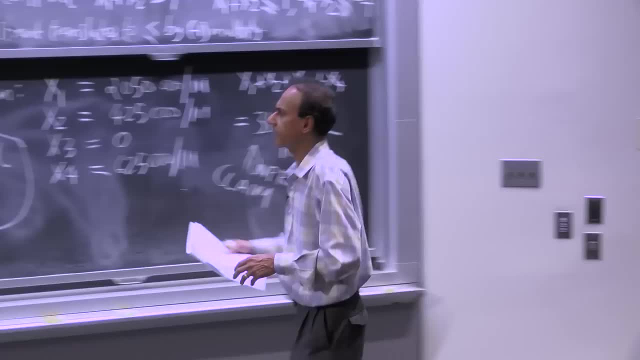 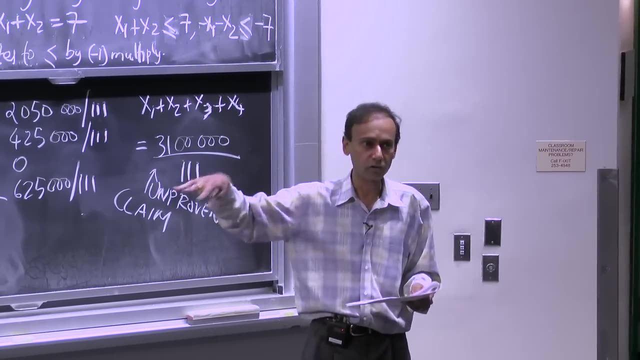 if you're using simplex- worst case- We won't actually do much analysis on simplex. It's really out of scope for 046. in terms of the analysis, The actual algorithm is certainly within scope. So what I want to do is give you some sense. 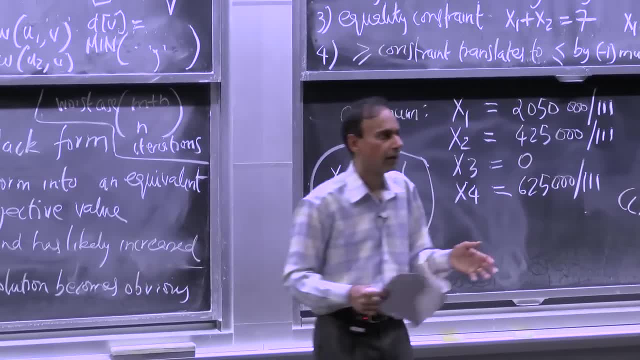 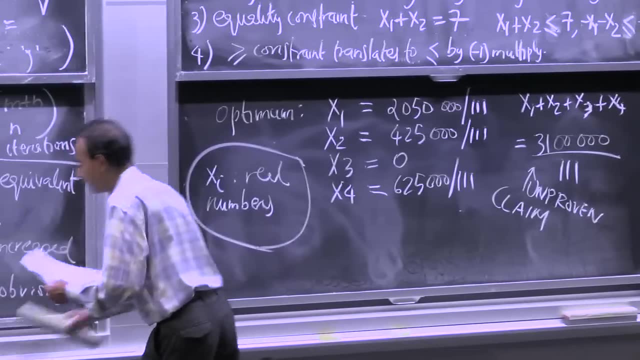 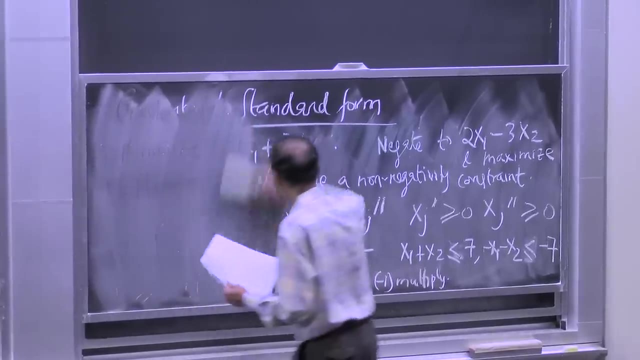 Give you some sense for what the slack form looks like And we'll do a couple of iterations of simplex And we'll get as far as we can before the end of the lecture. So we'll take a different example from our political example. 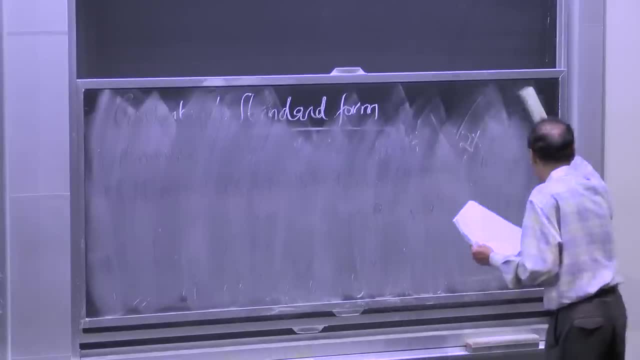 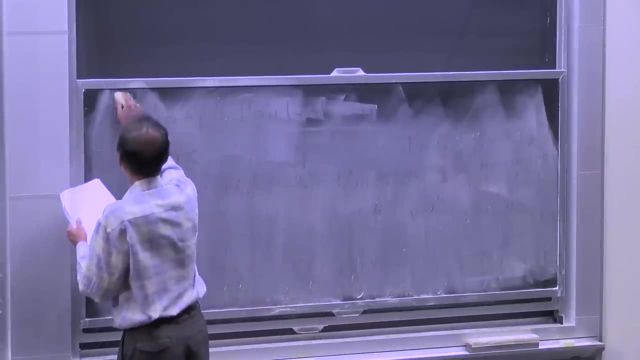 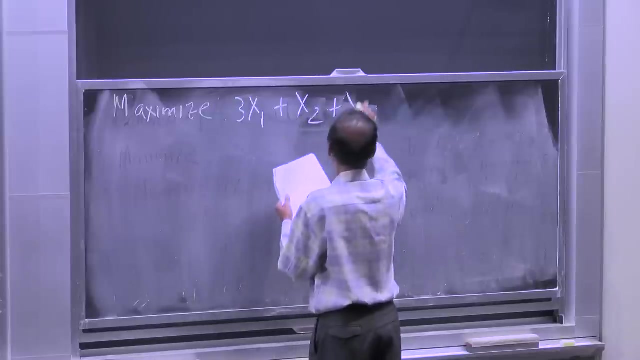 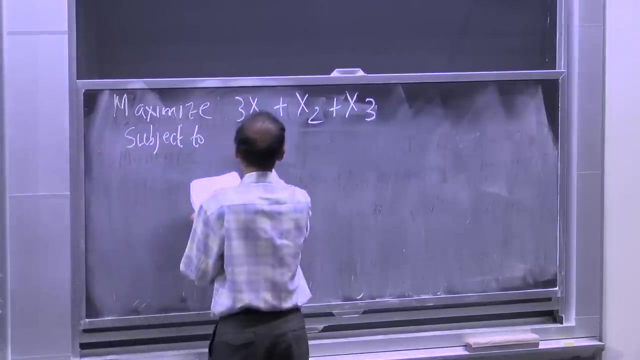 It's similar in size And I want to explain to you what the slack form is and why it's interesting. So what I want to do is maximize And I want to be able to find out what it actually looks like. So we're going to get 2x plus 3x2 plus 3x1 plus x2 plus x3,. 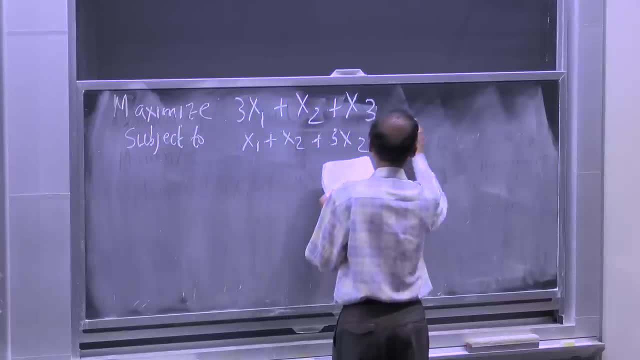 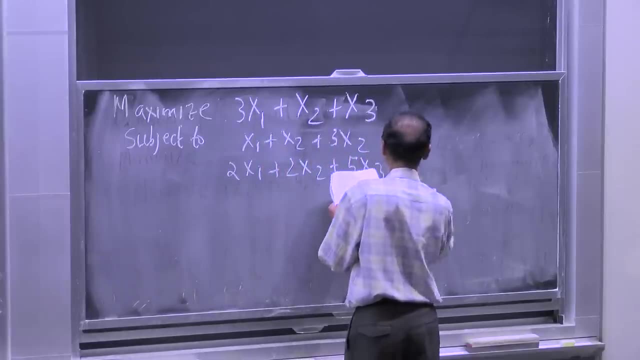 subject to the constraints that x1 plus x2 plus 3x2 is less than or equal to 30, 2x1 plus 2x2 plus 5x3 is less than or equal to 24.. 4x1.. 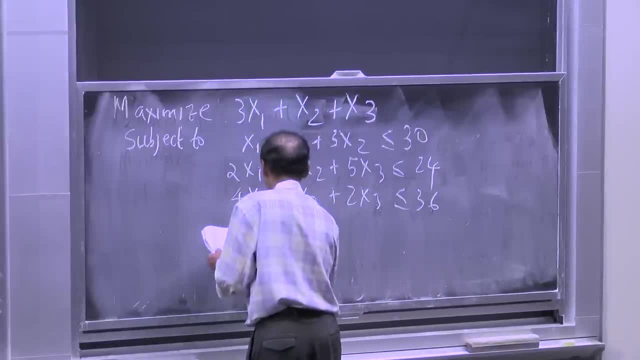 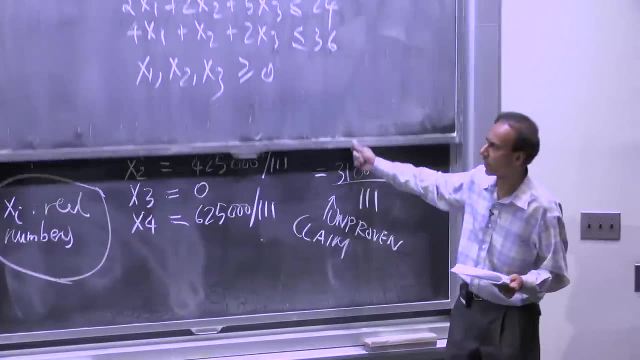 Where's x2?? less than or equal to 36.. And then non-negativity constraints: x1, x2,, x3, greater than or equal to 0.. So that's our example problem. I'll leave it up there. 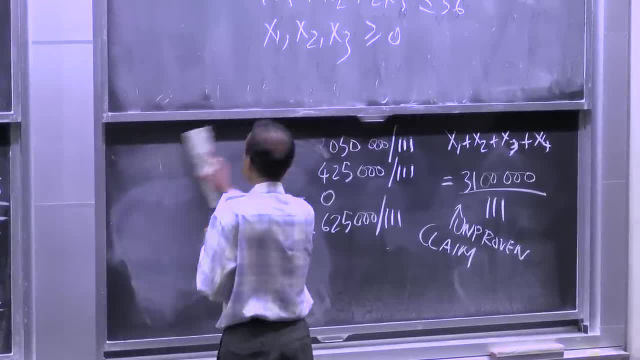 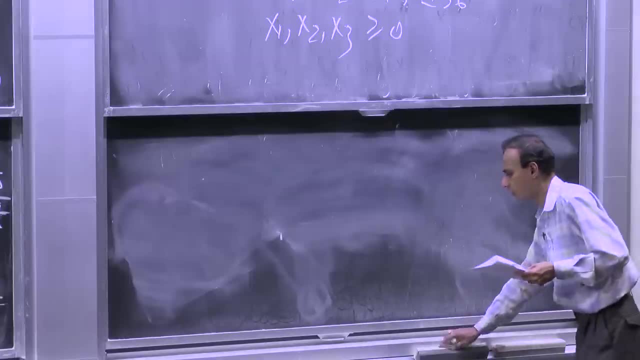 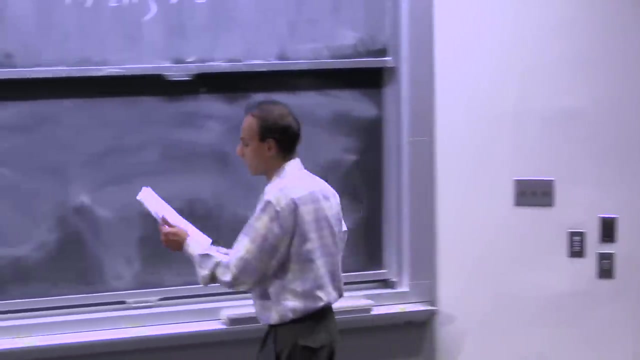 We're going to convert this to slack form. And so what is the slack form? We're going to introduce an additional number of variables that correspond to the number of equations that we have. So we're going to introduce, in this case, three new variables, because I have three equations. 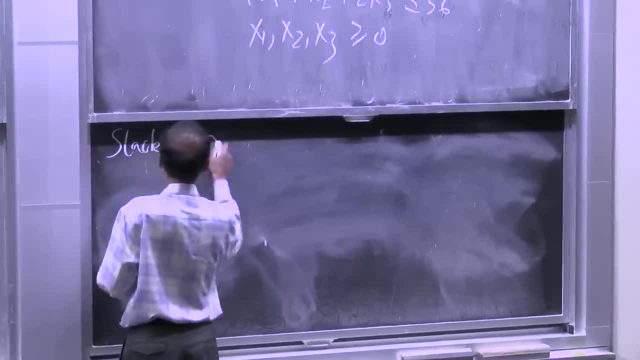 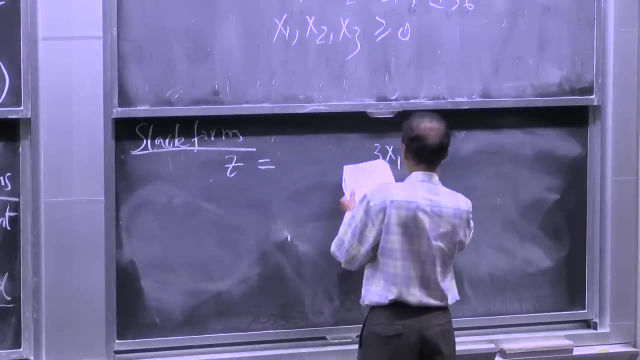 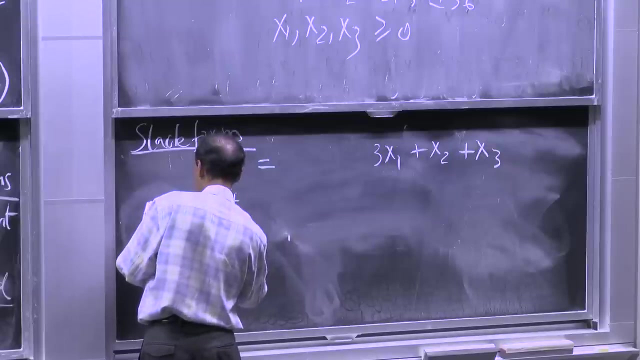 And the slack form for this problem looks like this: I'm going to have z equals 3x1 plus x2 plus x3, same as before- And then I'm going to have variables that represent. these are called basic variables And the original variables are called non-basic variables. 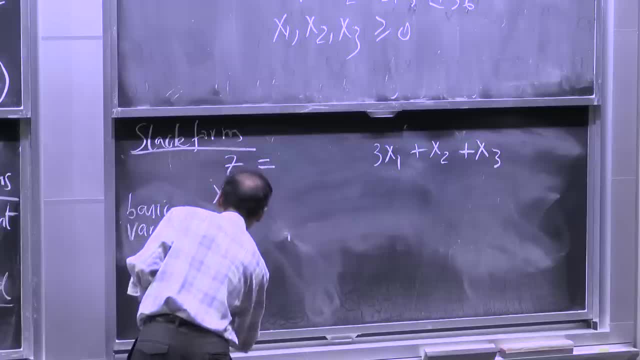 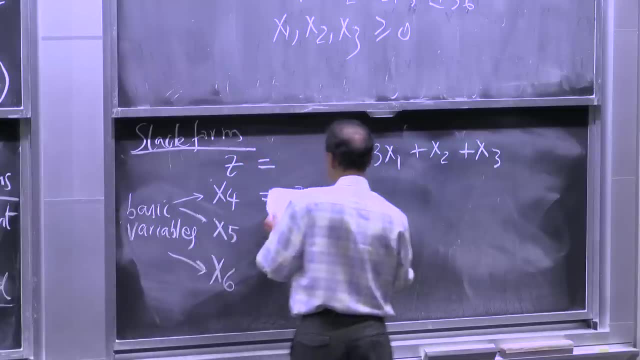 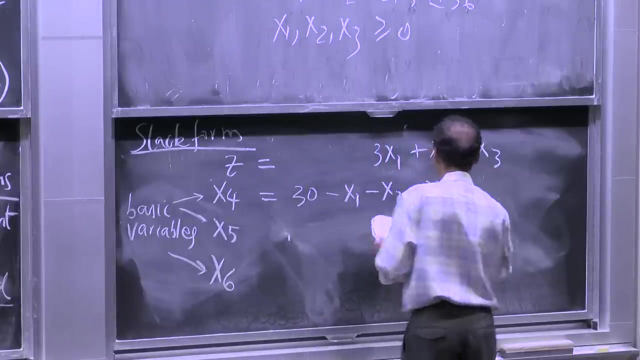 So I'm going to add three basic variables- x4, x5, and x6, corresponding to these three constraints, And they're going to represent slack in the sense that they're going to correspond to how much slack you have in the inequalities that you. 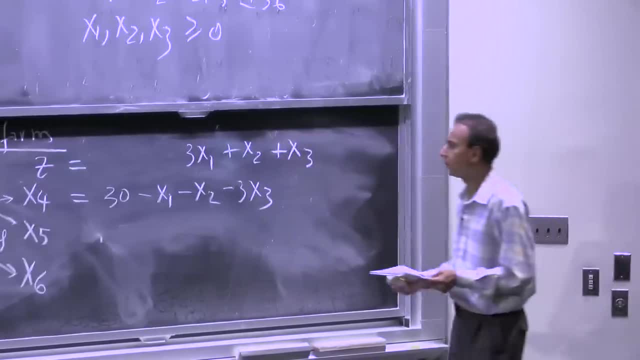 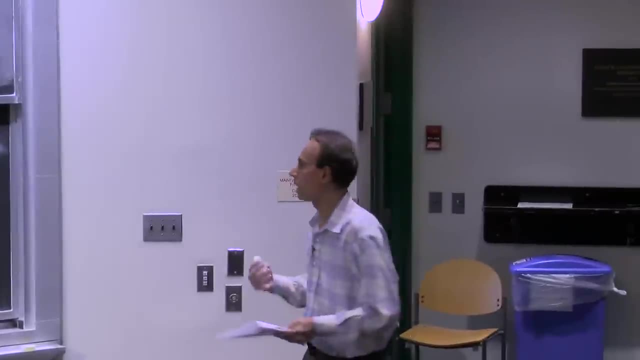 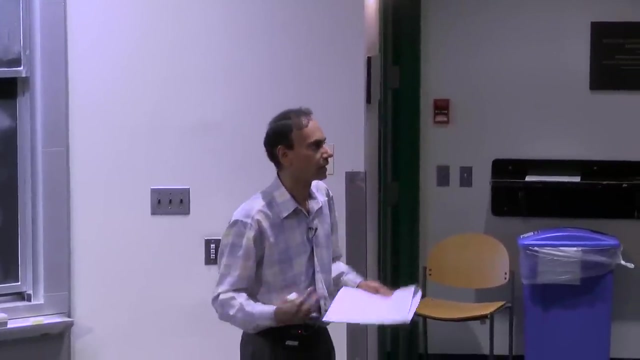 have in the original problem. So if x4 happens to be 0, then you're jammed up. You have no slack, because x1 plus x2 plus 3x3 equals 30. And increasing any one of them It will violate the constraint. 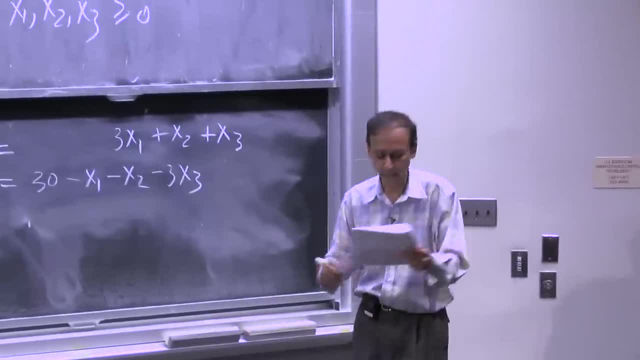 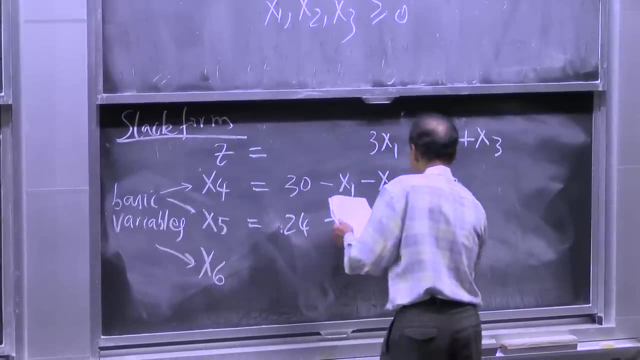 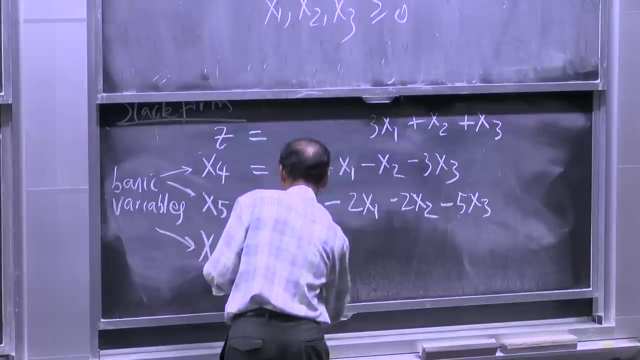 That's just simply the notion of slack. It's: how much room do you have? x5 is 24 minus 2x1, minus 2x2 minus 5x3.. And the last one is 36 minus 4x1.. 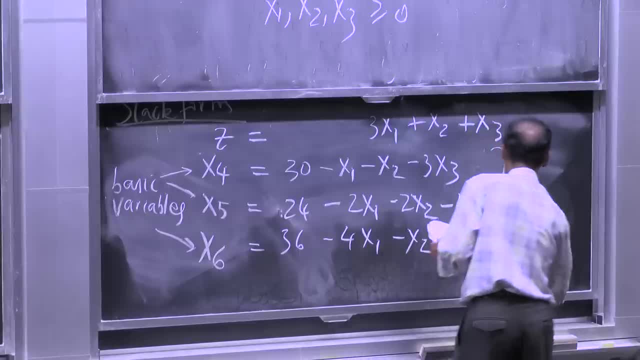 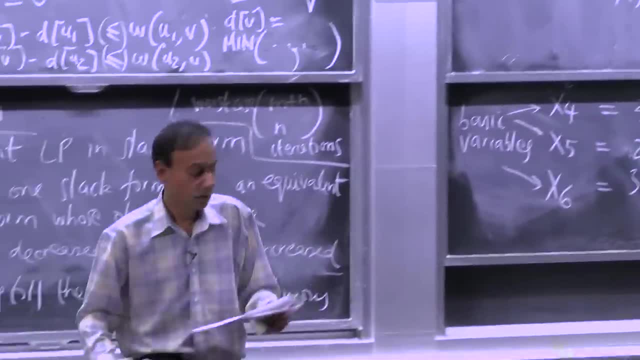 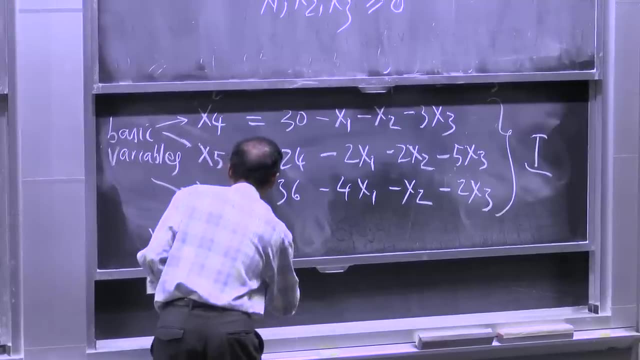 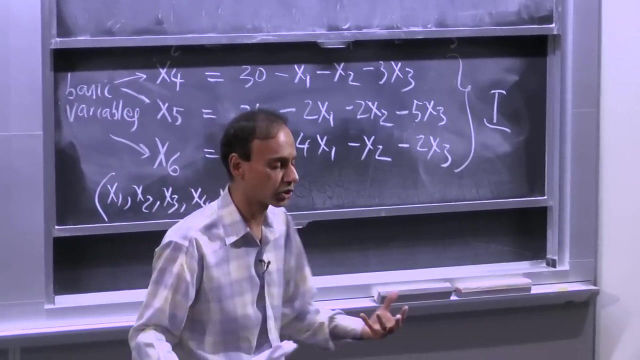 What I'm going to do is I'm going to now work on a space that corresponds to x1, x2, x3, x4, x5, x6.. So I'm going to have these solutions that now have six values associated with them, as opposed. 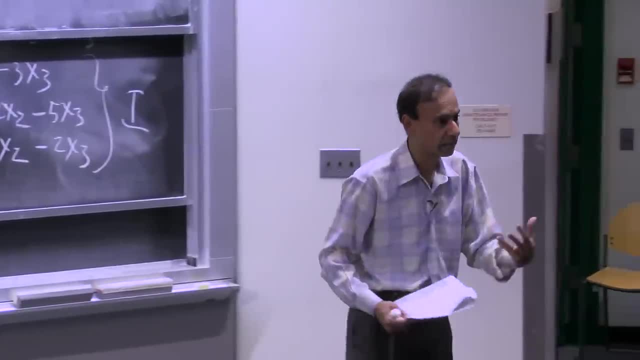 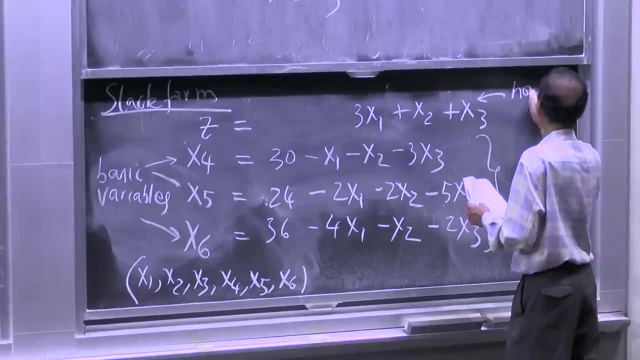 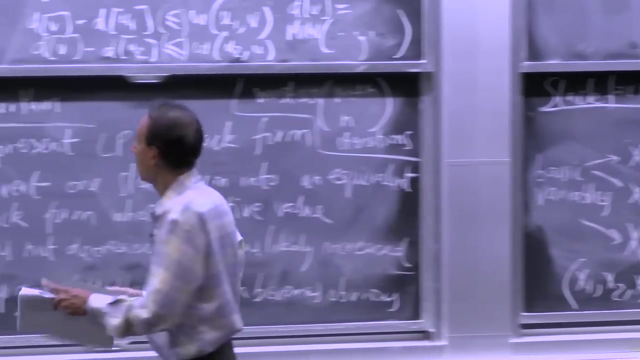 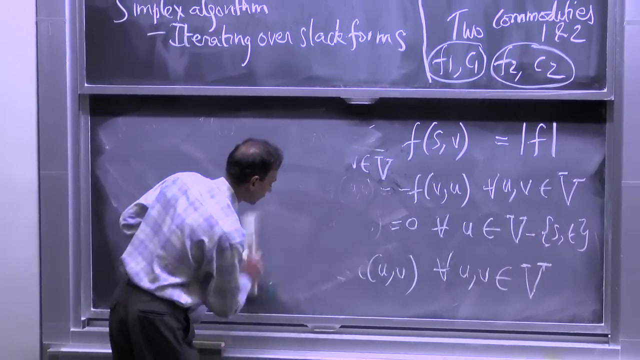 to just three values because they've added three variables- the basic variables- to my non-basic set. So the original variables are non-basic, non-basic, just to differentiate. So so far it's just set up its definitions. We can think about running through iterations of simplex. 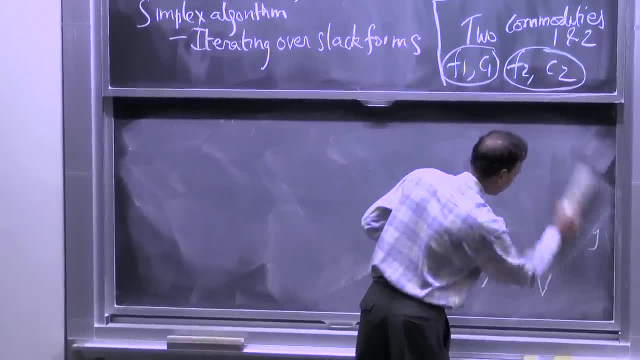 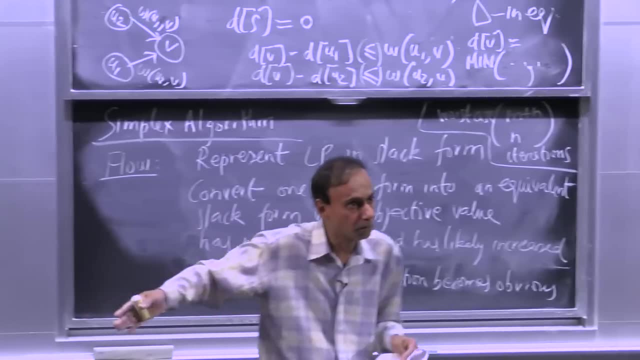 It takes about three iterations here in order to get to the point where the optimum is obvious. So you're going to convert through three slack forms And then finally, when you get to this fourth slack form, you see that you have an optimum solution. 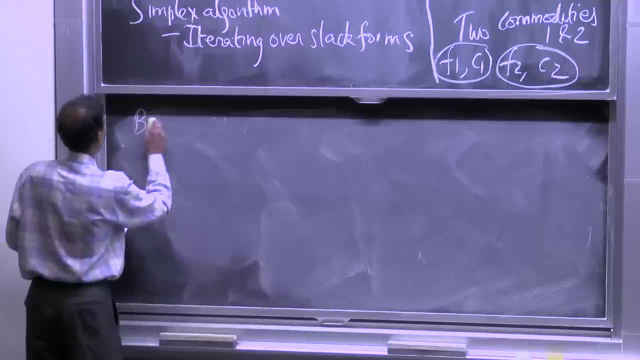 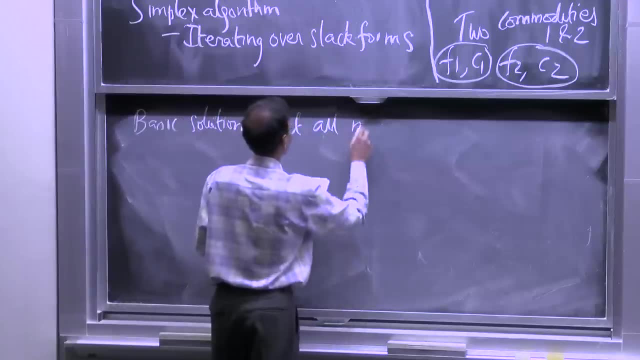 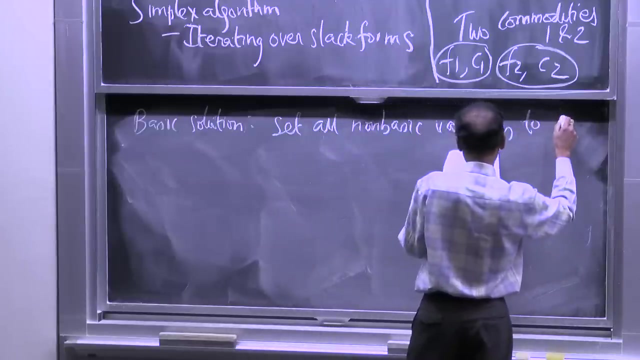 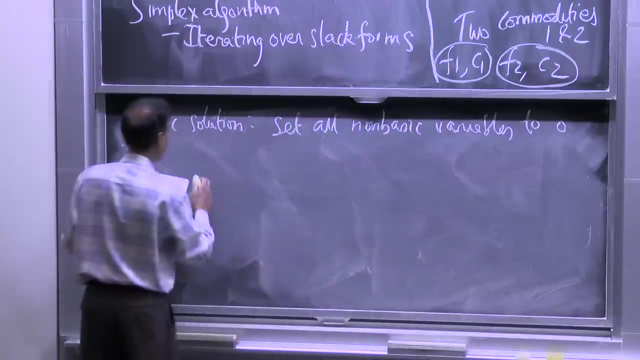 And how does that work? We're going to have the notion of a basic solution where we set all non-basic variables to 0. So in this case, what we're going to have, and then we're going to compute, We're going to have values of the basic variables. 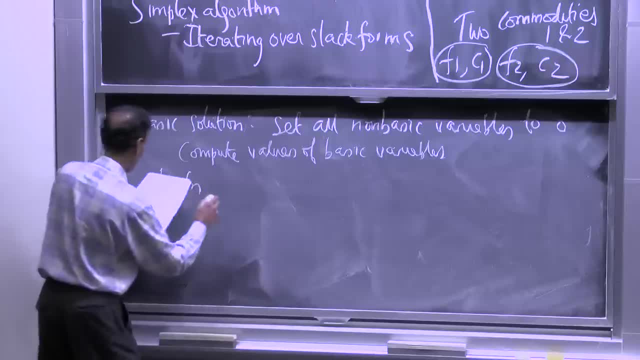 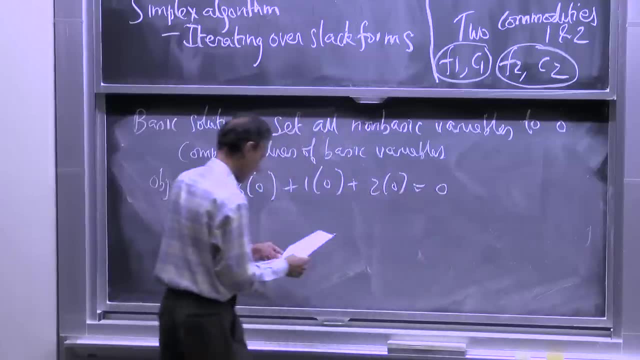 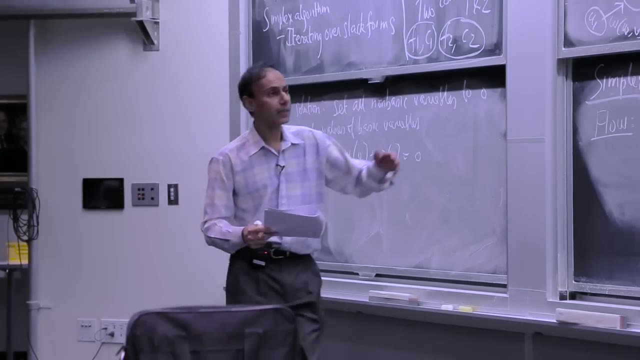 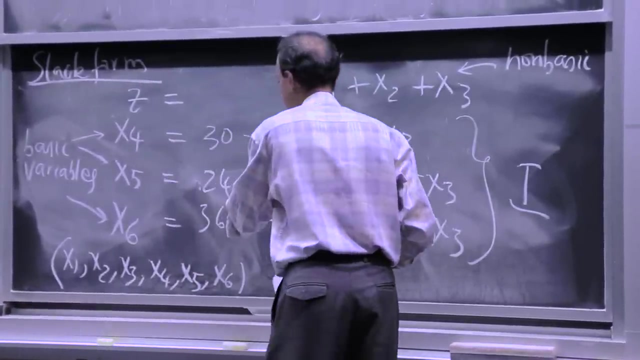 So our objective function here is going to be 3 times 0 plus 1 times 0 plus 2 times 0,, which is obviously 0.. And the values on x4,, of course, is going to be- because all of these are 0, is going to be 30.. 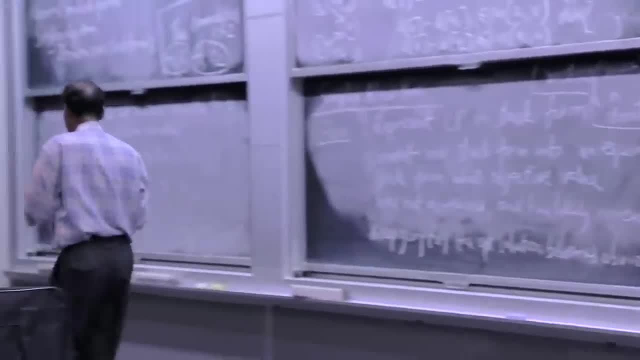 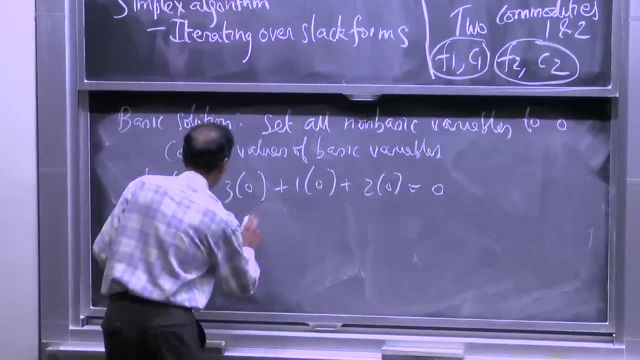 x5 is going to be 24.. And x6 is going to be 36.. So this is kind of a trivial starting point. So you can think of this as 0,, 0, 0, the solution that you're looking at- 30,, 20,, 4, and 36.. 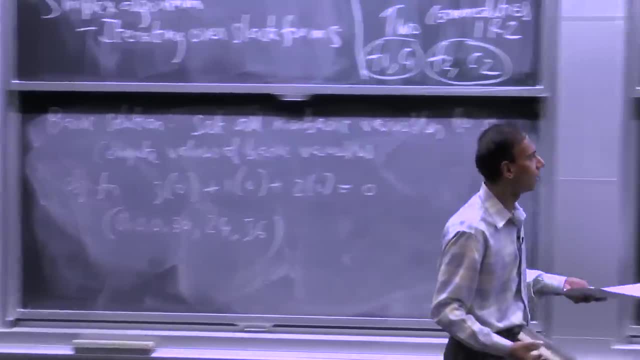 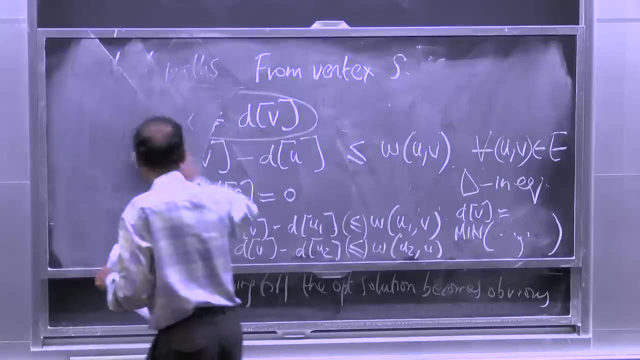 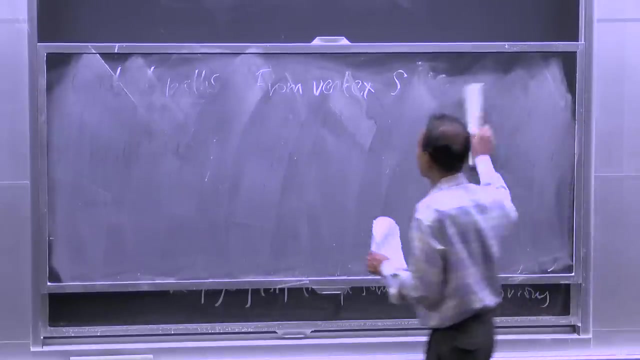 So that's our starting point, which doesn't really tell you much. But now comes the key step, Where we're going to do something that's called pivoting, And in pivoting you're going to swap a basic variable with a non-basic variable. 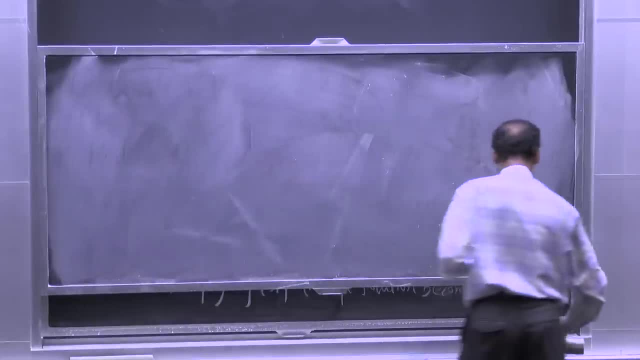 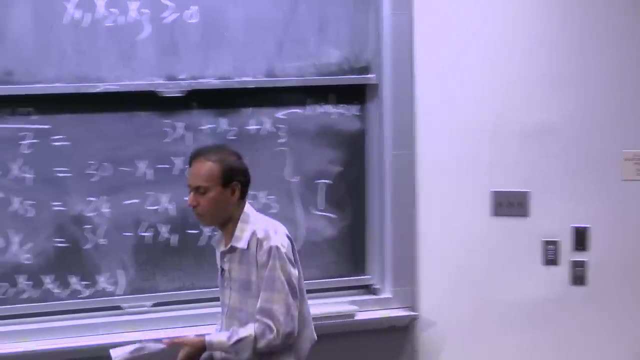 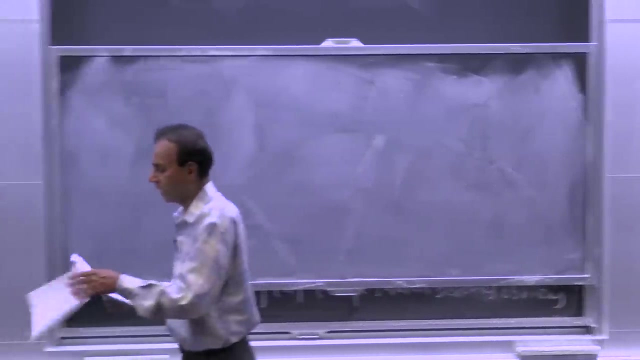 It is a step that requires some intelligence, but the basic step is a swap. So one of the basic variables is going to become a non-basic variable, and vice versa. And how do we select this? Initially, you can kind of do this. 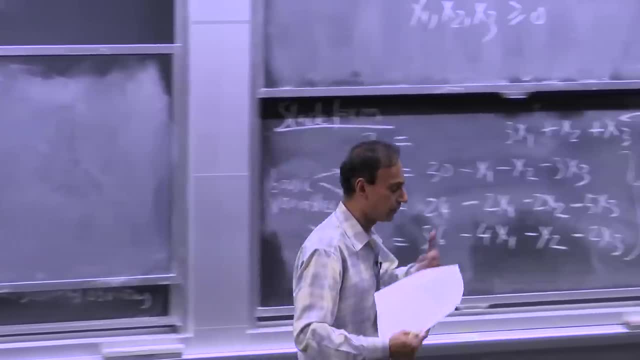 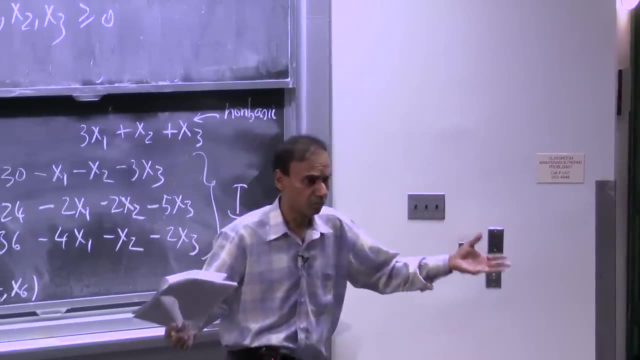 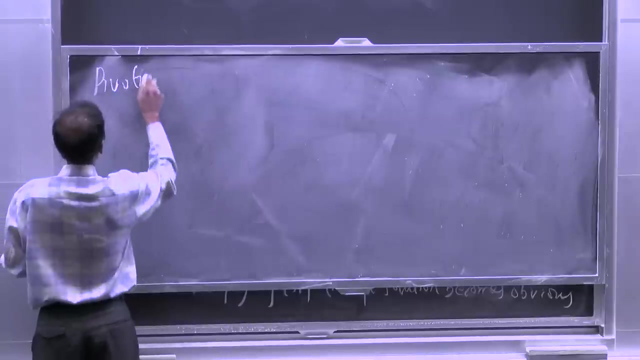 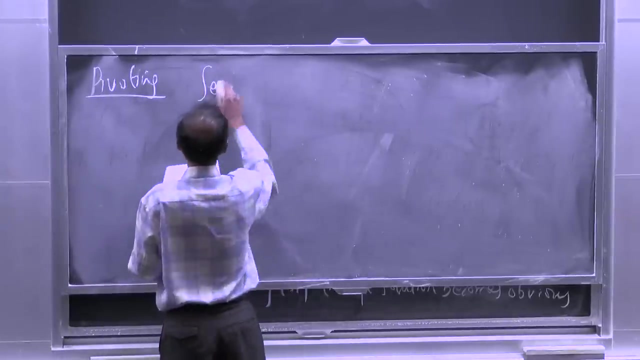 OK, OK, So we're going to do this in an arbitrary way. It gets a little more subtle as you go along. You don't want to do things in a random way, But let's just start with what pivoting actually does in a more generic setting. 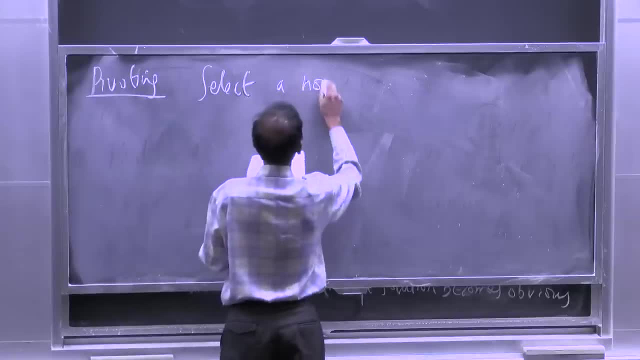 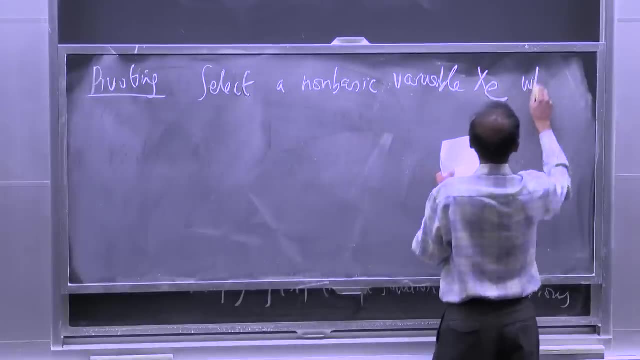 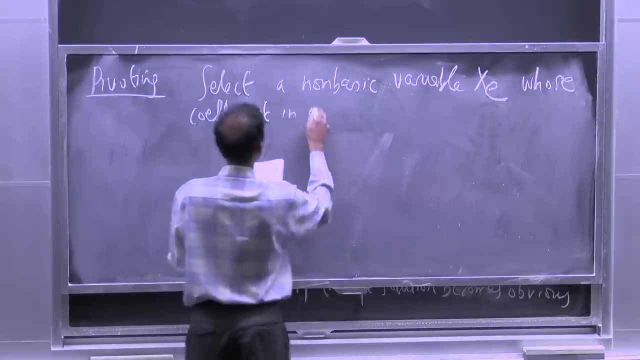 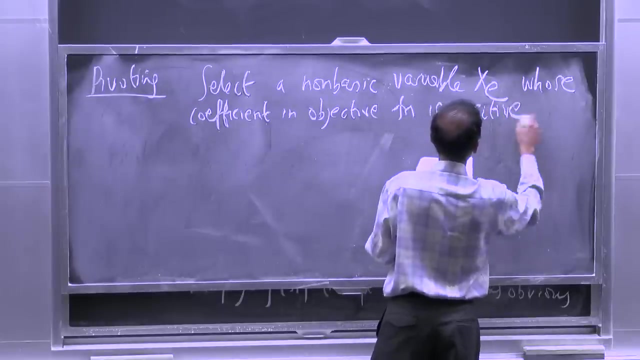 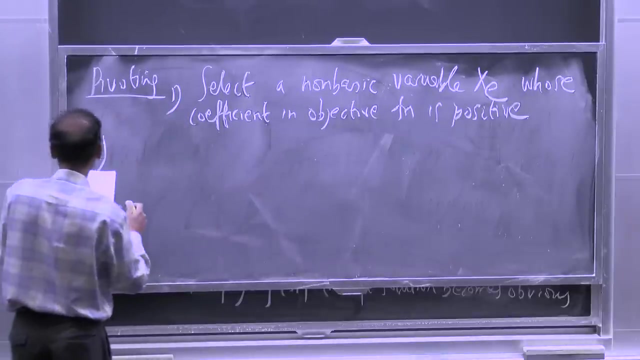 The basic step is select a non-basic variable, A variable- let's call it x sub e- whose coefficient in the objective function is positive. You can always redefine things if you can't find something like that, But we won't go there. 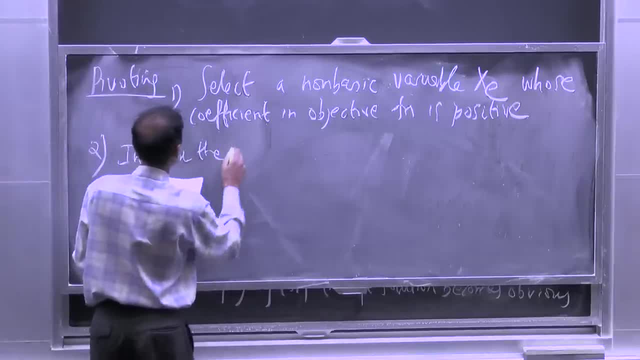 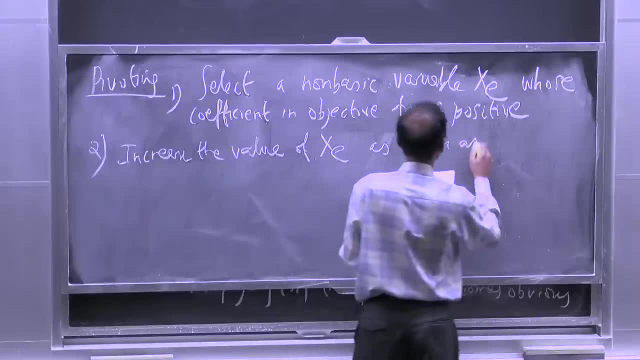 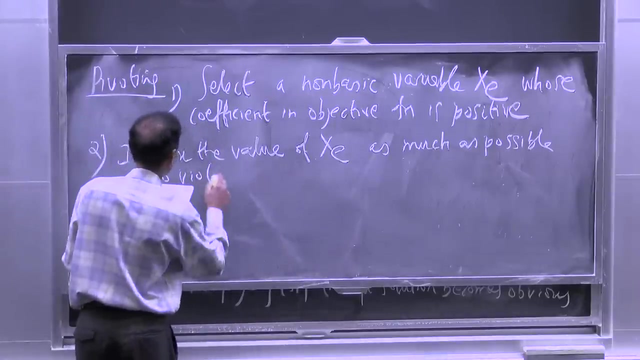 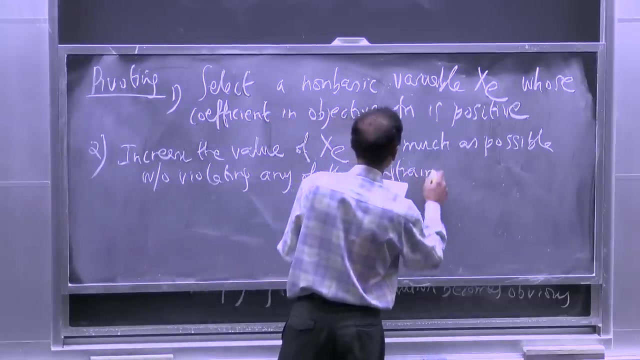 And then what we're going to do is we're going to increase The value Of x sub e As much as possible- And we always have constraints, of course, So we can do that without violating any of the constraints- And then, at this point, a variable: x sub c, b sub e. will get a constant. Let's look at the variable x sub e. Let's look at the variable x sub e. Let's look at the variable x sub e. Let's look at the variable x sub c. Let's look at the variable x sub c. 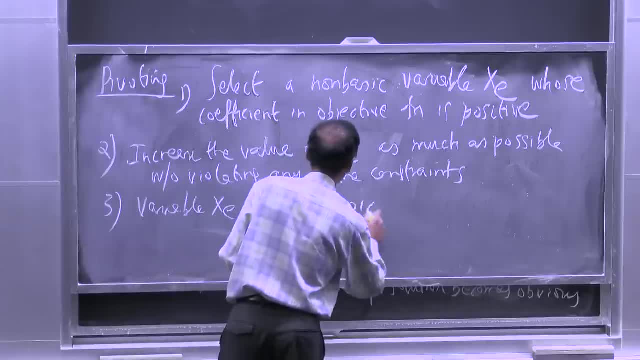 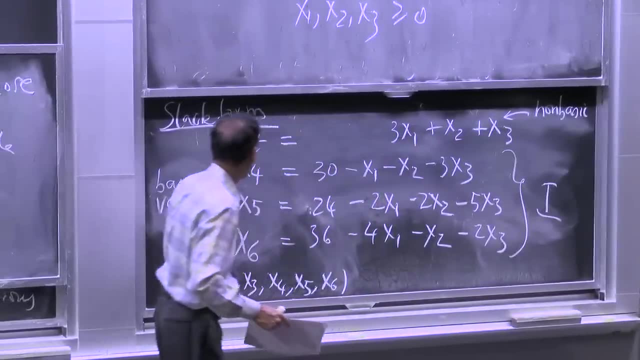 becomes basic. So it's going to turn into the left-hand side. It's going to move over. You're going to swap- The x1 might be over here And you're going to rewrite these equations so the x1 becomes basic. for example, 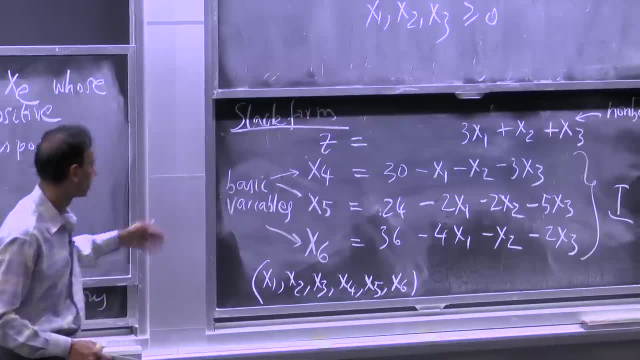 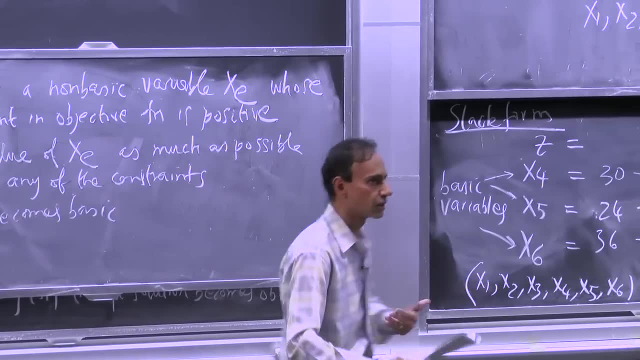 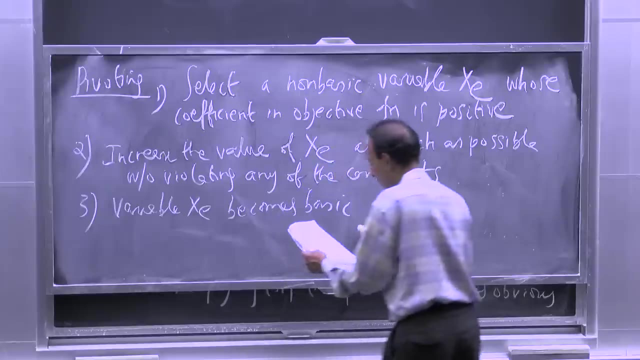 over to the left-hand side And the variable that it replaced goes over to the right-hand side. So you can think of this as Gaussian elimination, except with inequalities. There's definitely relationships there, if you recall your Gaussian elimination. If you don't, don't worry about it. 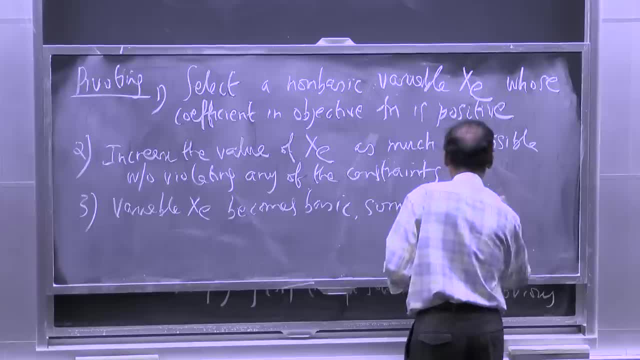 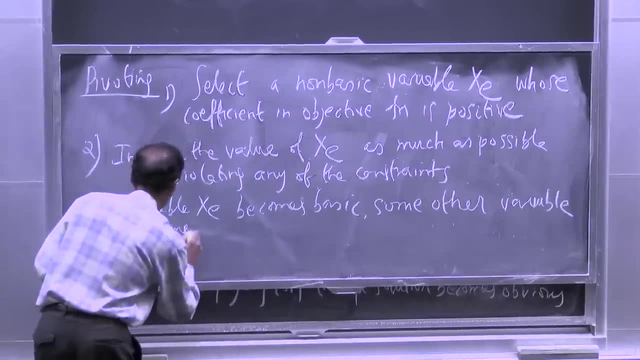 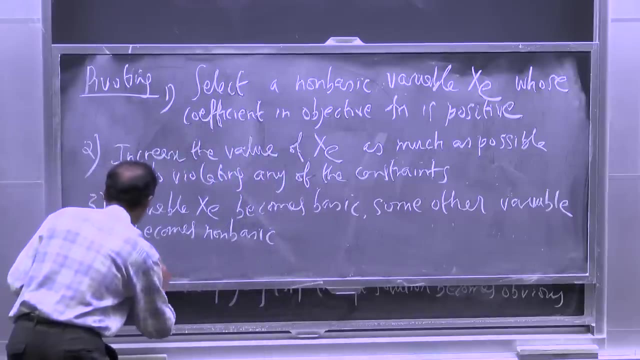 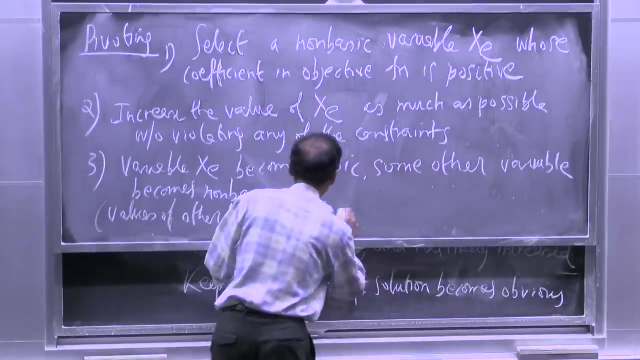 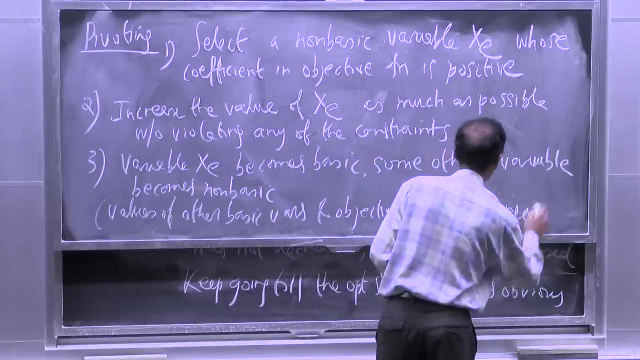 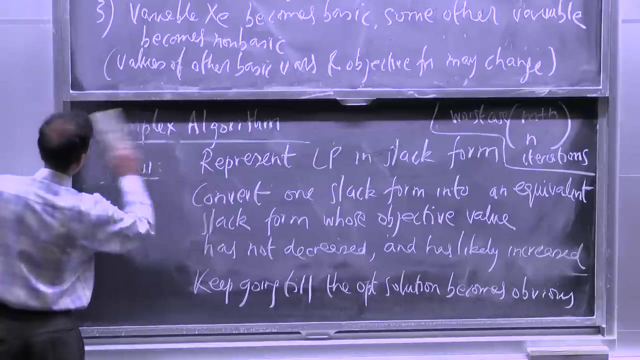 So xc becomes basic And some other variable becomes non-basic, The values of other basic variables and objective function, They may change. So we'll do one pivot step at least so you get a sense for the algebra involved And it becomes a little more concrete. 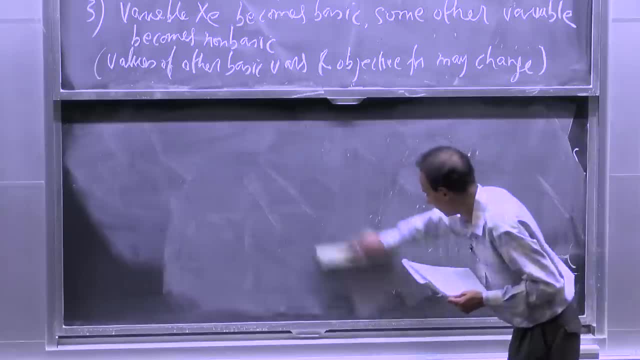 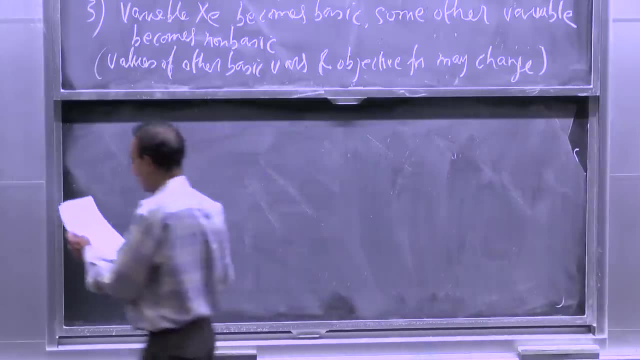 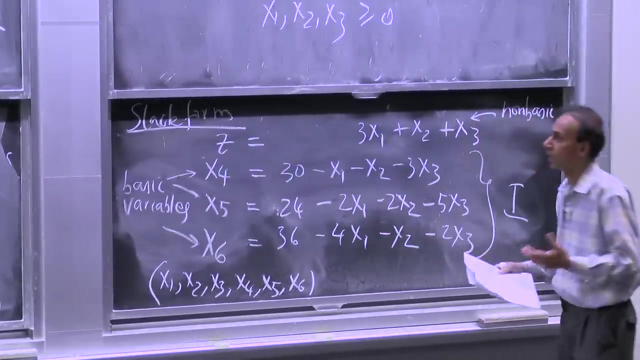 To motivate you further, you'll be doing this in problem set 8 on a different example. So what we're going to do here is we're going to select a non-basic variable, So let's just select x1.. Lexical, graphic order or numeric order. 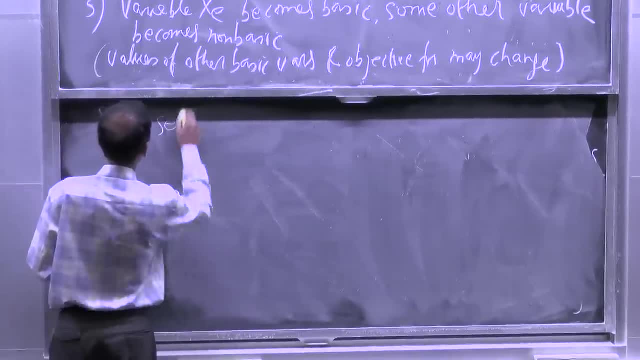 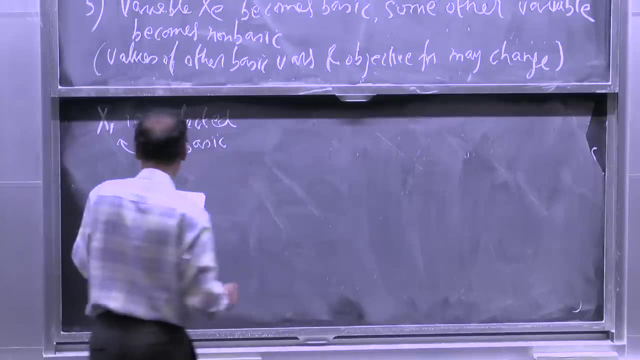 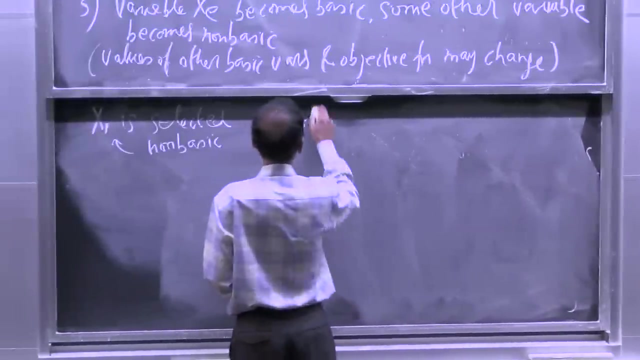 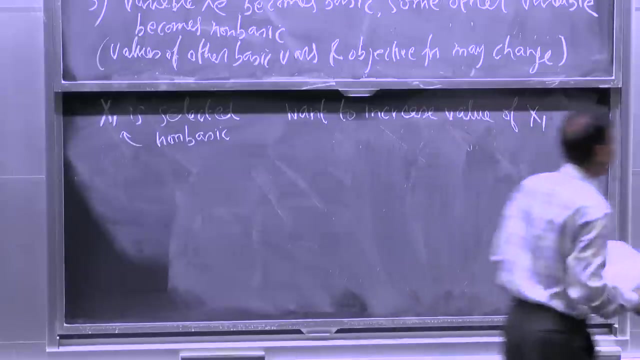 Let's select: x1 is selected, That's the non-basic variable, And what I want to do is increase the value of x1.. All right, So? OK, So I want to increase it without violating constraints. Now, which of these constraints do you? 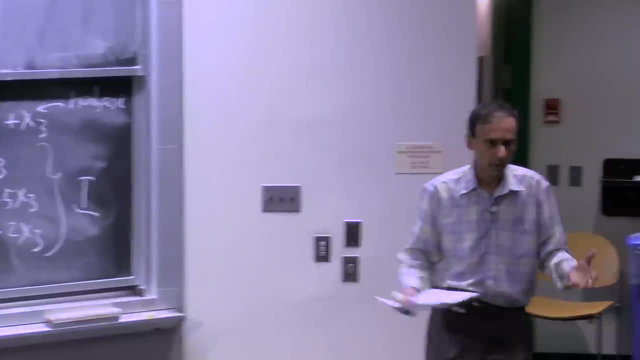 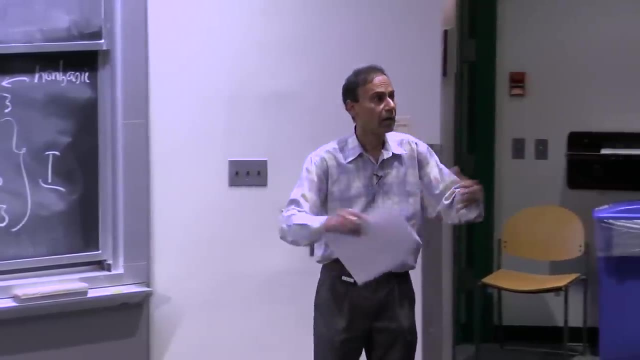 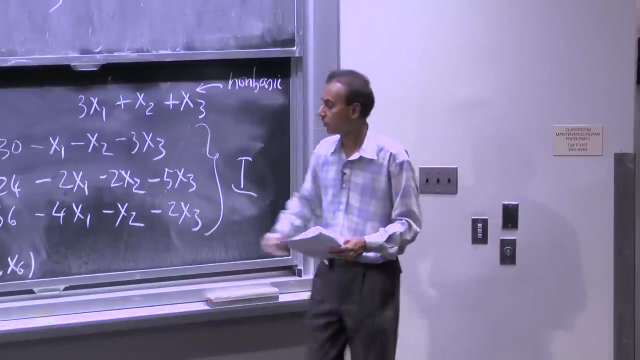 think is going to cause trouble. first, with respect to increasing the value of x1? x1 is now 0.. Right, We're at a ground level. We have all 0s. Things are feasible. Now, as I start increasing x1, remember you have non-basic 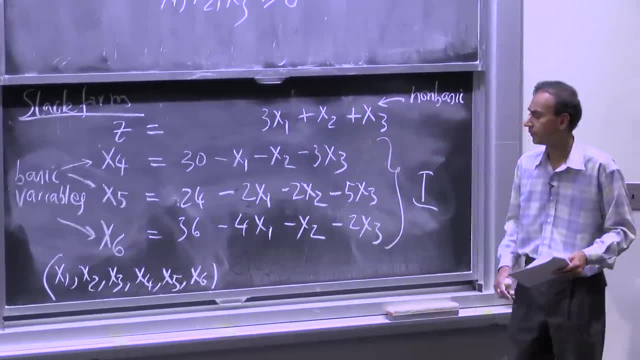 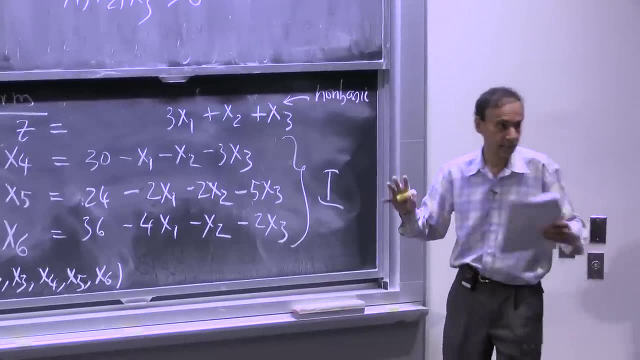 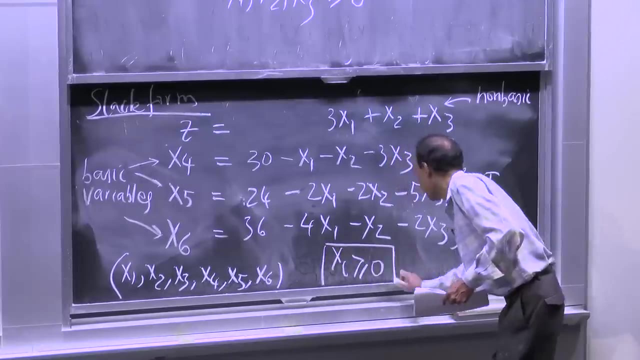 Remember, you have non-negativity constraints associated with each of the x4 values as well. That's what these basic variables represent, So don't forget the fact that the constraints are violated. You need all the xi's to be greater than or equal to 0.. 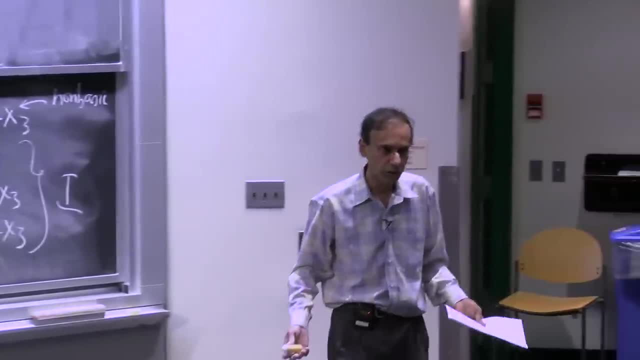 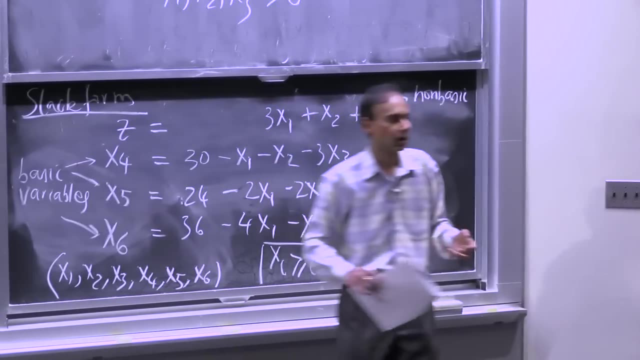 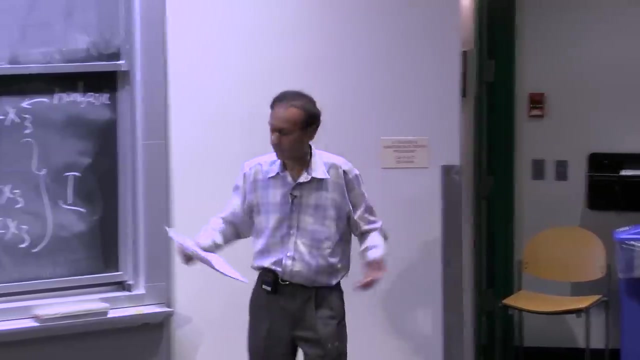 That was true for the non-basic variables. It's also true for the basic variables. So a violation of a constraint implies that one of the currently basic variables goes negative Right. That's exactly equivalent to the original inequality not being satisfied. So which of these constraints do you? 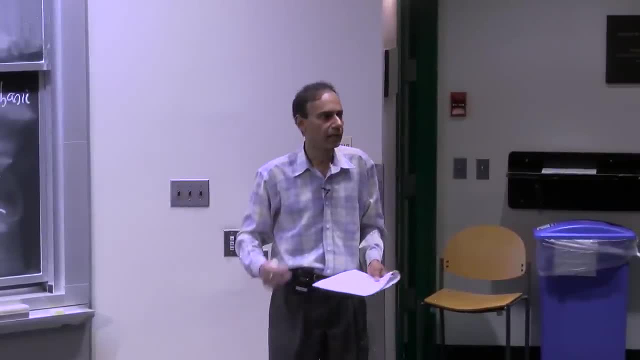 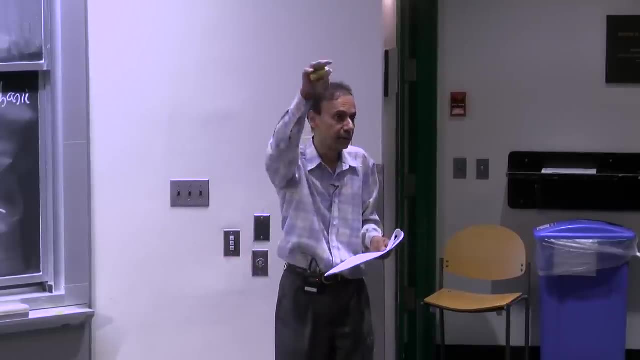 think is going to cause trouble here. Just look at it and should be able to look at the three equations and tell me, as I increase the value of x1, where am I going to hit my limit x6.. Yes, absolutely correct. 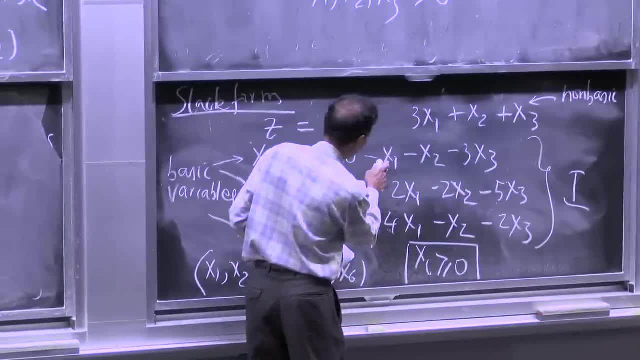 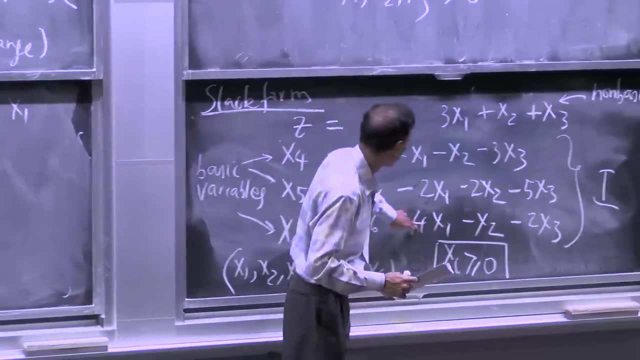 So that's because of the minus 4 here. This is a big multiplier. I got a minus 1 here, a minus 2 here and a minus 4 here, And if you just look at 4, the magnitudes 4 is bigger than 2. 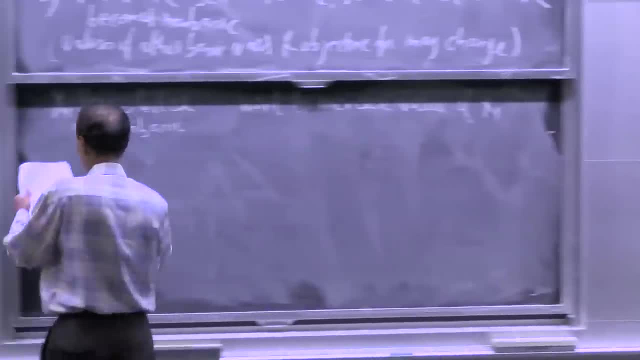 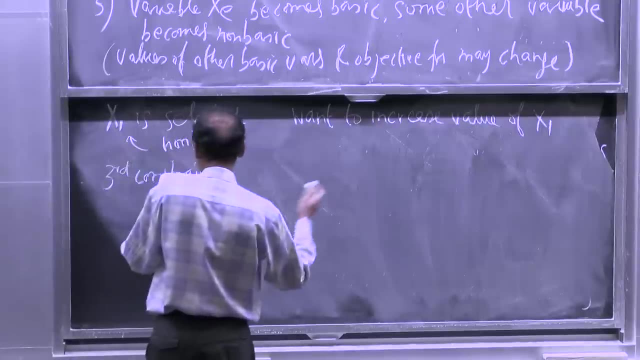 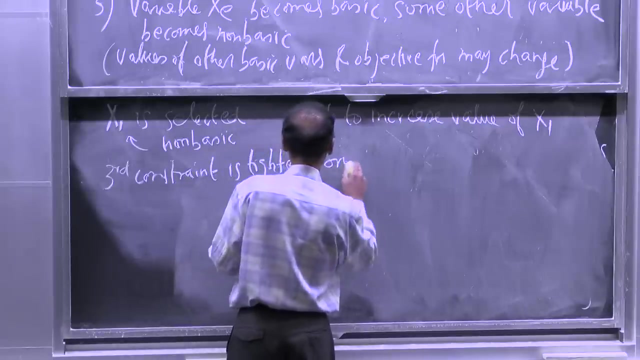 and it's bigger than 1.. So it's going to be that third constraint. So, third constraint: you can obviously compute this numerically or mechanically. It was just easier to do this in this example by eyeballing it. And so third constraint is the tightest one. 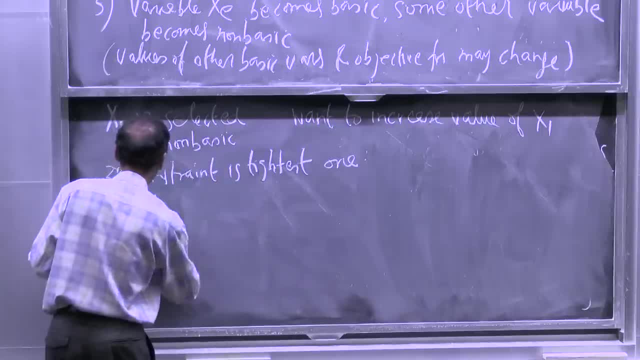 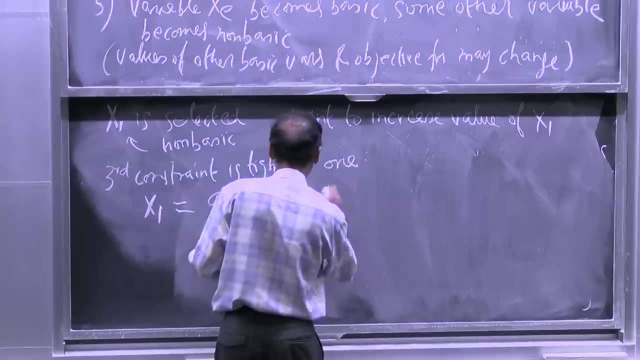 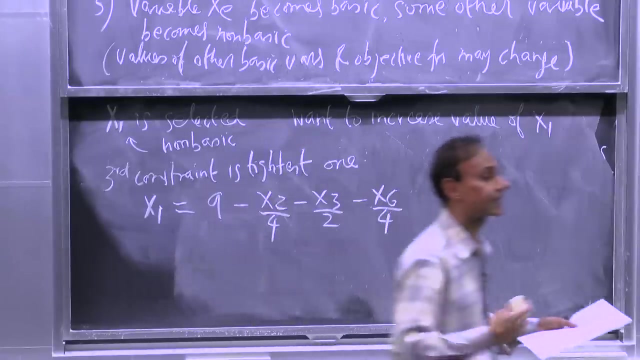 And it limits how much we can increase x1.. So I'm going to do my second step up there. This corresponds to rewriting on x1 as these other variables, And now I got x1 on the left-hand side and x6 on the right-hand side. 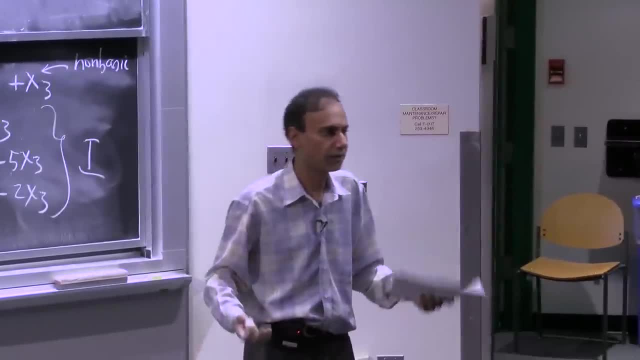 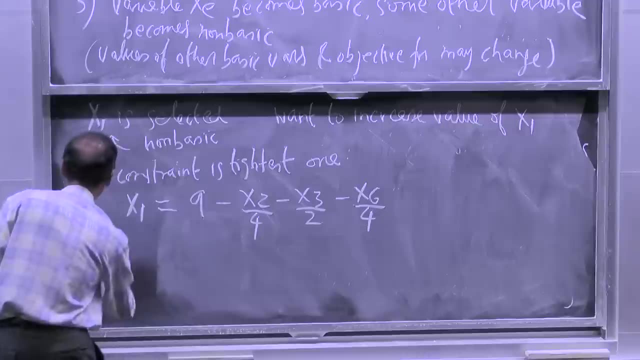 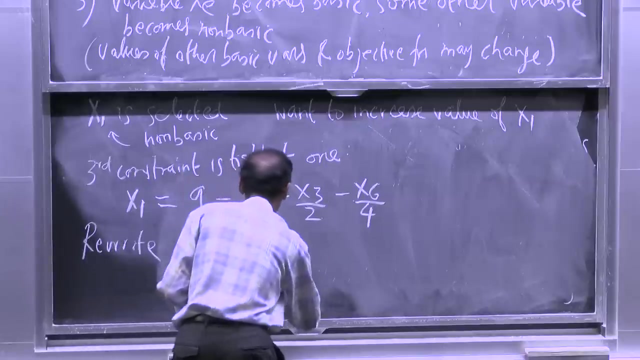 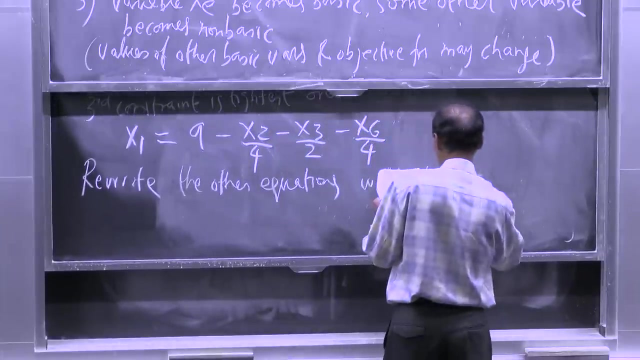 And now it's just merely a matter of substitution. Once I've done this, I'm just going to jam through and go in And I'm going to rewrite the other equations. OK, So I'm going to replace x1 with x6 on the right-hand side. 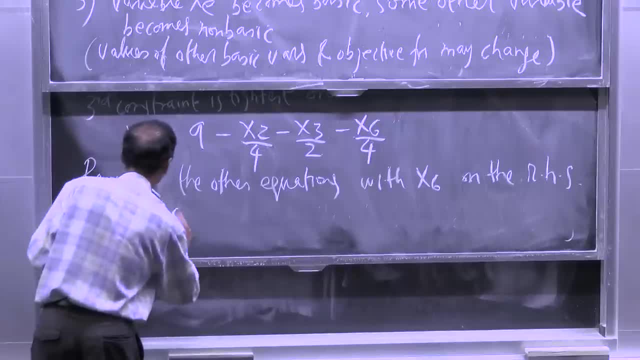 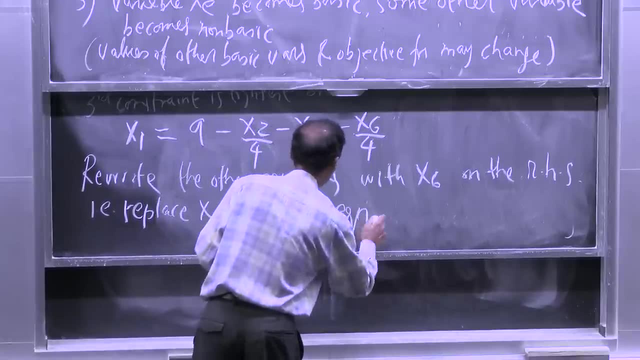 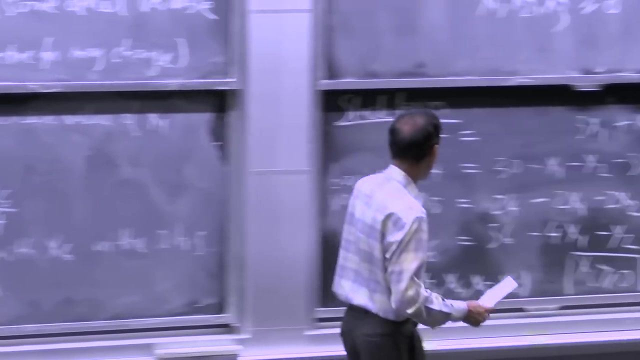 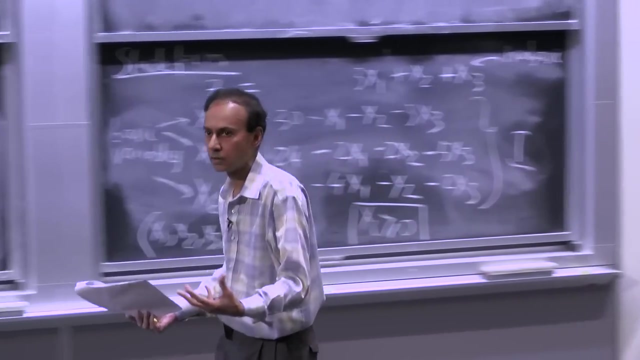 And that is I'm going to replace x1 with the above equation. That's really a simple substitution. So at this point, what's happened is because the third constraint, representing x6, was the one that was chosen. what's happened is that x1 and x6 are going to interchange roles. 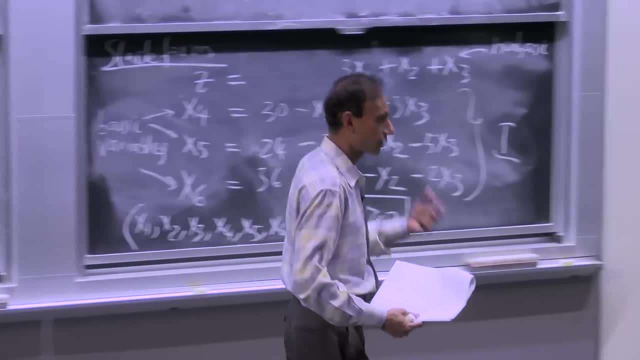 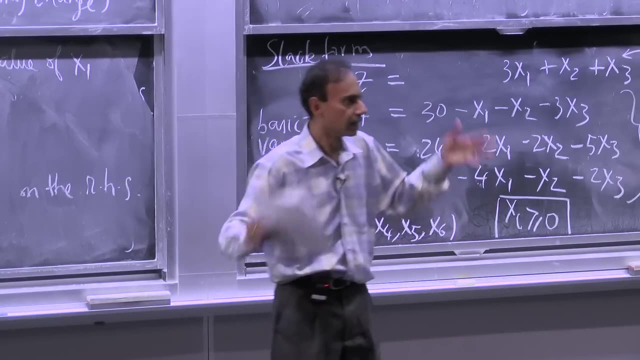 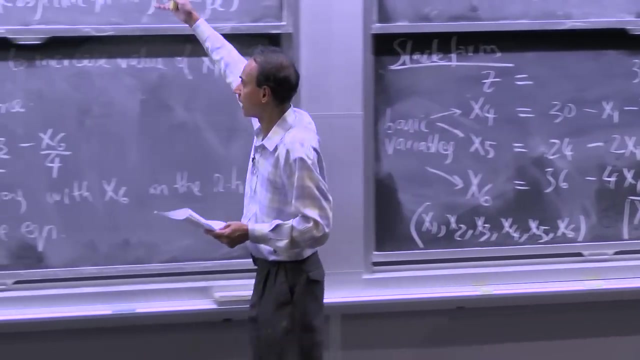 x1 was non-basic, It's going to become basic, x6 was basic And it's going to become non-basic, And that's basically the essence of the simplex algorithm: The iteration and then the convergence, and all of that is, as I mentioned, going to require getting to a point where 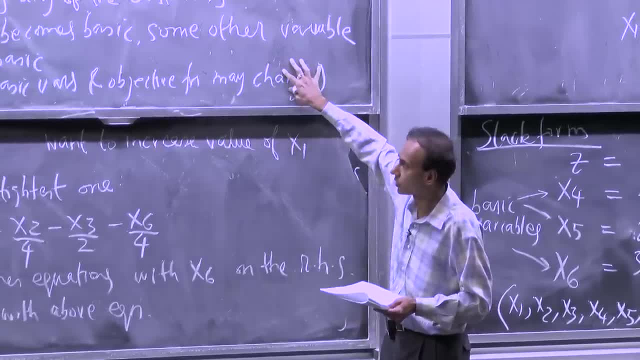 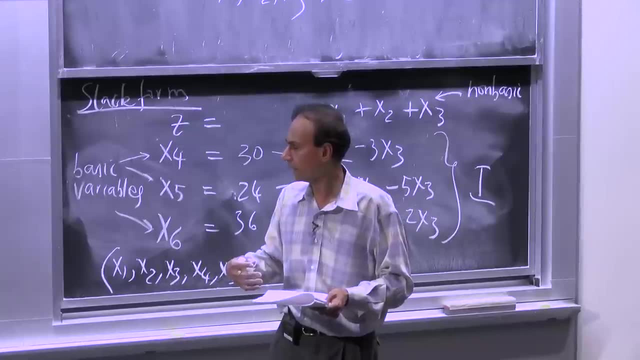 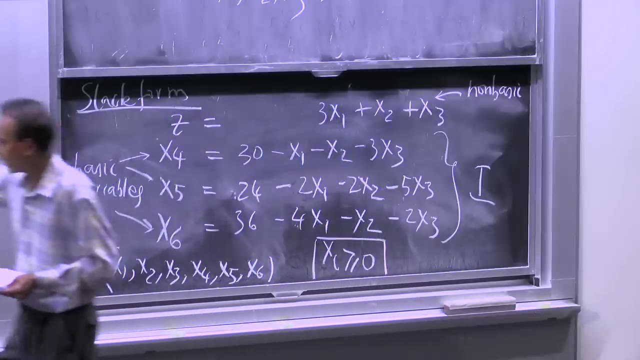 the optimality is obvious. but we won't be doing any proofs corresponding to convergence for simplex or any other specific LP techniques in this class. Maybe some constraint techniques. I take back what I said, but certainly not for simplex. But I just want to give you a sense for the flow here. 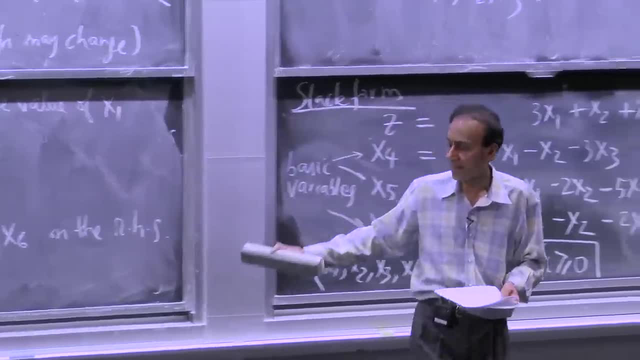 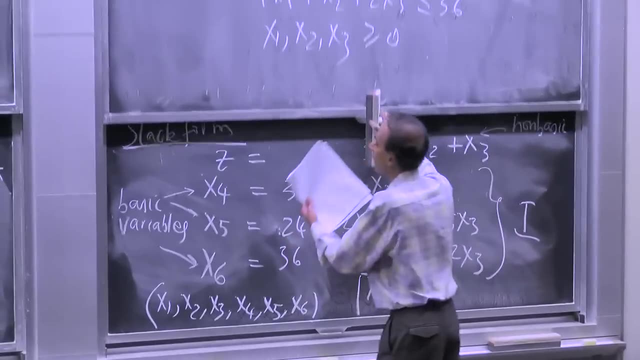 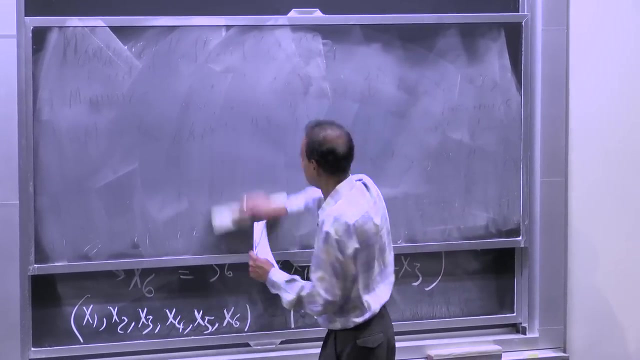 And so let's just go through this last thing here in terms of finishing off the pivot exercise, OK, OK, OK, And I want to show you what the equations look like. And if you just keep doing that, at some point you'll converge. 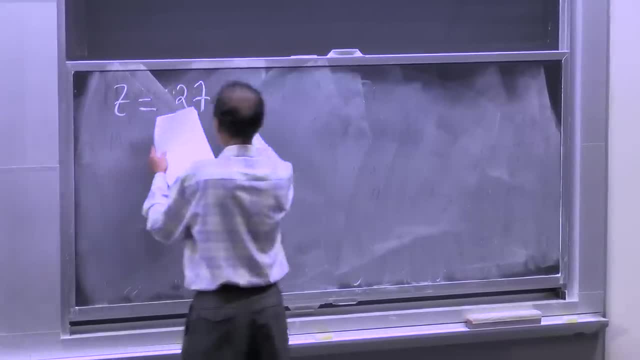 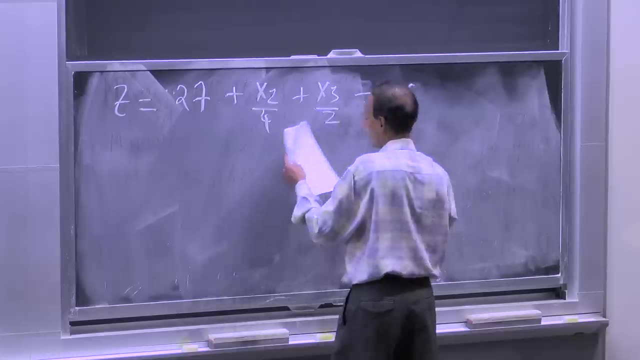 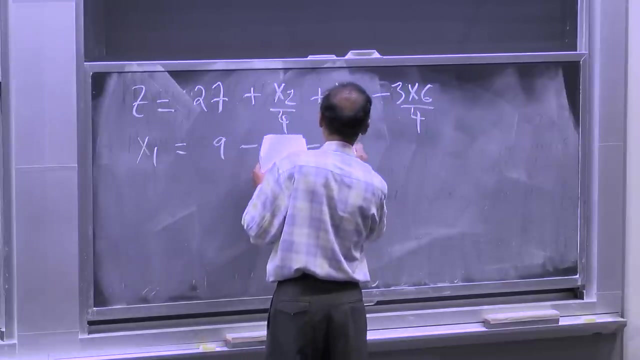 And so what happens here is you have z equals 27 plus x2 divided by 4, plus x3 divided by 2, minus 3x6 divided by 4.. x1 equals- There's a bunch of algebra here that I'm obviously skipping over. 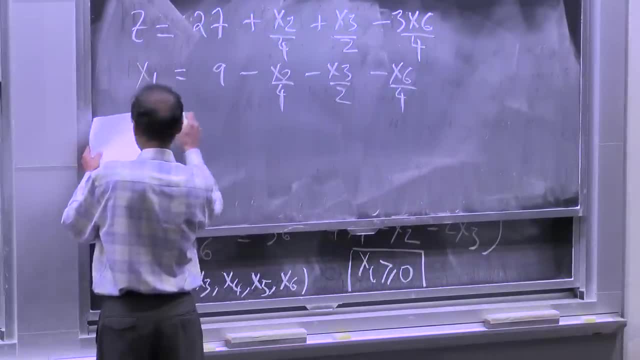 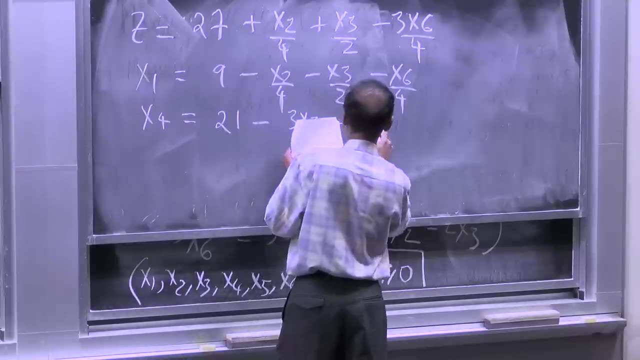 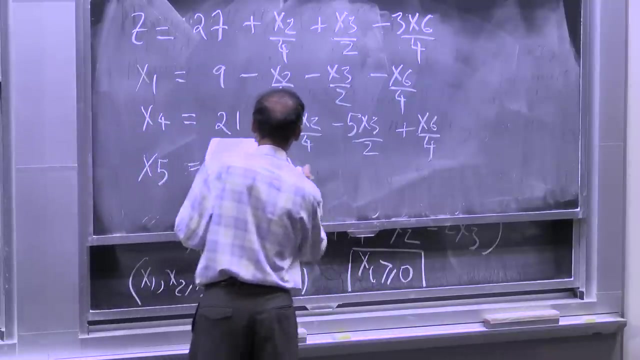 but it's simple algebra, And I have x4 over here, 21 minus 3x2 divided by 4, minus 5x3 divided by 2, plus x6 divided by 4.. And then one last thing here, OK. 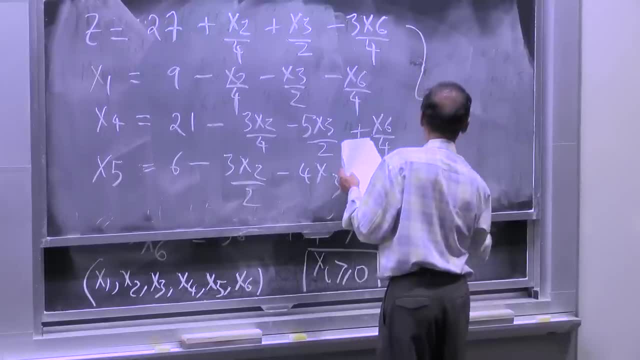 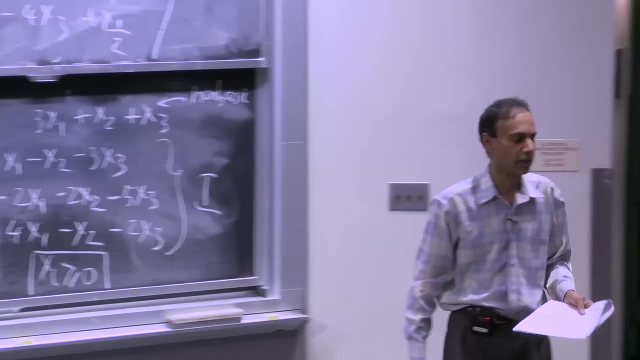 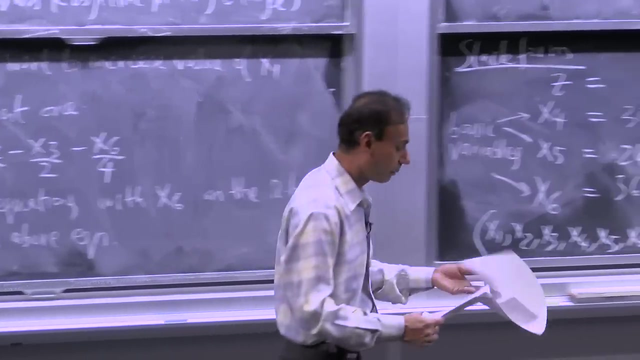 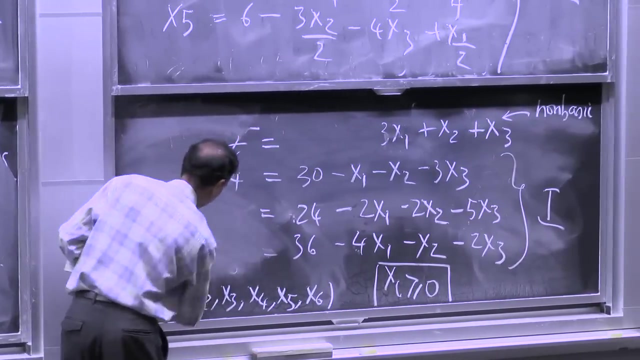 So that's my pivot step, where I've flipped x1 and x6.. So now you ask: what was the point? What was the point of this? Well, the point of this was that you actually increased the objective function value, and in this particular case, quite significantly. 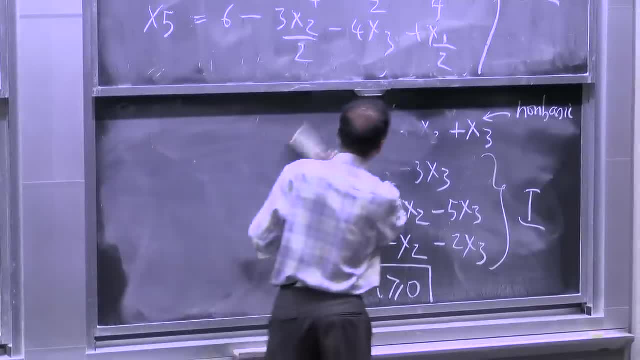 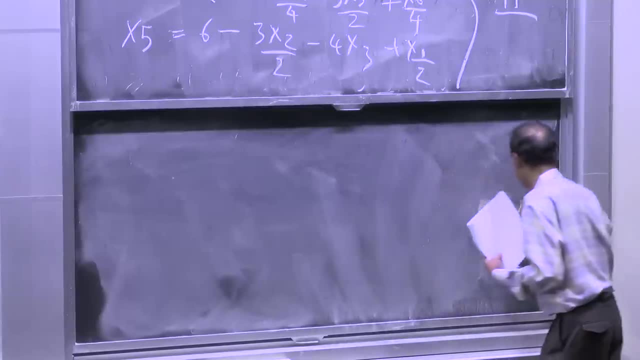 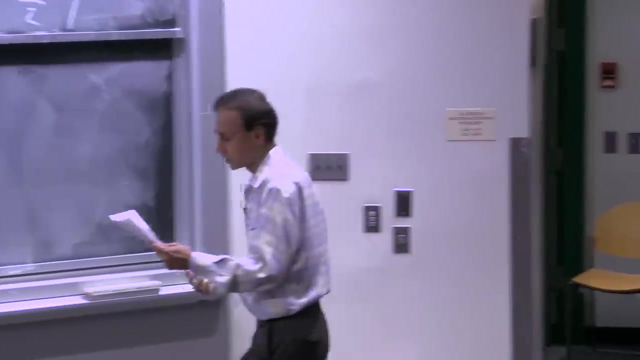 while maintaining correctness. And so let me just, OK, Make these observations and conclude here, because then that gets us to the point where you've seen the details of one pivot step and you can imagine applying it over and over to convergence, And let's just say, let's just look. 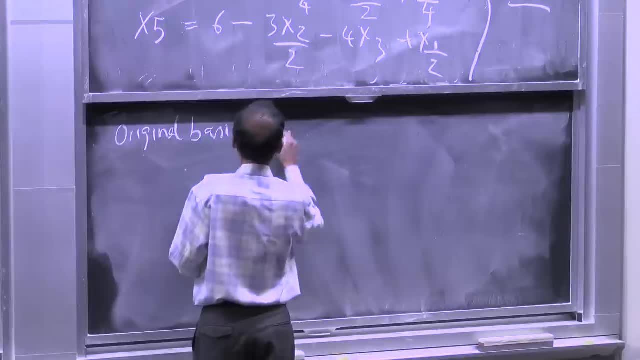 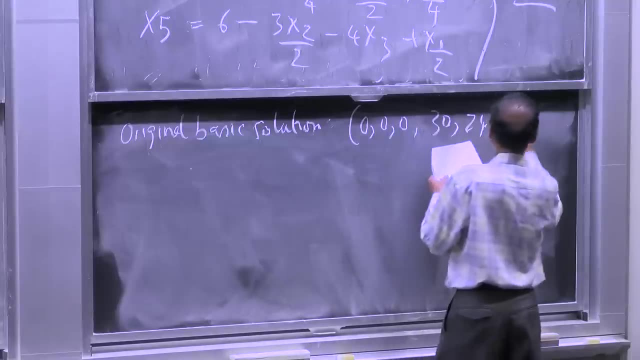 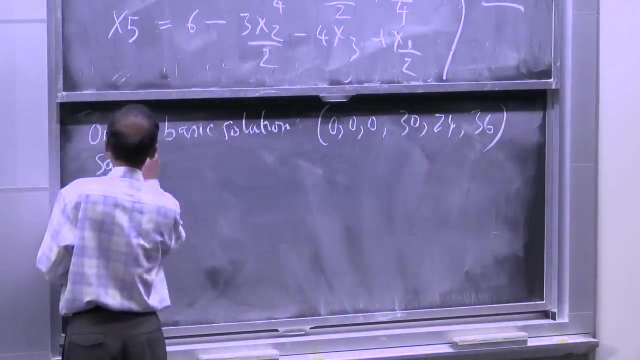 at the original basic solution which, as you recall, was 0,, 0,, 0,, 30,, 24, and 36.. And this is simply x1 through x6.. This original basic solution certainly satisfies these equations. equations 2,. 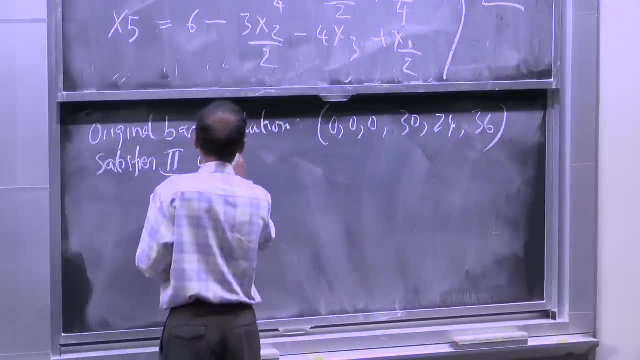 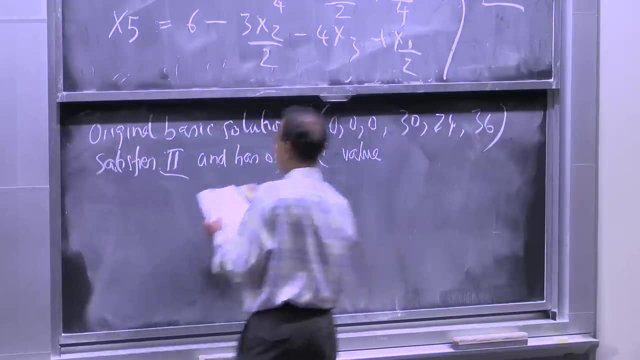 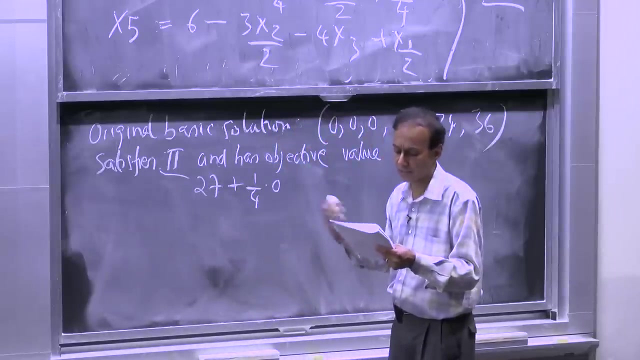 if you just put them in there And it makes sense that it would have the objective value of 0,, given equivalence. But you can verify that by seeing that you have 27.. The original had the objective value of 0, because all the x1,. 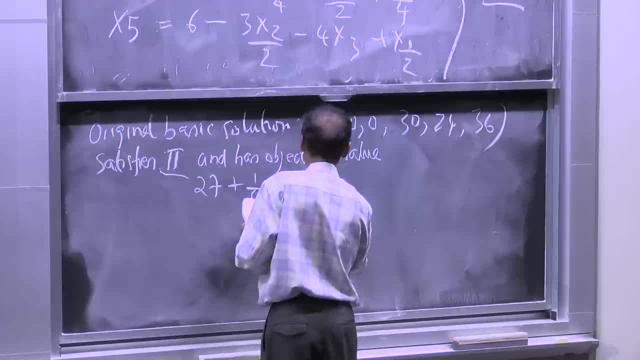 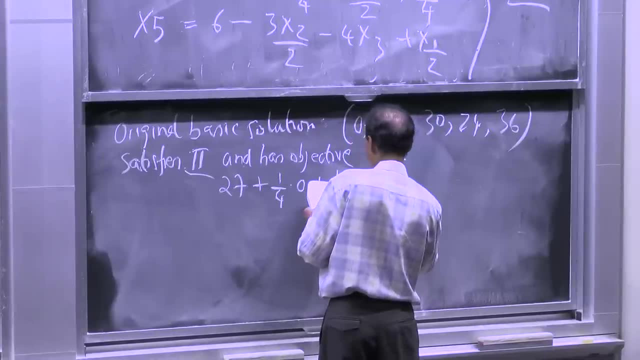 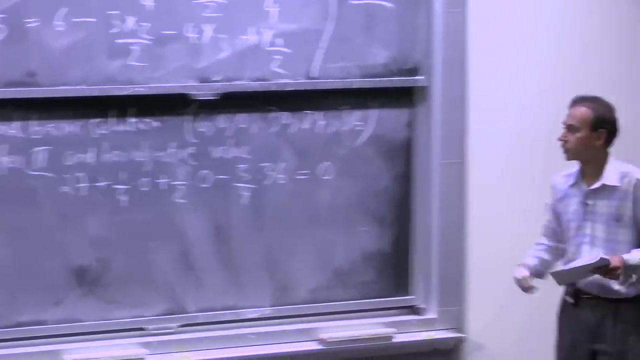 x2, x3 were 0.. So that was an easy check in the set of equations corresponding to the first set, which I've erased at this point. But no matter. And if you look at what I have here, I have 36 equals 0. 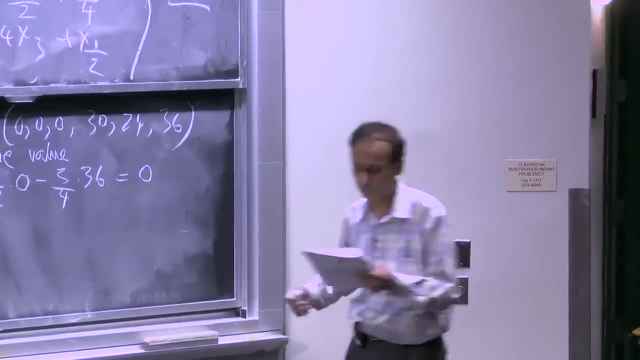 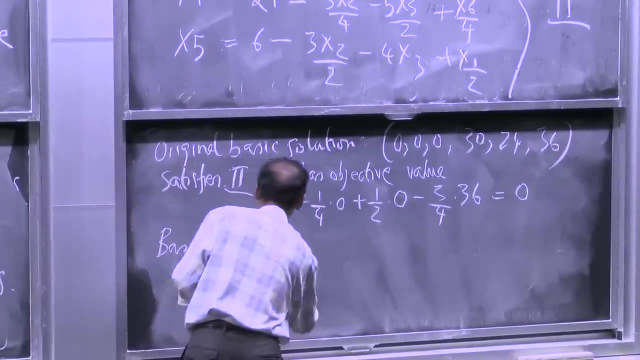 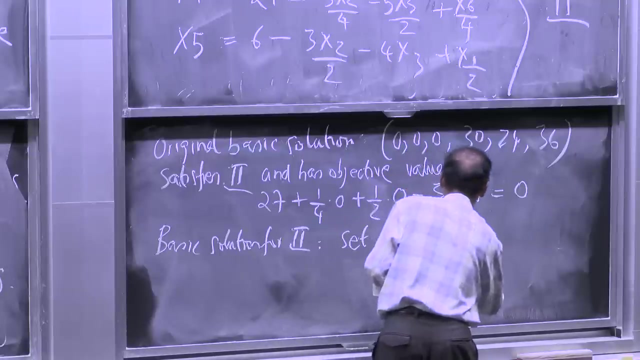 So the objective value here is 0. It matches what you had before. But the basic solution for 2, I'm going to say, is set the non-basic values. So what is the solution here? The non-basic values are 0.. 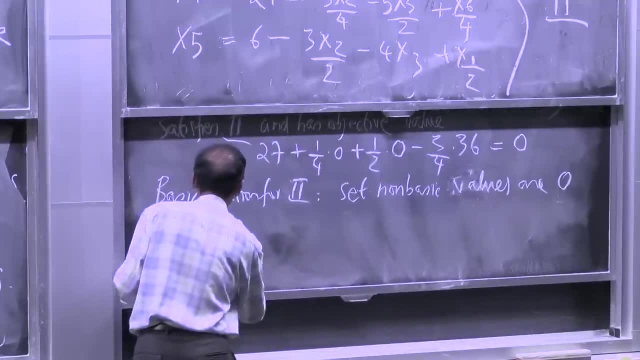 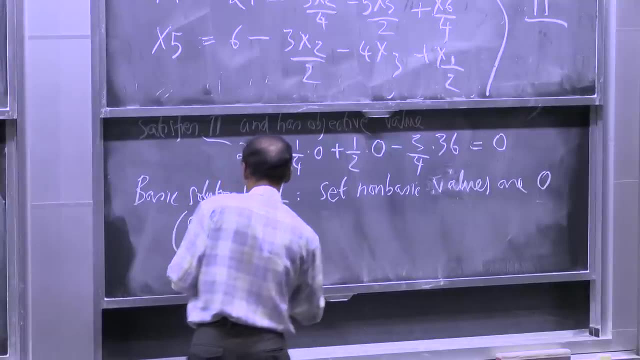 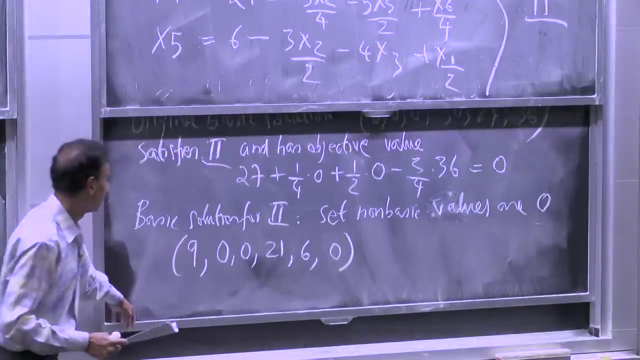 So the solution is going to be 9, because 9 is non-basic. x1 is now non-basic, x2 and x3 are still basic, And then I have 21 and 6. And x6 now has become basic. 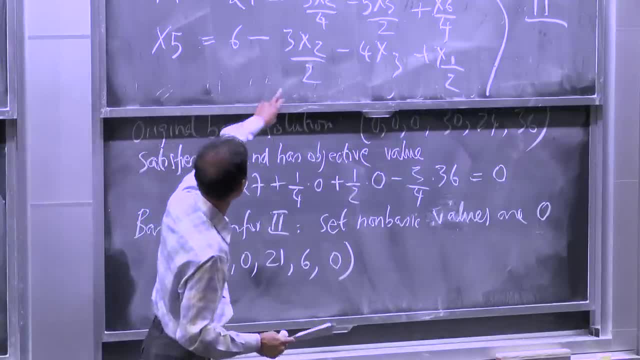 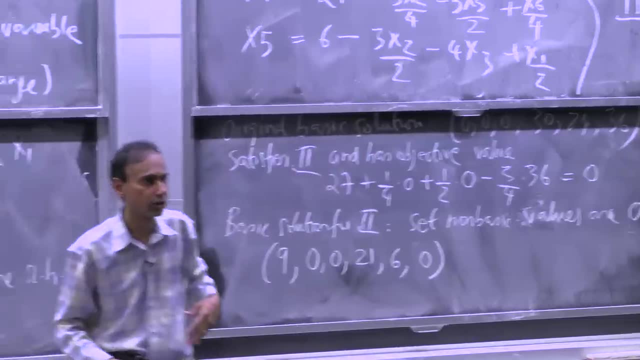 So the way I get the solution is simply by plugging in 0s on this side, and I get 9,, 21, and 6. Because I just plugged in 0s on the right hand side. So that's how I got a new solution. 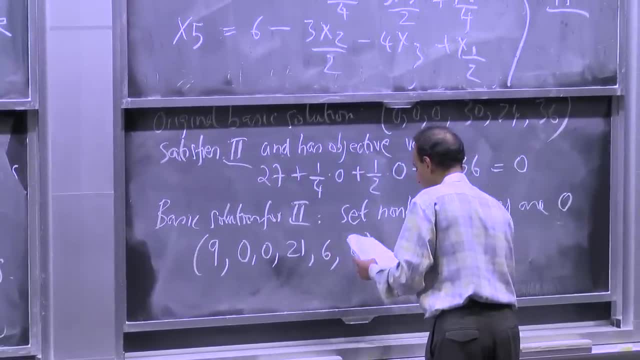 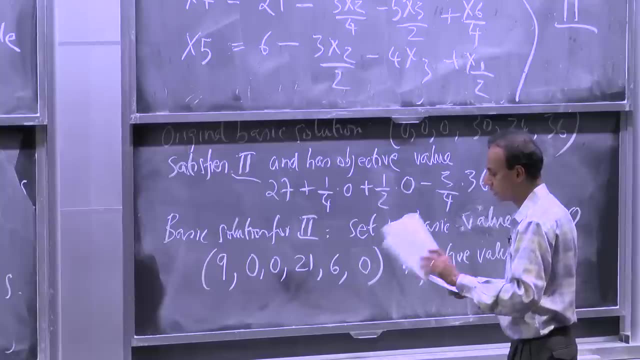 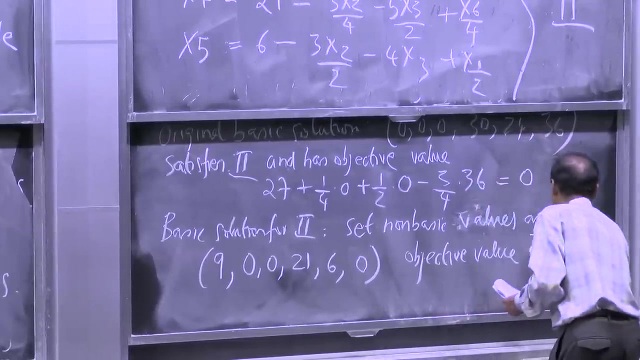 And if you look at the objective value for this, the objective value, you can look at this objective value simply by looking at the original problem, And the original problem had 3x1.. So you have 3x1 plus x2 plus x3 as the objective value. 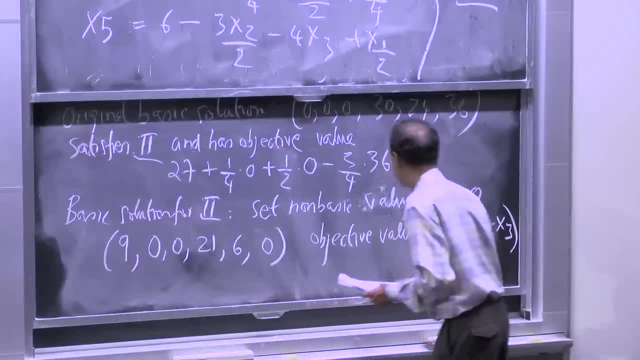 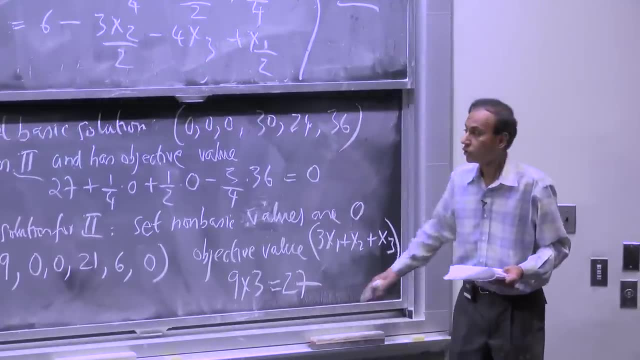 And so if you go off and you see, well, you had 0s for the other ones, But you have 3 times 9.. So you have an objective value of 27.. So this flip of our pivot basically got you from an objective value of 0,. 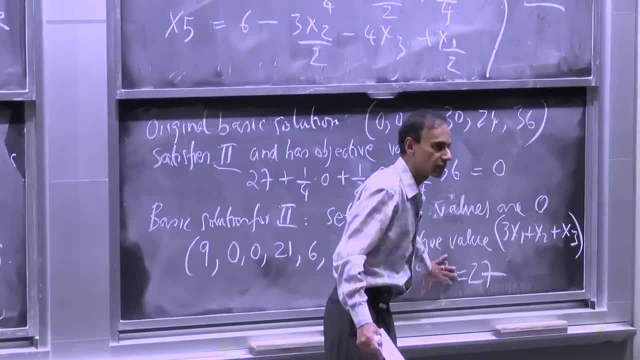 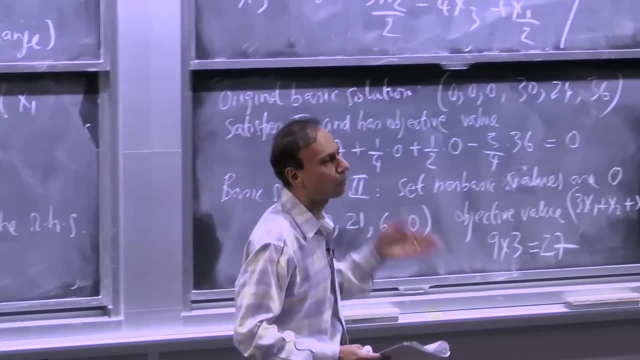 while maintaining correctness to an objective value of 27.. OK, And You can look at this in the notes or in CLRS, But you have to do two more pivots corresponding to two other variables. the same grungy stuff. 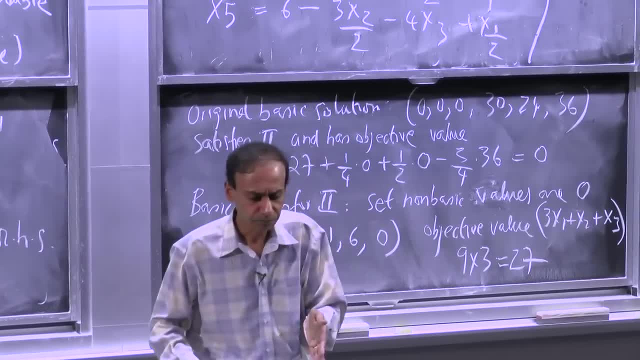 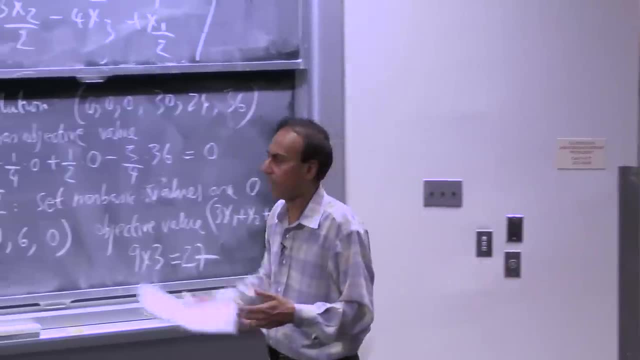 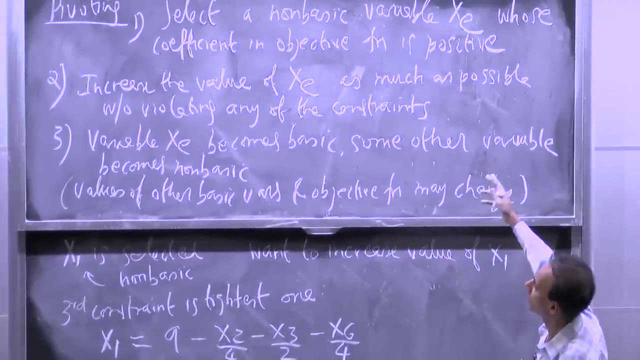 that I went through here, substitution after selection, And the objective value is going to increase. And you might ask: how do I know that I'm done Right? And so that was the last thing here, which is increase the value until it becomes obvious. 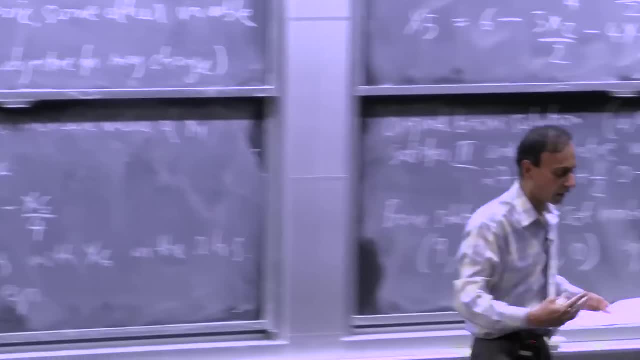 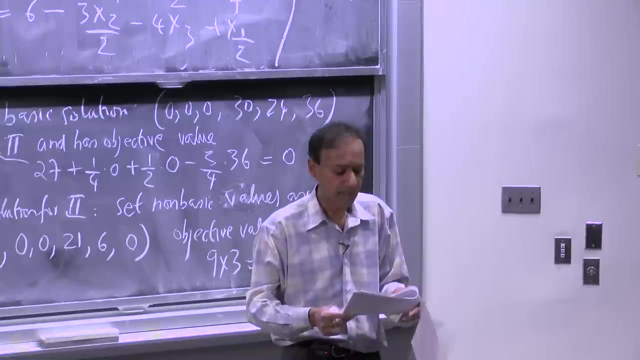 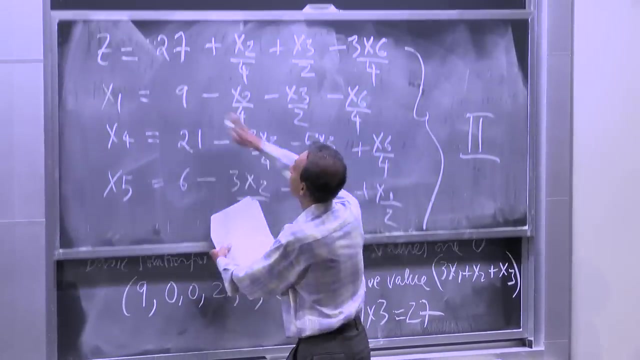 No, this is pivoting, I'm sorry. Increase the value until it becomes obvious what the optimum is, And what ends up happening is you end up with an objective function, in this case, The objective function. mind you, This thing over here is the objective function.